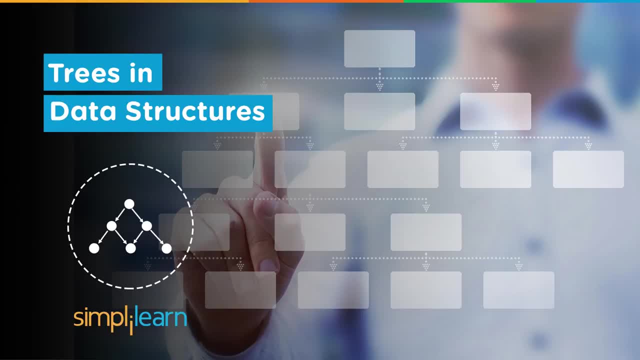 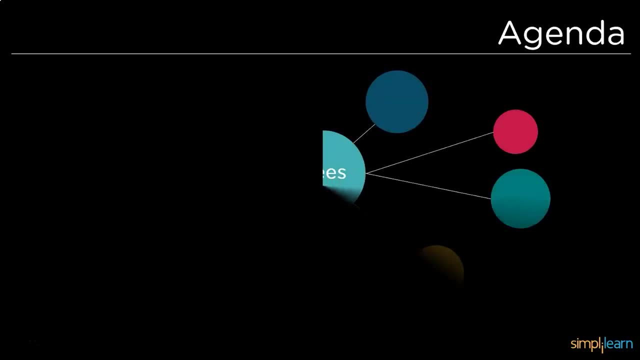 And don't forget to hit that bell icon to never miss an update from Simply Learn Now. without any further ado, let's get started with the agenda for today's session. Today we will be discussing trees in data structures. So first we will understand what exactly are trees in data structures? 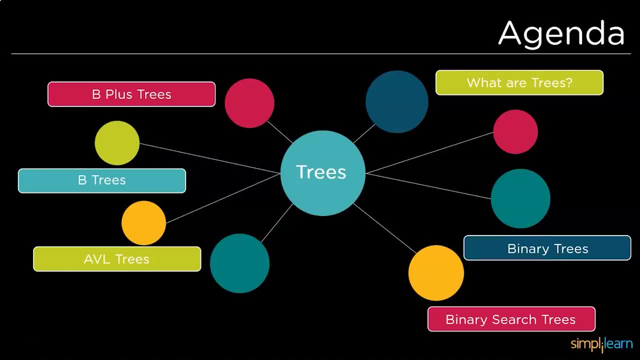 Followed by that, we will understand the first type of trees in data structures, which are the binary trees. Then, moving ahead, we will learn the binary search trees in data structures, Followed by that we will learn the abl trees in data structures. 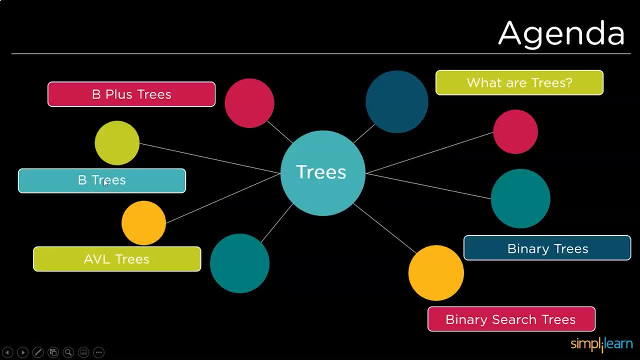 Next we have b trees in data structures And finally we will wind up the session by discussing b plus trees in data structures. Hope I made myself clear with the agenda. Now let's get started with our first topic. Over to our experts. 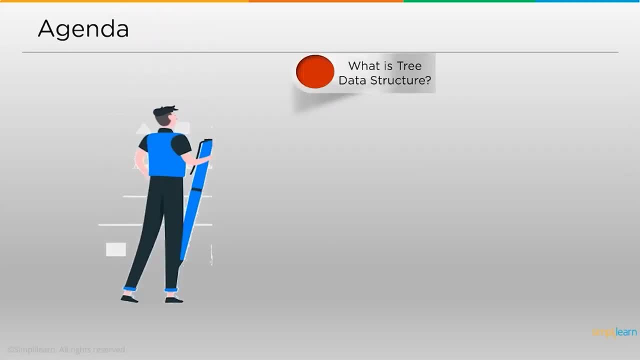 So we will be discussing what exactly is a tree data structure, Followed by that we will understand why we need a tree data structure. Then we will learn the tree terminologies, Followed by that we will understand tree node. 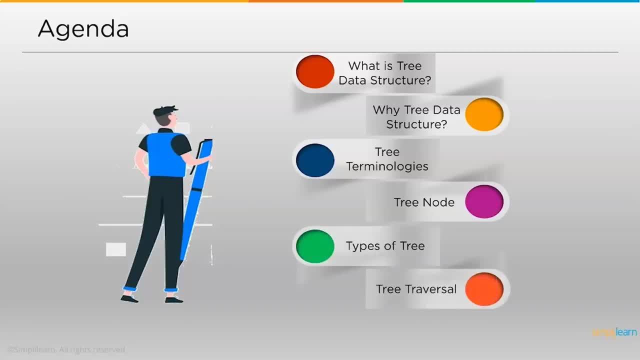 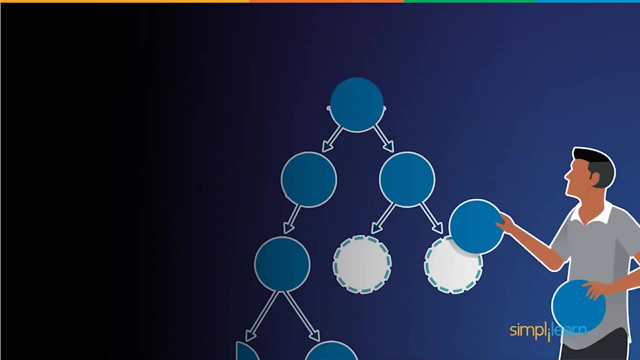 Then we will see the types of trees And followed by that we will understand the tree traversal And finally we will see some applications of trees in real time. I hope I made myself clear with the agenda. Now let's get started with the first topic, That is, what is a tree data structure? 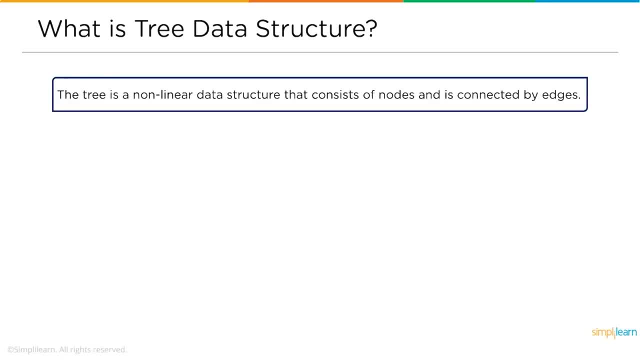 So what exactly is a tree data structure? The tree is a non-linear data structure that consists of nodes And is connected by edges. I know it's a little difficult to understand just by the definition, So let me show you the pictorial representation. 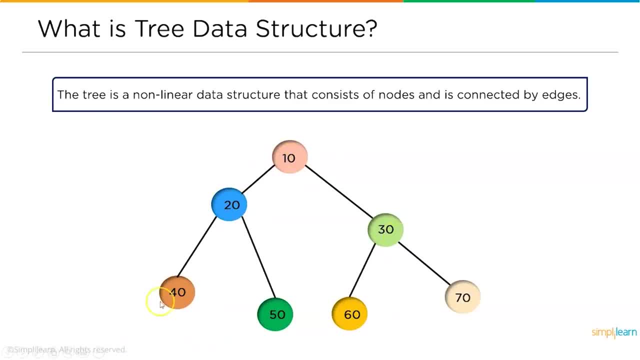 As you can see, we have the elements, That is, 10,, 20,, 30,, 40,, 50,, 60 and 70. And all these are stored in the tree data structure. They are stored in a non-linear structure. 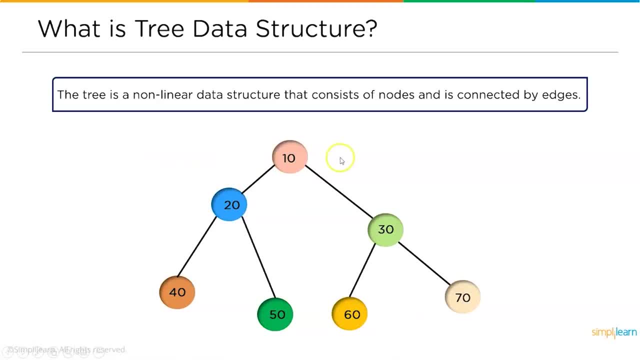 If we had used arrays, it would have been in a linear, consecutive way Where 10 starts first and 70 ends at the last position. Now, in the next section, we will discuss why we had made to a switch to the tree data structure. 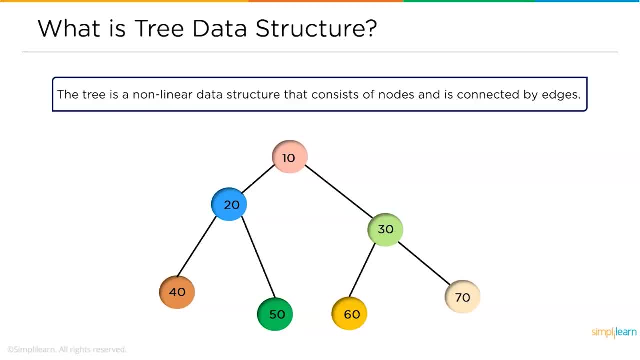 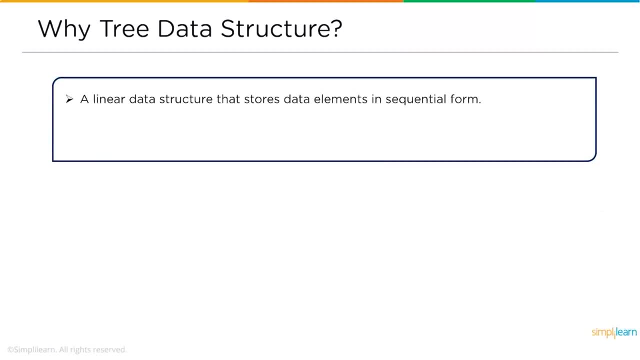 When we already had a linear data structure, That is array, Now the next topic. That is why we need tree data structure. So there are many reasons why we had switched into tree data structure, And one of the reasons is a linear data structure always stores the elements in a sequential form. 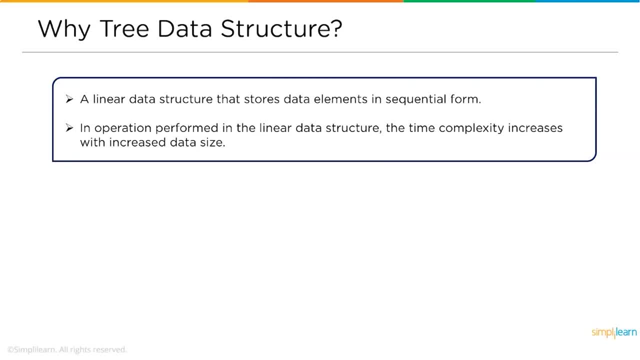 That is one after the other. And in operations to be performed in linear data structure, the time complexity increases as the data size increases. You can see here that, as discussed before, the elements are stored in a linear form. That is 10 at the first place and 70 at the last place. 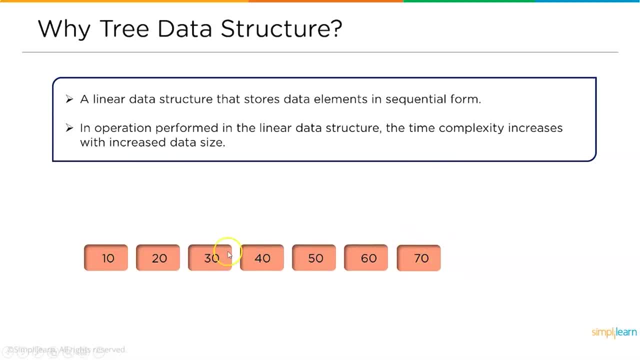 Imagine you wanted to access the element 70. Then, using the traversal, you had to start from the first position, That is, 10, 20,, 30,, 40 and slowly at the end is 70. So accessing that particular element is really time consuming. 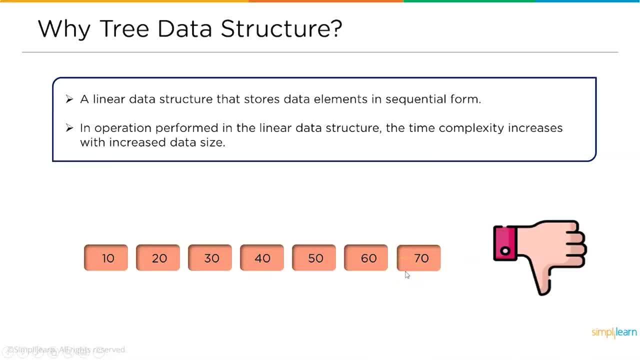 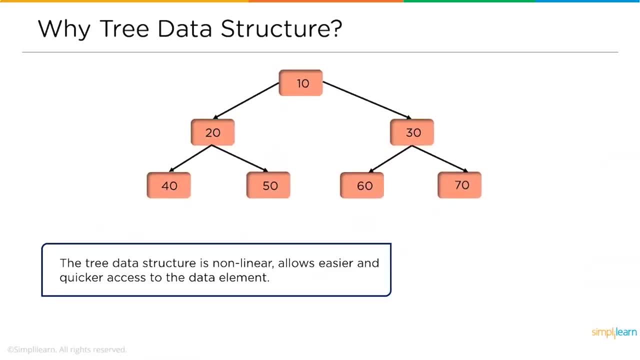 We are facing this just for 70 elements. Imagine if we had 700 elements, Right? So that is exactly why we had made a switch to tree data structure And using tree data structure we have many advantages, As the tree data structure is completely non-linear. 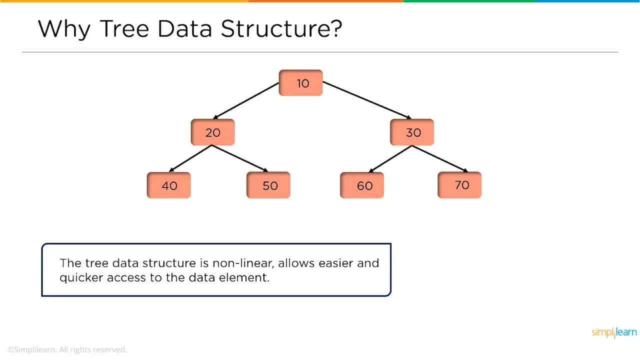 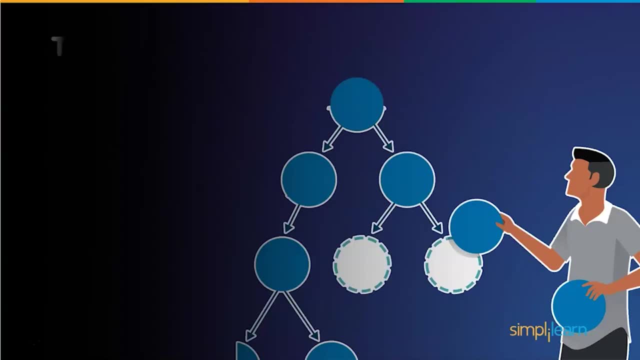 And it allows easier access and quicker access of the data elements. How is that possible? We will look into it in the next segment, where we will discuss about the traversal of trees. Now, before we understand the traversal of trees, we should understand another important point. 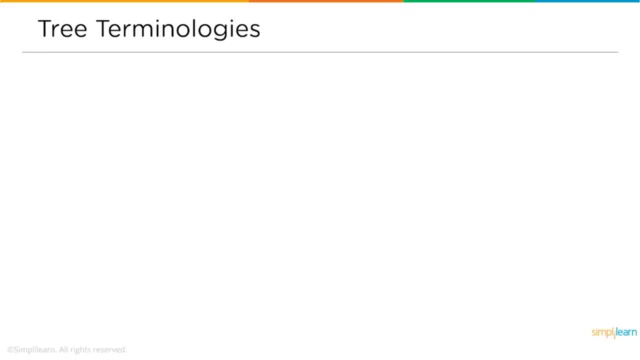 That is the terminologies of tree. So the first one is the node. Node is the entity that contains the keys and pointer to its child nodes. So here you can see that the elements a, b, c, d, e, f and g are the elements. 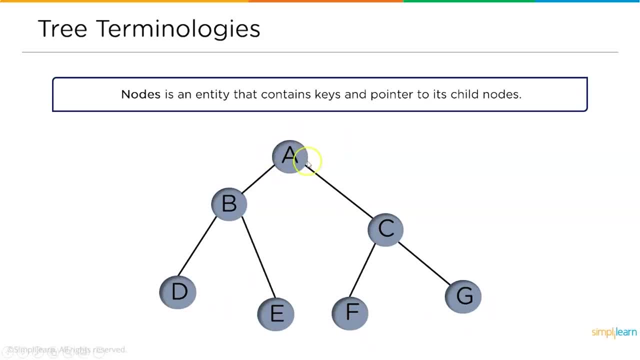 So each and every element or the blue dot is called as a node, And the blue dots here are 1, 2, 3, 4,, 5,, 6,, 7,, 8,, 9, 10.. 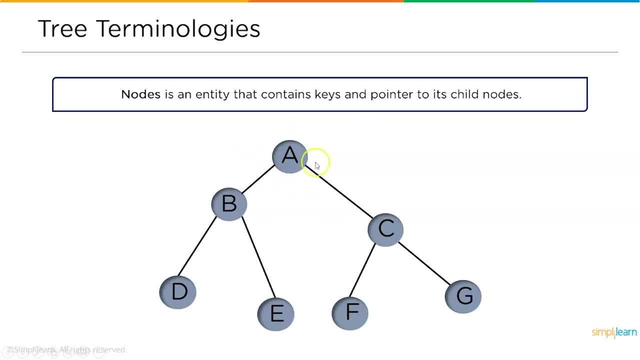 So we have 7 blue dots, So we have 7 elements here. So you can see the line between each elements, right. So this particular line is called edge. Now we will discuss about the edge in the next part. 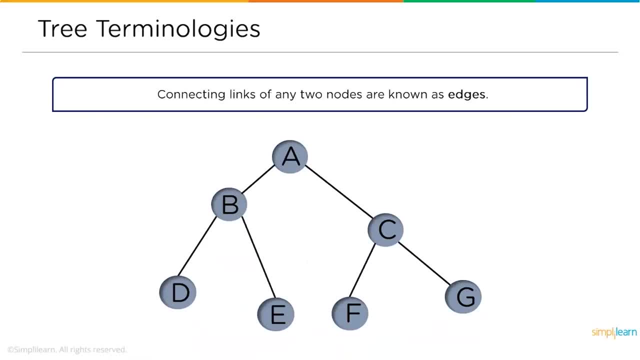 So the connecting links between any two nodes are called as edges. So we discussed about the nodes right Where the element is stored. the blue dots are the nodes And the lines connecting between the elements or nodes is called as the edge. 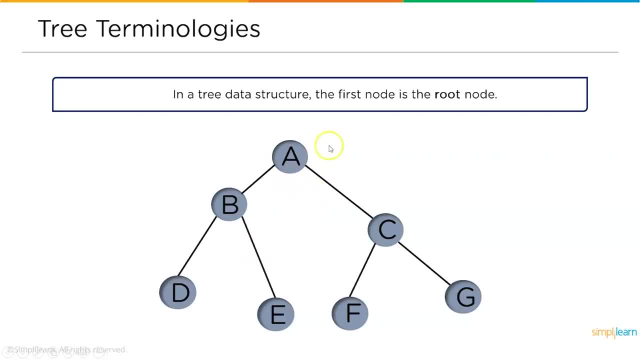 So out of all the nodes, this first node, that is, the element a, is called as the root node in a tree data structure. So indirectly, root node is also called as the parent node of all the nodes. Now we will understand what are parent nodes and children nodes? 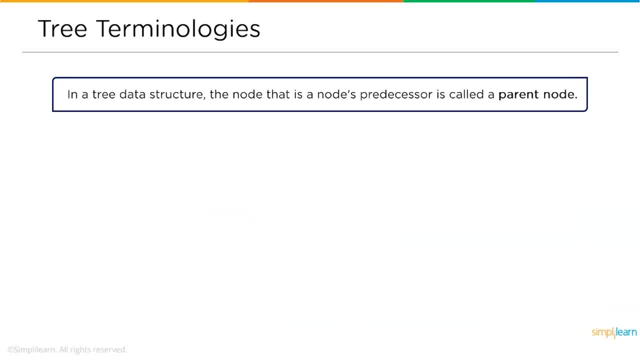 So in a tree data structure the node that is the node's predecessor is called as parent node. So here we have discussed that a or the root node is the parent of all nodes. So for a, b and c nodes are children nodes. 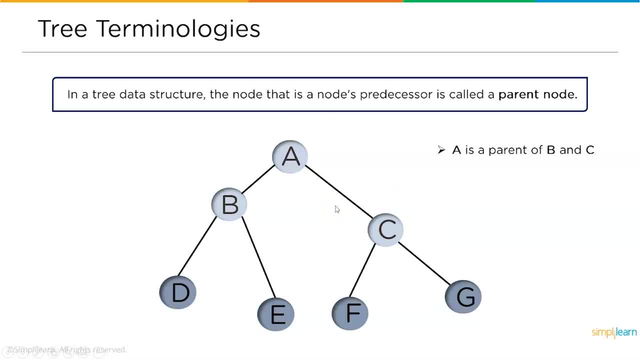 And for b and c nodes, a happens to be the parent node. Similarly, d and e are the children nodes of b, and f and j are children nodes of c, And the nodes d and e have b as a parent node and the nodes f and j have c as the parent node. 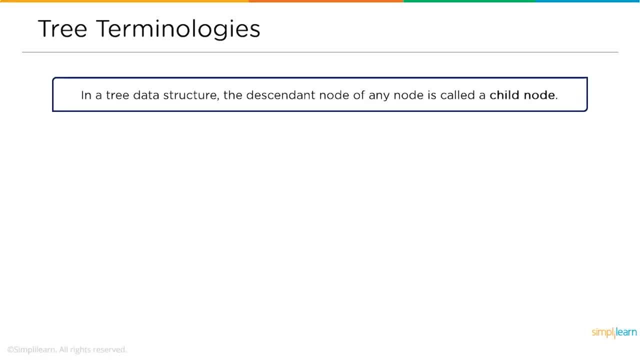 Now, followed by that, we will understand the descendant node. So, as discussed before, the descendant node is the node that comes after the parent node. Here the b and c are the descendants of a and d and e are descendants of b. 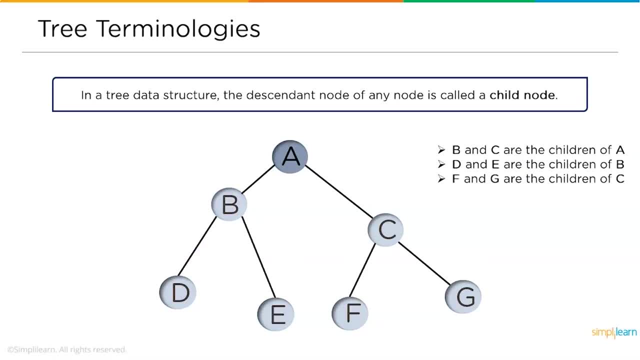 And similarly f and j are the descendants or children of the node c. So in a tree data structure the node which does not have any child is called as the leaf node. Now at the end we have d, e, f and j. 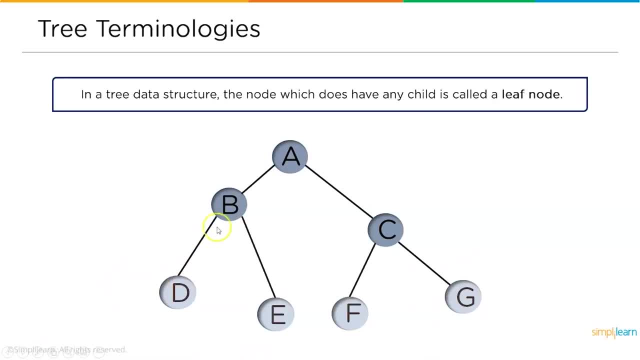 So these particular nodes do not have any children, nodes like b and j. So these particular four nodes which do not have any children are called as the leaf nodes. In a tree data structure the node with at least one child node is called as the internal node. 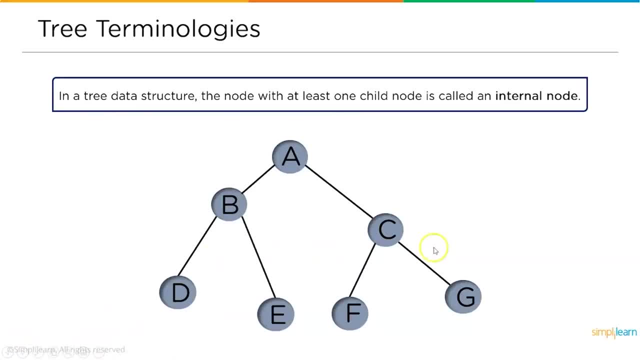 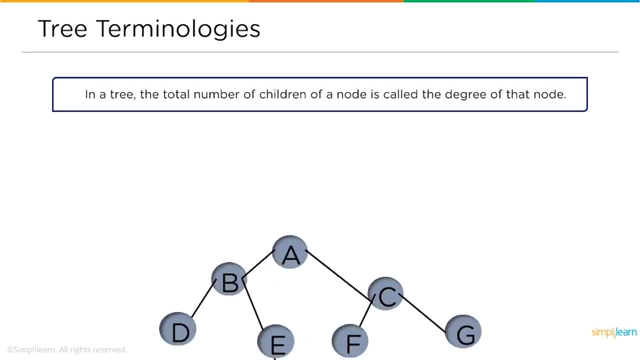 So here the internal nodes are b and c, which have at least one child. In a tree the total number of children of a node are called as the degree of that node. So in this particular diagram the degree of a root node is 2 because it has two child nodes. 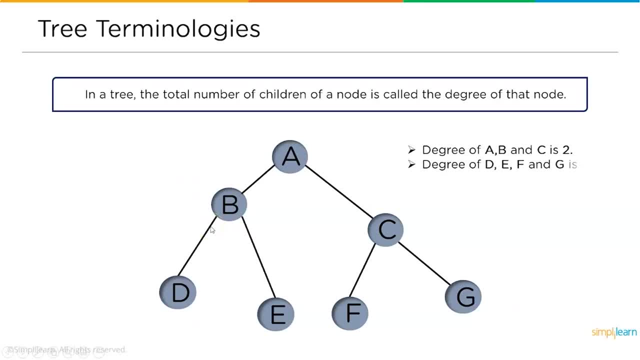 and the degree of b is 2 as it has two child nodes. Similarly, the degree of c is 2 because it has two child nodes, But when it comes to d, e, f and j, the degree is 0 because they do not have any child nodes. 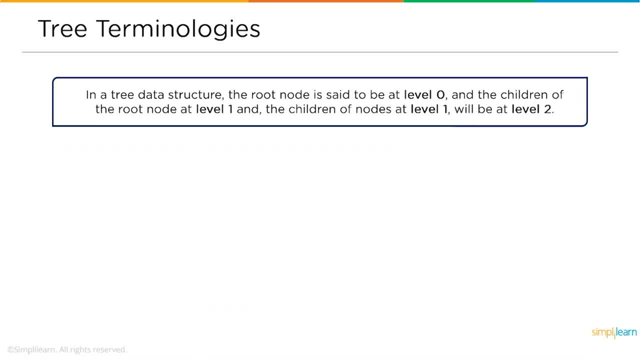 In a tree data structure, the root node is said to be at level 0 and the children of the root node are said to be at level 1, and the children nodes of the level 1 are at level 2.. So to understand this, let us go through the diagram. 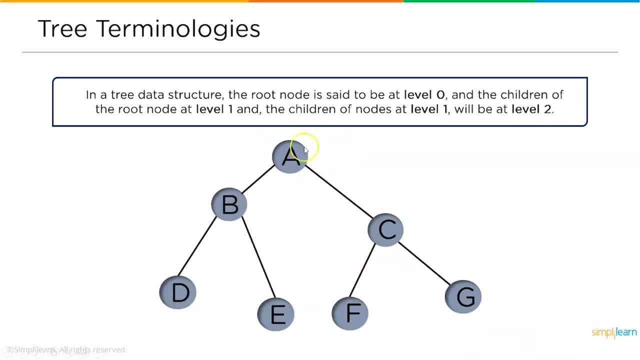 As you can see, this particular root node is called as level 0, and followed by that we have the children nodes of a, that is, b and c, and that level is called as level 1, and followed by that we have level 2.. And if this tree goes forward, the levels also increase accordingly. 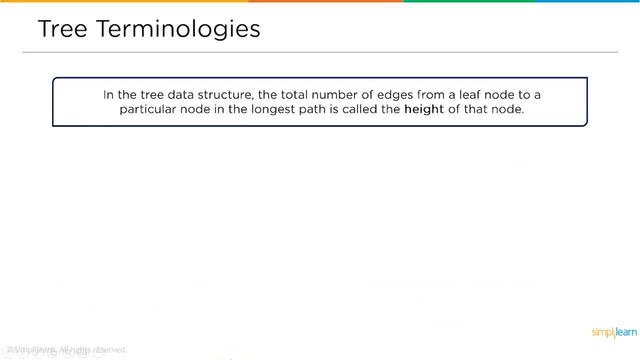 Now in a tree data structure, the total number of edges from a leaf node to the particular node is the longest path and this particular path is called as the height of that node. Now here we have our general tree data structure and here you can see the height of node a is 2. 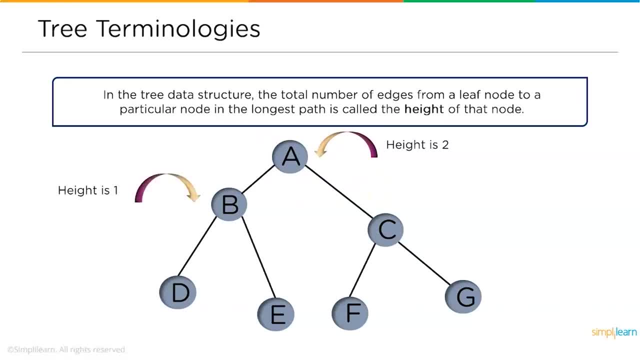 and the height of node b and c together is at 1, and the height of the last leaf nodes happens to be 0.. Next, in the tree data structure, the total number of edges from the root node to a particular node is called as the depth of that node. 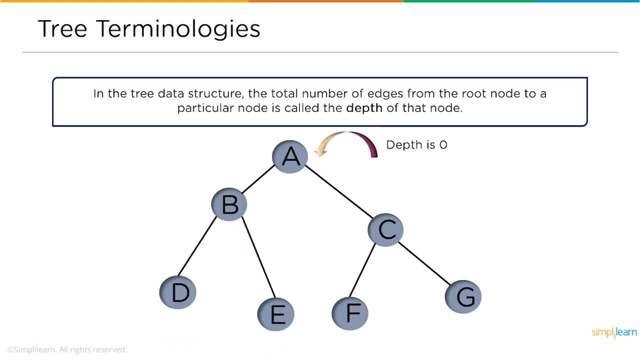 Now, in this particular tree data structure, the depth of the root node is 0 and the depth of b and c together is 1, because the number of edges connecting to the node a from b is just 1, and similarly, the number of edges connecting the node c from a is just 1.. 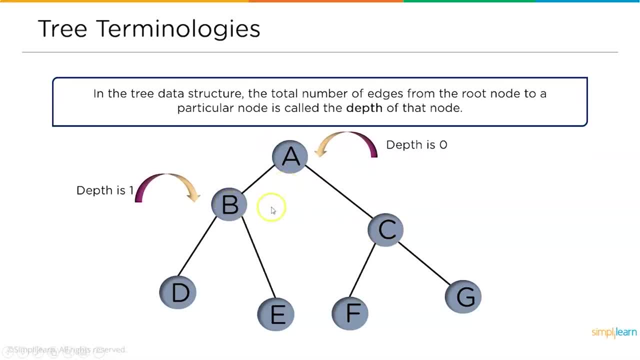 So the depth of both b and c is 1.. Now, if we consider the last leaf nodes, then the depth is 2 because, if you see, g is connected to a using 2 different edges. Similarly, f is connected to a using 2 different edges. 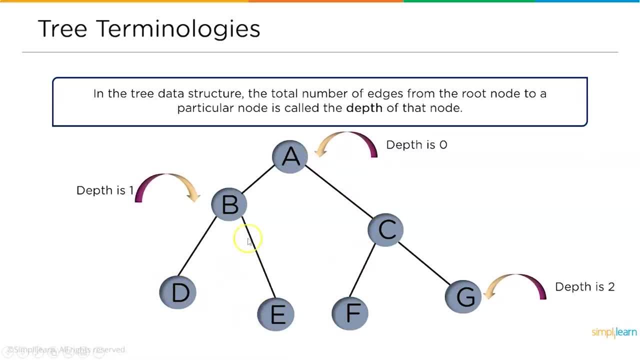 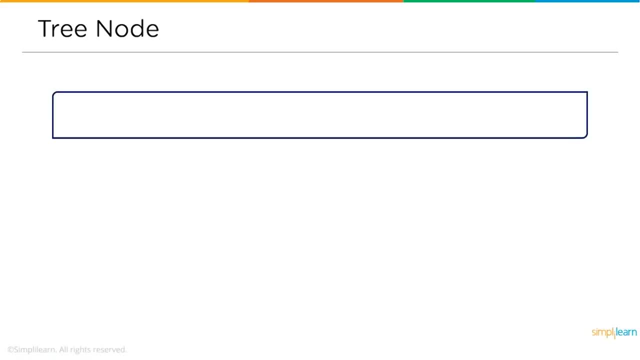 and e and d also have 2 nodes to connect to a, So the depth is 2.. Now in the next segment we will understand the tree node. So the tree data structure has data part and references towards left and right child node in the tree. 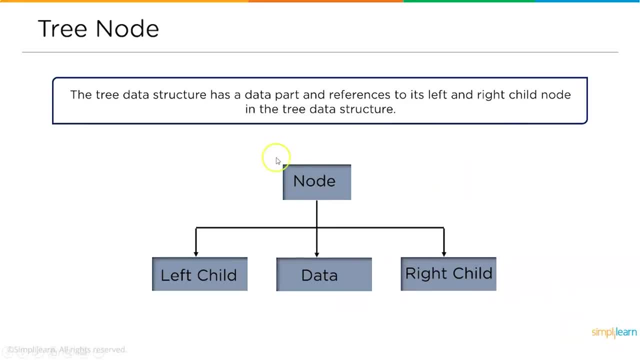 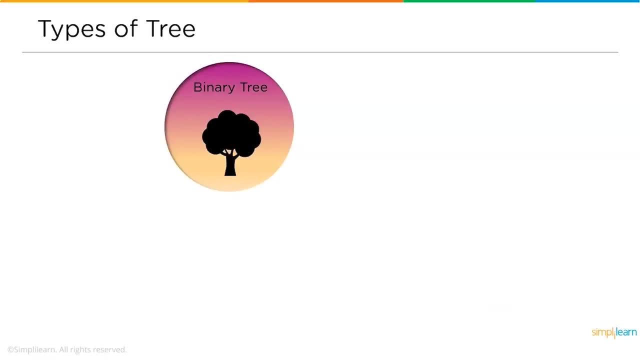 So here you can see, this is the node, and the node has 3 segments, that is, data element and the references towards left child and the references towards right child. Now there are 4 different types of trees. The first one is the binary tree, followed by that we have the binary search tree. 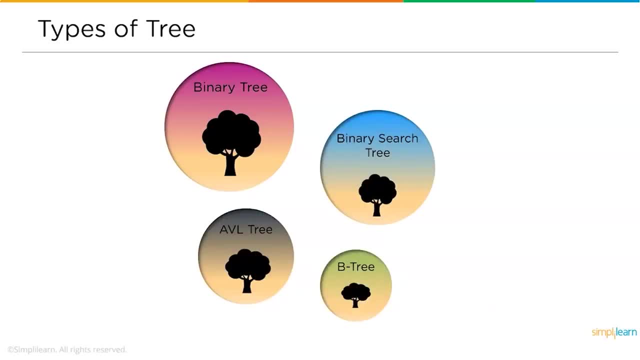 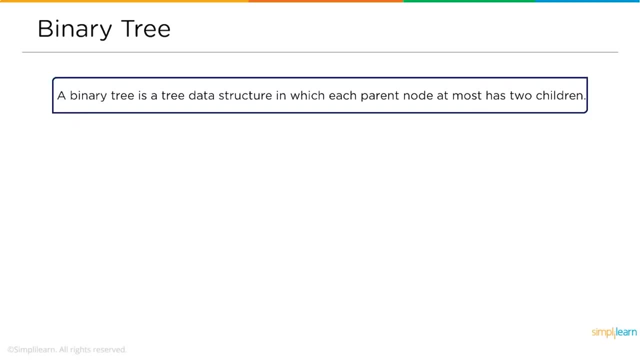 Then we have AVL tree and finally we have the B tree. Let us discuss each one of them. The first one is the binary tree. A binary tree is a tree data structure in which each parent node at most has 2 children. So in this particular tree we will have at most 2 children. 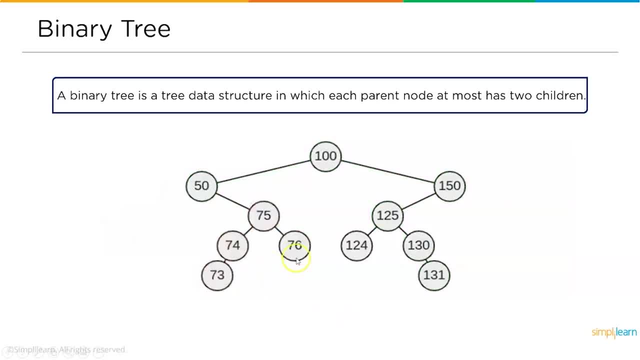 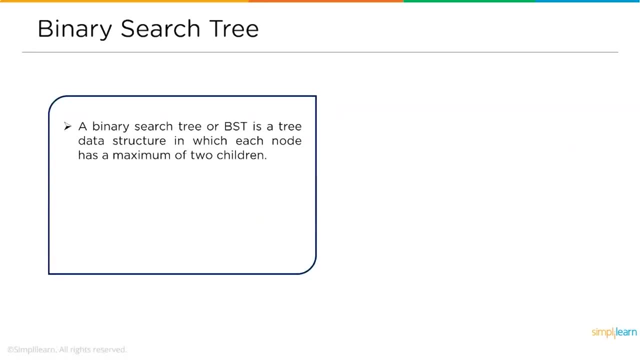 That means it might have 1 or more than 1, but not more than 2 children per node. Moving ahead, we have the binary search tree. So a binary search tree or a BST is a tree data structure in which each node has a maximum of 2 children. 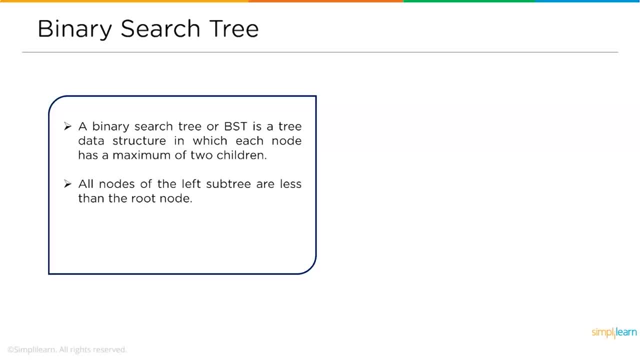 All nodes of the left side of the tree, the left subtree, are less than the right node. All nodes on the right subtree are more than the root node. So here you can see the image, or the GIF, which represents the image of a binary search tree. 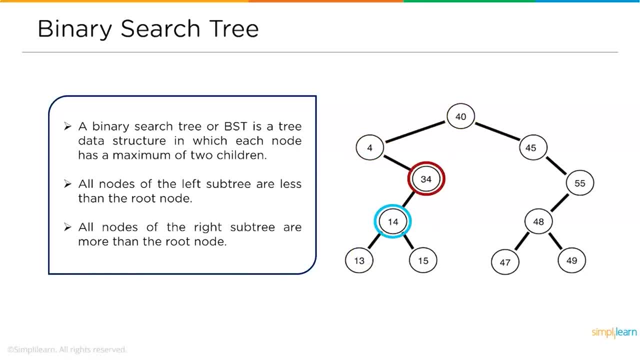 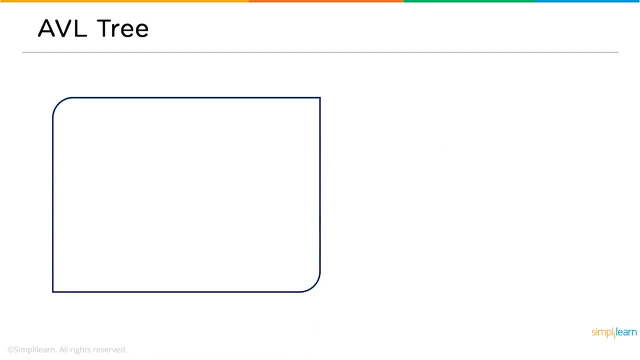 So here all the nodes of the left subtree are less than the root node and all the nodes of the right subtree are more than the root node. The next type of the tree is the AVL tree. The AVL tree got its name after inventory Georgi Adelsonvelsky. 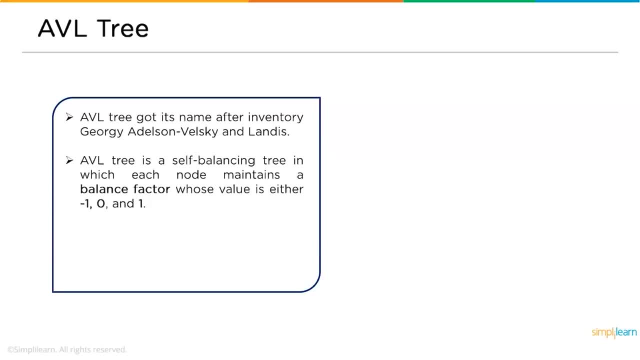 Adelsonvelsky and Landis AVL tree is the self-balancing tree, in which each node maintains a balance factor whose value is either 1, 0 or minus 1.. Balance factor is equals to height of the left subtree minus height of the right subtree. 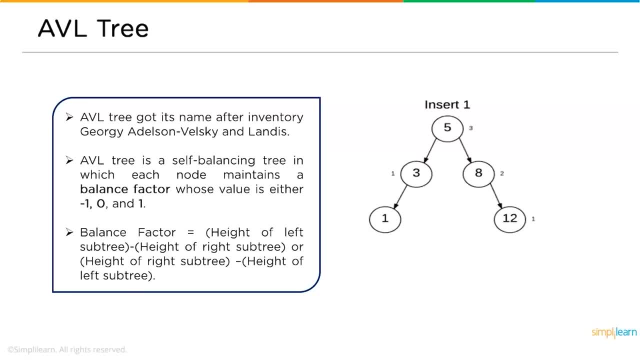 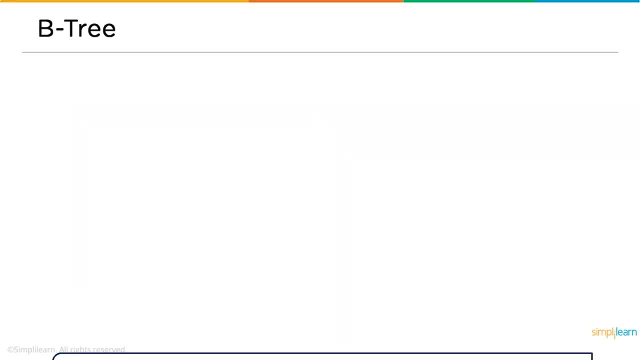 or height of the right subtree minus height of the left subtree. So in this particular image you can identify it is an AVL tree. And now the last type of tree, that is, the B tree. B tree is a special kind of self-balancing search tree. 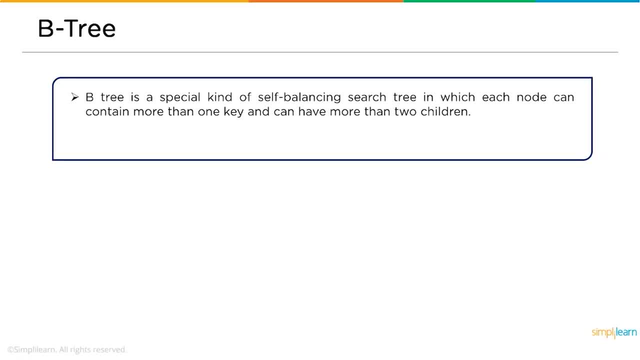 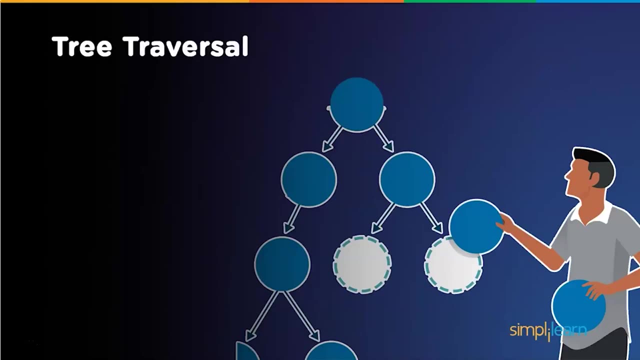 in which each node can contain more than one key and can have more than two children. B tree is also known as the height-balanced M-way tree. Now, in this particular GIF, we can see how a B tree looks like. Now, followed by this, we will discuss the tree traversal. 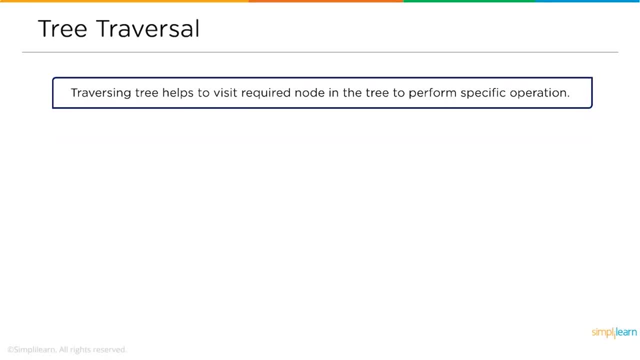 So traversing a tree helps to visit required node in the tree to perform specific operations. Tree traversal can be performed in three different ways. The first one is the pre-order traversal, where we visit the node and visit all the nodes from the left side. 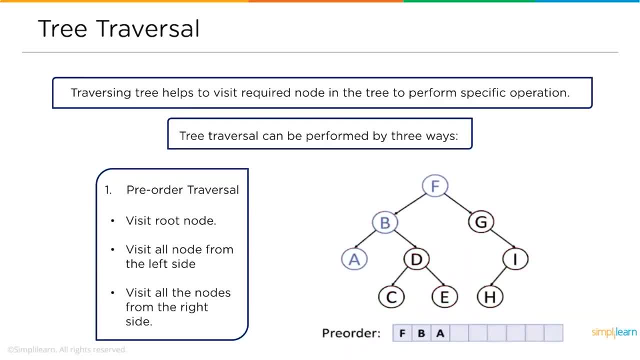 then visit all the nodes from the right side. So this particular GIF is an example for pre-order traversal, where we visit all the left side nodes first, then we visit the right side nodes. Now we will move ahead into the next type of traversal. 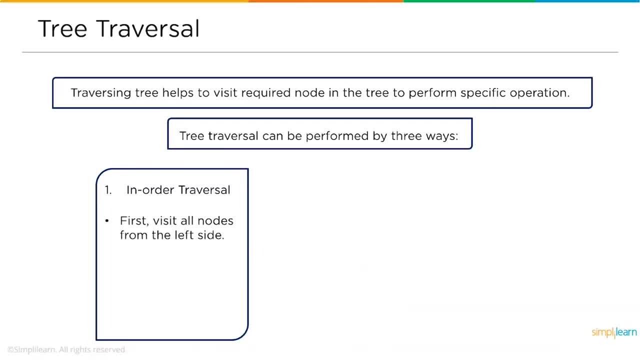 That is the in-tree traversal. This is an in-order traversal. First we visit all the nodes from the left side, then we visit the root node and then we visit all the nodes from the right side. So this particular GIF will be an example for the in-order traversal. 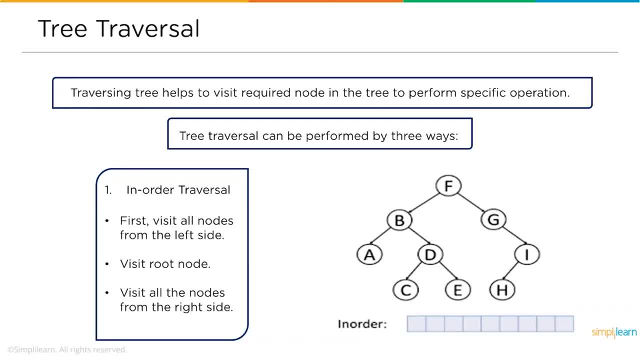 where we visit all the left side nodes. then we visit the root node and followed by that we will visit the right side nodes. And the last type of traversal is the post-order traversal, where we visit all the nodes from the left side first, then we visit all the nodes from the right side. 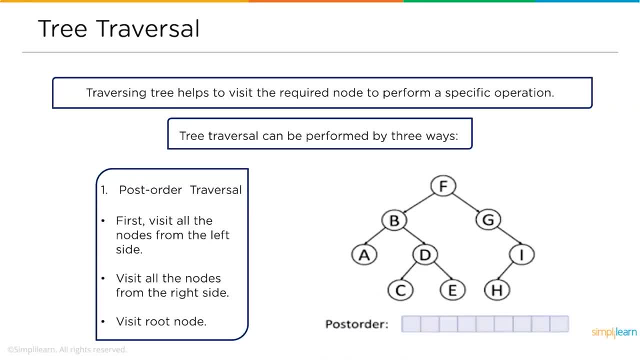 and finally visit the root node. So this particular image on the right side is an example for post-order traversal. Now, before we get into learning the applications of trees, we will try to execute one example based on the post-order, pre-order and in-order traversals in tree data structure. 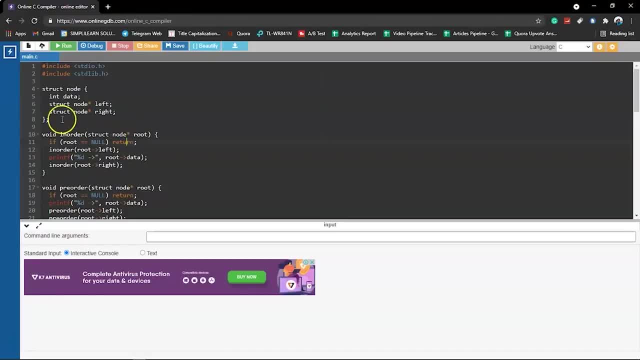 So you can see that we have an example on my screen right now. So here we have the node structure. then we have the in-order traversal function, Followed by that we have the pre-order traversal function and finally we have the post-order traversal function. 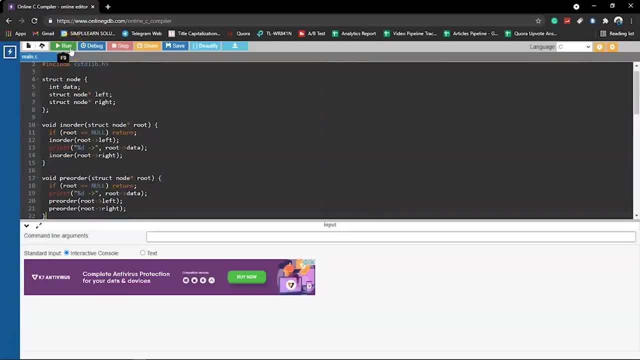 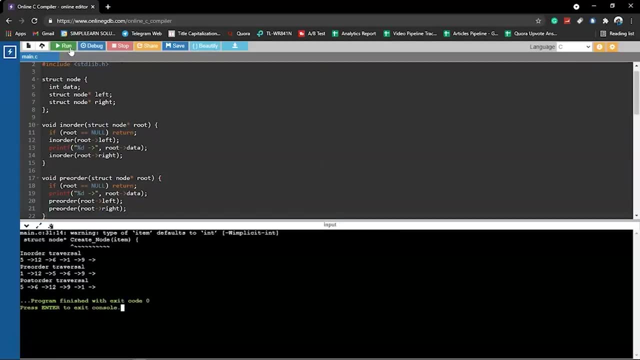 Now let's quickly run this program and see the output, and don't worry about the code. This particular code document will be attached in the description box below and you can have access to it. Now we have the run option over here and the program got successfully executed. 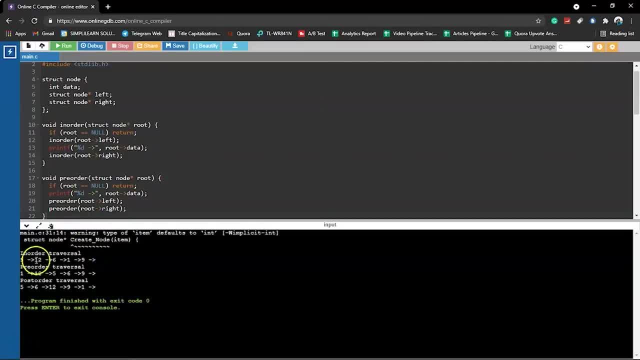 You can ignore this warning. and here we have the in-order traversal of the tree in the first output, Then we have the pre-order traversal of the tree and finally we have the post-order traversal of the tree. Now let's discuss the last part. 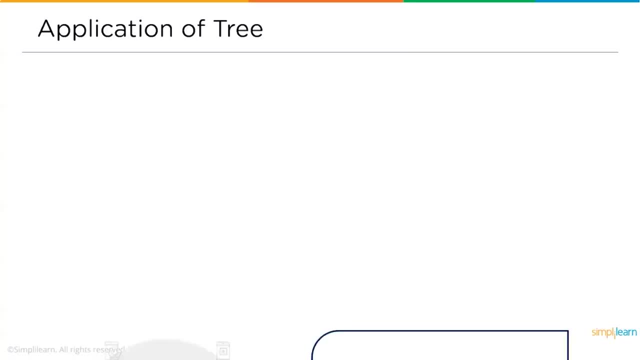 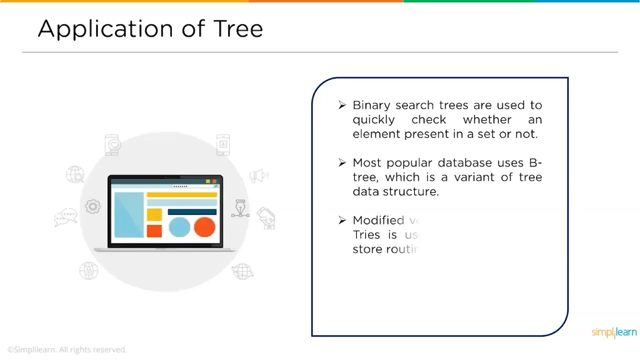 where we will learn the application of trees. So the application of trees are as follows: Binary search trees are used to quickly check whether an element is present in the set or not. Then we have the most popular database usage of btree, which is a variant of tree data structure. 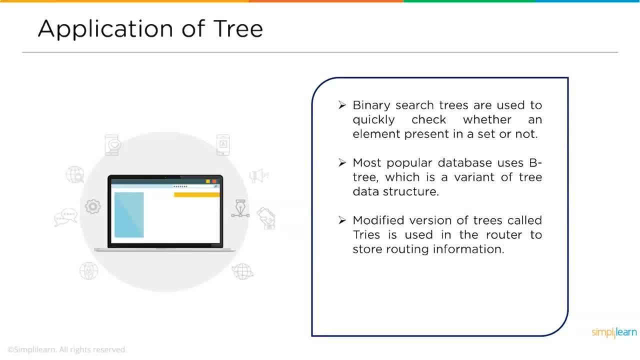 Then we have the modified version of trees, called as trice, which is used in the router to store routing data. And finally, the compiler uses a syntax tree to validate the syntax of every program you write. So we shall begin our session by learning a binary tree. 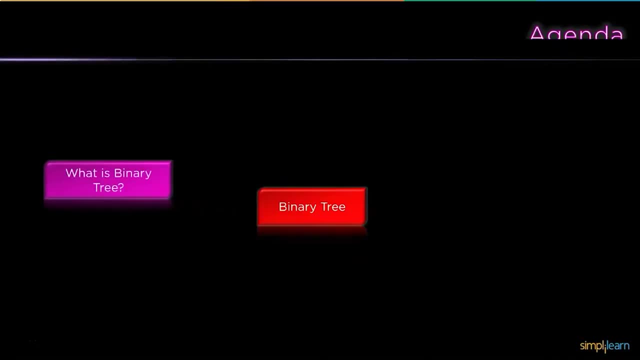 and some basic terms related to binary tree, Then we will try to implement it in the code editor. After that we will discuss its properties. Then we will discuss different types of binary trees. Then we will try various operations on them. 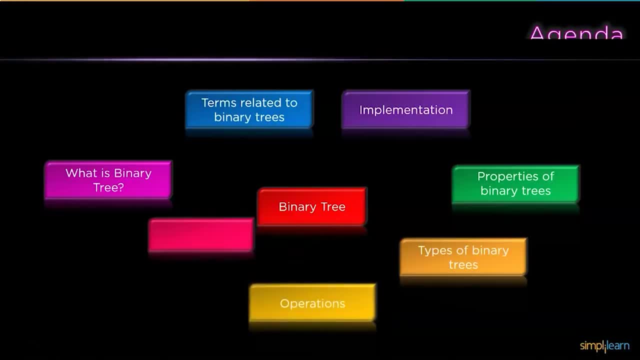 like traversal insertion and deletion. And finally, we will take a glance on what are our final key takeaways from this session. But before we begin, make sure that you have subscribed to our YouTube channel and clicked on that bell icon to never miss an update from Simply Learn. 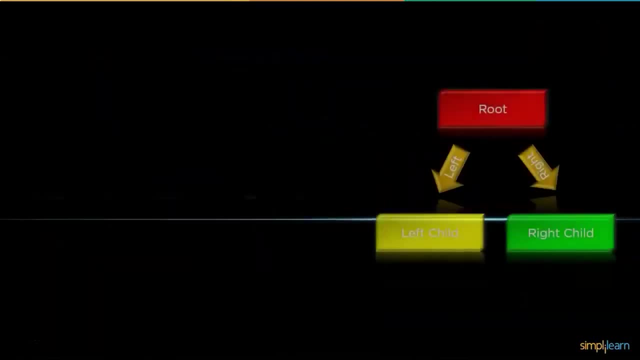 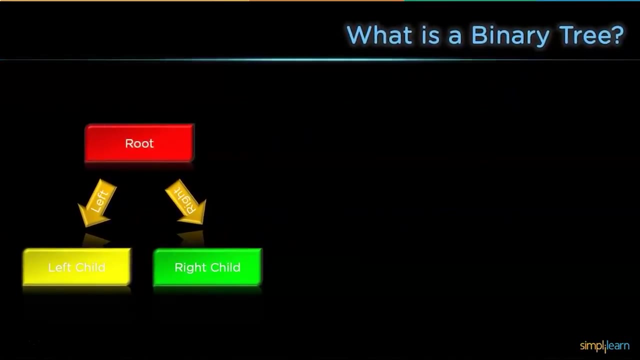 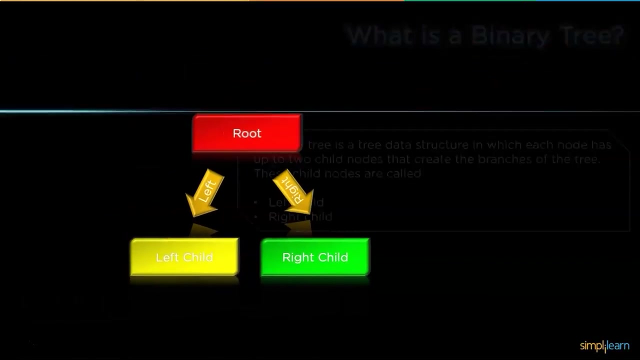 So, without further ado, let's get started with our first topic, that is, what exactly is a binary tree? So it is a tree data structure in which each node can have at most two child nodes. These nodes are referred to as left child node and right child node. 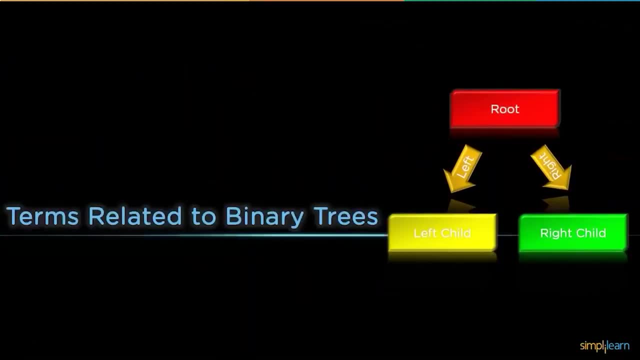 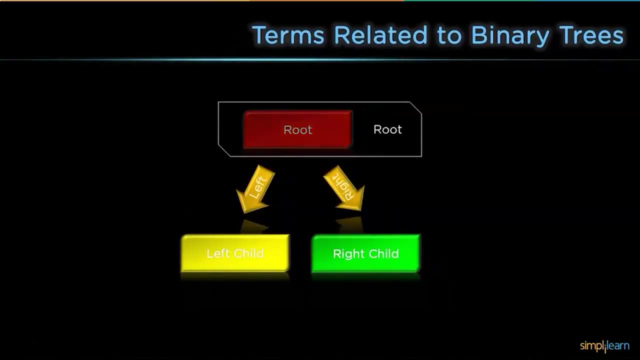 Next let's discuss about some terms related to binary tree. First up, a node. A node consists of data and linked to its both child nodes. Next, the root node. Root node is the first node of the tree. Next, leaf nodes. 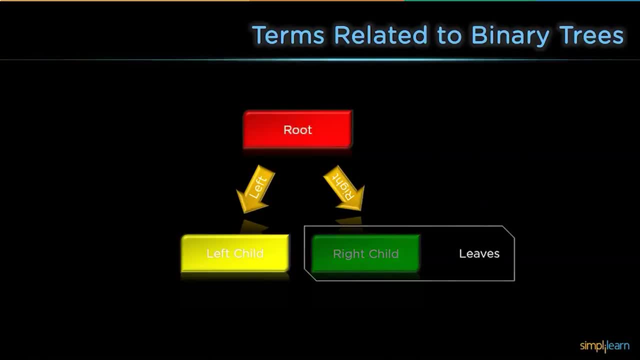 These are the nodes which has no child. Next parent node: Apart from the root node: any node which has at least one child is called as parent to that child node. Next up a child node: Any node with a parent is called as a child node. 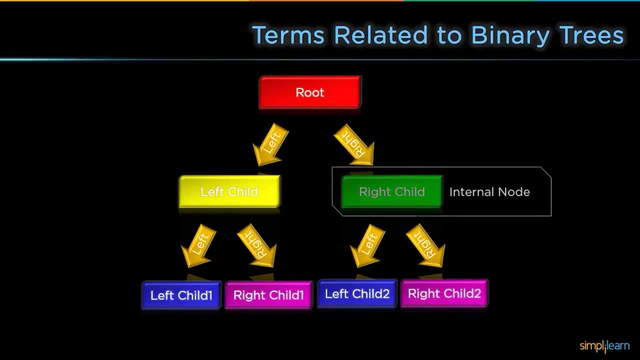 Next up is the internal node. Any node with a child and a parent is called as an internal node. Next up is the height of the binary tree. The longest path from the root to any leaf node is called as the height of the binary tree. 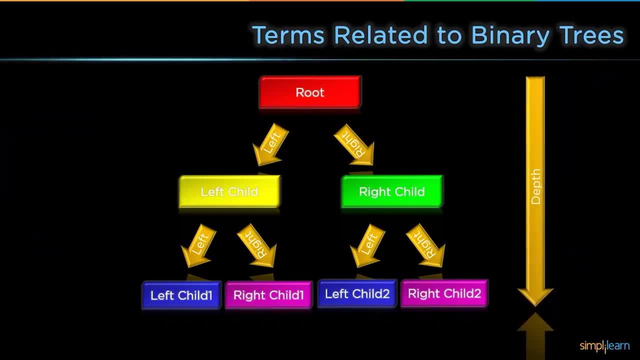 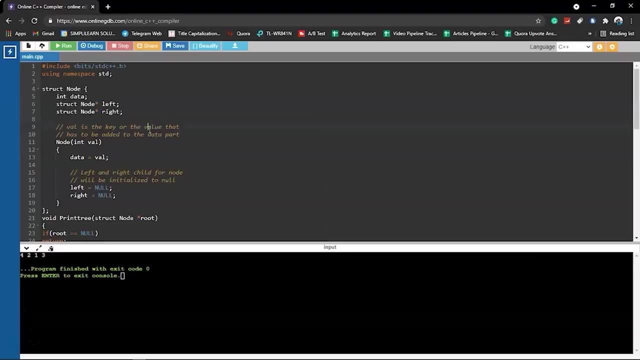 Next up is the depth of the binary tree. The depth of the node is the total number of edges from the root node to the target node or the last child node. Now let's try to implement the binary tree in the code editor. As you can see, now we are on the code editor. 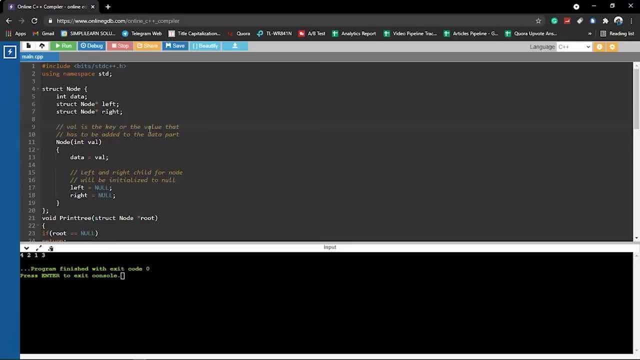 And the code on my screen is an example for binary tree. Now, here you can see that we have created a structure for node. Followed by that, we have a function where we will print the tree, And this is our main function. 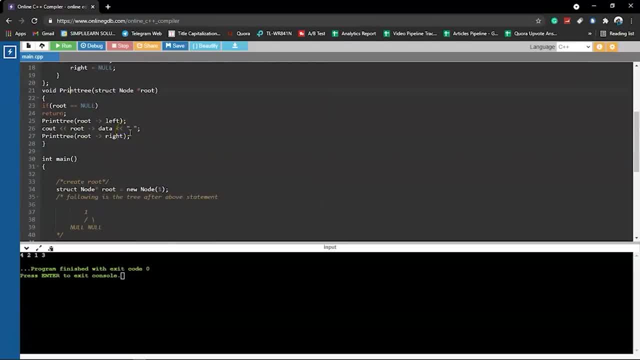 Now don't worry about the code. This particular code segment will be available in our description box below And you can always have access to it and try to edit and run this code on your own local system to have a better learning experience. Now, without further ado, let's try to run this program quickly and see the output. 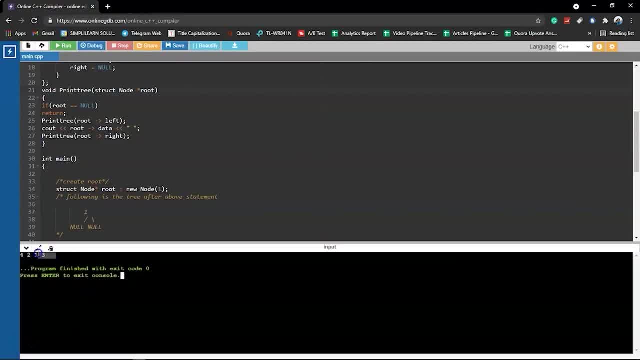 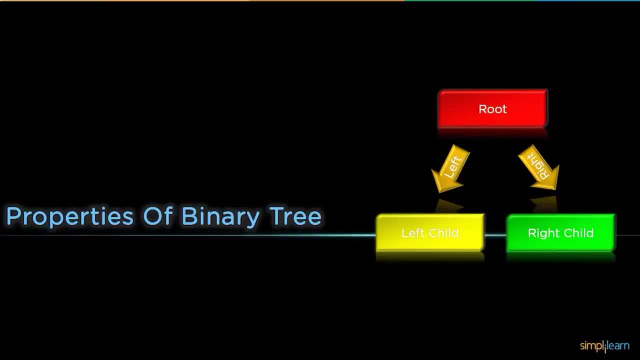 So there you go. The code got successfully executed, And here you can see the output of this particular binary tree. Now let's get back to the theory part. So, as discussed before, followed by the implementation part, we will learn about the properties of a binary tree. 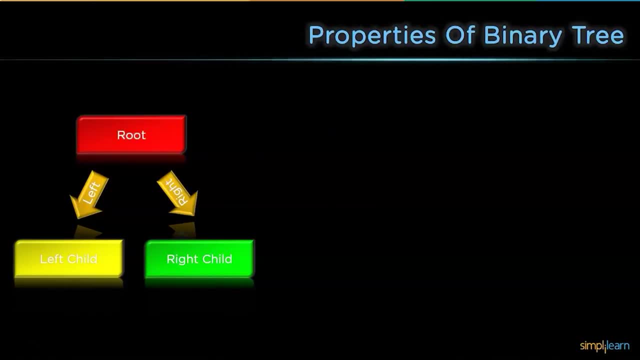 Now let's discuss the properties of the binary trees. First up, maximum number of nodes at a level L is 2 to the power L. Next up, maximum number of nodes in a binary tree of height H is equals to 2 to the power of H minus 1.. 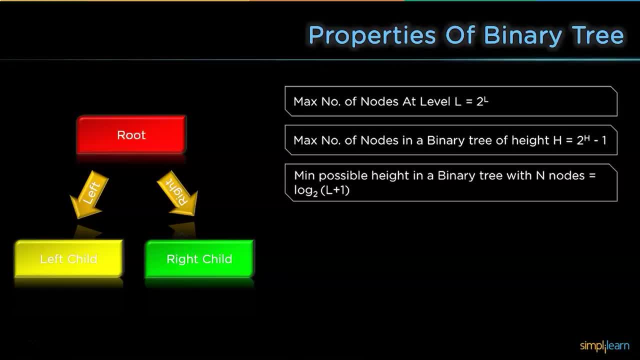 Next up: minimum possible height in a binary tree with two nodes is equals to log of L plus 1 base 2.. Next up: the minimum possible level in a binary tree with n nodes is equals to log of L plus 1 base 2.. 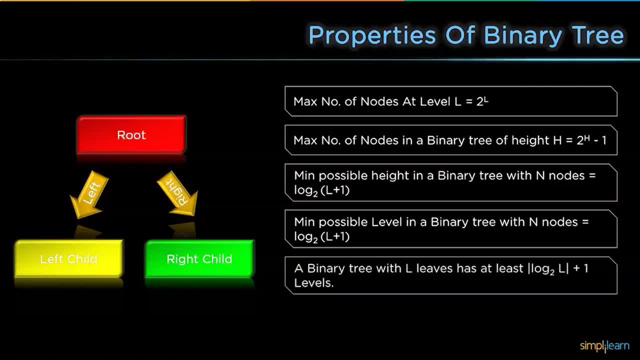 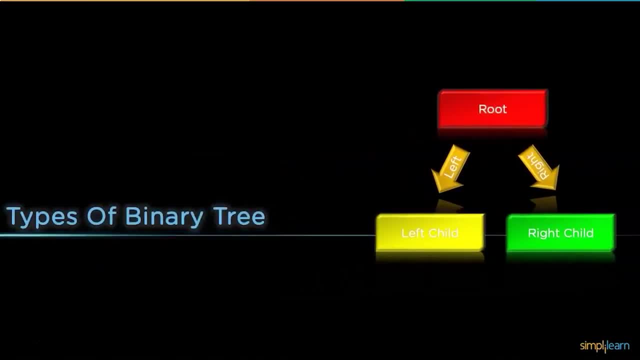 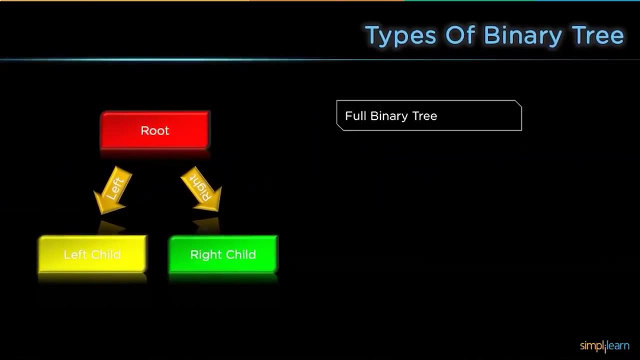 Finally, a binary tree with L leaves has at least log L base 2 plus 1 levels. Now let's discuss about the different types of binary trees. First up, we have the full binary tree. Followed by that we have the complete binary tree. 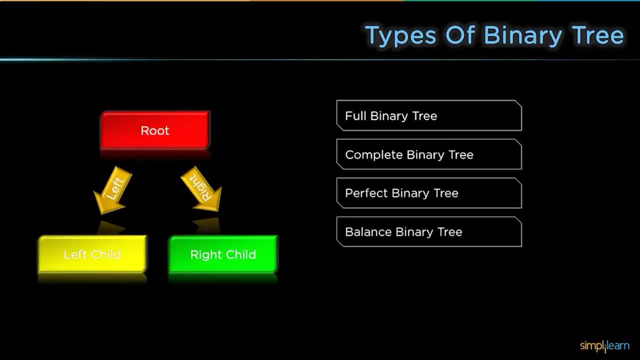 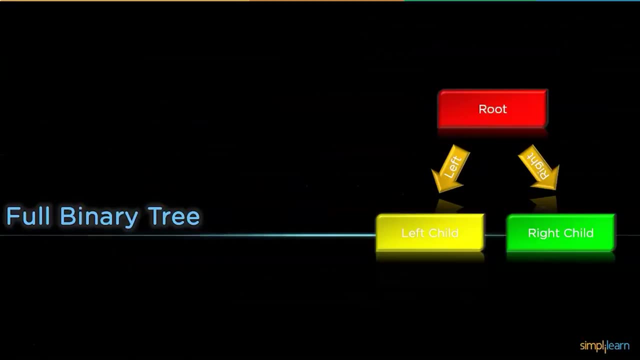 Then we have the perfect binary tree, Followed by that we have the balanced binary tree And lastly, the degenerate binary tree. Let's discuss about these in detail. First up, full binary tree. A full binary tree is a unique tree data structure. 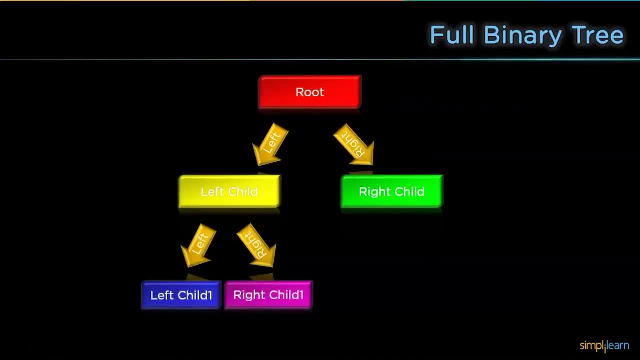 in which a node can have either two children or no child. Next, a complete binary tree. So a complete binary tree is another specific binary tree where each node, on all levels except the last level, must have two children and at the lowest level, all leaves should reside possibly on the left side. 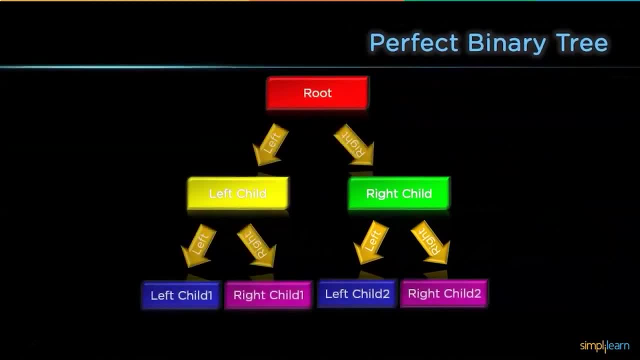 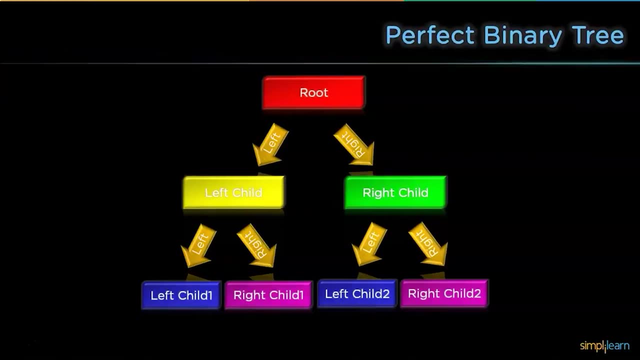 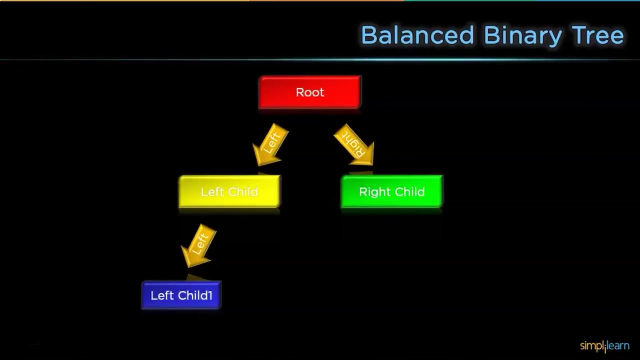 The next one is the perfect binary tree. A binary tree is perfect if every node must have two children and every leaf is on the same level. The next one is called as the balanced binary tree. A binary tree is balanced if, for each node, 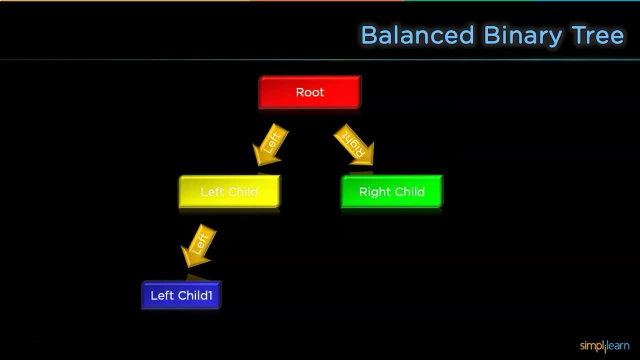 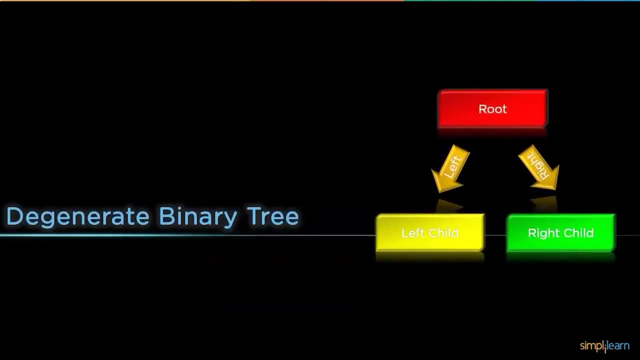 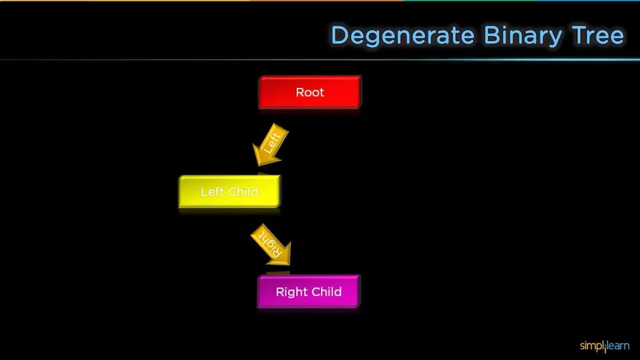 the height of the left subtree and the height of the right subtree varies at most by just one. At last, we have the degenerate binary tree. A binary tree is said to be degenerate if every internal node has only one child. We have now discussed the binary tree. 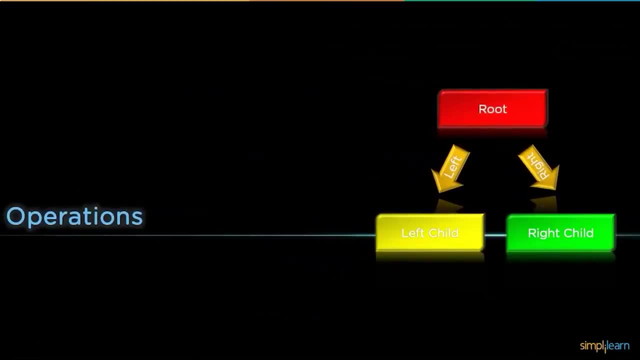 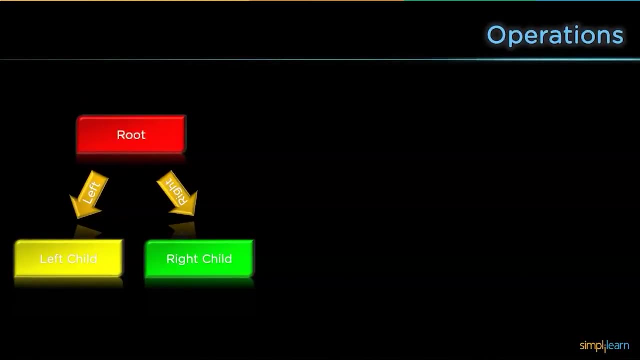 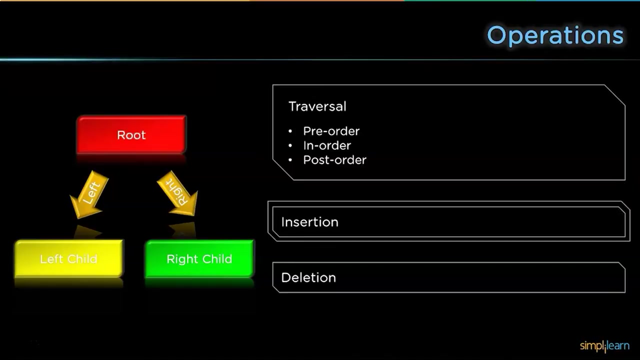 some terms and properties related to binary trees and types of binary trees. Now we will look into the operations that needs to be performed on the binary tree. So there are basically three types of operations that can be performed on binary tree, which are traversal, insertion and deletion. 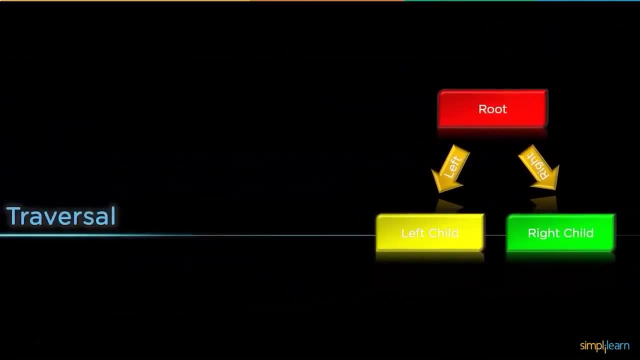 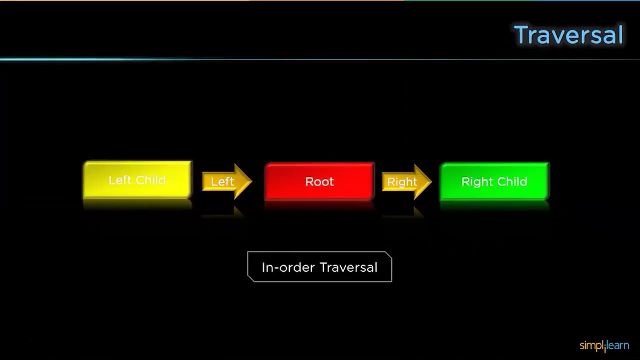 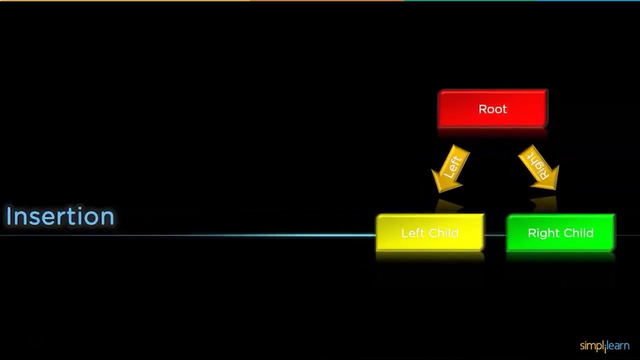 So first we will look into the traversal operations. There are three different types of traversal operations possible on binary tree, which are pre-order traversal, in-order traversal and finally the post-order traversal. Now let's get back into the text editor mode and try to execute our example. 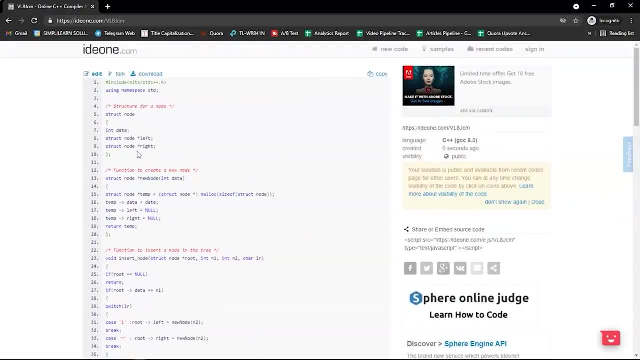 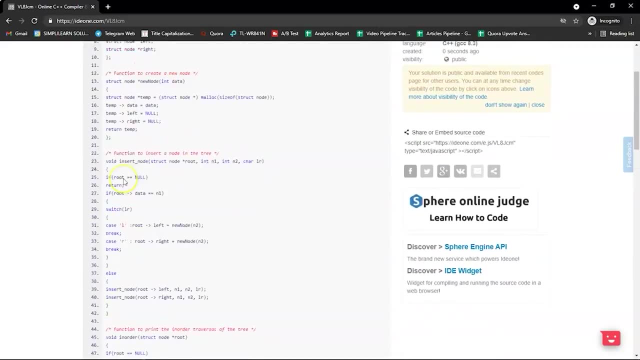 So right now we are on the text editor and this particular code is for the traversal operations on our binary tree. And here you can see we have the structure for node and we have also the in-order function, pre-order function and post-order function. 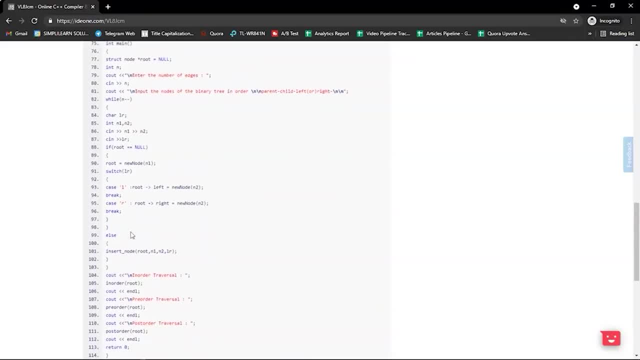 Do not worry, This particular code will be available in the description box below And after you have written the code, we have some standard input over here. You can see that we are giving the number of edges as 4 and the left subtree elements are 2 and 1. 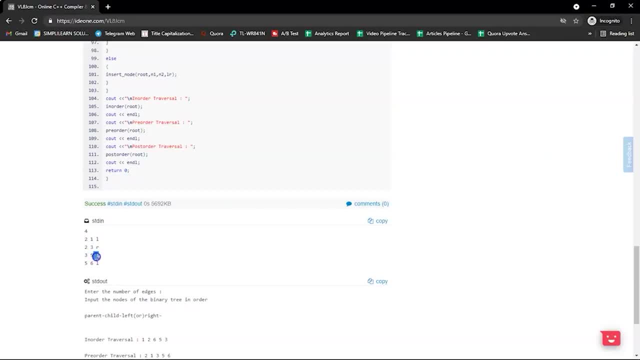 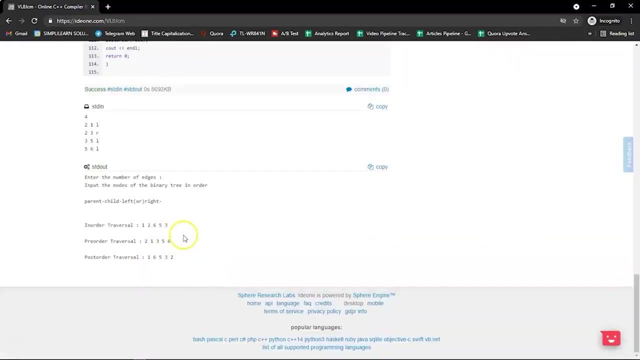 and the right subtree elements are 2 and 3 and another left subtree elements are 3 and 5 and lastly, we have 5 and 6 for another left subtree. Now let's try to execute this code Now. we have already executed the code. 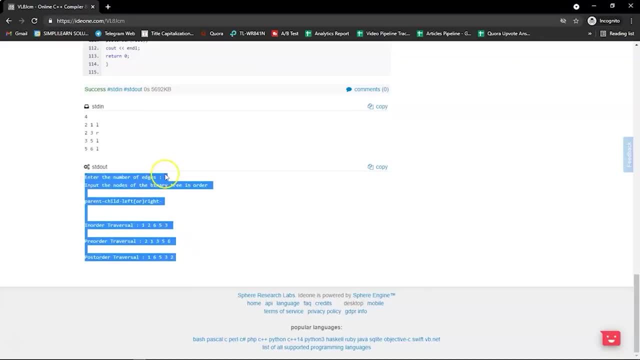 and we also have the output over here, And here you can see we have entered the number of edges as 4 and the traversal is in-order traversal, which is 1,, 2,, 6,, 5 and 3, and the pre-order traversal output is 2,, 1,, 3,, 5,, 6. 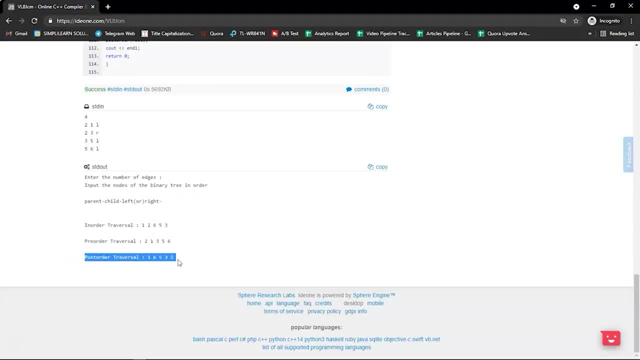 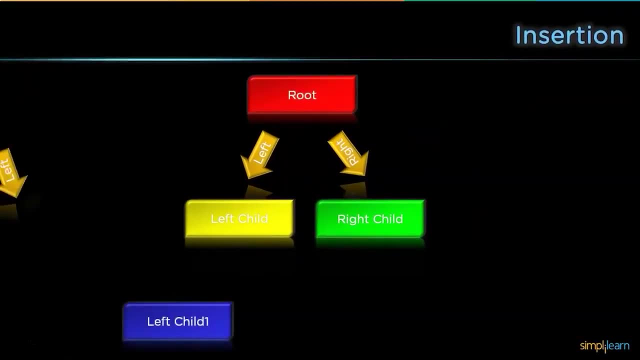 and the post-order traversal is 1,, 6,, 5,, 3 and 2.. Now let's get back to the PPT. Now we have the insertion operation. And now we have the insertion operation. And now let's get back to our text editor. 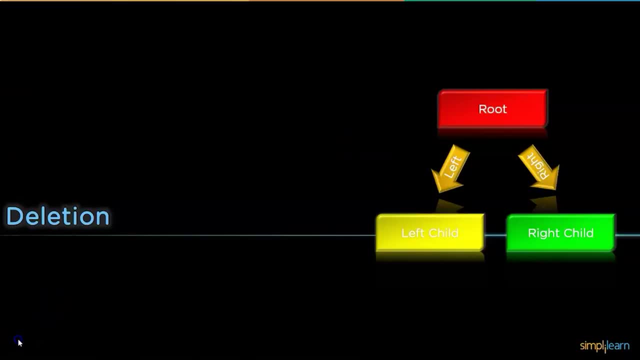 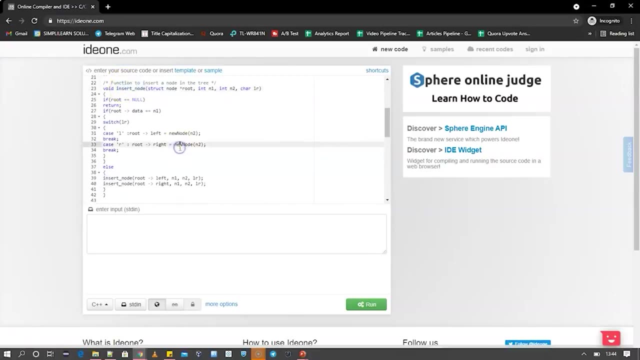 and try to see an example for insertion operation as well. So on my screen you can see an example for insertion operation. So here we have the insert function. As I said, this particular code will be available in the description box below. 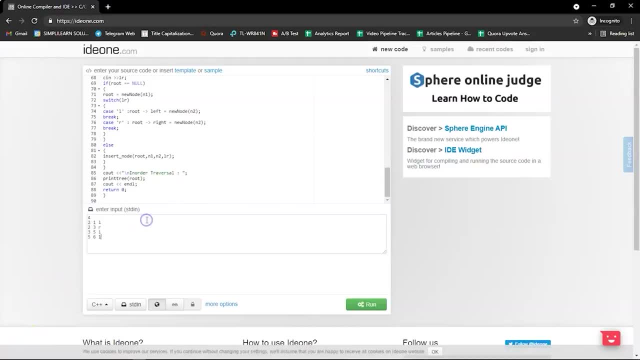 Now let's provide the standard input. So the standard input will be 4 edges and we have 2 and 1 as the left subtree and 2 and 3 as right subtree, 3 and 5 as left subtree again and 5 and 6 as the left subtree. 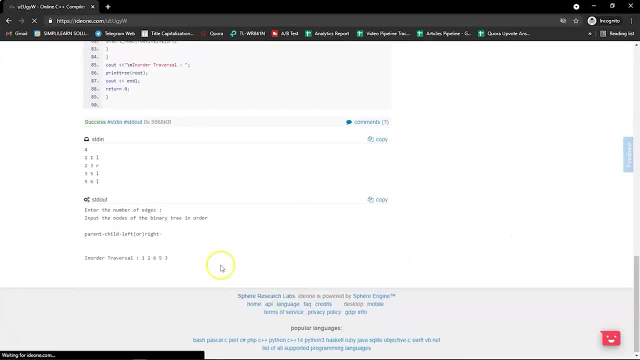 Now let's quickly run this code, And there you go. The program got successfully executed and here we have the output. The nodes got inserted and it has provided an in-order traversal, that is 1,, 2,, 6,, 5 and 3.. 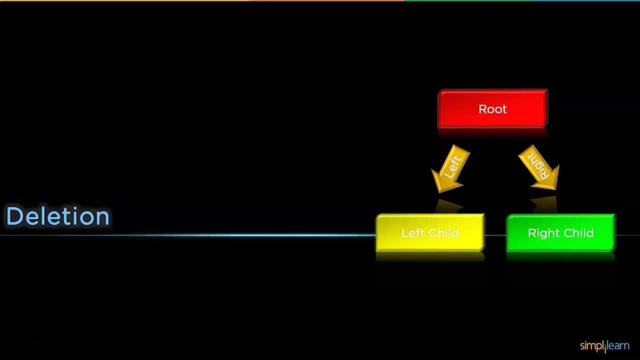 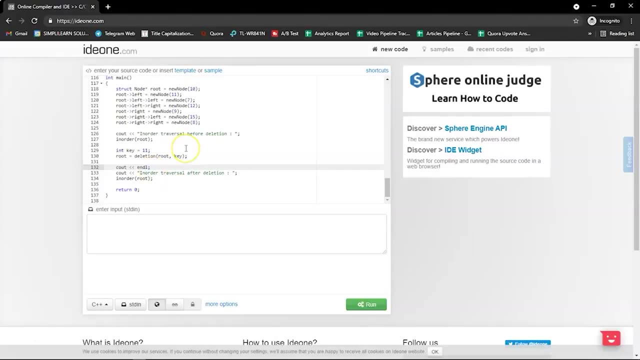 Now let's get back to the presentation, and the last type of operation is the deletion operation. Let's quickly execute an example based on deletion operation as well. Now, as you can see, we are on the text editor again. Now, here, the example is for deletion operation. 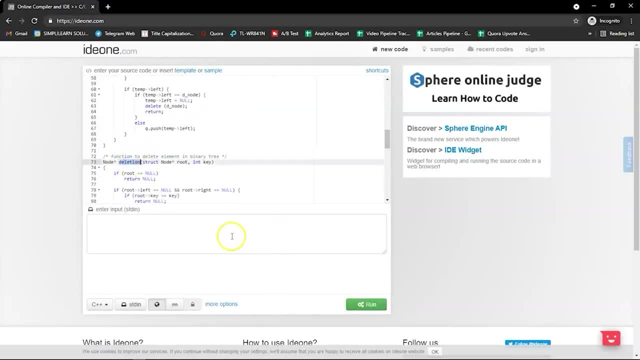 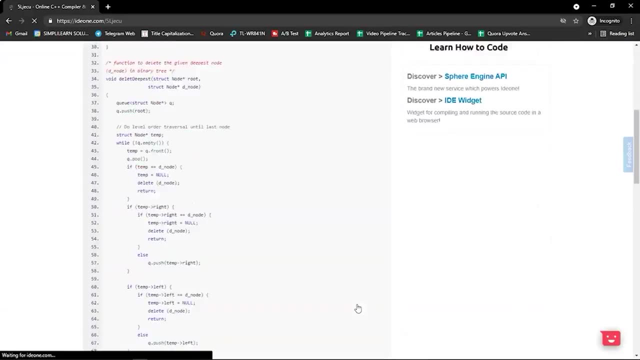 We have the delete function over here Now for this particular program. we don't need any standard inputs, So just let's run the program. So there you go. The program got successfully executed and we have the output over here And in-order traversal before deletion. 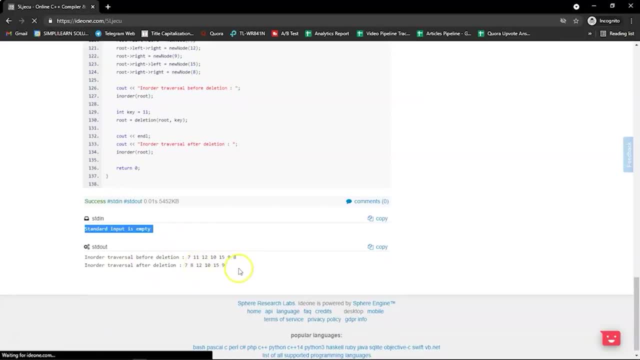 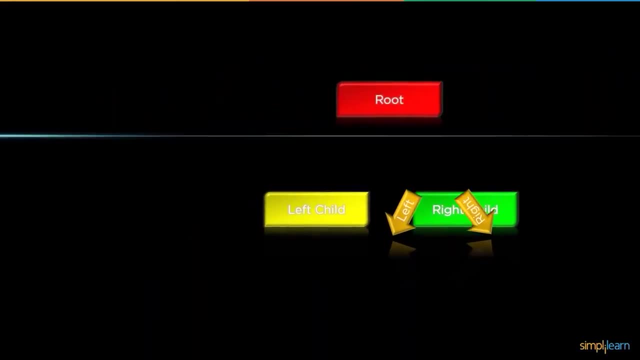 and in-order traversal after the deletion of an element. So the deleted element is element level. Now with that let's get back to the presentation mode again. So that's how the element got deleted. Now we have reached to the last part of this session. 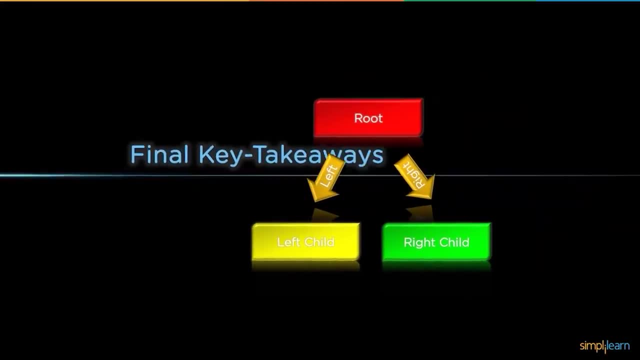 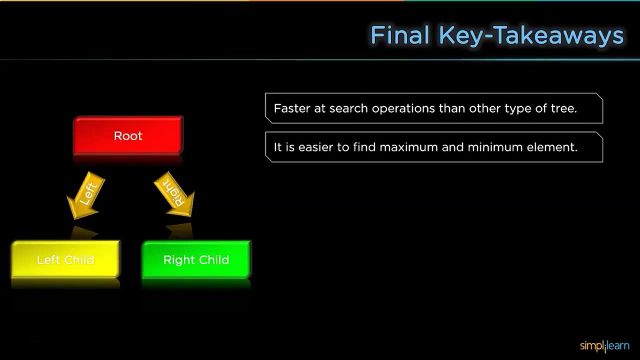 that happens to be the final key takeaways. So what are the final takeaways? So binary tree is faster at search operations than other type of tree and it is easier to find maximum and minimum elements in the binary tree. Binary tree does not allow duplicate values. 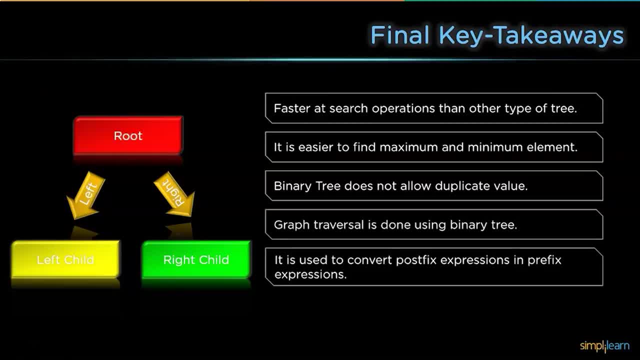 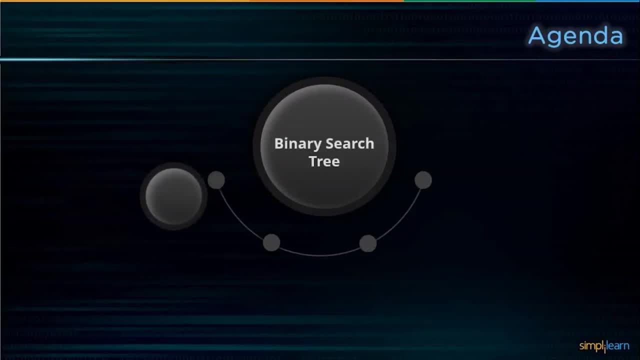 and graph traversal is done using binary tree. It is used to convert the postfixed expressions into the prefix expressions. We shall begin by introducing binary search trees. Then we will discuss some of the properties of binary search trees. After that we will try various operations. 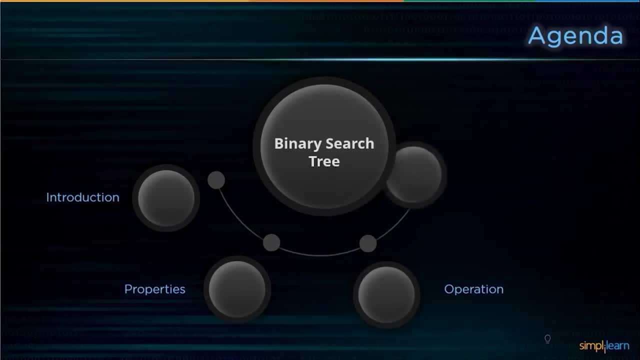 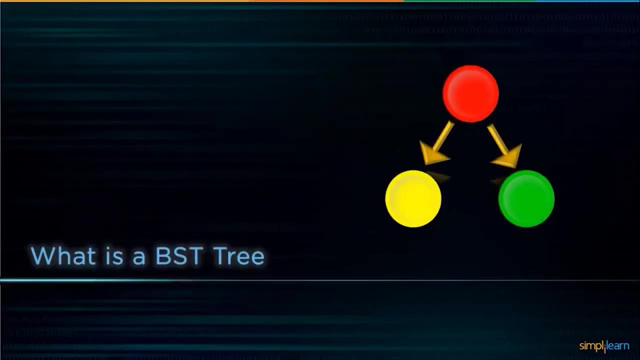 on them, like insertion and deletion. Finally, we will sum up what we have learned from this session, But before we begin, make sure you have subscribed to our YouTube channel and clicked on the bell icon below So you never miss an update from Simply Learn. 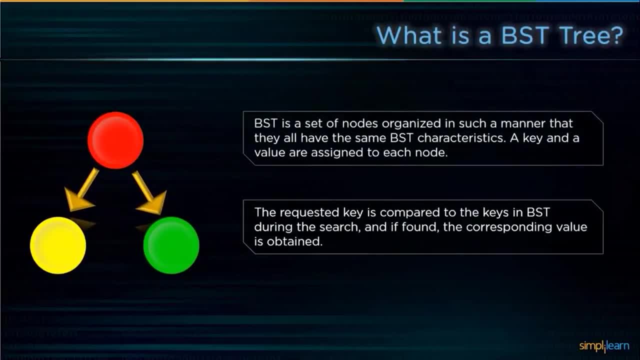 So, without any further ado, let's get started with introduction to binary search tree. Binary search tree is a set of nodes organized in such a manner that they all have the same binary search tree characteristics. A key and a value is assigned to each node. 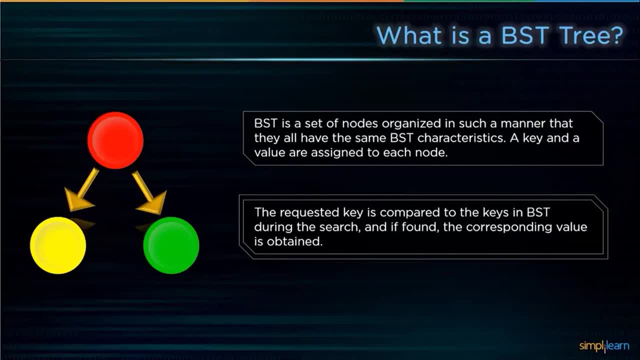 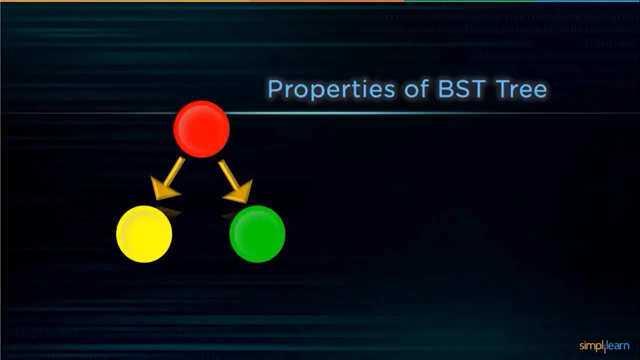 The requested key is compared to the keys in binary search tree. So during search, if the key is found, then the corresponding value will be retrieved. Next up properties of binary search tree. First up, the left subtree of a node contains only nodes. 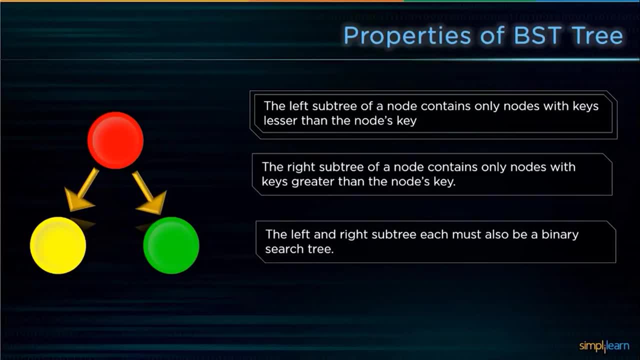 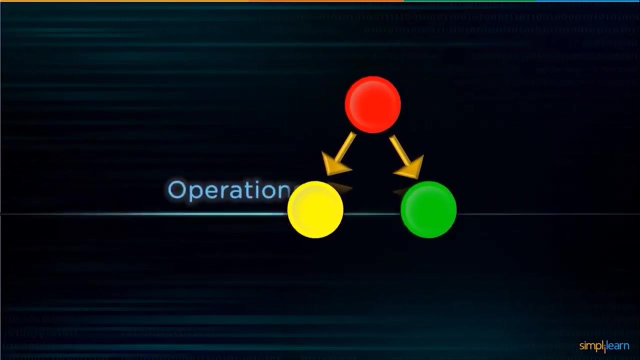 with keys lesser than the parent node Next up. the right subtree of a node contains only nodes that are greater than the parent node. The left and the right subtree each must also be a binary search tree. Next let's discuss what are the operations we can perform. 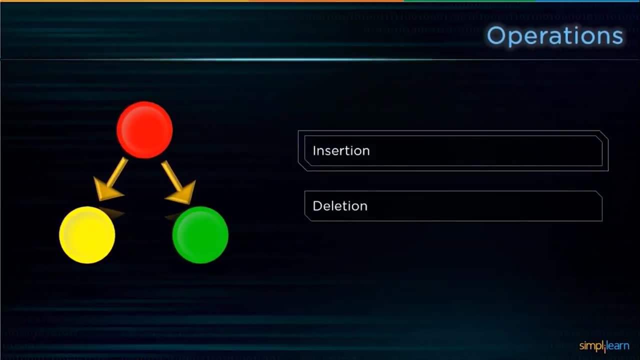 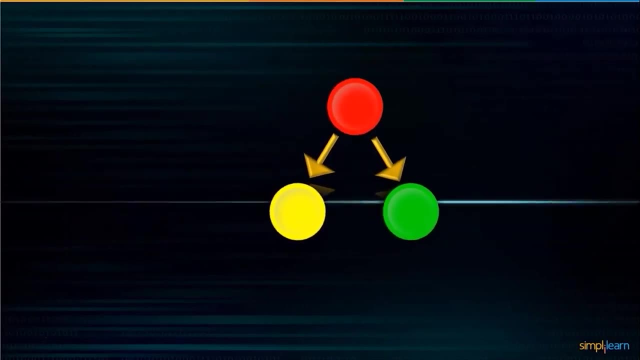 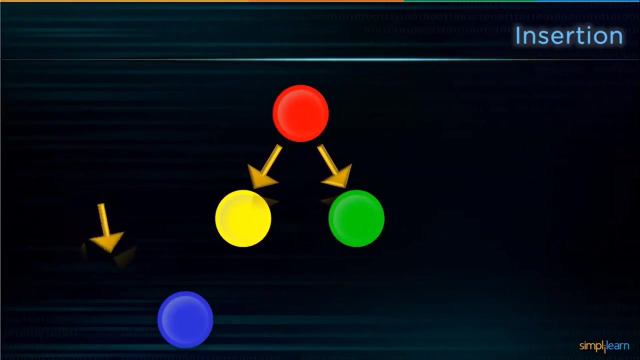 on a binary search tree. First up insertion, Last deletion. Let's discuss them in detail. First up insertion: We can insert a node in such a way so that we obey binary search tree rules. That is, the new node should be either less than the parent node. 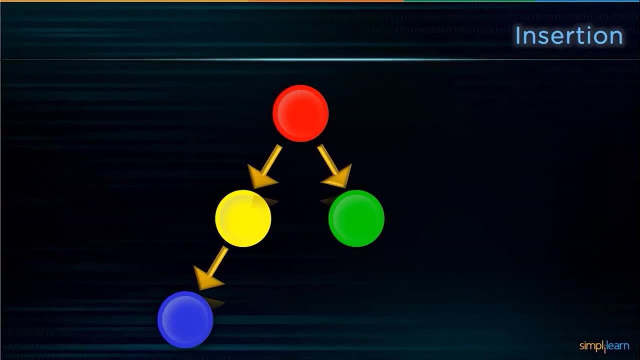 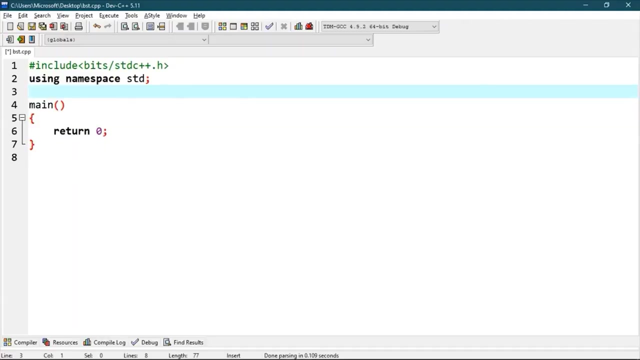 if it's on the left subtree or if it's on the right subtree, it should be greater than the parent node. Let's execute this in the code editor. We will start by creating a class for the binary search tree, So class PST. 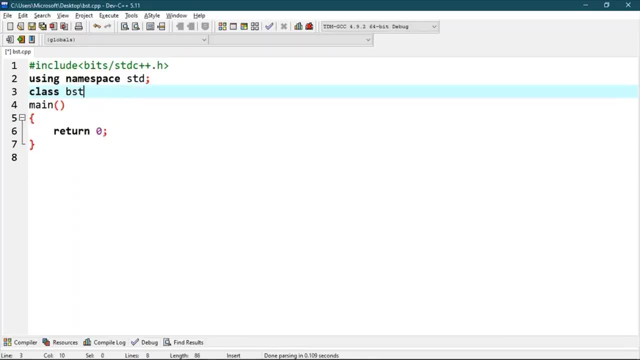 PST int data and PST pointers left, comma right. Next we will define some functions: publicly: public First default constructor And a parameterized constructor. A function to insert the value And a function to first function And a function to first function. 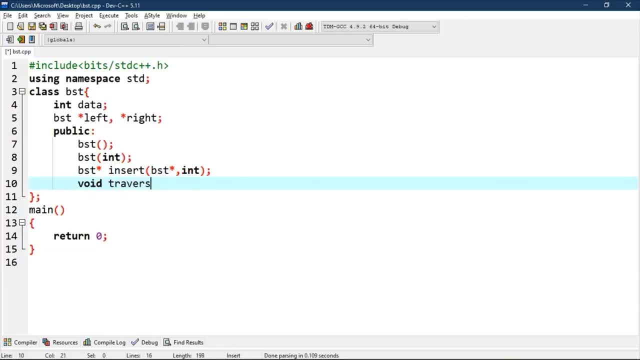 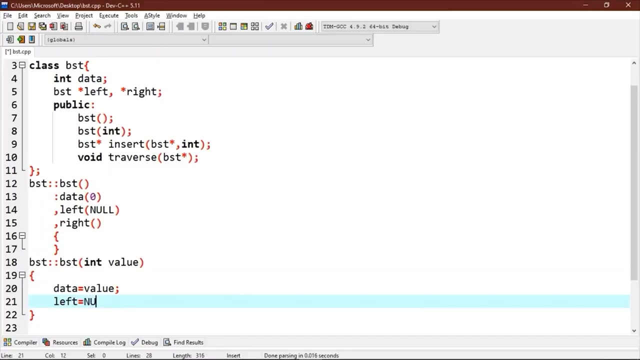 And a function to traverse the node. We can smells vectors once weρί, so that a parameterも. now let's write default constructors definition: BST- BST. now let's write the parameterized constructors definition: BST- int value, data is equals to value and left is equals to null. 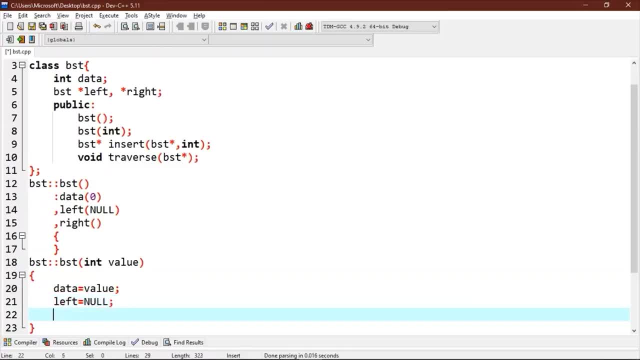 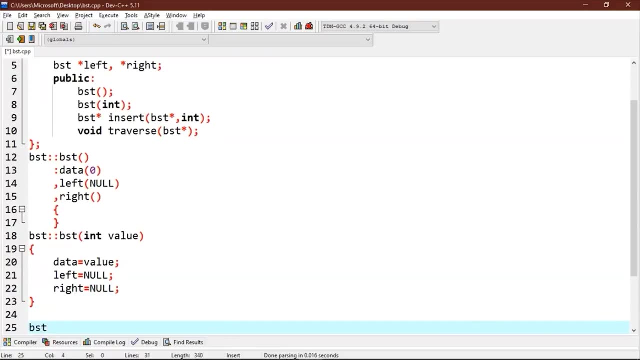 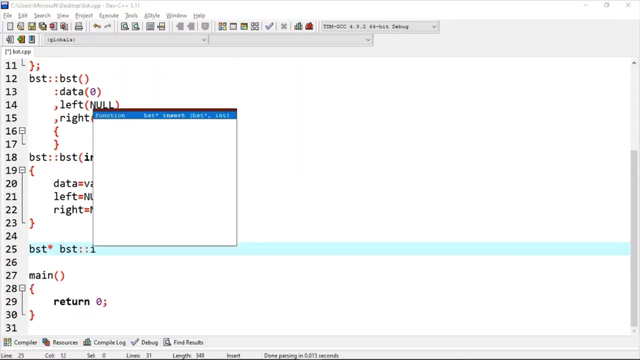 and right equals to null. now let's write the definition for the insert function. so BST, BST, BST, star, BST, root, comma, int value. now we will check if the tree is empty or not. so if root, then we will insert the first node. so we will insert the first node. 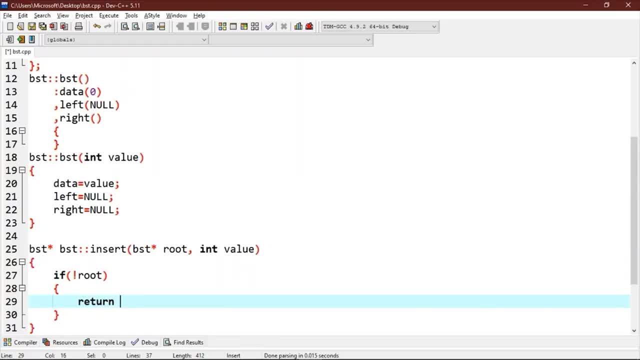 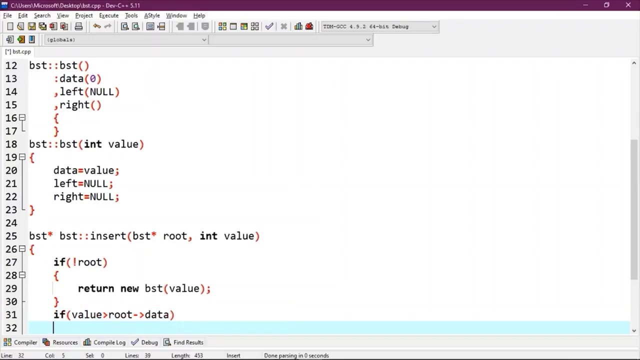 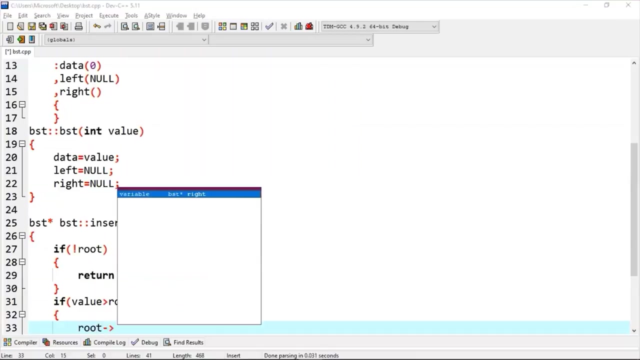 so we will insert the first node now. i will return new BST value. otherwise we will insert the data. so if the value is greater than 1, then we have to insert it in the right subtree. so root right is equals to insert root right comma value. 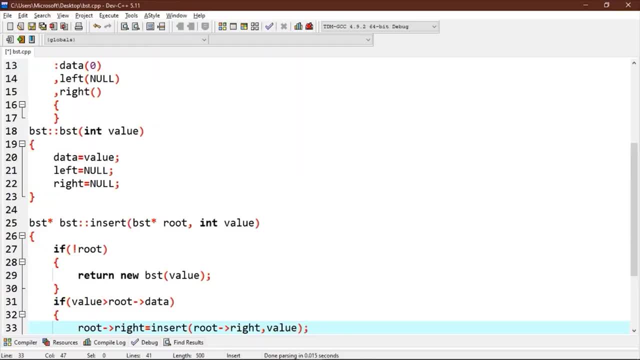 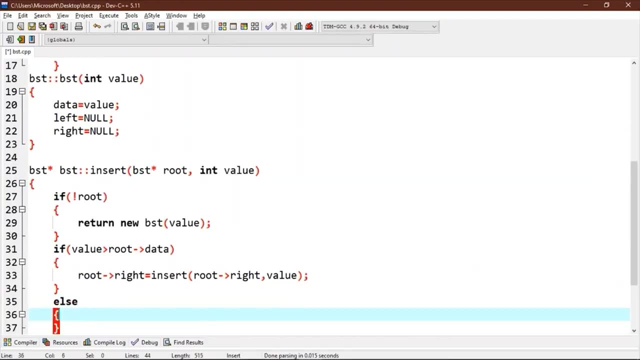 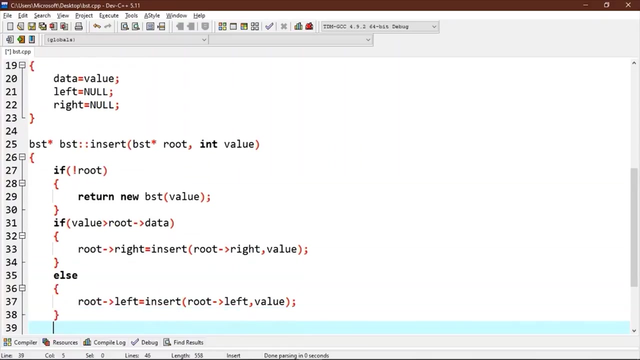 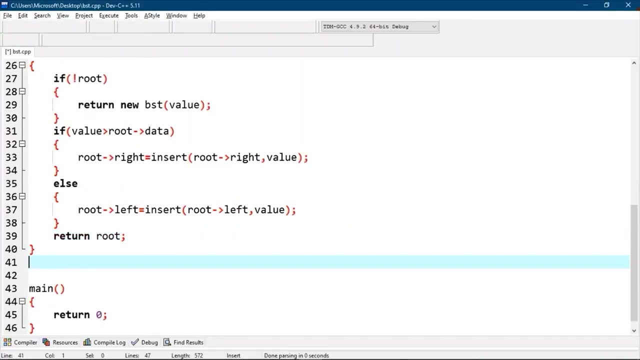 so we have to insert it in the right subtree once else, else is the value which should be inserted in the left side. so root left is equals to insert root left, comma value, and then we will return root. now let's write the traverse function so: void: tst, traverse, tst, star root. 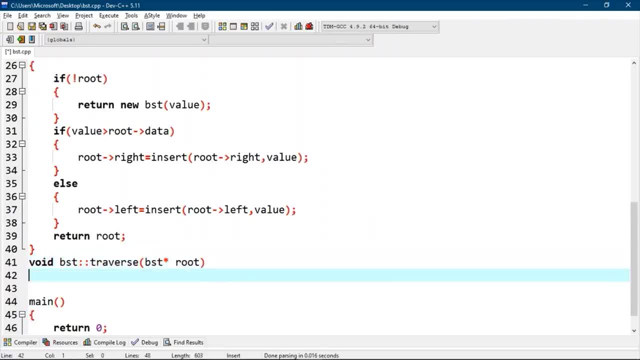 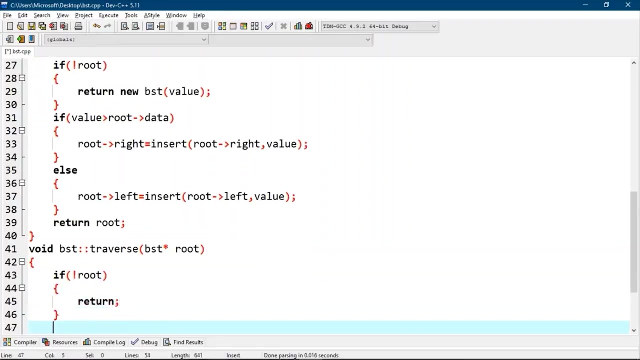 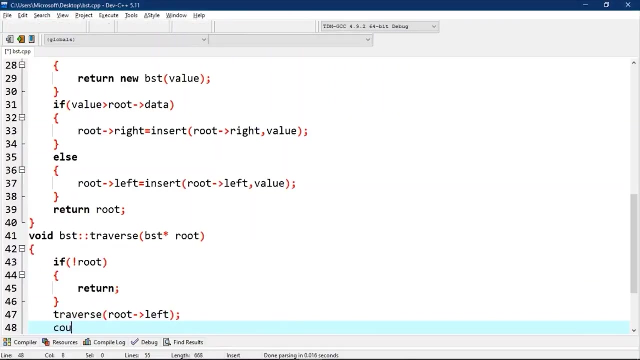 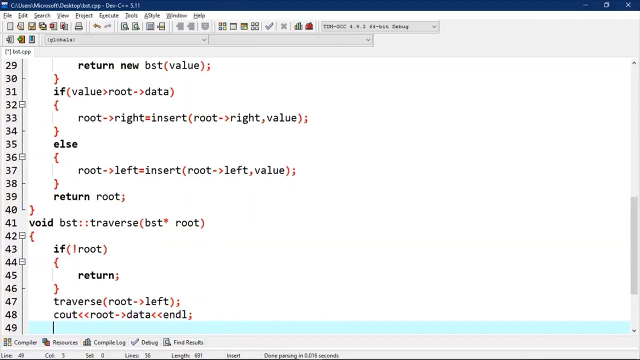 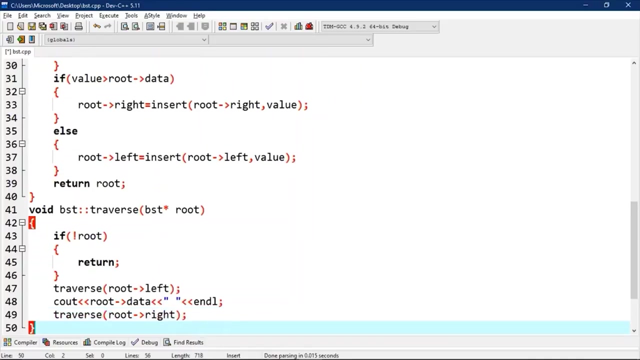 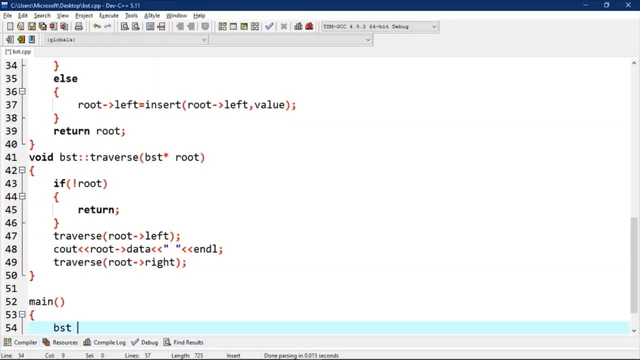 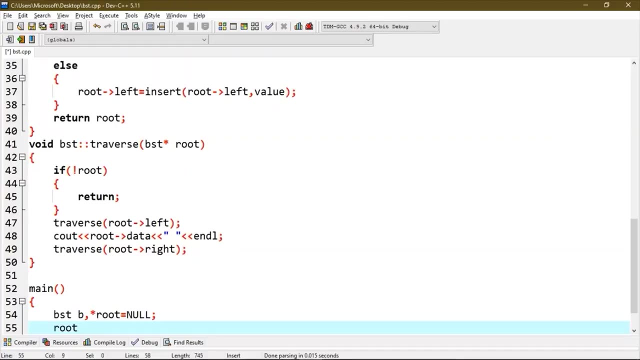 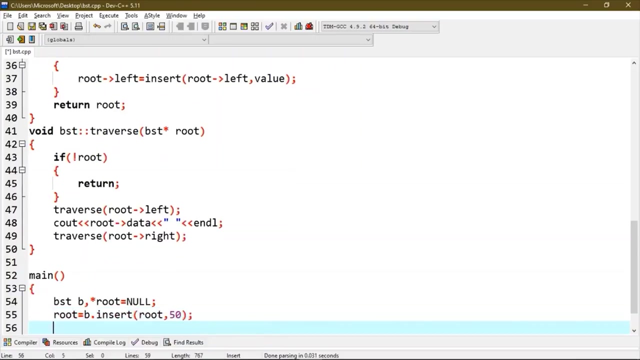 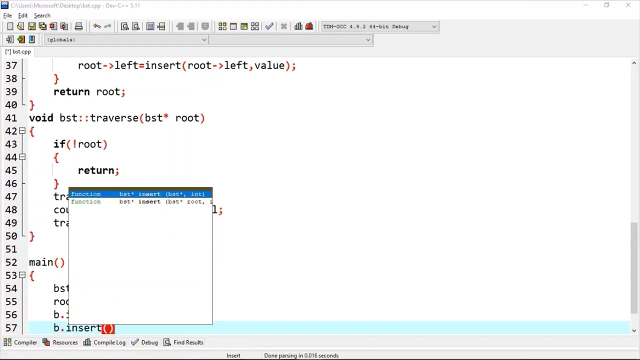 so we will start with an empty tree. so bsd b star root, b star root, b star root equals to equals to null. the root is equals to binsert root comma 50. binsert is equals to root comma 10. binsert is gonna be: 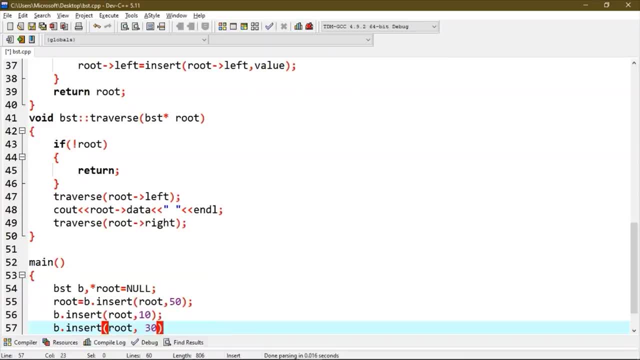 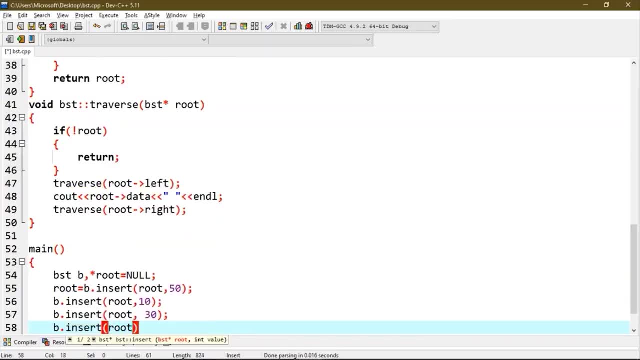 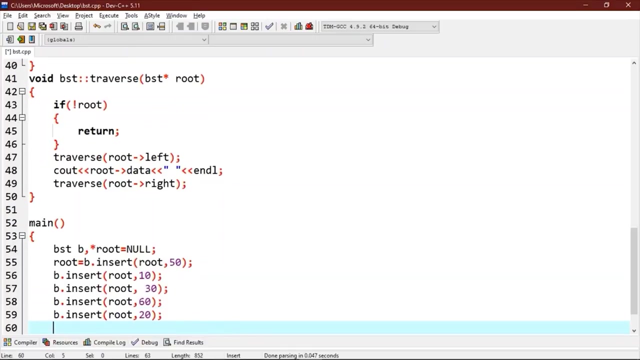 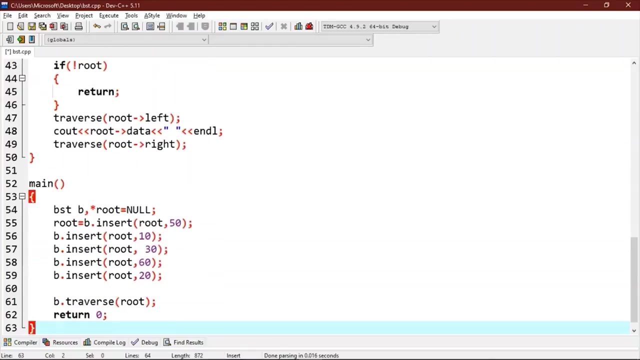 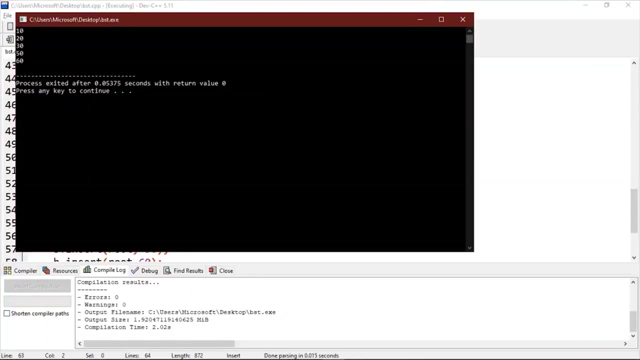 root comma 50 binsert. gonna be root comma 50 binsert. Sorry, we already used 50, so we will use 60 binsert root comma. let's use 20. let's try to traverse this, so b dot traverse root. let's execute this. as you can see, we have successfully. 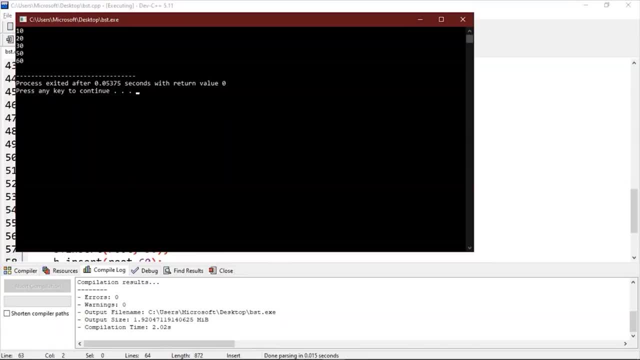 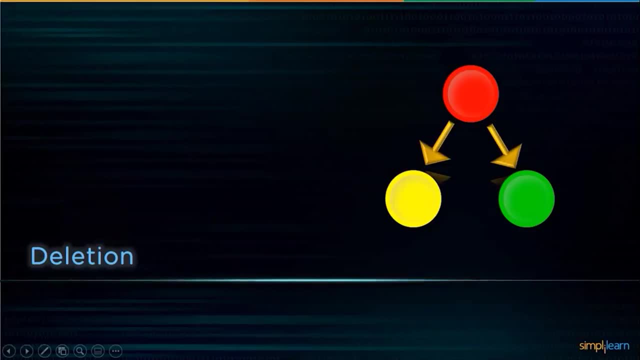 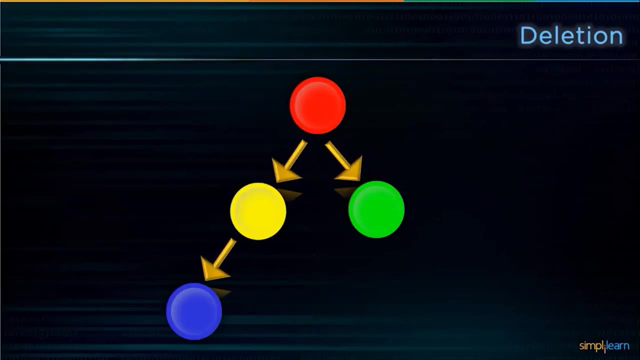 created and traversed our first binary search tree. let's get back to slides at last. deletion. we will delete a node following the binary search tree rules, that is, the value of the left sub-tree should be less than the parent node and the value of the right sub-tree should be greater than the parent node. let's try these in the code editor. 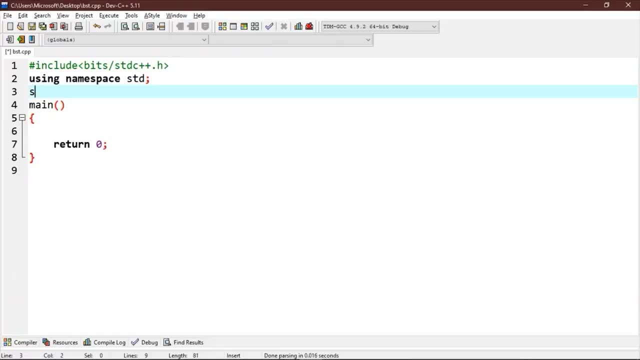 let's start by creating a node. this time we will use structure so struct node: int key struct node star: left comma star. right now we will create a utility function to create a new binary search tree node. so struct node star. new node: int item: struct node star: temp equals to. 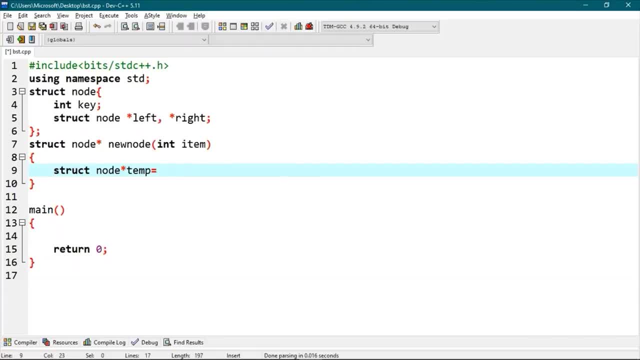 struct: node star malloc. size of struct. size of this and this next, Next temp here we assign the key is equals to item, Temp left Equals to null And temp Right is equals to null. Now let's write a function to traverse the tree. node star root. So if root is equals to null, 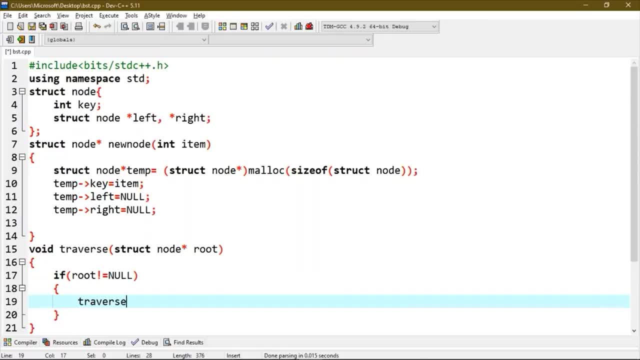 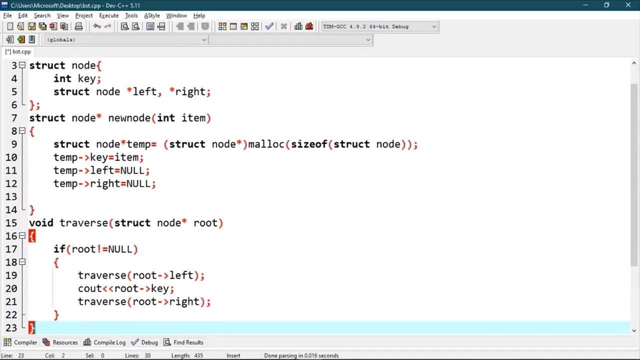 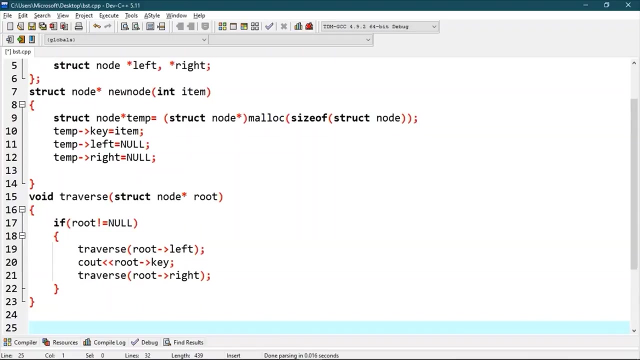 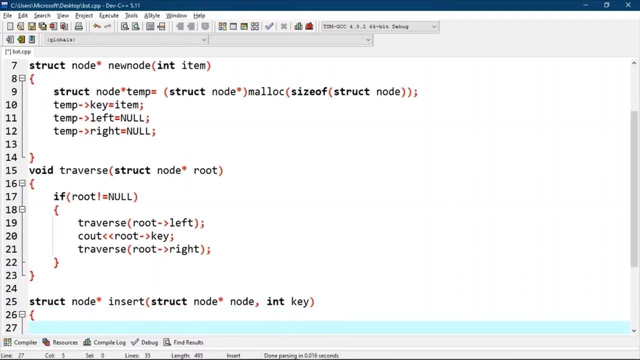 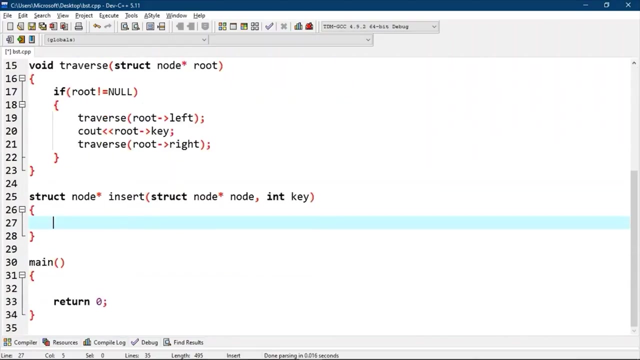 Traverse Root left: See out Root Key: Traverse Root. Right Now let's write a utility function to insert the new node with the given key in the Binary search tree: substruct- node- star- Insert- substruct- node- star. node comma- int key- insert- substruct. So if node is equals to null, 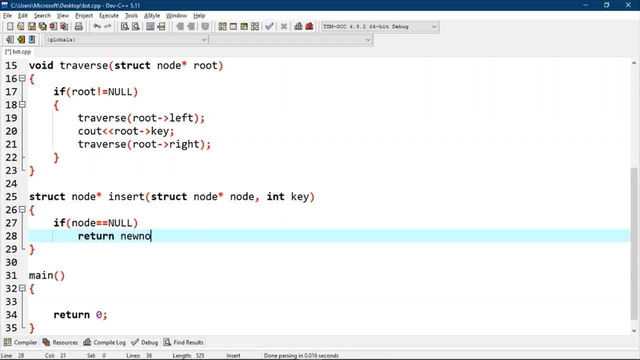 Then we will return new node key key otherwise. otherwise we will recur down the tree. so if key is less than the node's key then we will insert in the left subtree. so node left is equals to insert node left comma key. else node right should be inserting. 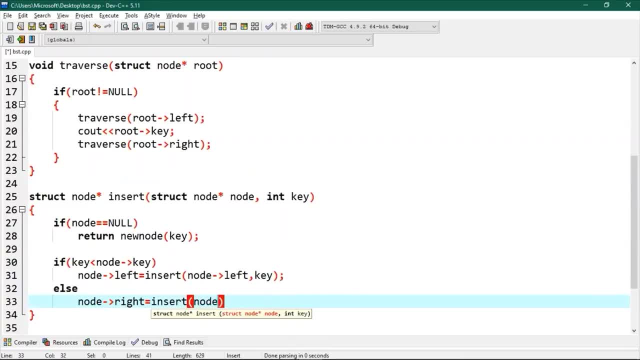 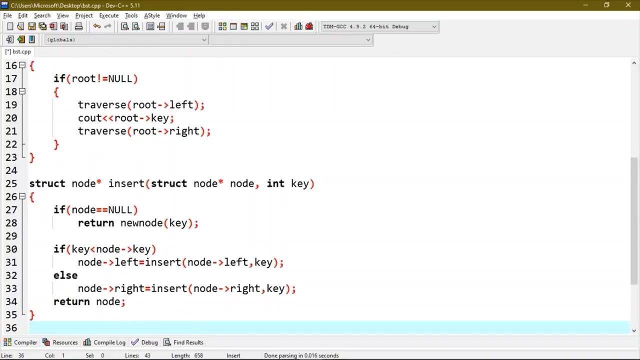 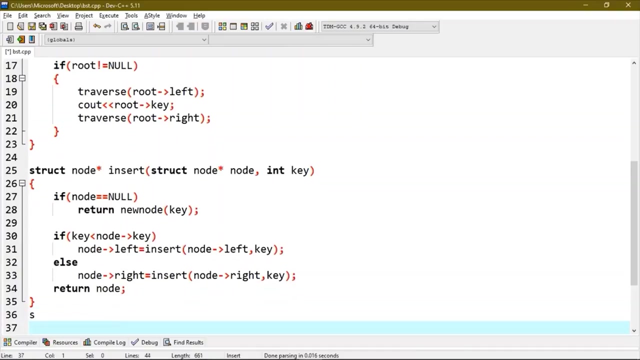 key, left comma key. Now let's return the node. Let's return the node Now. we have given a known empty binary search tree so we have to return the node with the minimum key value found in that tree. so we will start construct node: star min value node. 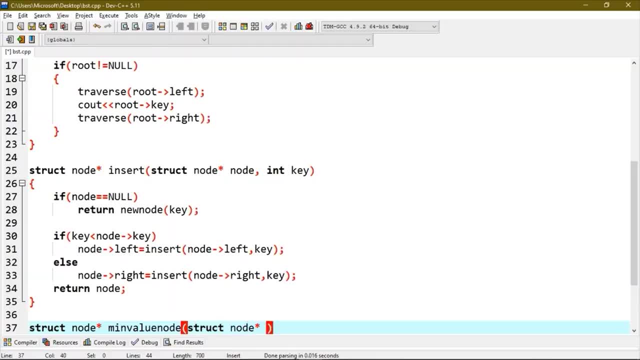 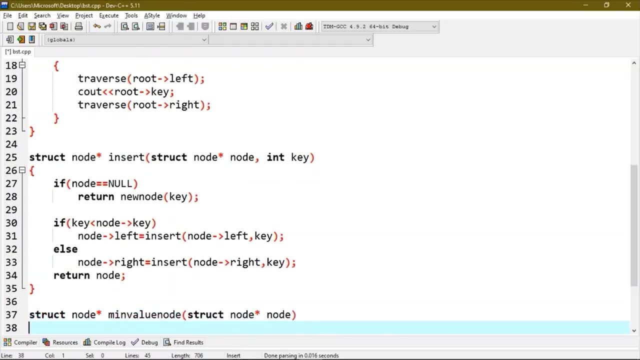 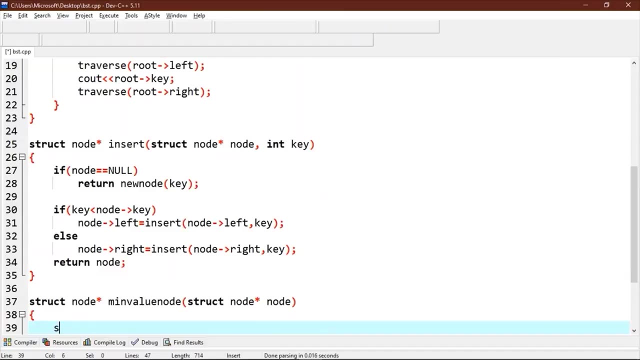 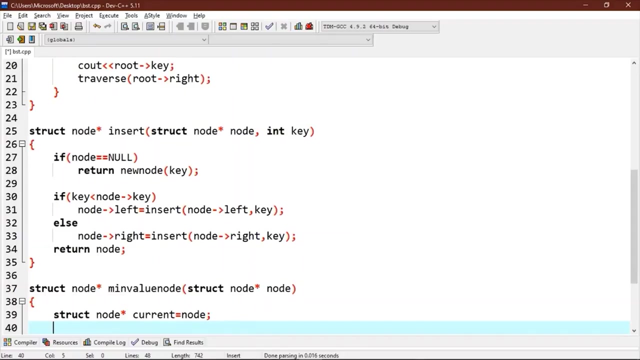 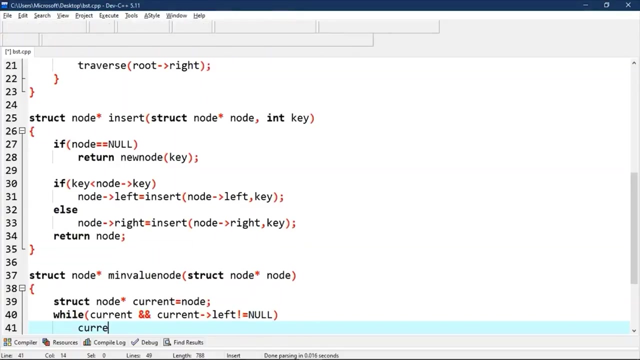 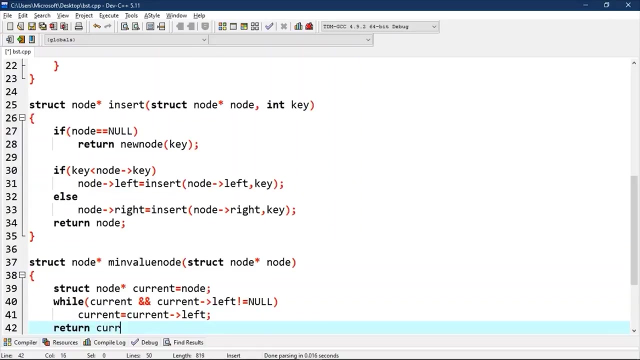 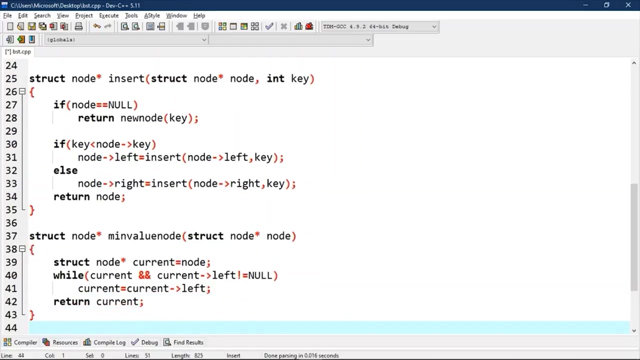 construct node star node. construct node star. current is equals to node, so we will look down to find the leftmost leaf. so while the current and parents left is not equals to null, so current should be equals to current return. current return. current return- current script, script script. 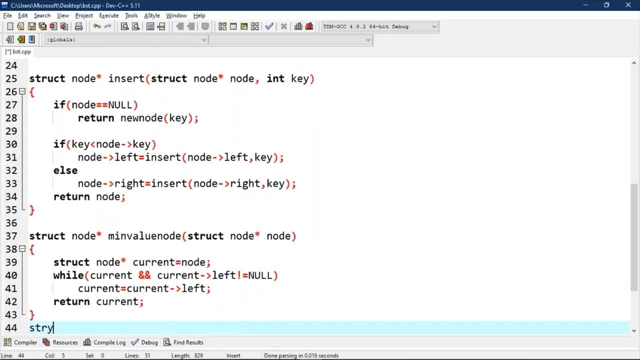 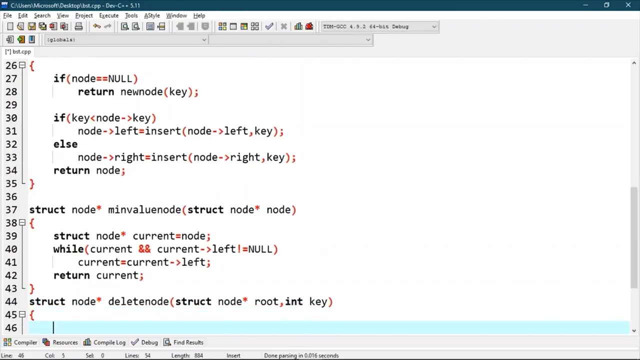 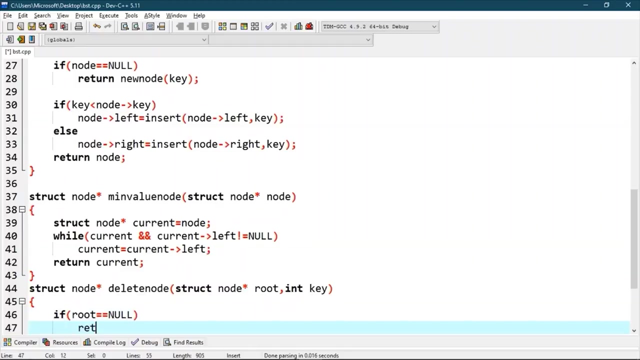 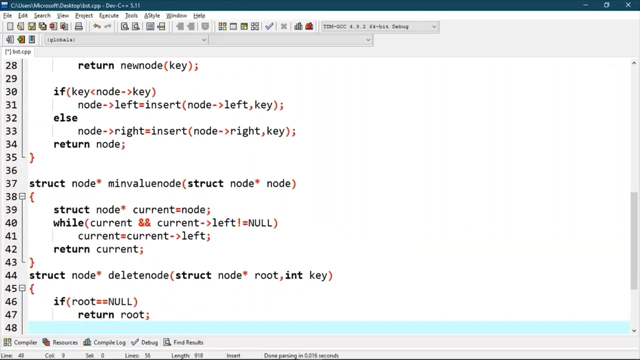 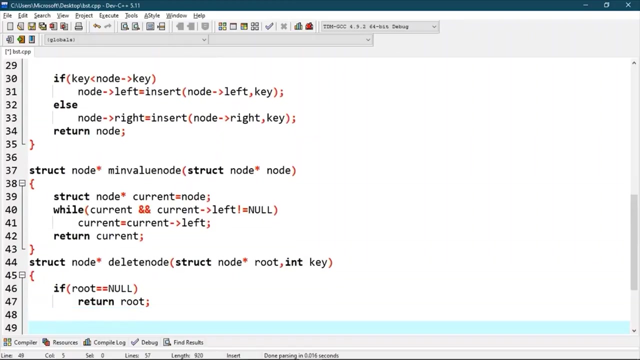 route: route $ mode: star elite node- corrupt node: star root comma forward and key. if root equals to null, return root. now, if the key to be related is smaller than the roots key, then it lies in the left sub-tree. so we will check if key less than root key. 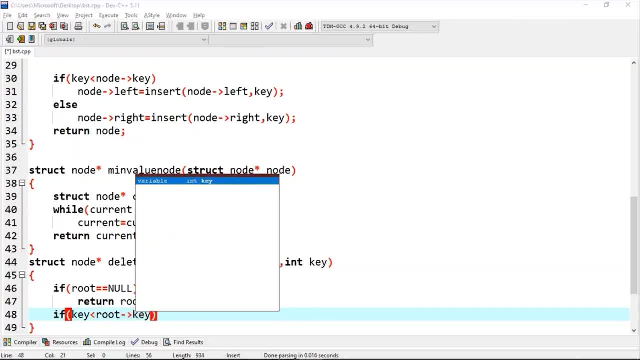 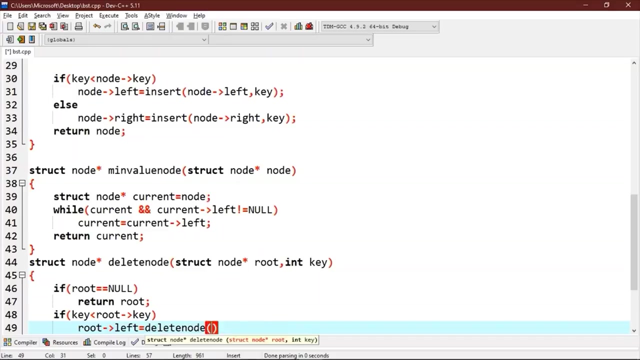 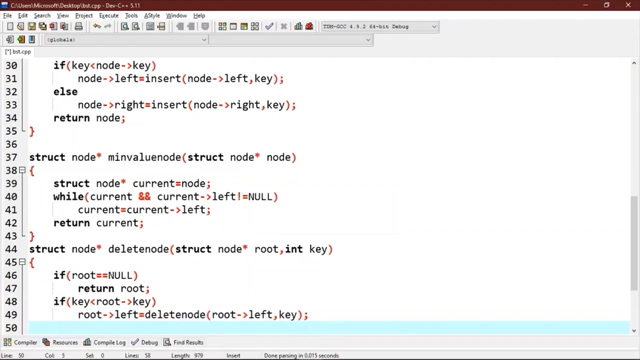 then root left sub-tree, it will be equals to delete node root left key, comma key. now, if the key is deleted is greater than the roots key, then it lies in the left sub-tree. then it lies in the left sub-tree, then it lies in the right sub-tree. 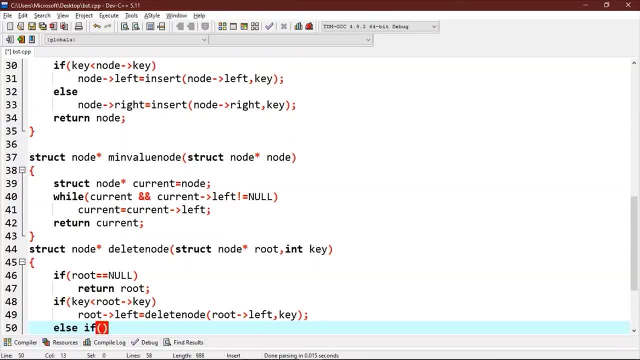 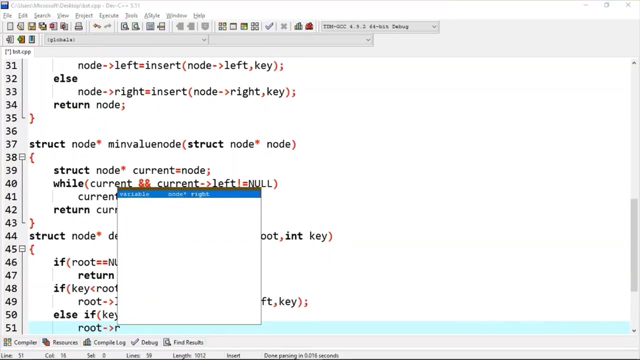 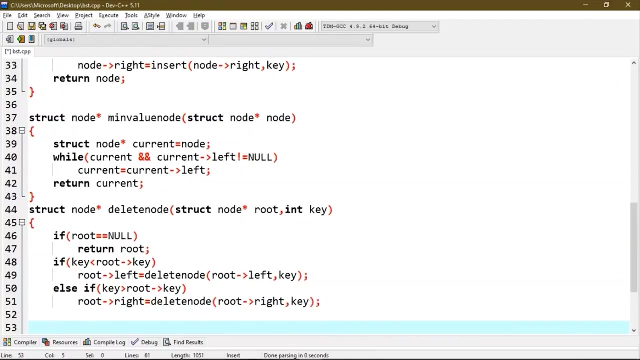 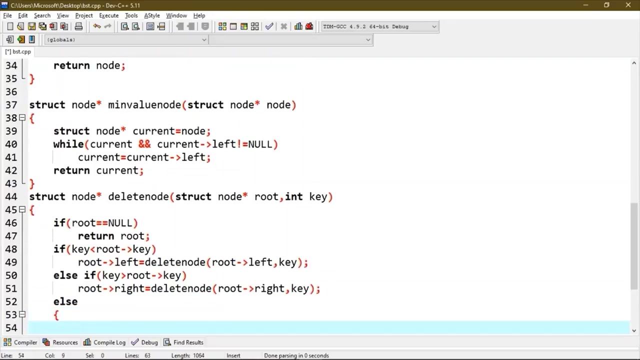 so else, if key is greater than root root right root is equals to delete node root right comma key. else, if, if, if, if roots roots, if roots dot left, dot left, if roots dot left equals to null and root root dot right, dot right is equals to null. 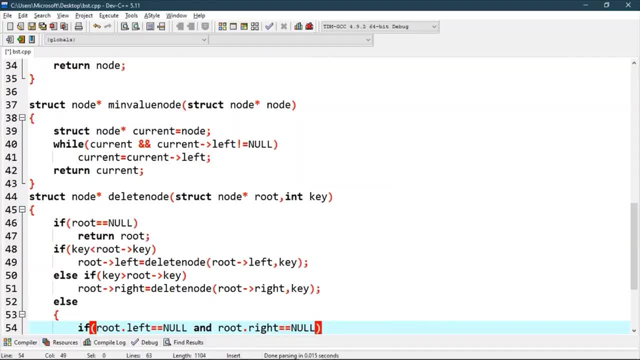 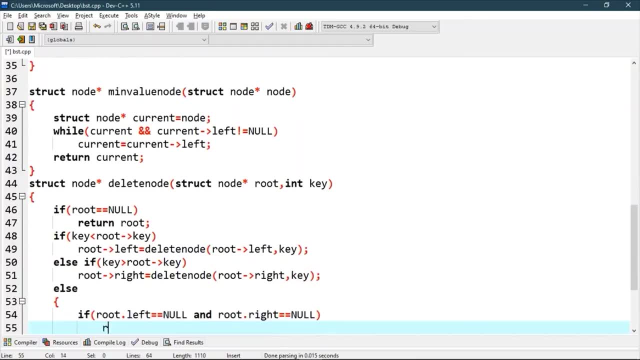 is equals to null. so well, if we can find out that if we want to our parent, we can do so. we can if we have, if we have zero in some and we have this, if we put zero here, then we can. we can if we want to. 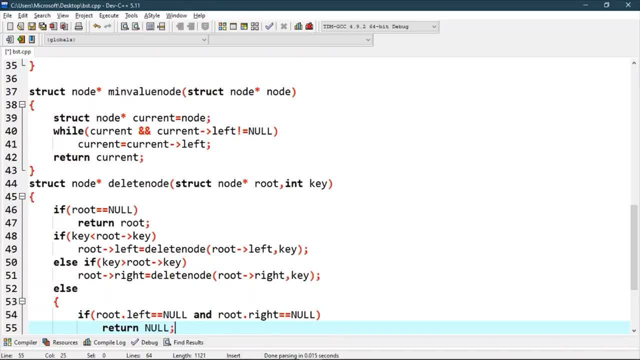 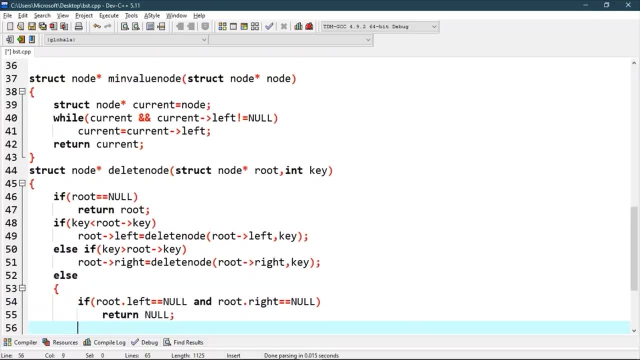 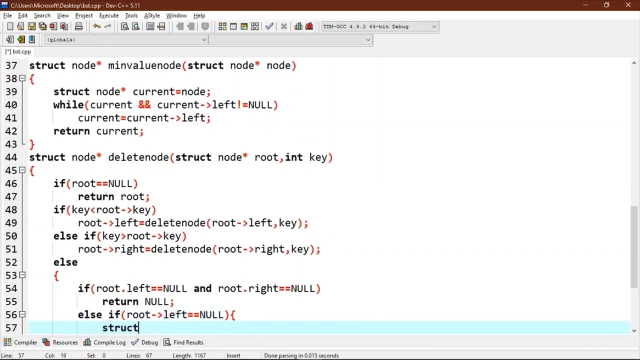 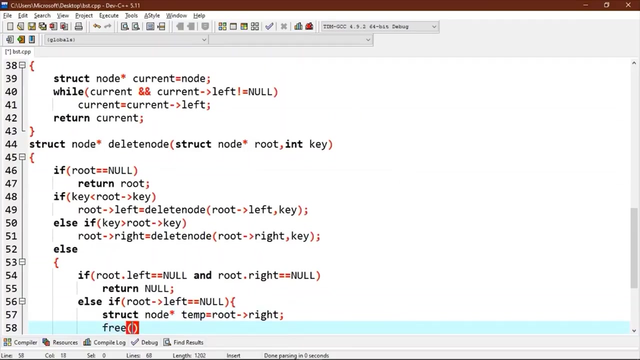 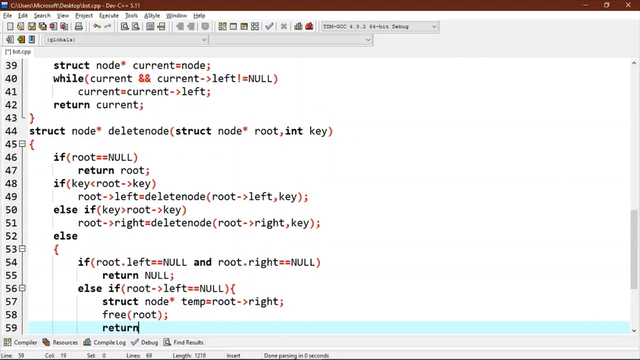 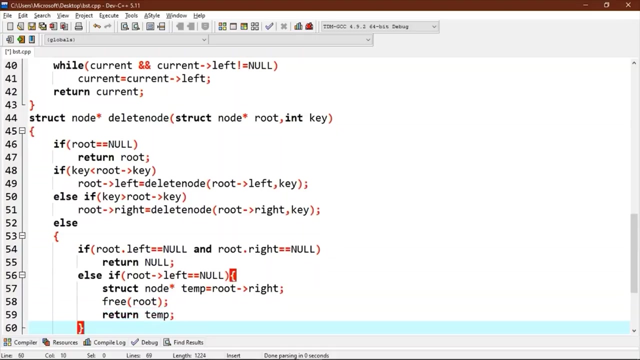 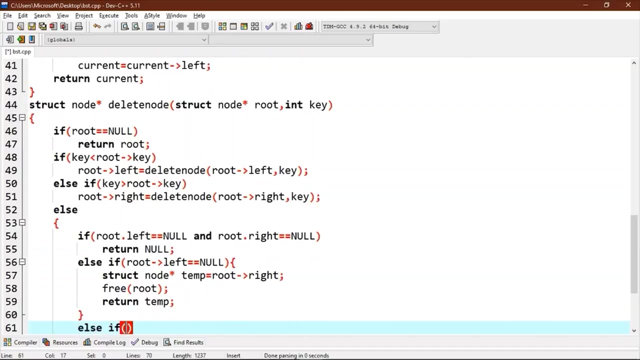 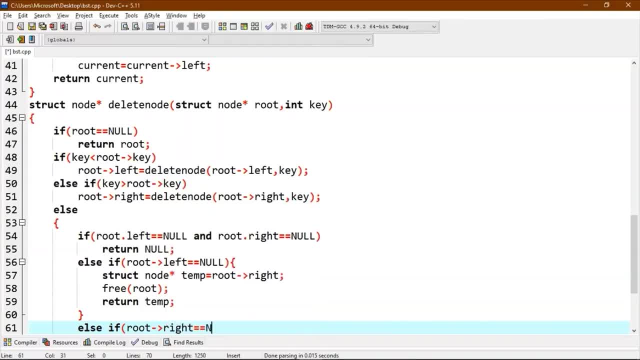 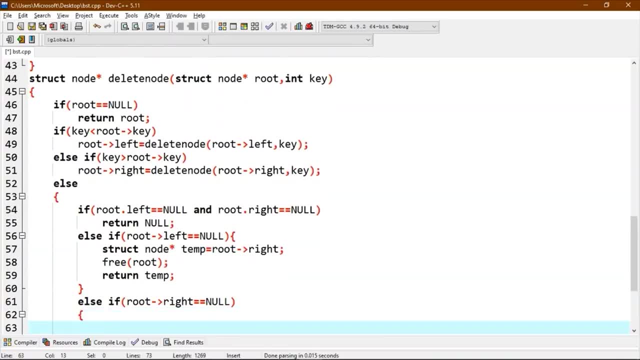 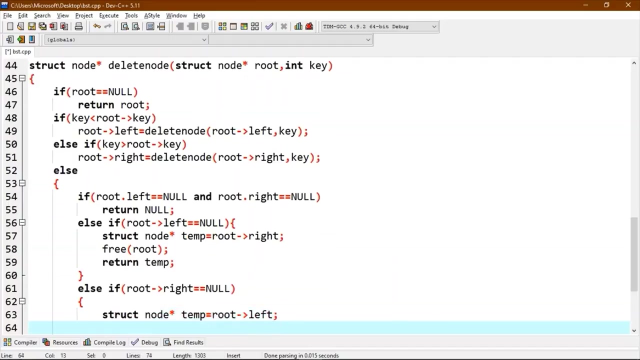 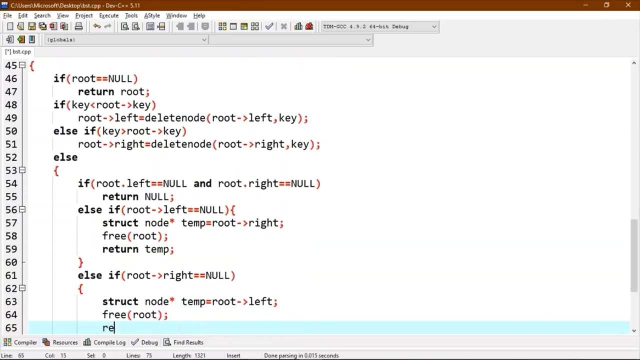 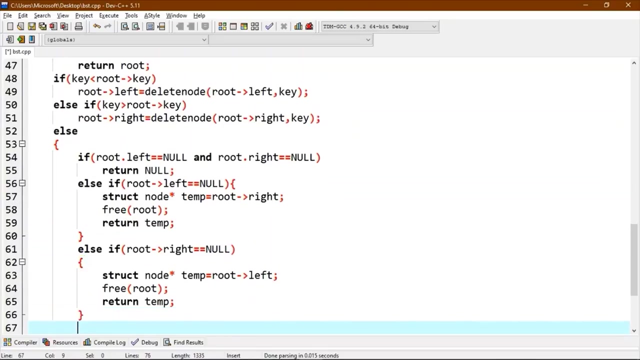 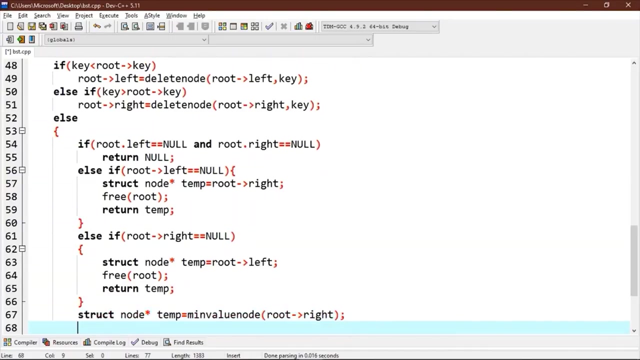 return temp is equals to null, then struct node star temp is equals to root. Now note: with the two children get the inorder successor smallest in the right subtree. so struct node star temp is equals to min value. node root right is equals to temp. now we will copy the inorder successor's content to this node, so root is: 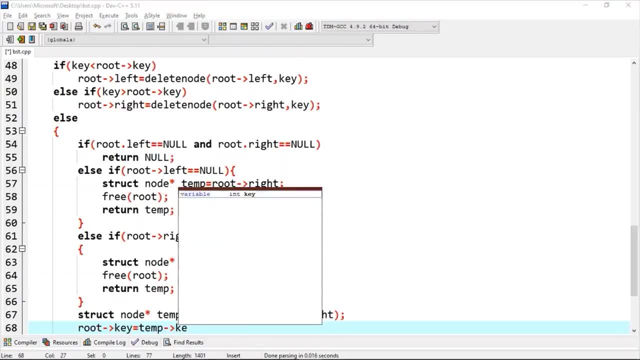 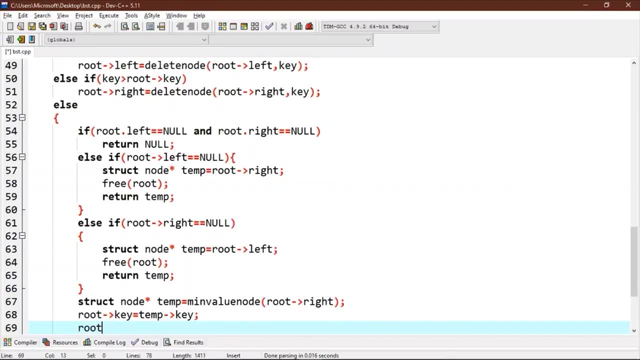 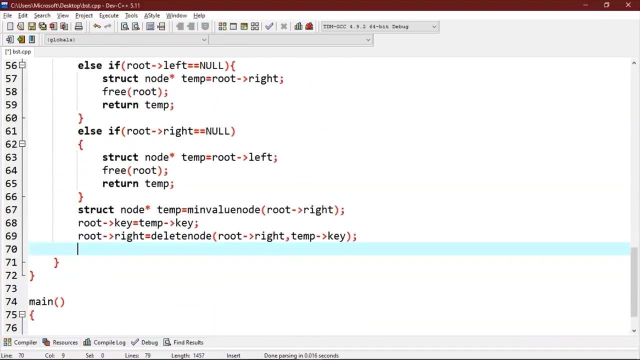 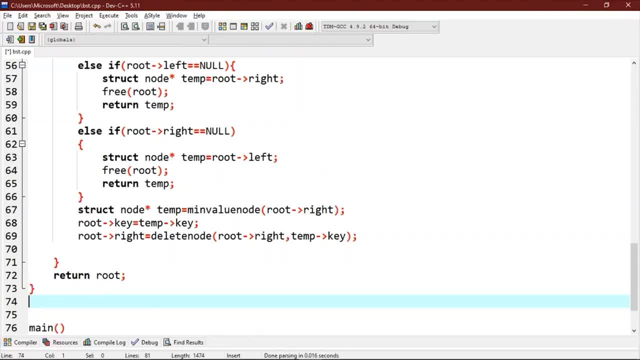 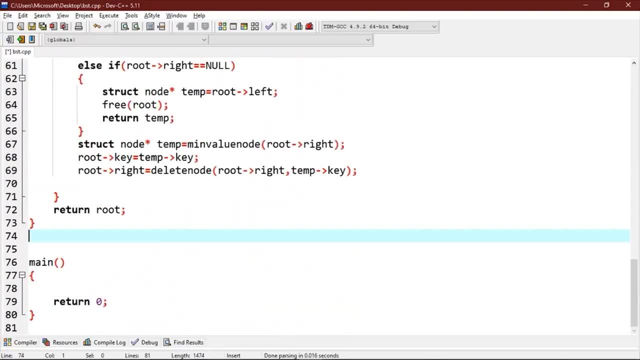 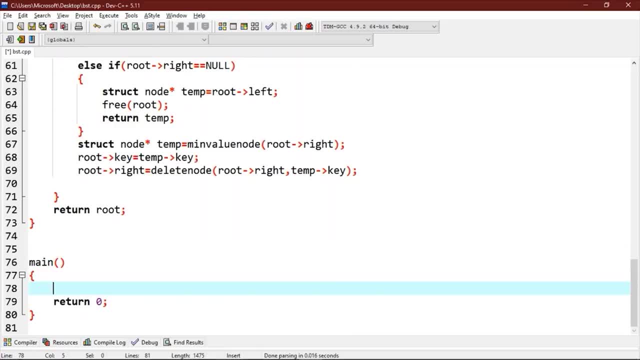 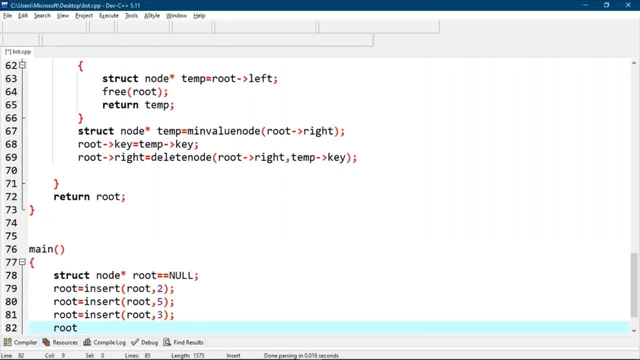 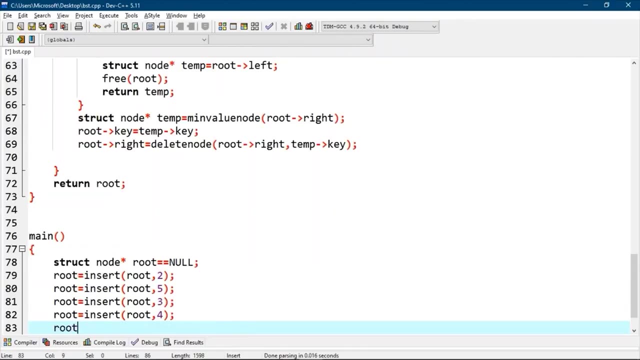 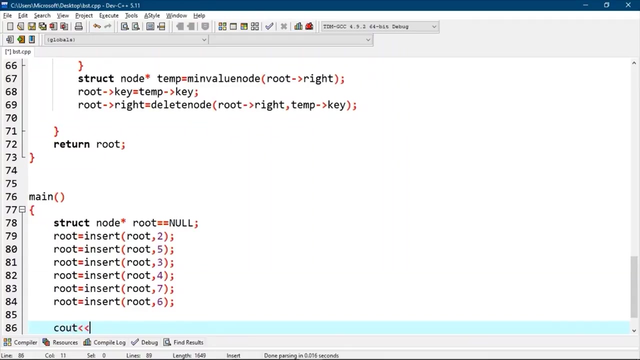 So root is equals to insert root comma 4, root is equals to insert root comma 7 and root is equals to insert root comma 6.. Let's try to traverse this. so cout traversal of the given tree. Let's start traversal of tree. 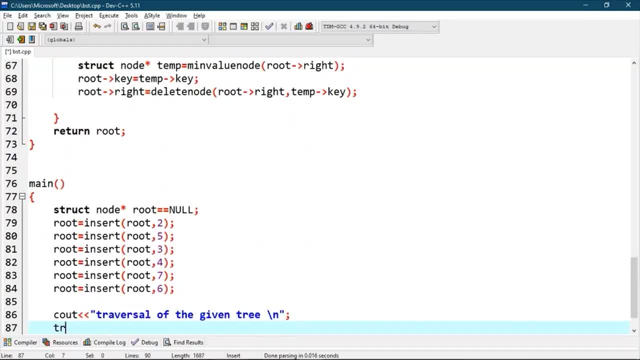 Verise to see pattern under grief. savior. if trying to go the right way Now where we find root of cout traversal, How to get a part ofaneellog, Let' me show you. Let me take a bit of data. can you see what's on the right side? 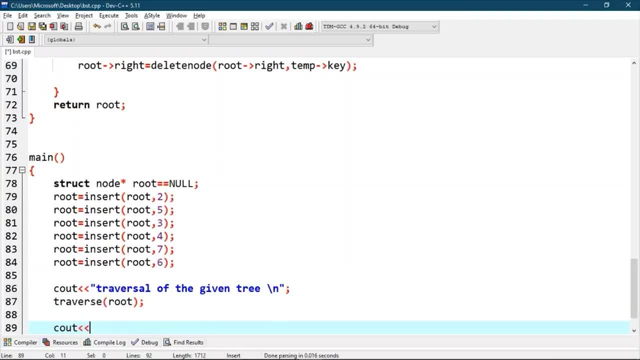 Now move a little bit the thing. Now move a little bit to the left side. Now move a little bit to the left side. now move, and we need again the same, the same. first we will delete a value to see out. delete to our root is equals to delete node. 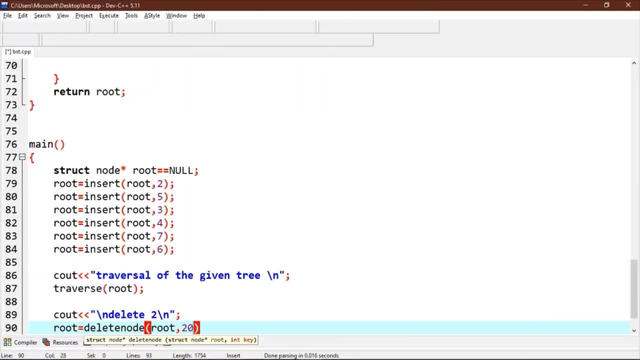 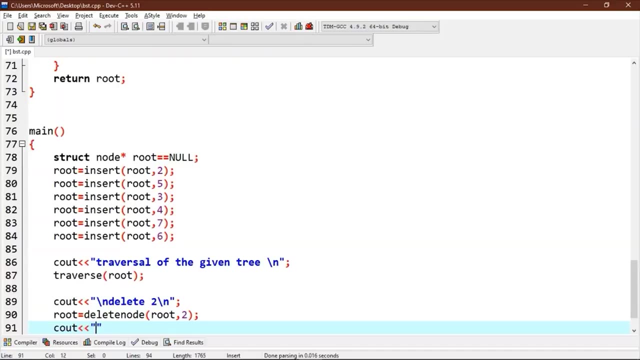 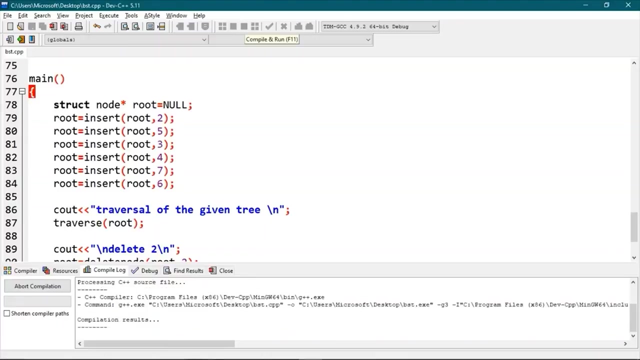 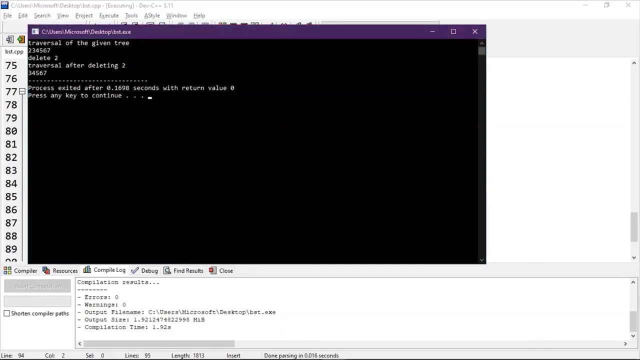 root comma. to of see out our root is equals to delete node, traversal, traversal, traversal, after, after, after deleting to traverse, to traverse, to traverse, root. let's execute this. as you can see, we've successfully deleted to and traverse the tree again. let's get back to our slides. 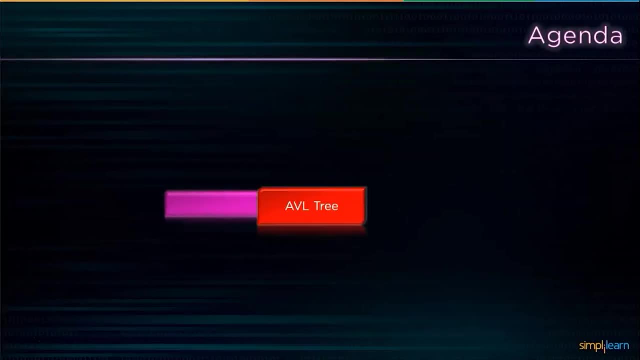 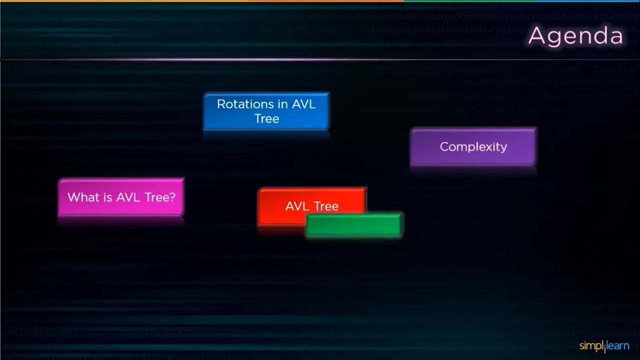 in this we will talk about avial trees. we shall begin our session by what is an avial tree. then we'll discuss various rotations we can perform to balance avial tree trees. then we will discuss the complexity of avial trees. after that we will try various operations on them, like insertion, deletion. finally, we will sum. 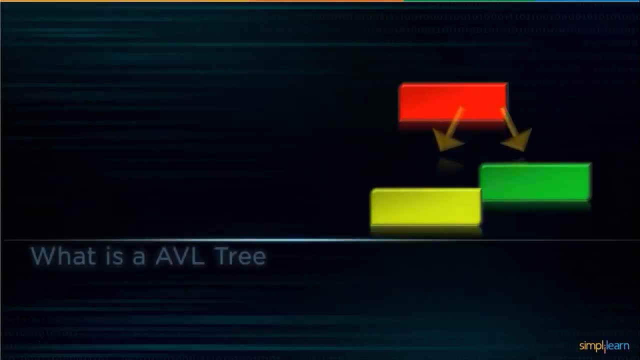 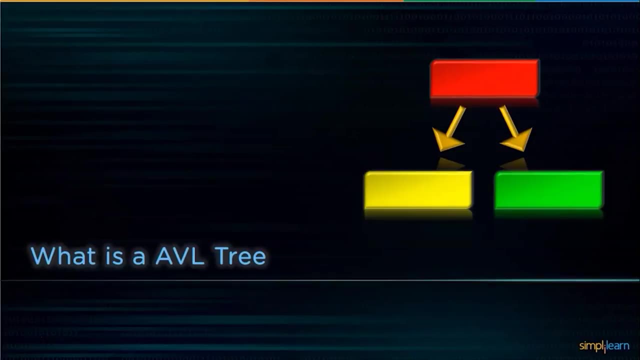 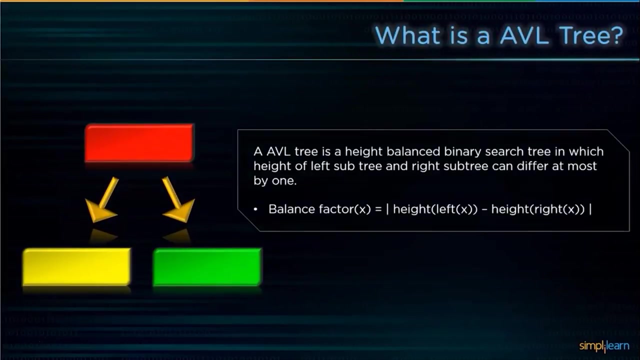 up what we have learned from this session. but before we begin, make sure you subscribe to our YouTube channel and clicked on the bell icon below so you never miss an update from simply learns YouTube channel. so let's get started with introduction to a alias. an alien tree is a height balance. binary search. 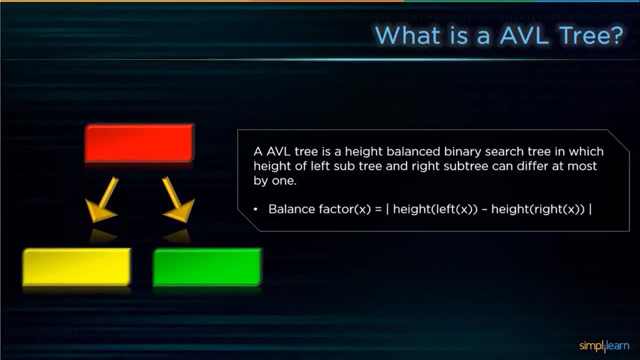 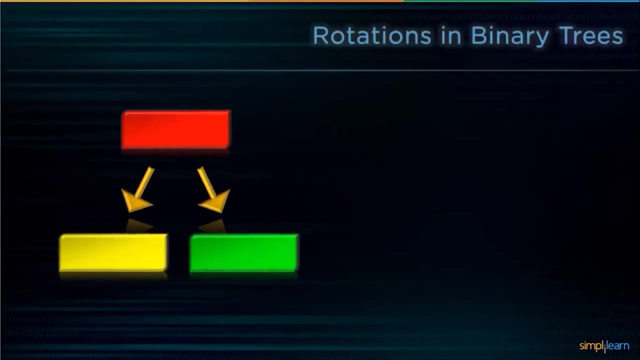 tree. for each node, we have to make sure that the height of the left subtree and the right substrate can differ by at most one. we can calculate this balance vector by subtracting the height of the left subtree from the height of the right subtree. now let's discuss various rotations we can perform on avial trees. 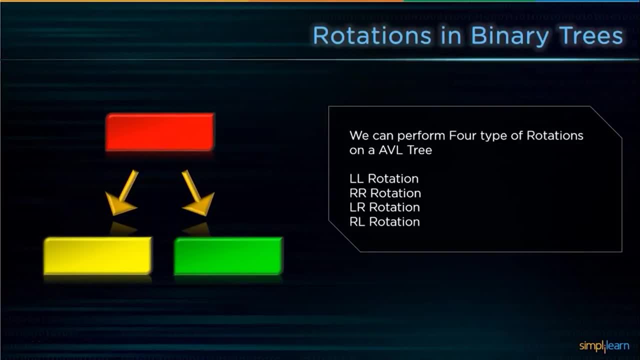 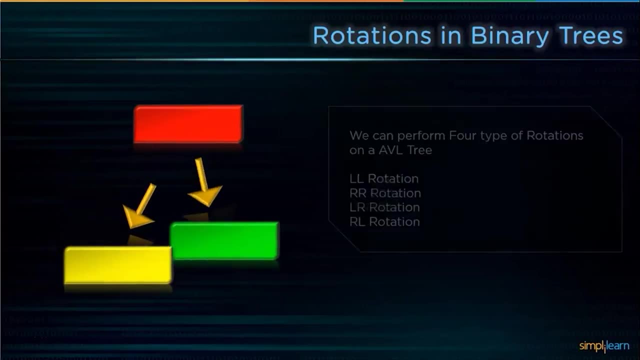 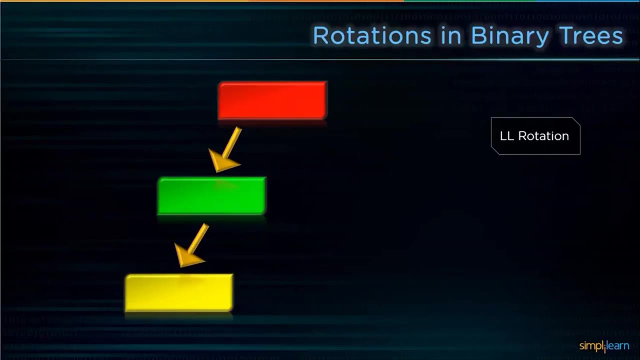 first up, LL rotation, next RR rotations, Next LR rotation, At last RL rotation. Let's discuss them in detail. First up, LL rotation. It is a clockwise rotation. when a node is inserted on the left subtree of the left subtree of a node, then we apply this rotation to balance the tree It is applied on. 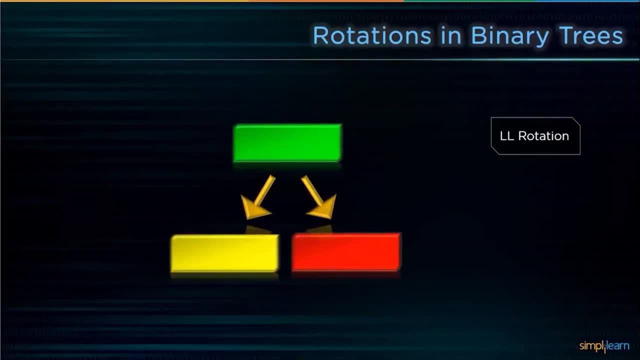 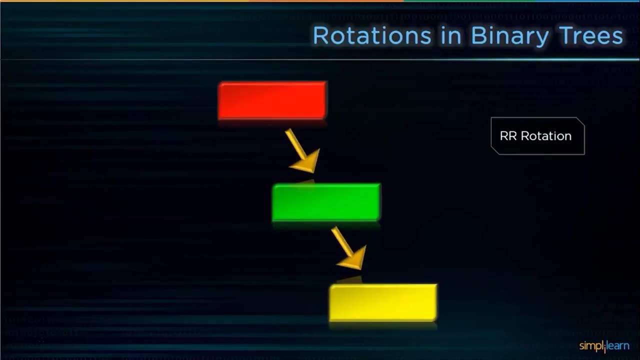 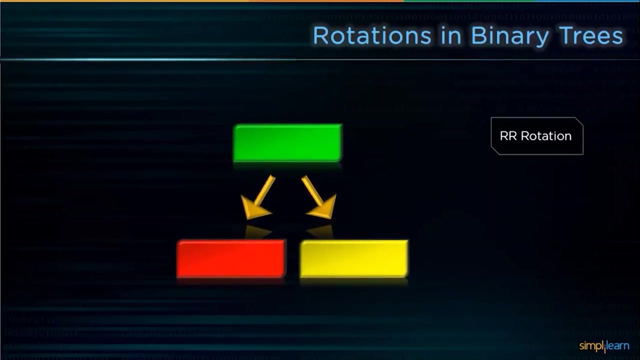 the node below the balance factor 2 node, that is, we will apply right rotation on the green node. Next RR rotation. When a node is inserted into a right subtree of the right subtree of a node, then we perform RR rotation. It is an anticlockwise rotation which is applied on the node below a. 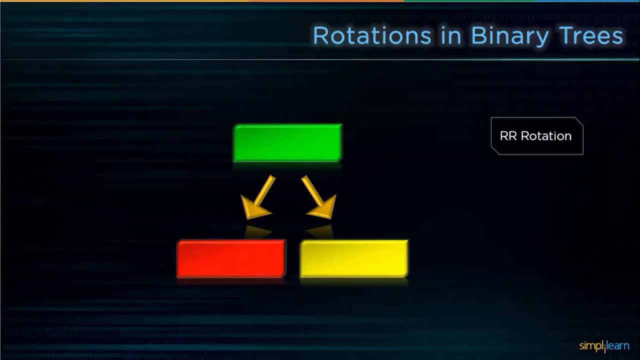 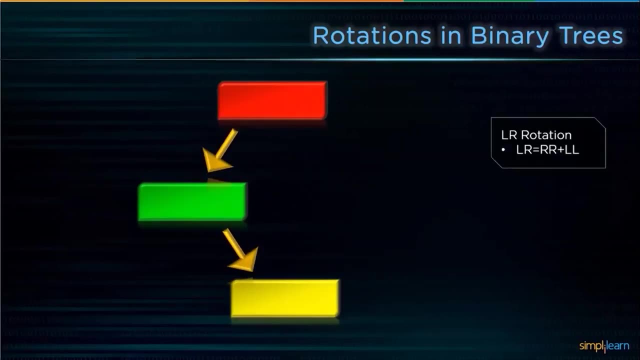 node having balance factor minus 2, that is, we will apply it on the green node. Next up, LR rotation: When a node is inserted into right subtree of the left subtree of a node, then we perform LR rotation. It is a combination of RR and LL rotation. First we will apply RR rotation on the green and yellow node. 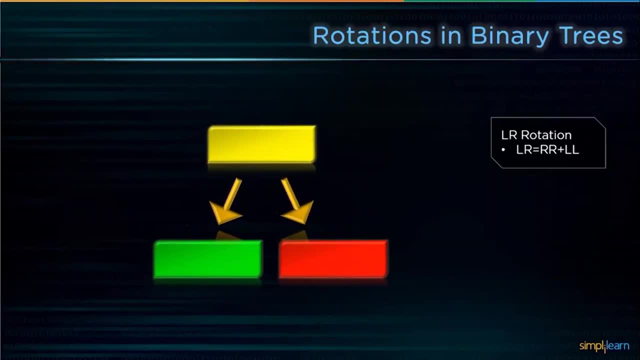 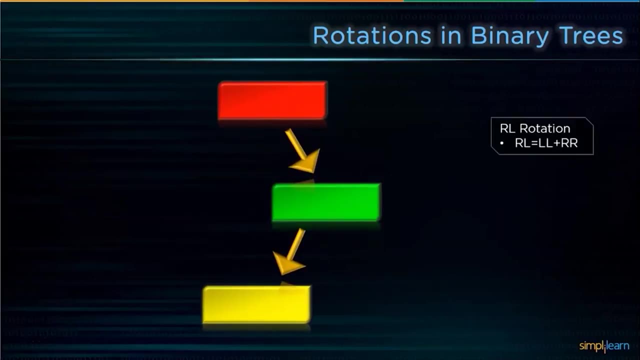 After this, red node is still unbalanced, so we will perform LL rotation on the yellow node. Finally, RL rotation. When a node is inserted into the left subtree of right subtree of a node, then we perform RL rotation. It is a combination of LL and RR rotation. First we will apply. 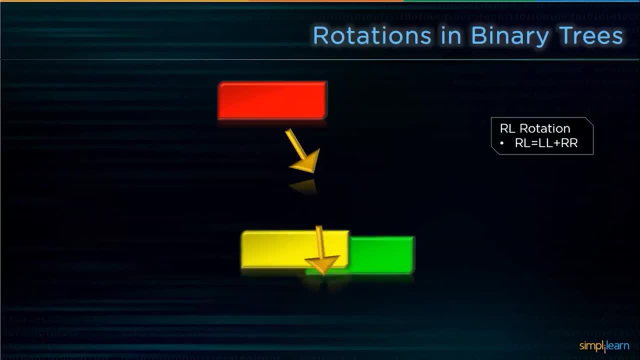 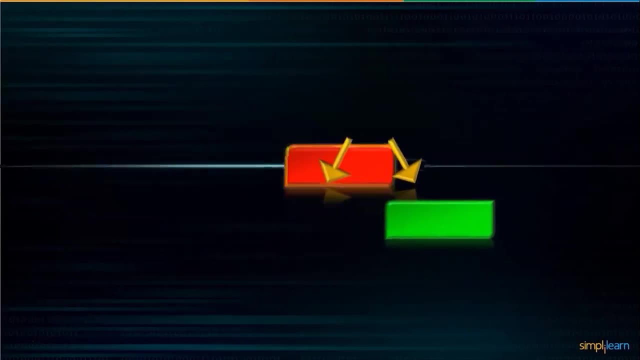 LL rotation. Lastly, RL rotation is applied on the left subtree and we will perform RL rotation rotation on green and yellow nodes. After this, the red node is still unbalanced, So we will perform RR rotation on the yellow node. Now let's discuss complexity of avial trees. First, up space. 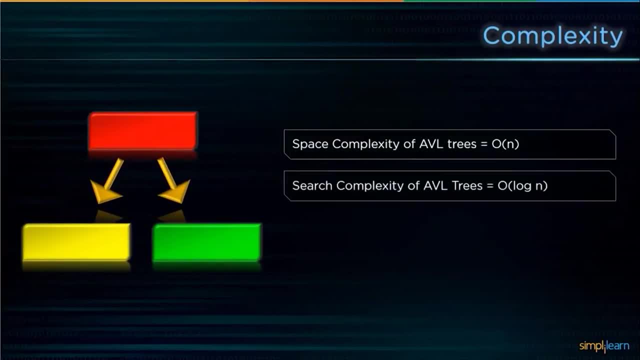 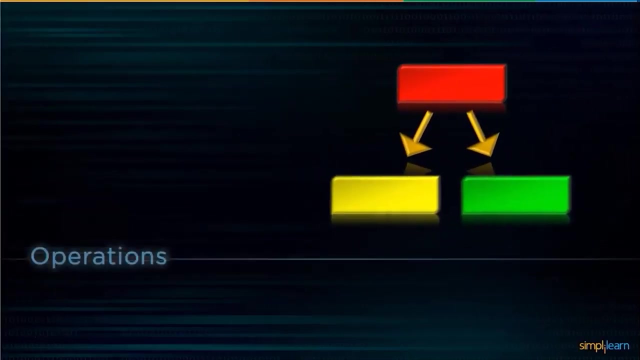 complexity is a bigger of n. Next up avial tree offers a complexity of bigger of log n for searching. Next up avial trees offer a complexity of bigger of log n for insertion. Finally, avial tree offers a complexity of bigger of log n for deletion. We have now introduced an avial tree and rotations. 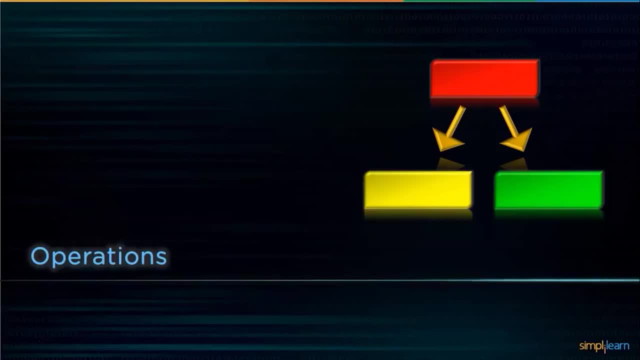 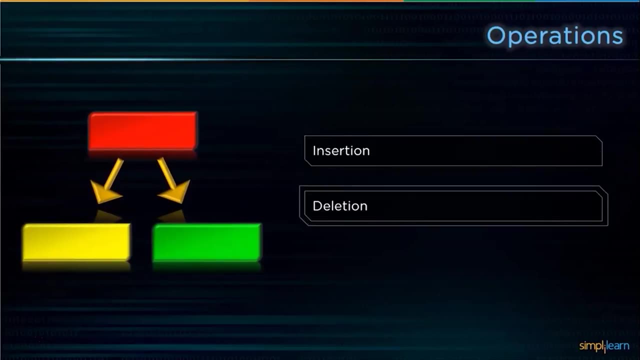 on it. Now let's discuss some of the operations we can perform on avial trees. First up, insertion and deletion. Let's discuss the avial tree and its rotation. Thank you very much, sir. Good, good, Thank you, It's my pleasure. 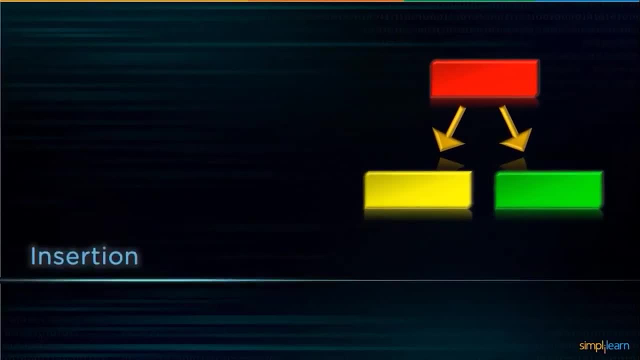 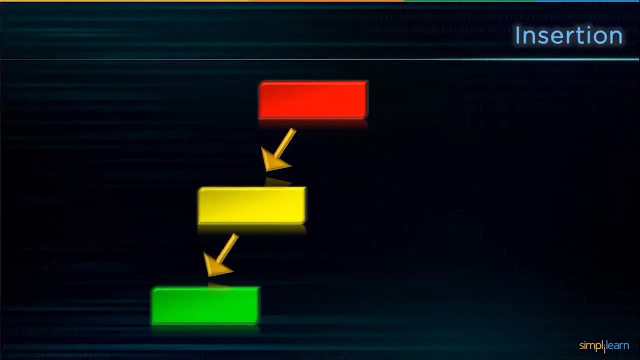 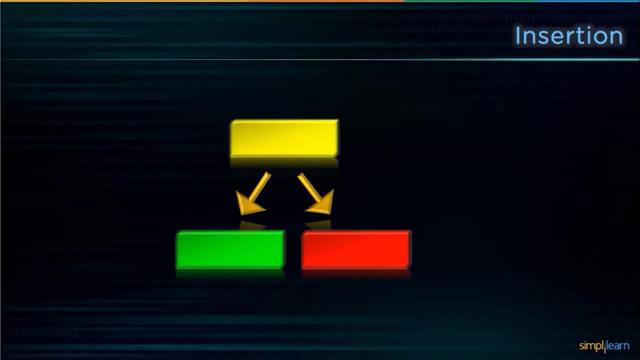 You are welcome, Thank you. Thank you them in detail. first up insertion: we will insert a node following binary search tree rules. then we will check if the nodes are balanced or not. if they are not, then we will balance it by using suitable rotations. now let's try these operations in a code editor. let's start by creating a node. 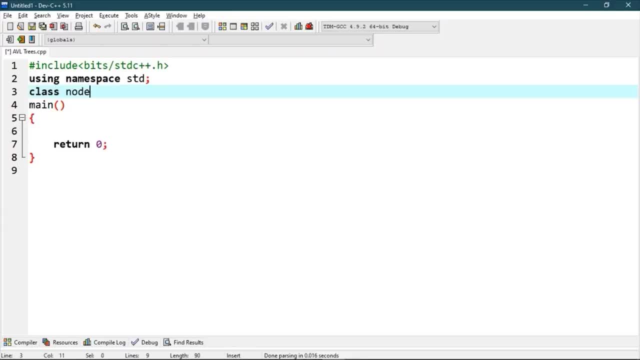 to create a node, we need a class node. we will create its member as public and key: code: star left, code star right and height. now let's write a function to get maximum of two integers, so int max, int a comma, int b a comma and p. now let's declare a utility function to get maximum of two integers, so int max. 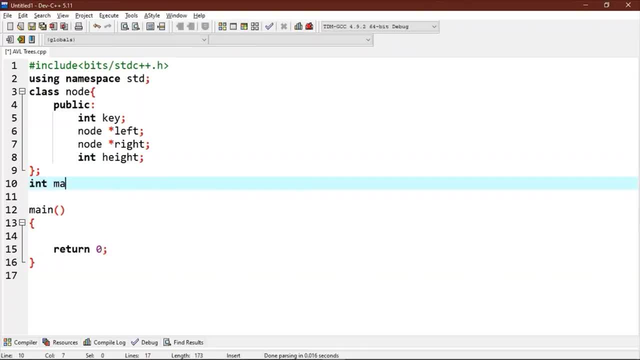 a comma: int p now. if it works NOW for our all node. Now let's write a function to get the height of the tree, int height. node star n Now. if n is null, then we will return 0.. Else we will return n calls height. 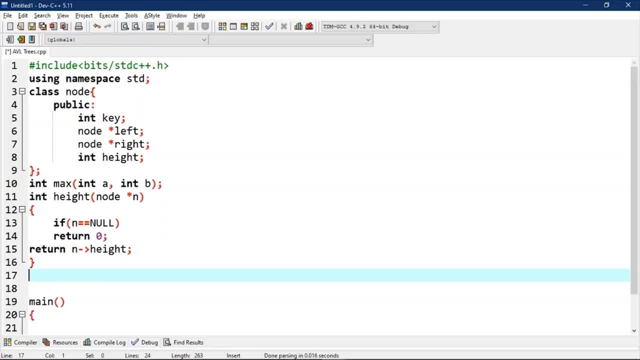 Now let's write that function to get maximum of two integers: int max, int a and int max- We will return a comma. int b: We will return. if a is greater than b, then we will return a, Else we will return b. 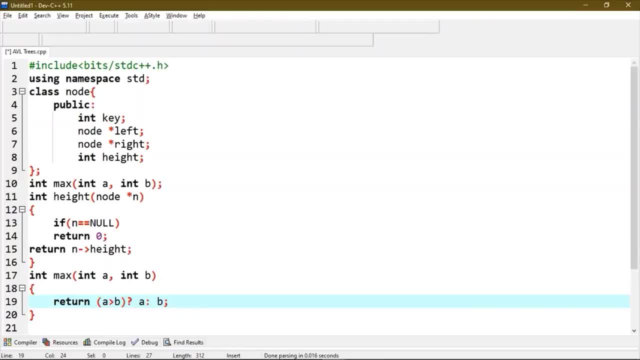 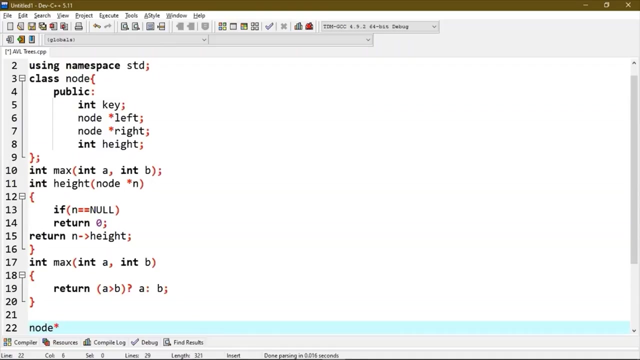 Now let's write a helper function that allocates a new node with a given key and null left and right pointers. So node star, new node int b. Now let's write a helper function that allocates a new node with a given key and null left. 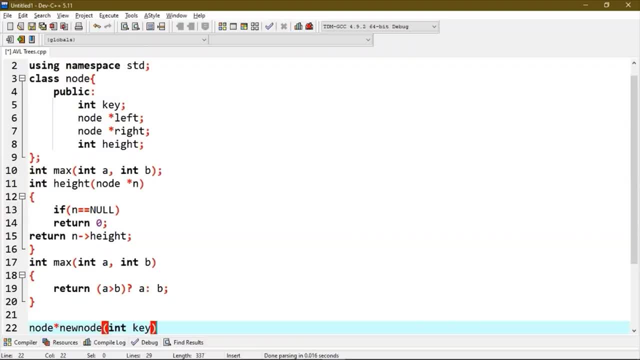 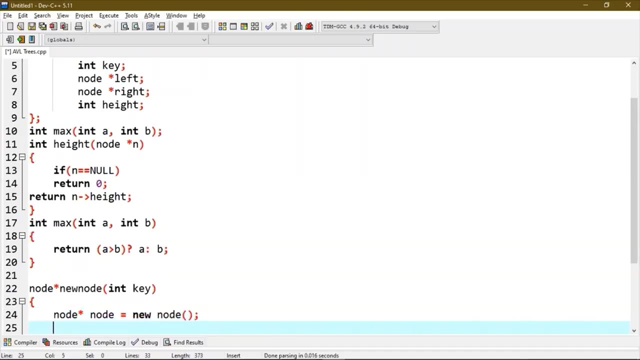 and right pointers And what will be the bar, The value of a special node. Also, we will return node key, int key and node star node equals to new node. The node key will be equals to key node left and right. Enjoy. 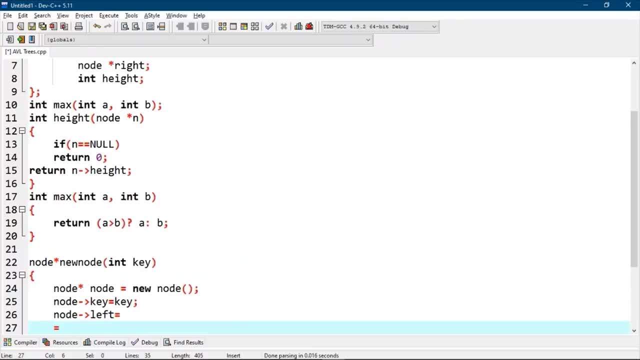 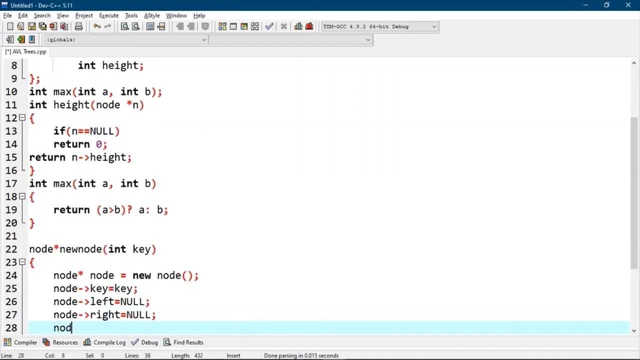 will be equals to left, node left will be equals to null and node right will be equals to null and node right will be equals to one and node right will be equals to one and return node. here we have kept height as one, because at the new node is initially added at: 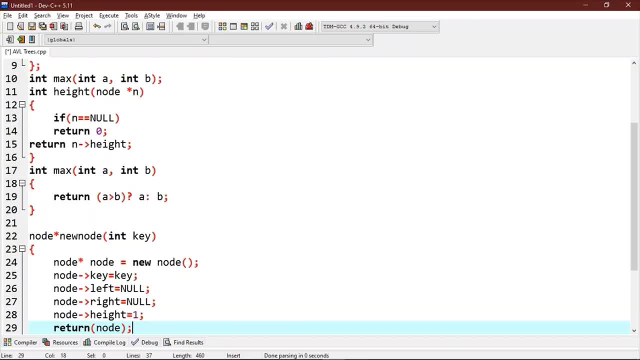 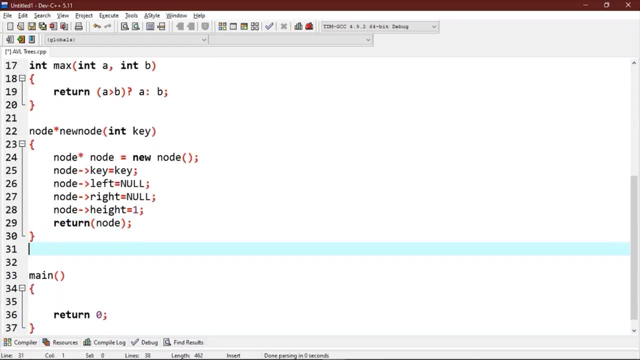 leaf, so by default it will always be at one. now let's write a utility function to right rotate subtree rooted with y, node star right, node star y, now node star x, node star y. node star y is equals to by is left. is equals to by is left. 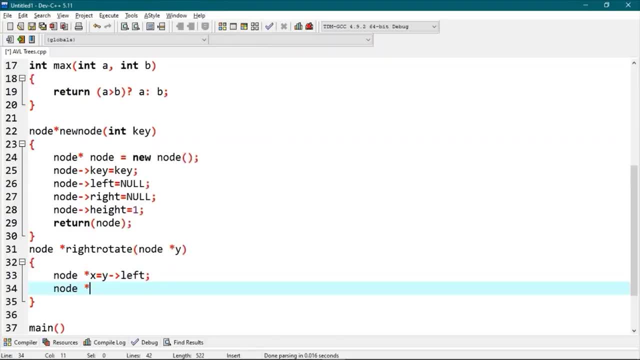 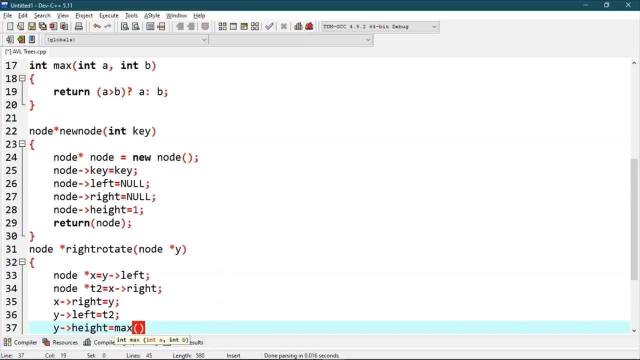 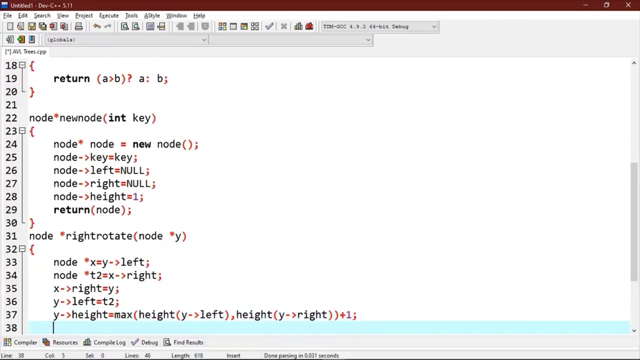 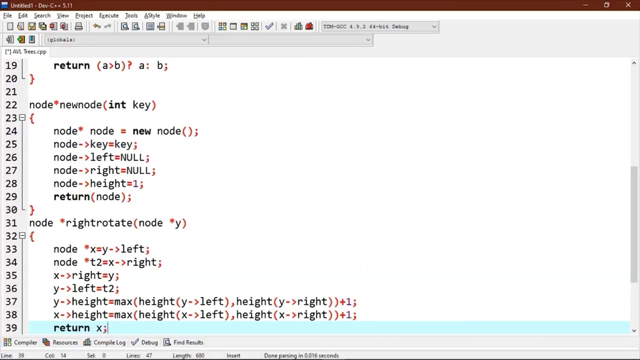 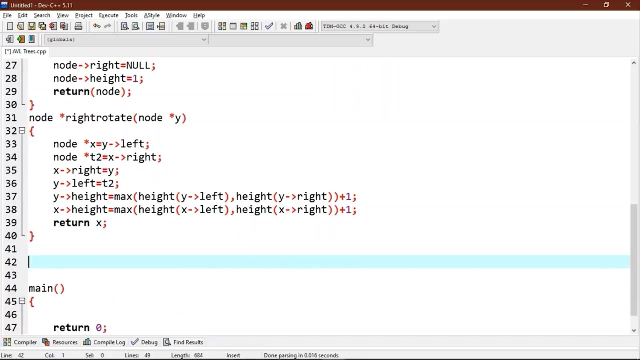 equals to max of height of y left comma. height of y height plus 1. now x height equals to maximum of height. x height, x left comma. height of x right can be looped crafts 程. that is a y cube, that is a form of y left rotate. 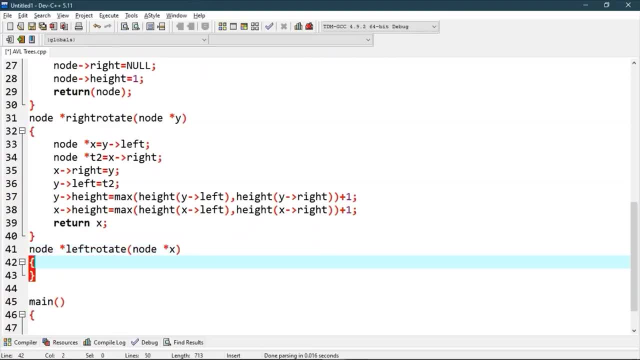 node star x, node star y will be equals to xs right and node star t2 will be equals to xs, sorry, ys. now we will perform rotation, so y left will be equals to x and x right will be equals to t2. now let's update height, so x. 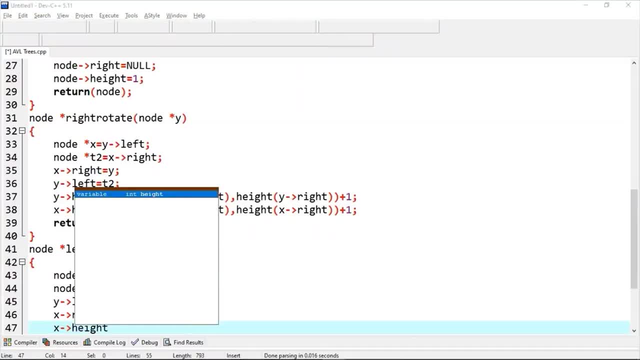 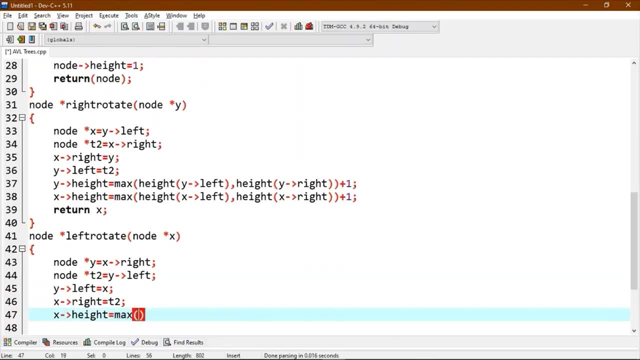 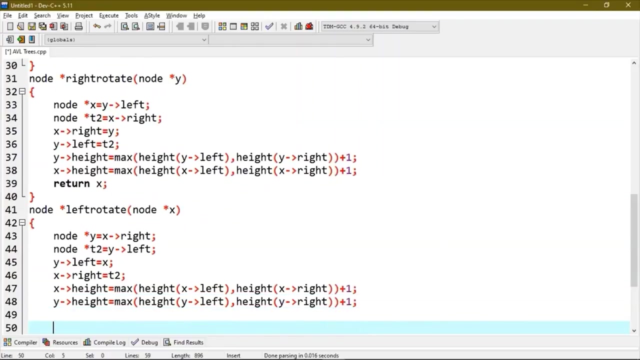 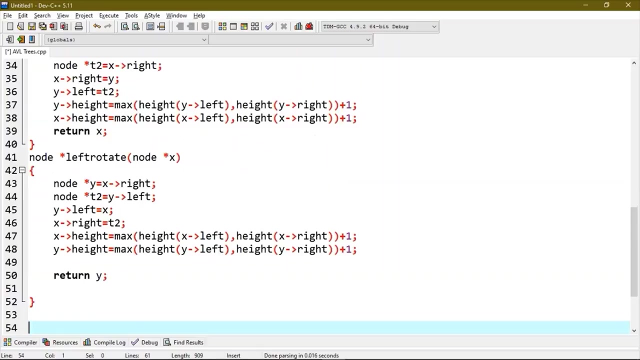 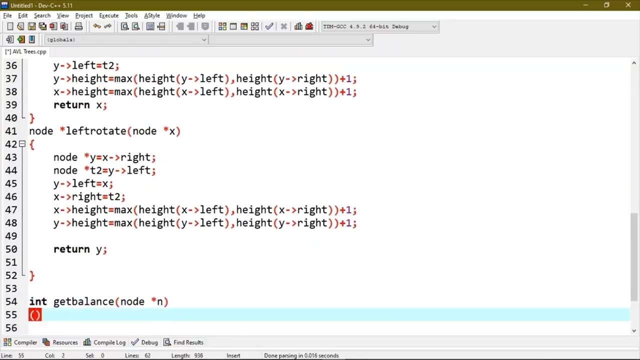 height is equals to maximum of height of xs left comma height of xs right and ys height equals to maximum of height of ys left comma height of ys right and return y. now let's write a function to get balance vector of node n: n. so int set balance argument as node pointer n. 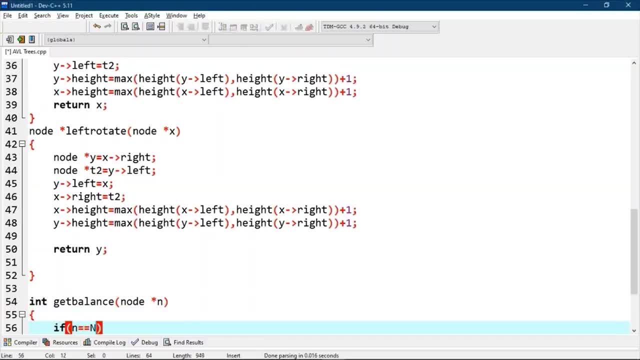 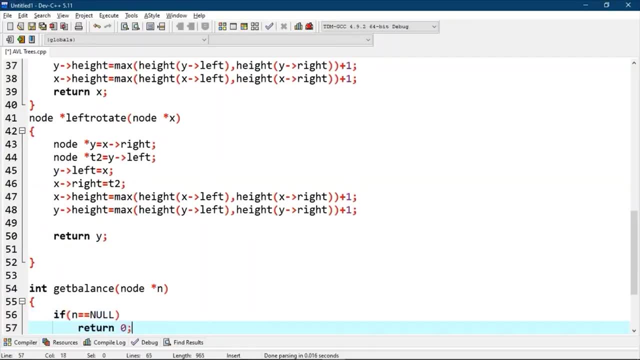 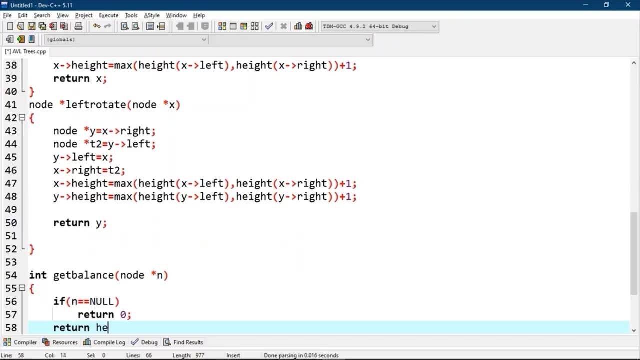 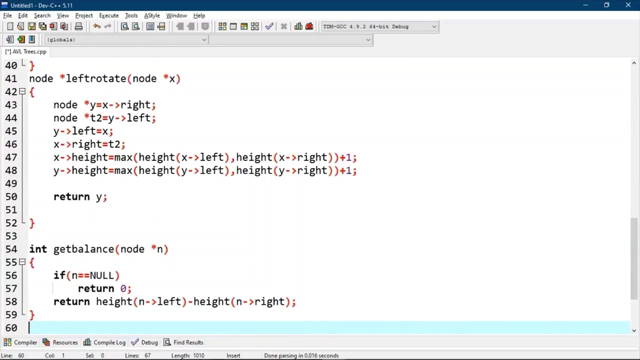 if n is equals to null, then we will return 0. otherwise we will return height of n's left minus height of n's left minus height of n's. right now, let's write a recursive function to insert a key in the subtree rooted with node and. 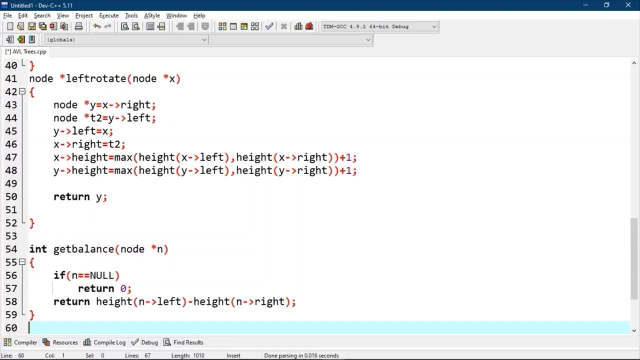 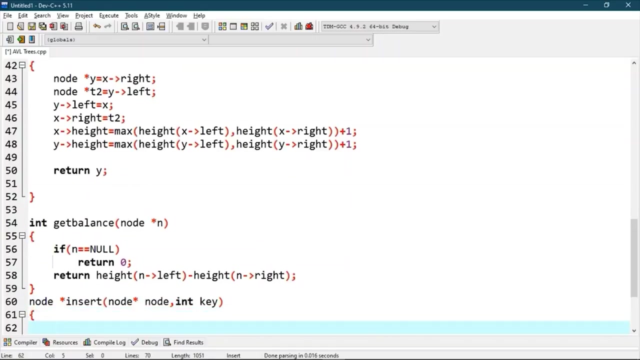 returns the new root of the subtree. so node star, insert. nodes star, node comma int key. now we will perform the normal bst insertion. so if node is equals to null, then we will return bst insertion. now we will perform the normal bst insertion. so if node is equals to null, then we will. 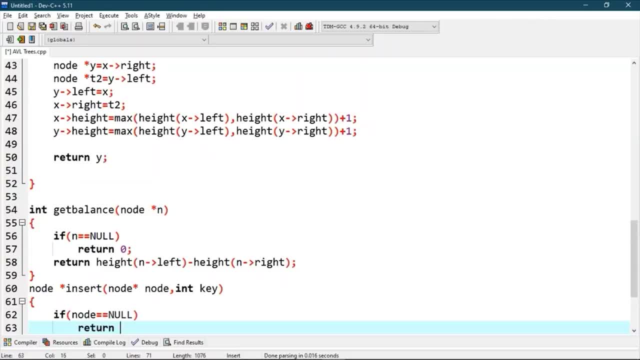 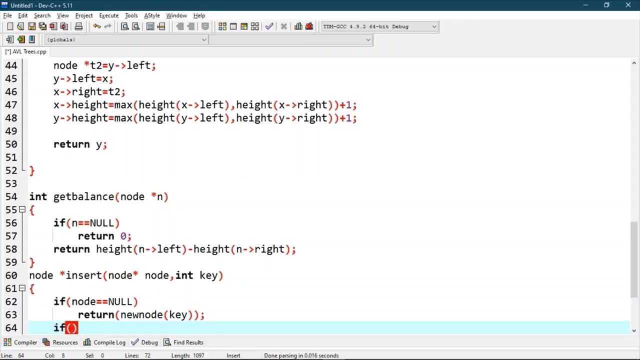 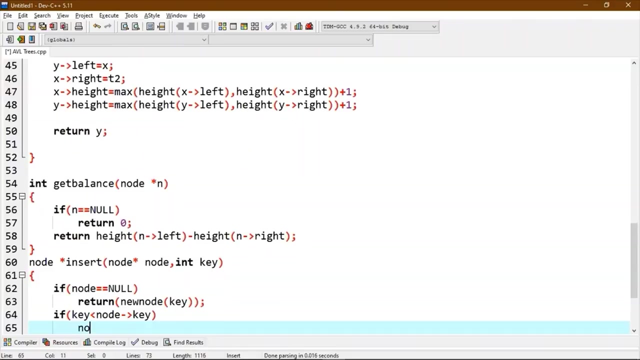 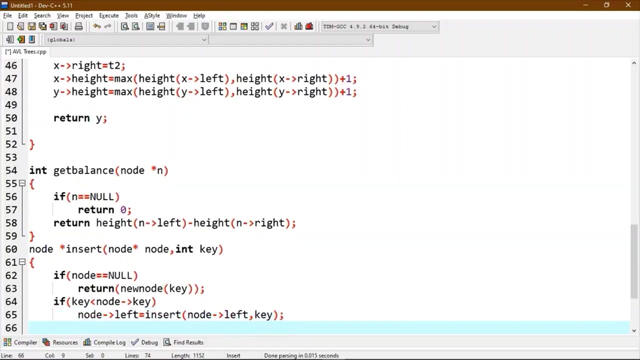 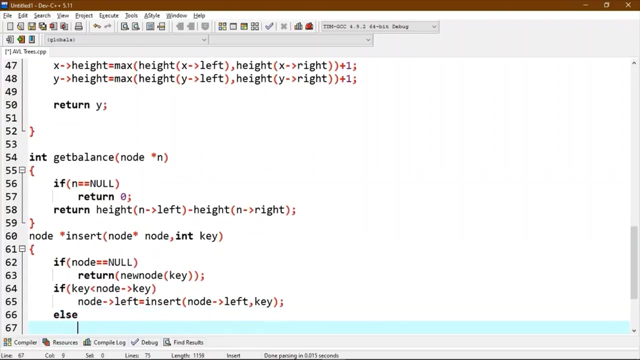 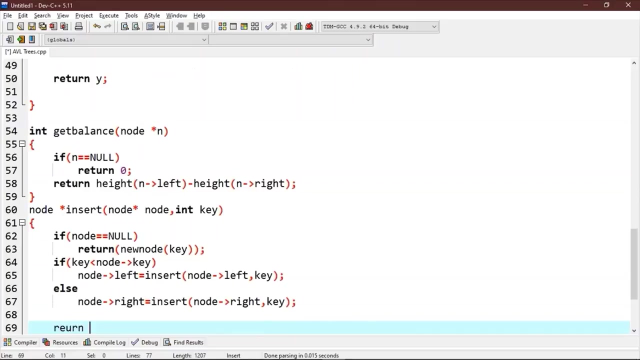 return, then we will return newNodeKey. now if this key is less than nodesKey, then nodeLeft will equals to insert nodeLeft comma key, or else we will insert that in the right nodeRight is equals to insert nodeRight comma key. now we will return node. 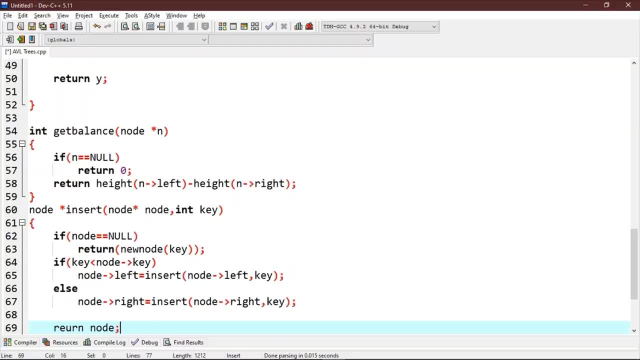 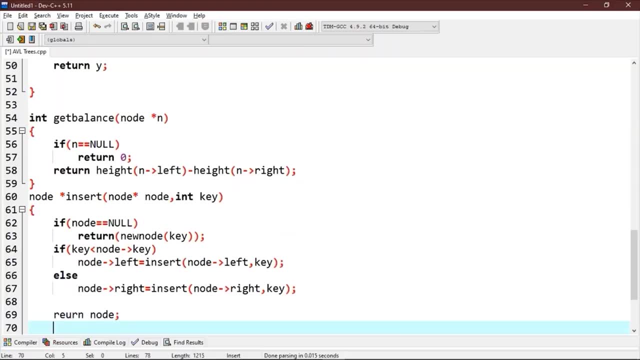 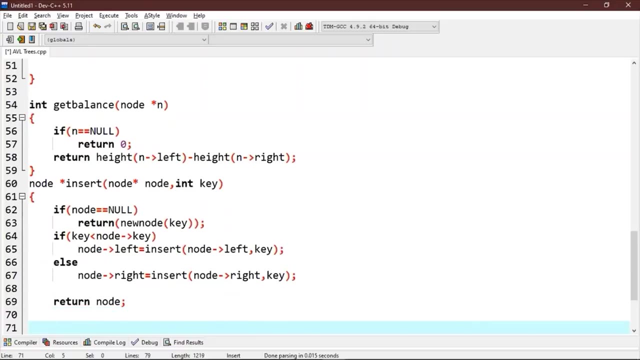 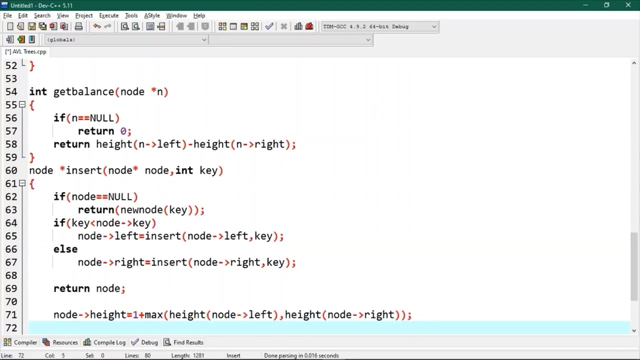 this ifelse will make sure that we will reach to the leaf node and then we will insert the key. now we will update the height of this ancestor node. nodeHeight is equals to 1 plus max height of node left comma height of node. right now we will get the balance factor for this ancestor. 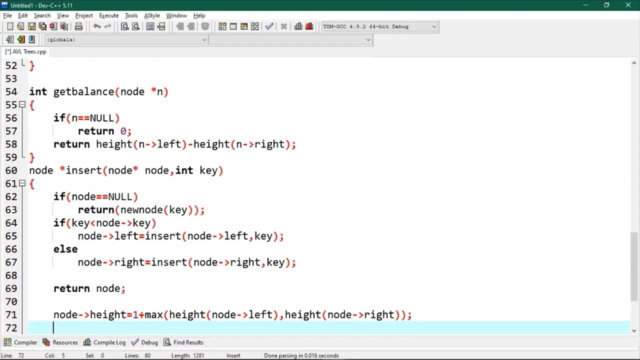 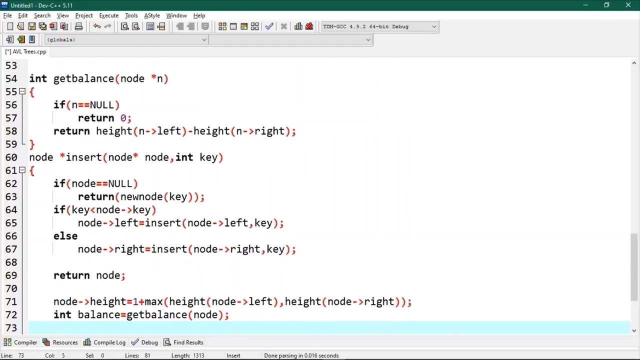 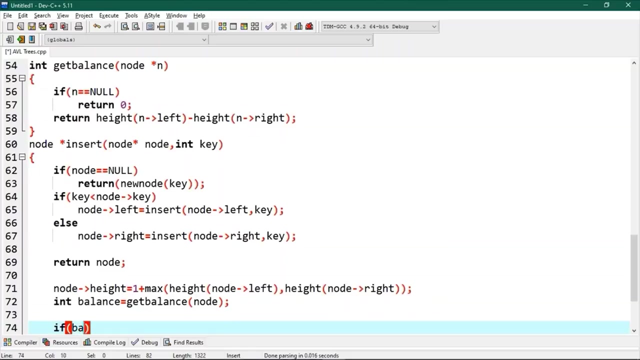 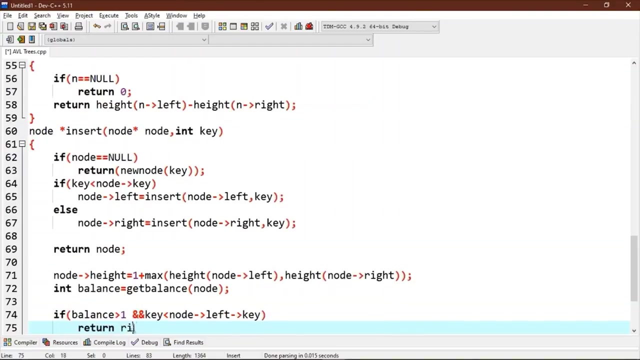 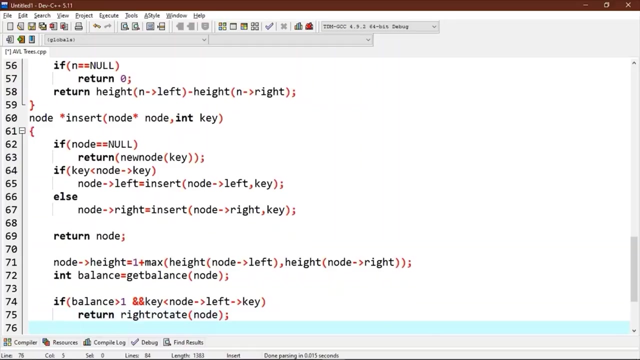 node to check whether this node became unbalanced. so int balance is equals to get balance. now, if this node becomes unbalanced, then there are four cases. so if, if balance is greater than one and key is less than node left key, then we will return right right rotate node. this is statement for the left left case. so or LL case. now, 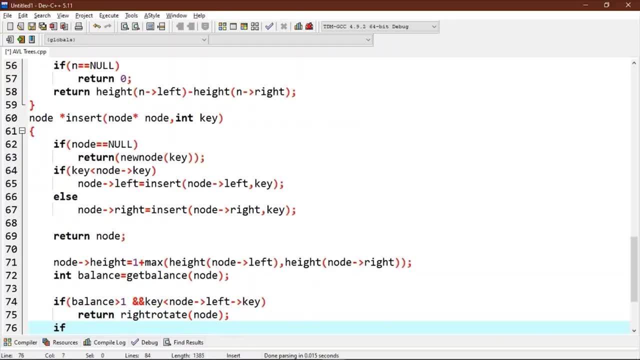 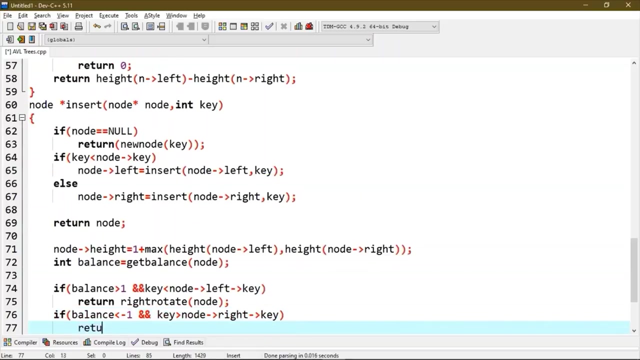 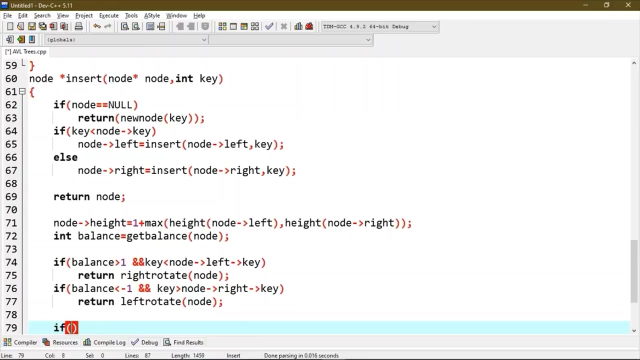 let's write it for the right right case or our case. so if balance is less than minus 1 and E is greater than node right key, then we will return left rotate node now right for the left right case or LR case. so if balance is greater than 1 and 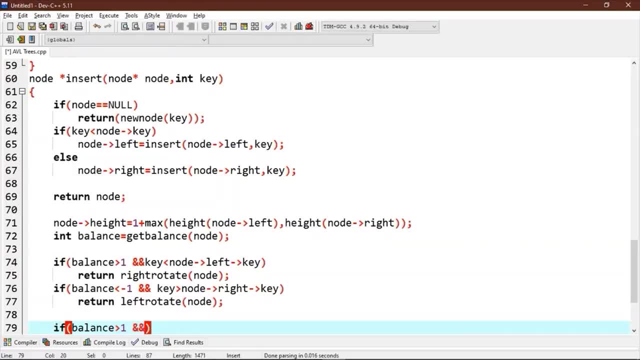 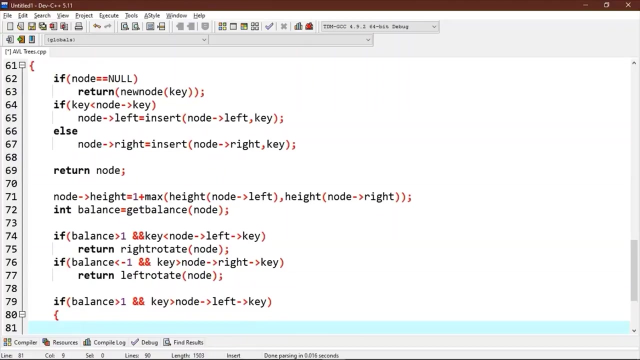 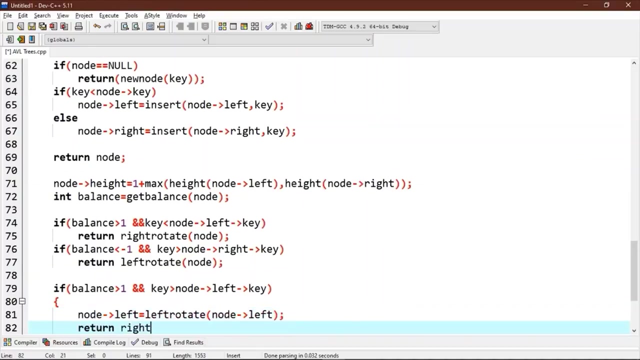 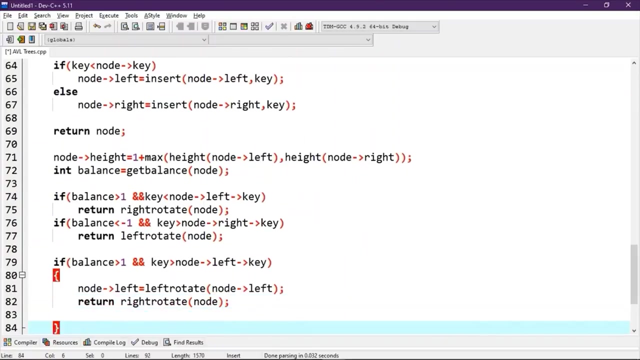 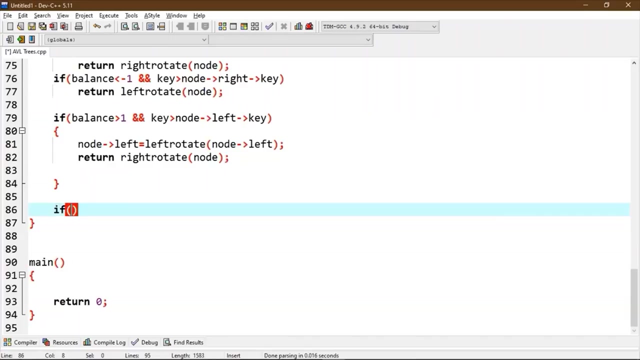 key is greater than node left key. the node left is equals to left rotate node left. now. return right rotate node. now let's write the right left case or rl case. so if balance is less than minus one and key is less than node to the right, key is less than node to the right. 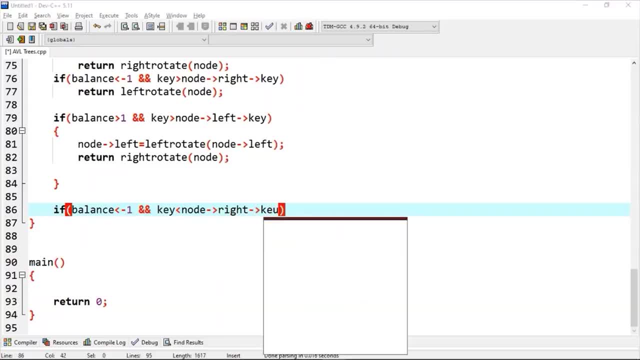 key is less than node to the right key key is less than node to the right key and node right and node right and node right will be equals to. will be equals to. will be equals to: right rotate node to the right node to the right rotate node to the right rotate. 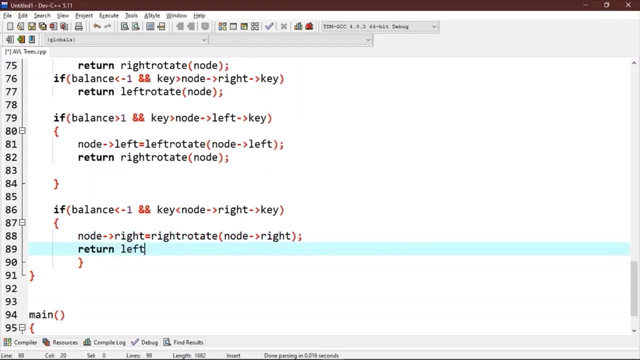 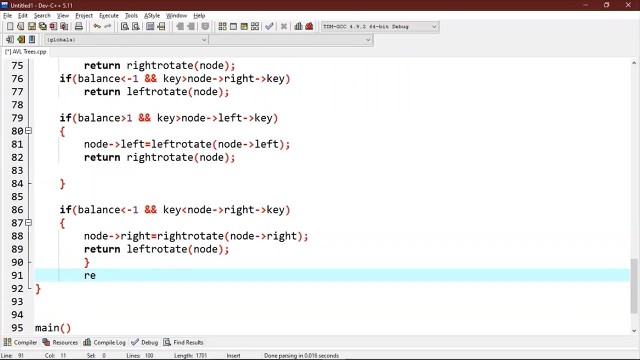 and we will return left. now we will return this node node to the right node to the right rotate node to the right rotate node to the right rotate. now let's write a function to print pre-order traversal of this tree. so void pre-order node: star root. 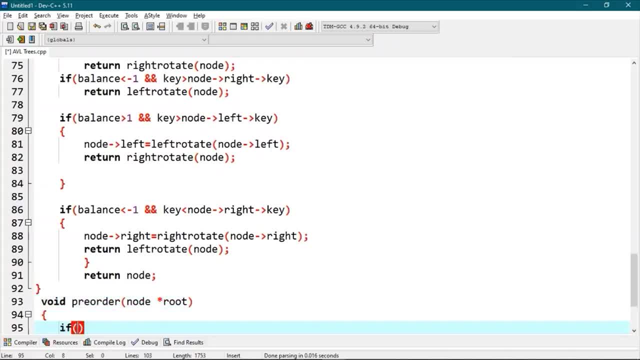 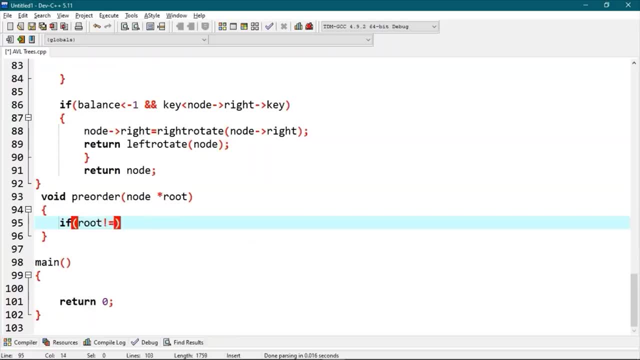 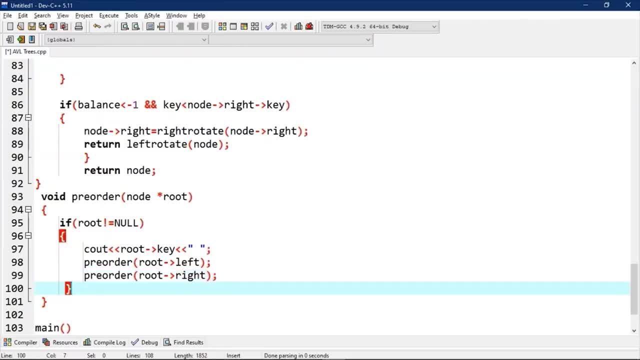 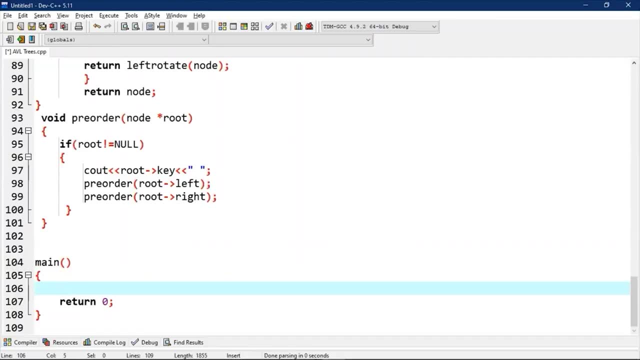 root. now let's write the code for the main block. we will start with an empty tree. node star root is equals to null. now we will try to construct tree. the root is equals to insert root comma 10. a root is equals to insert root comma 5. 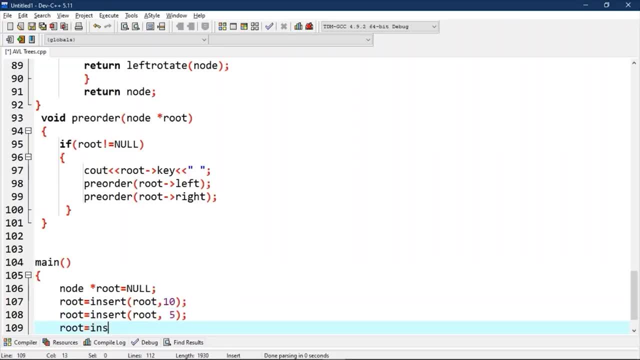 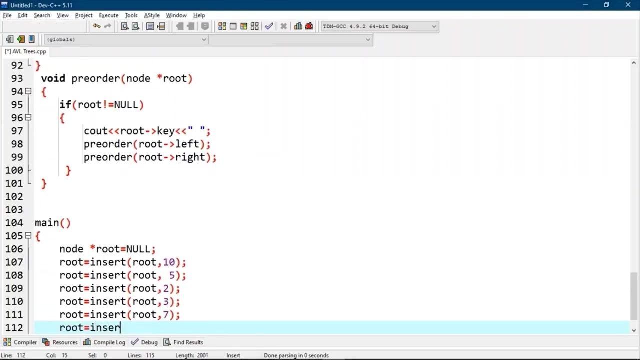 root is equals to insert root comma 2. root is equals to insert root comma 3. root is equals to insert root comma 7. root is equals to insert root comma 7 and root is equals to insert. root is equals to insert root comma 9. 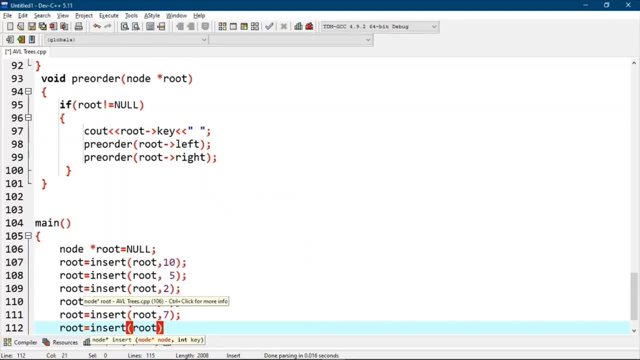 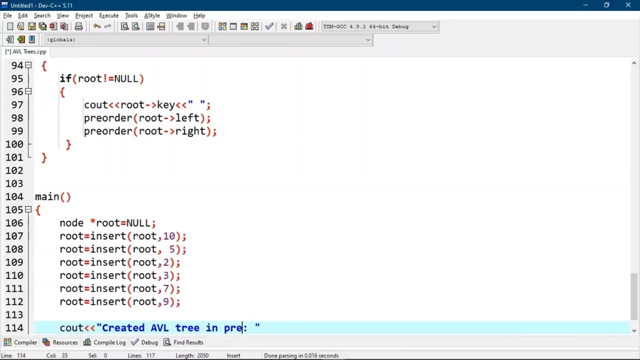 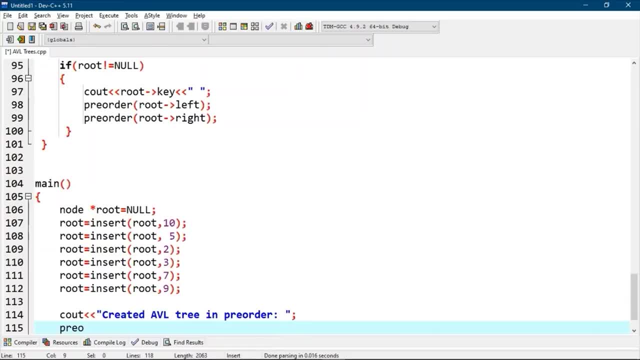 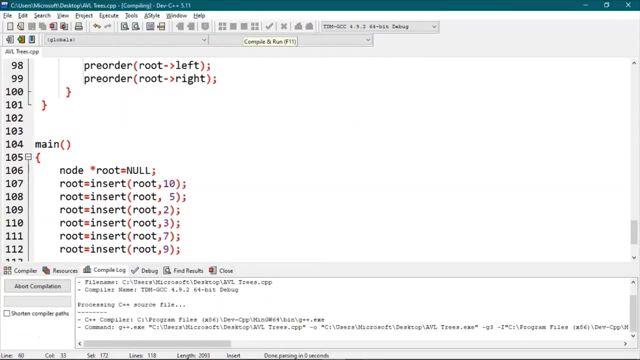 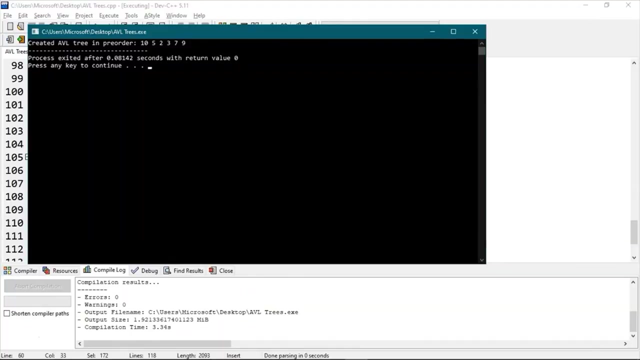 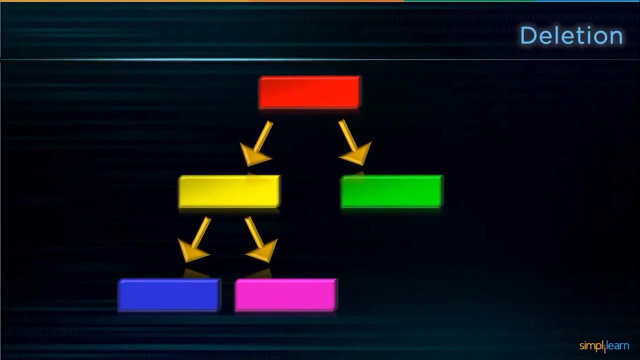 Let's execute this. As you can see, we have successfully created our first aviary tree. Let's get back to slides At last. deletion: We will delete a node following a binary search tree rules. Then we will check if all the nodes are balanced or not. 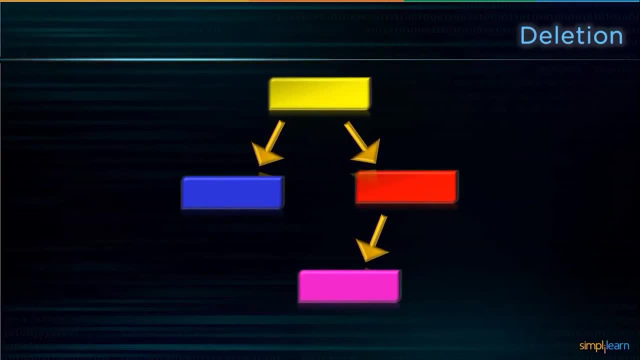 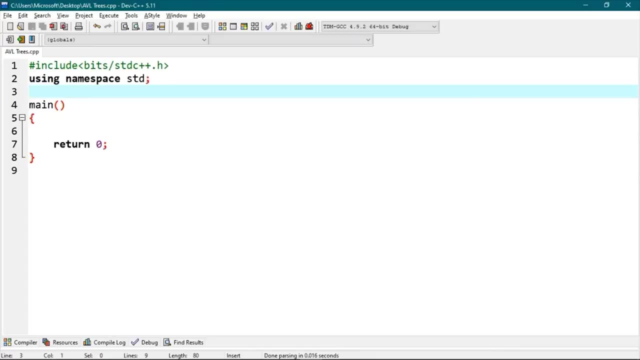 If they are not, then we will balance it by using suitable rotations. Now let's try these operations in a co-deleter. Let's start by creating a node. To create a node, we need a class node. we will define its members as public. 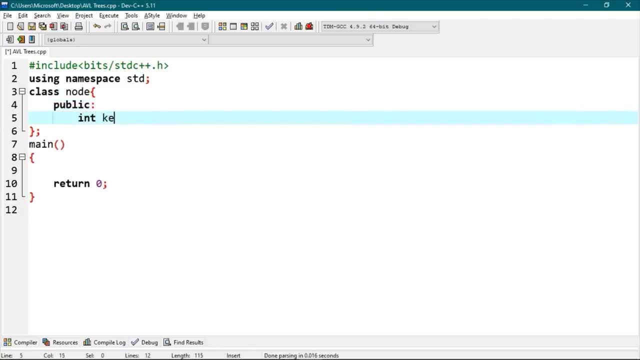 int key node star left, node star right. int height. Now let's write a utility function to get height of the tree. So int height, node star n: if n is equals to null, then in that case we will return 0. otherwise we will return 0. 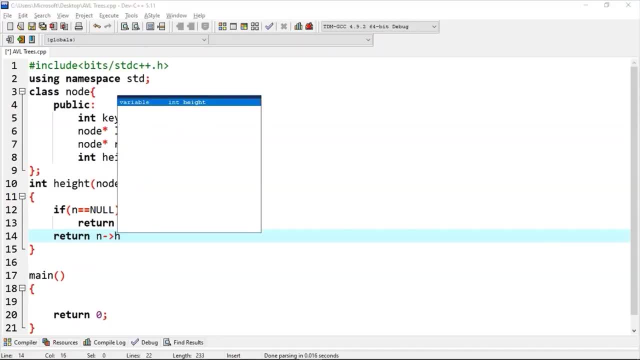 Hence height. Now let's write a utility function to get maximum of two integer: int max, int a, comma, int b. So we will return: If a is greater than b, then a, else b. Now let's write a helper function that allocates: 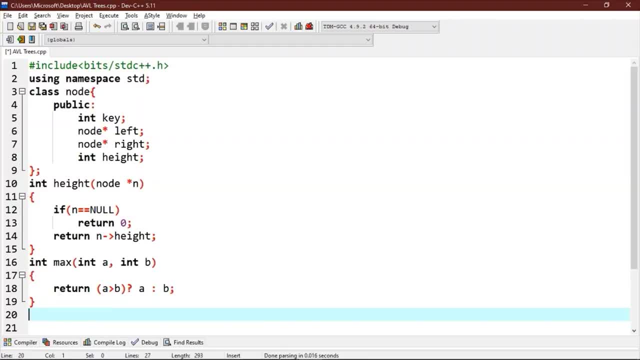 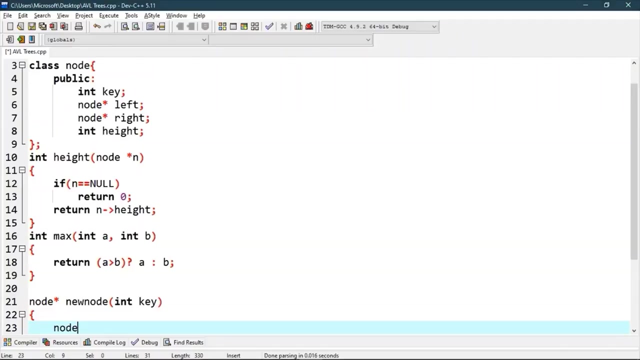 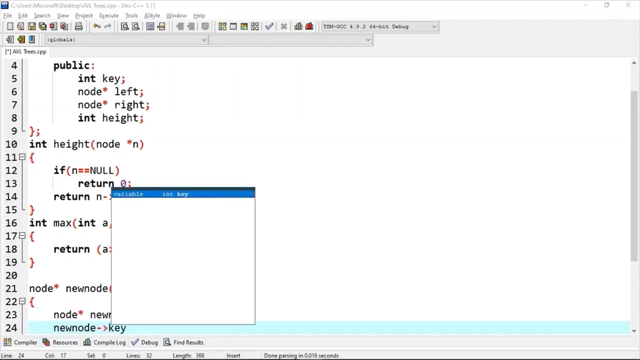 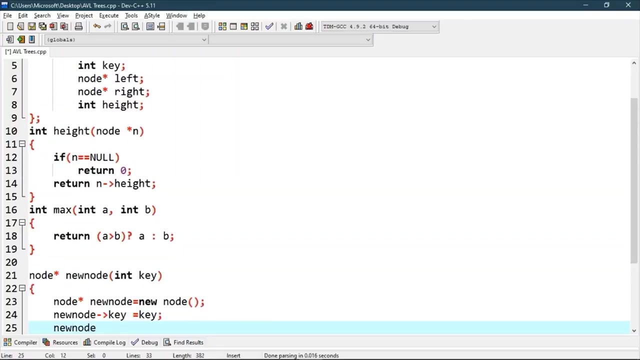 a new node with a given key and null left and right pointers. So node star, new node int key. So node star, new node is equals to new node parenthesis. Now new node is equal to new node parenthesis. So node star, new node will get key as key new node left is equals to null and new node right is equals to null and new node's height is equal to null. 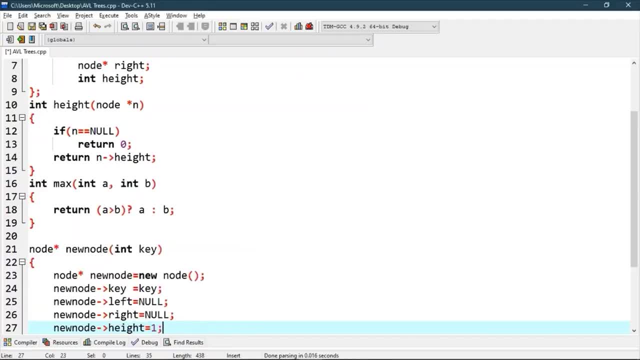 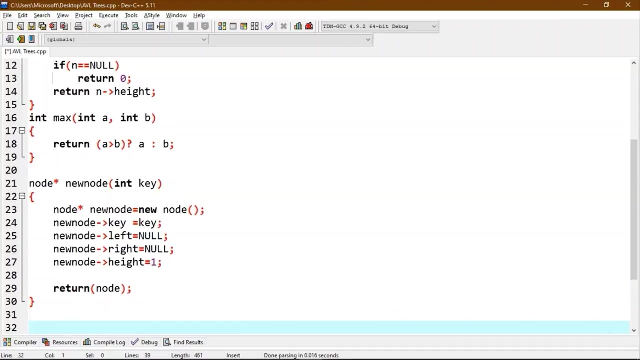 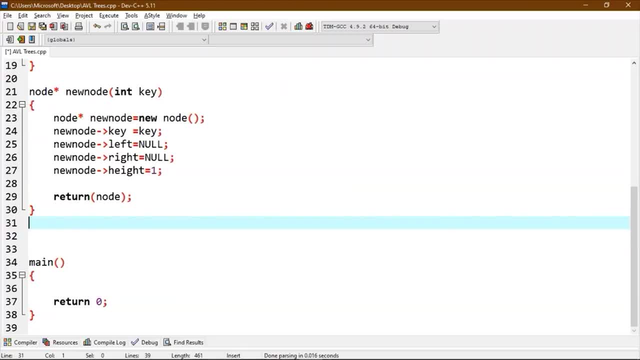 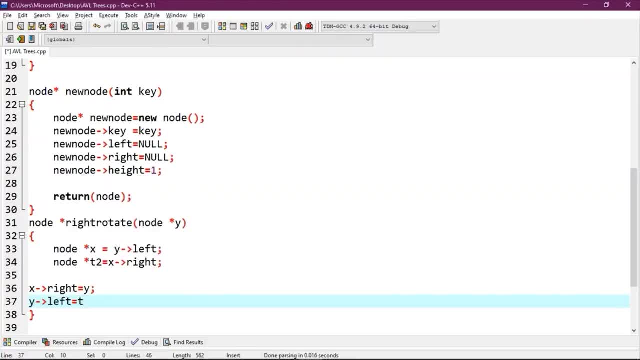 Y left is equals to T2. now we will update heights. so Y height equals to maximum of height of Y is left In thisرا eight comma. height of Y is right, It is an extra one. and X height is equals to maximum of height of X left. now we will. 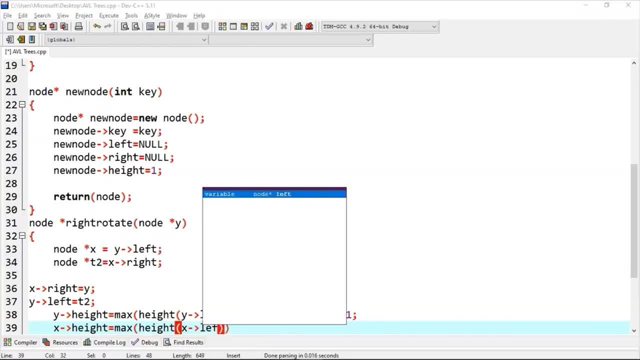 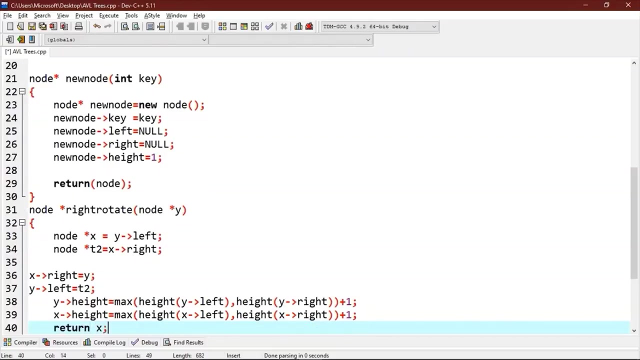 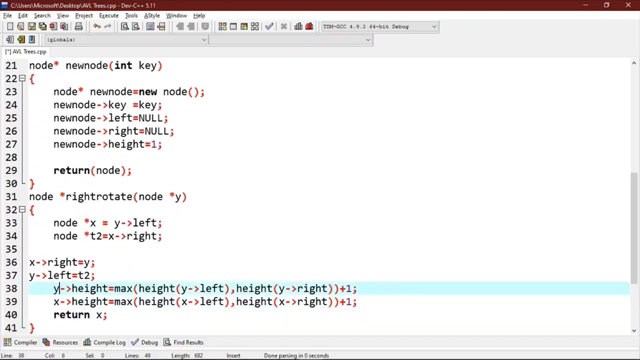 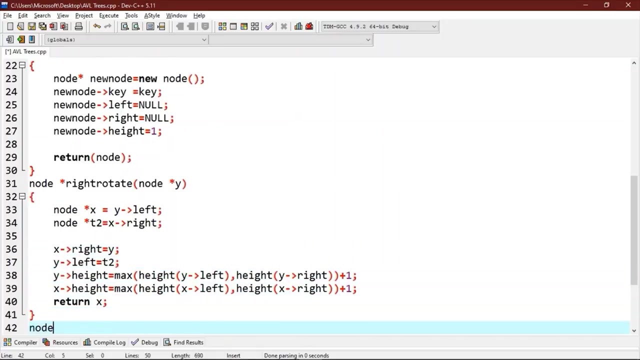 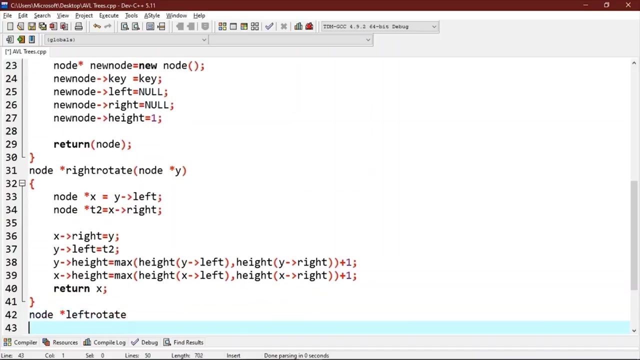 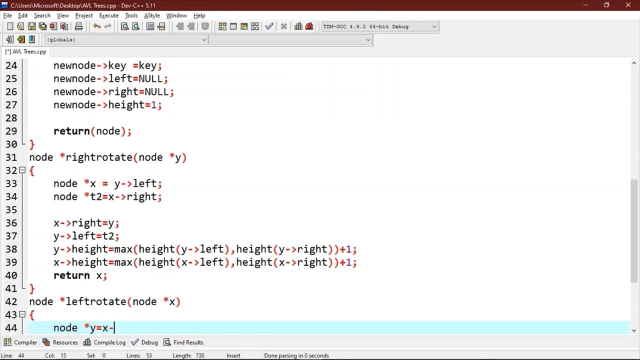 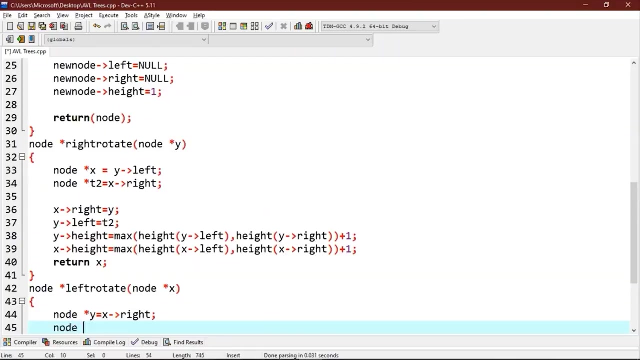 xsLeft, xsRight plus 1.. Now we will return this new root, so return x. Now we will write node star left: rotate. Now we will write node star x. Node star y will be equal to xsRight and node star t2 will be equal to ysLeft. 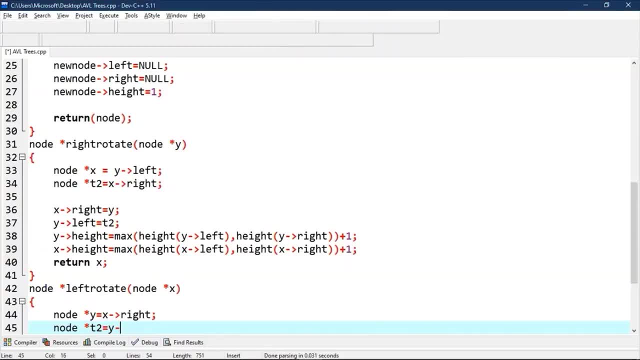 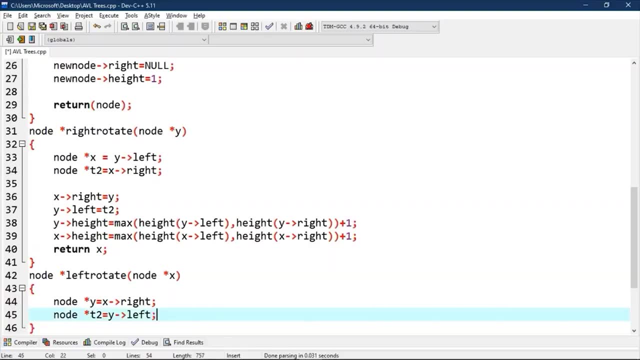 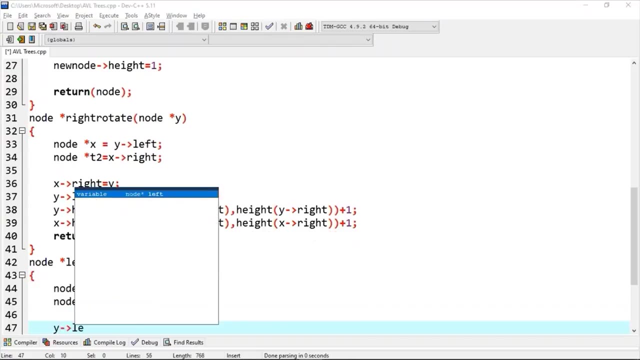 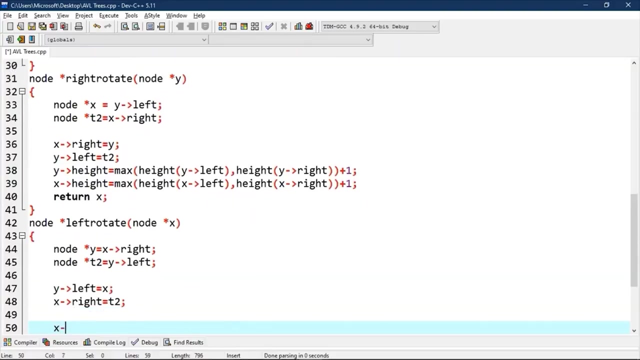 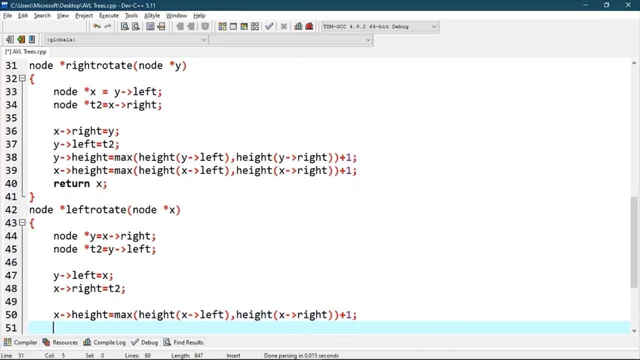 Now we will return this new root. Now we will perform rotation, so yLeft is equal to x and xRight is equal to t2.. Now we will update these heights, So xHeight is equals to maximum of height of xLeft, height of x right plus 1, and the 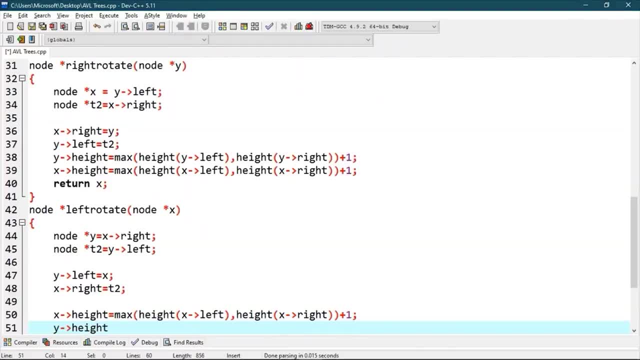 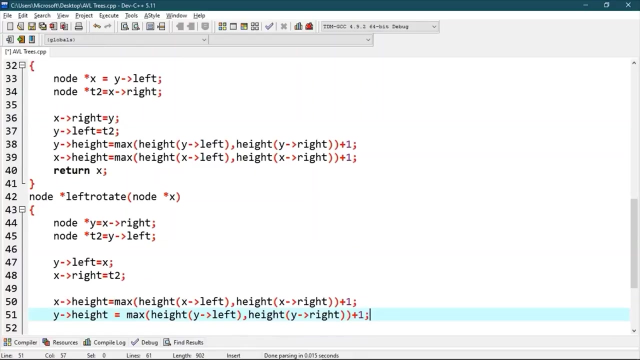 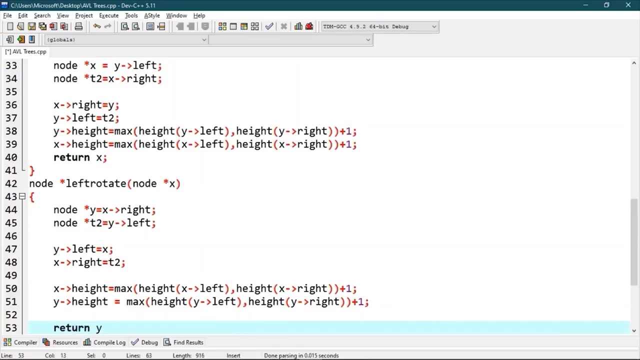 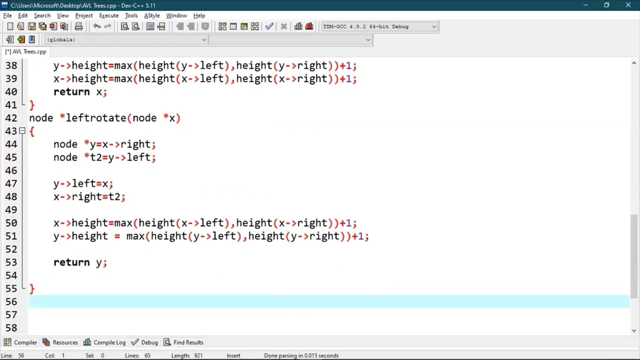 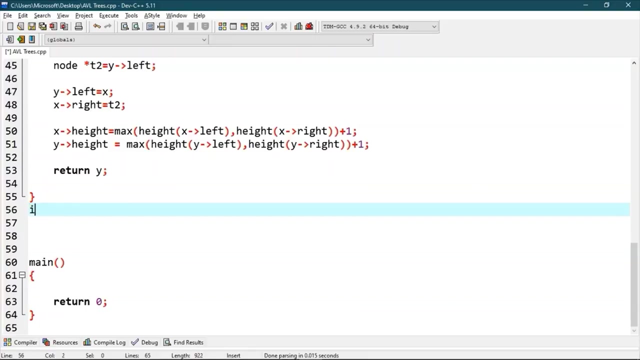 yZ height is equals to max of height of y's left comma height of y's right, plus one. plus one. now we will return this y. now we will write a function to get balance factor of node n. so int get get balance of node star n. 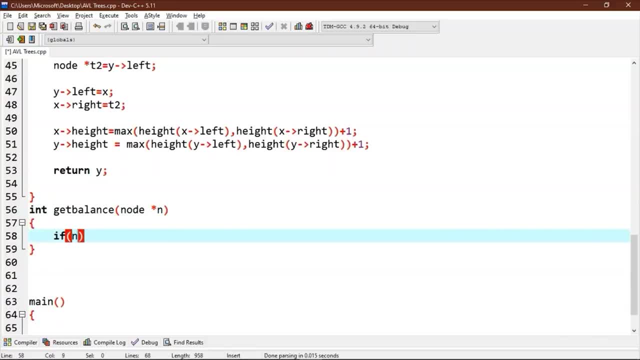 so if n is equals to null, then we will return zero, otherwise we will return height of n's left minus height of n's right. now let's write a function to insert a node. so node start: insert the first variable. so node start. node comma int key. 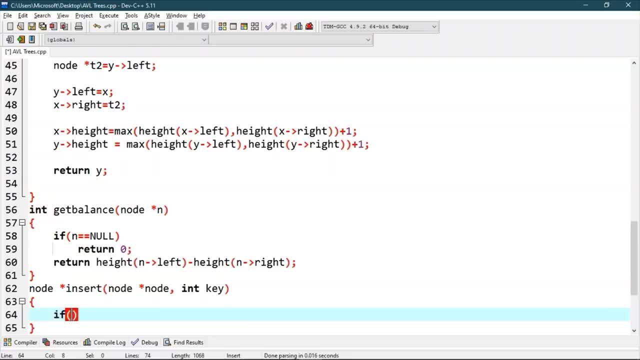 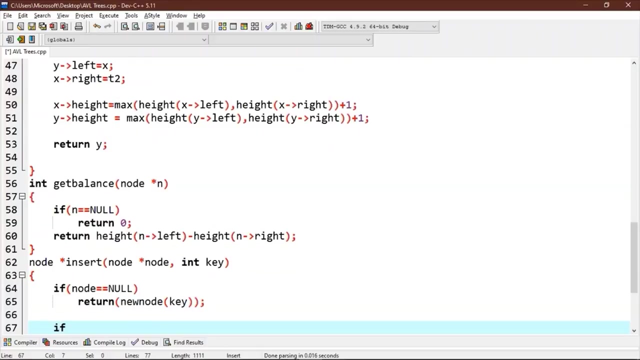 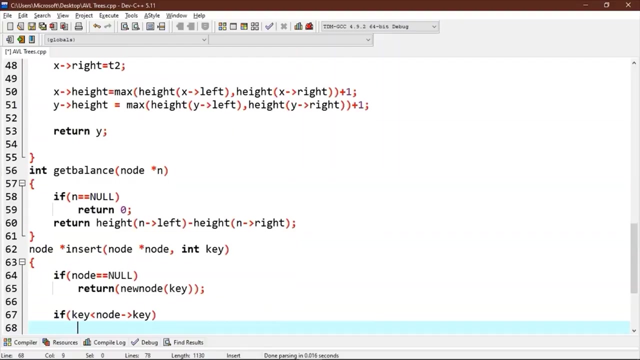 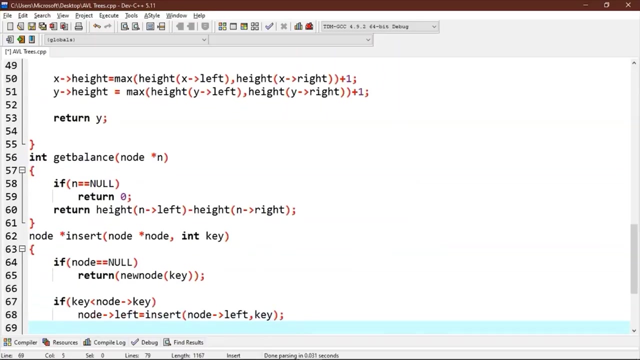 we will perform normal bst rotation. so if node is equals to null and we will return new node key. so now, if key is less than node key, then node left will be equals to insert node left comma key. now, if key is greater than node key, then node left will be equals to insert. 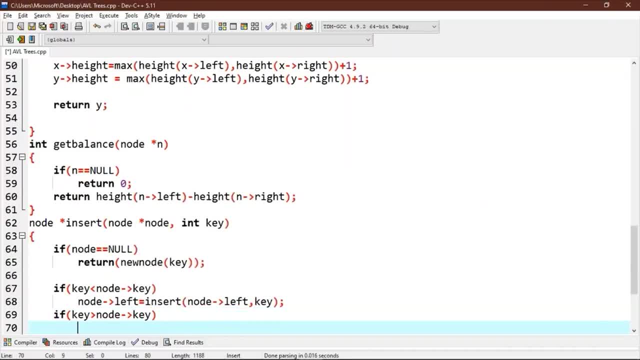 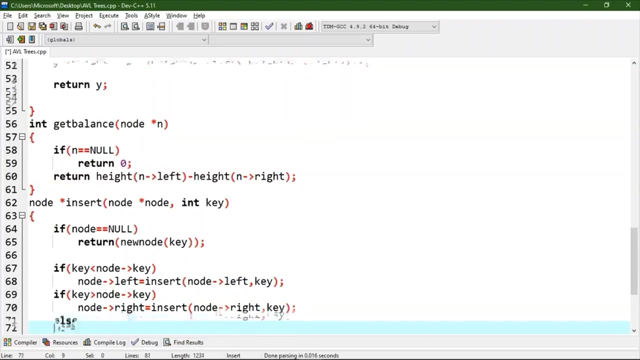 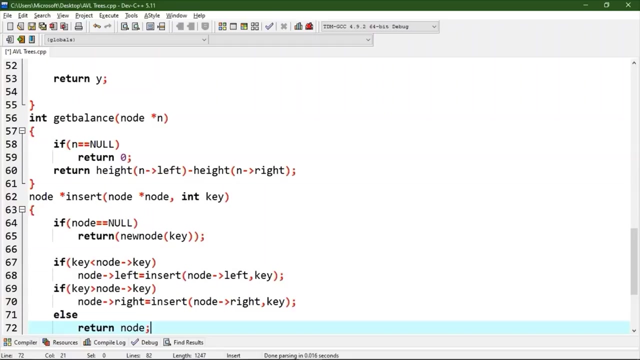 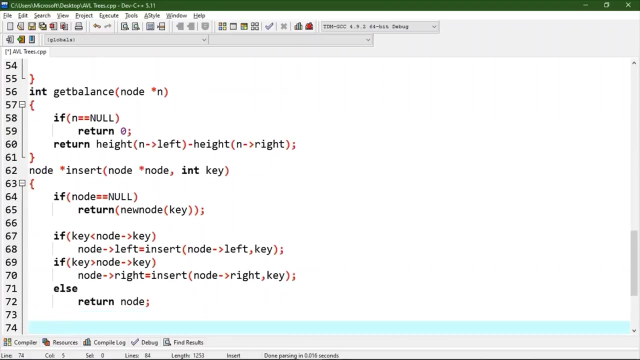 then node right is equals to insert node right glyphs comma key. else we will return node because equal keys are not allowed. now we will update the height of the ancestor node node height as to 1 plus x. height of node left: comma height of node right. Now we will get the balance vector of this ancestor node to: 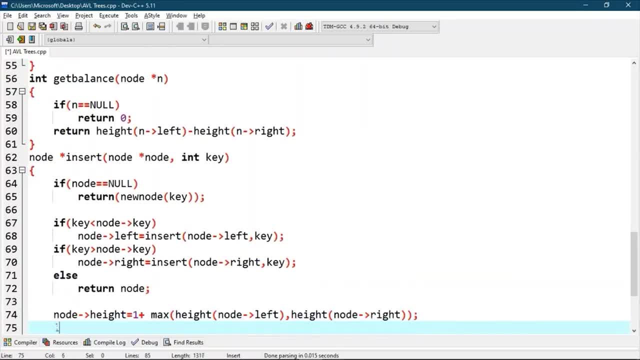 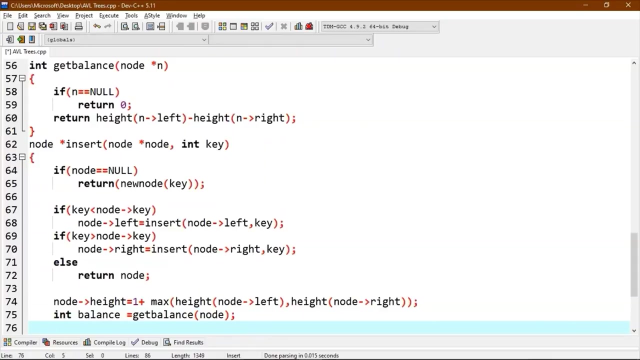 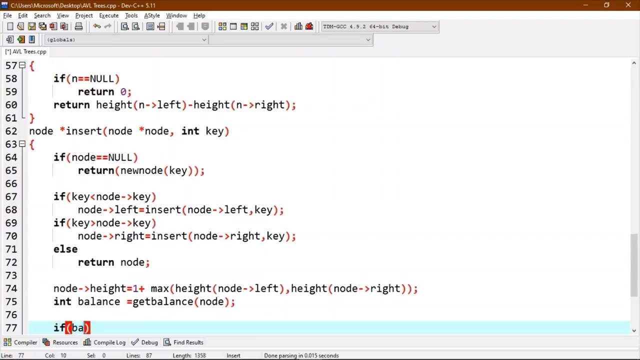 check whether this node becomes unbalanced. So if int balance equals to that balance of this node, Now if this node becomes unbalanced, then there are four cases that could be possible. First up: LL case. So if balance is unbalanced, then there are four cases that could be possible. First up, LL case. So if balance 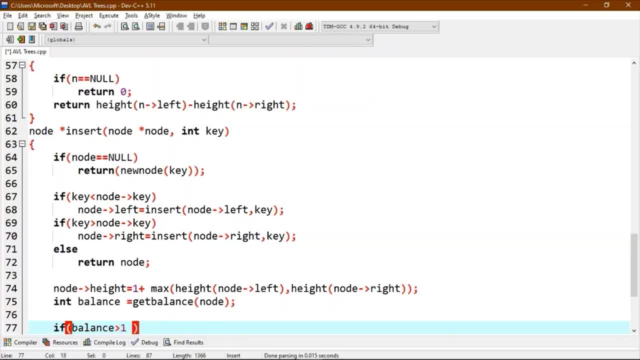 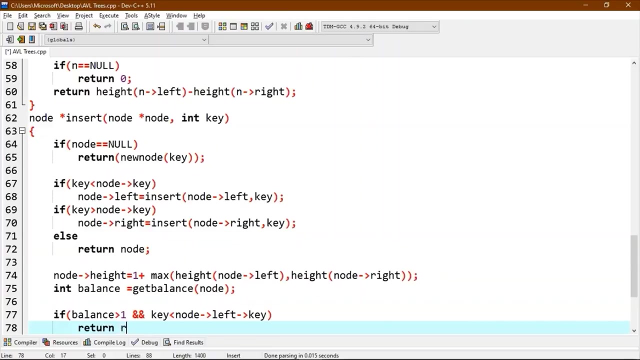 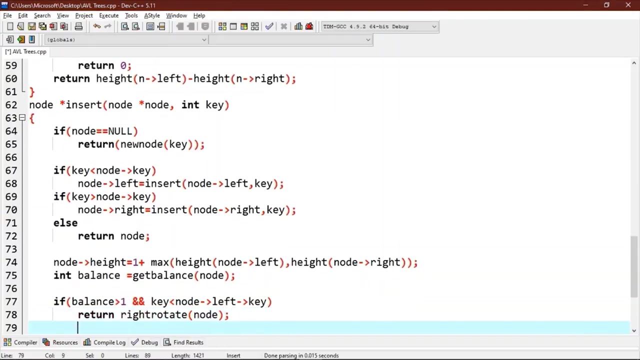 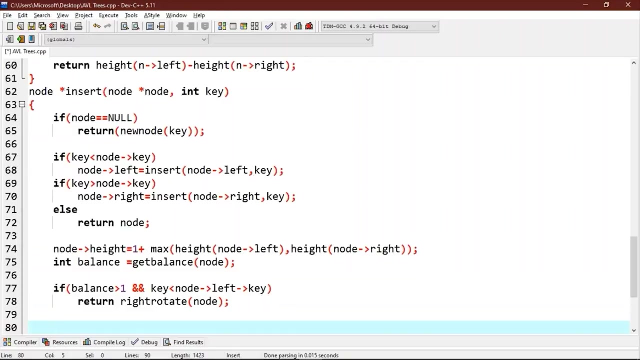 is greater than 1 and key is less than node left, return, right rotate. Now let's write locked node case: if balance is less than and key is equal to 3.. Now let's write right right case. So if balance is less than minus 1. 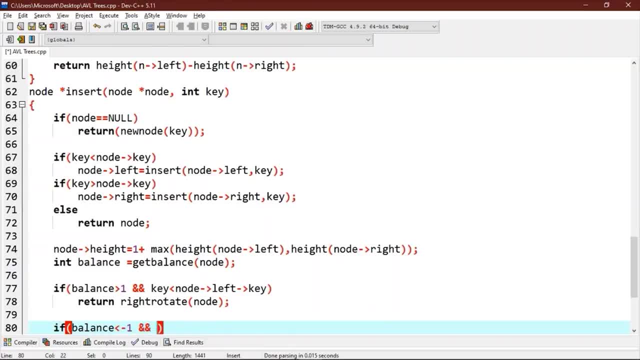 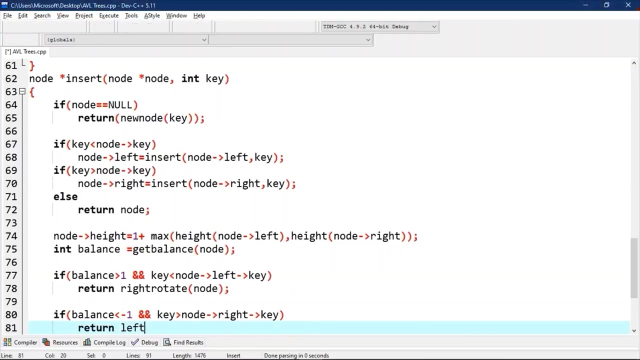 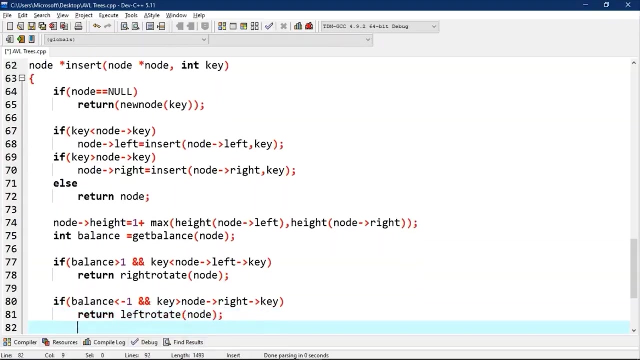 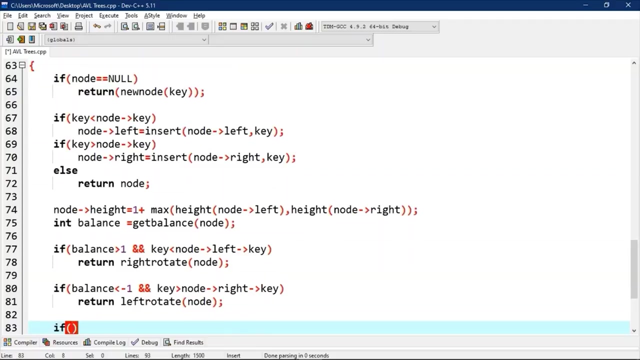 then there are four cases that could be possible. So if balance is greater than or equal to 1 and key is equal to 3.. then we will return left rotate node. now let's write left right case. so if balance is greater than 1 and key is greater than, 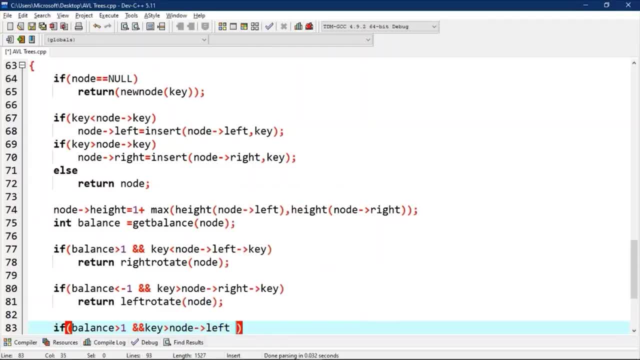 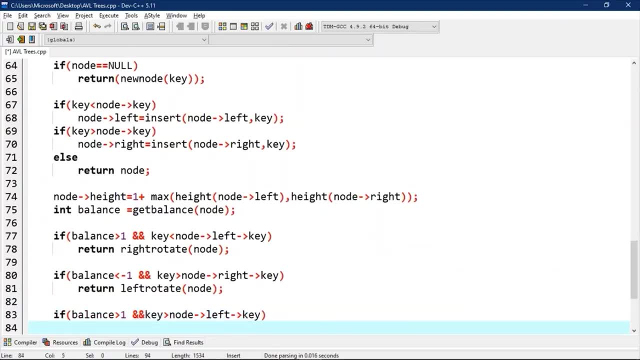 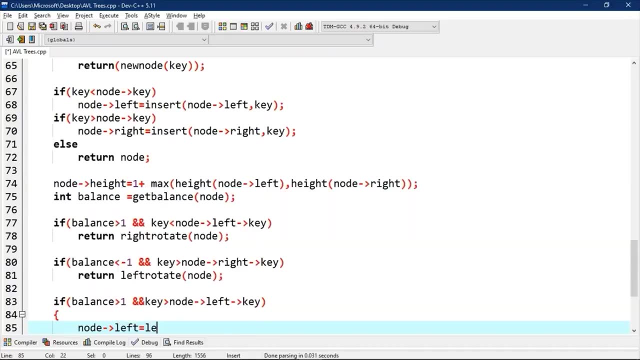 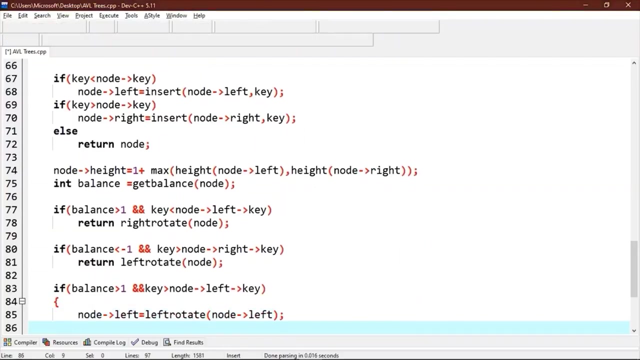 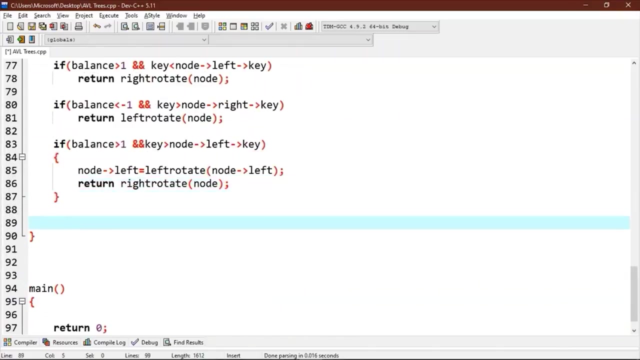 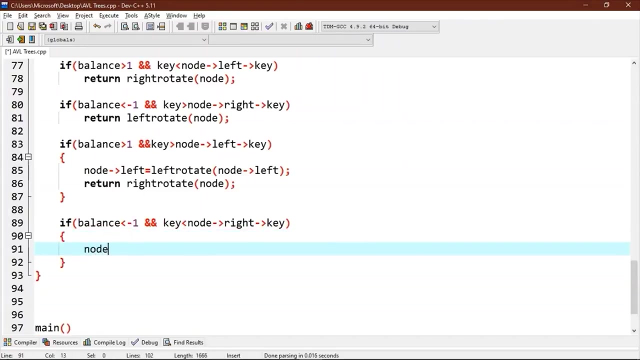 node left key, then node left will be equals to left rotate node and we will return right rotate node. now let's write the case for right left case: if balance is less than minus 1 and key is less than node right, well, So node right is equals to right rotate node right. 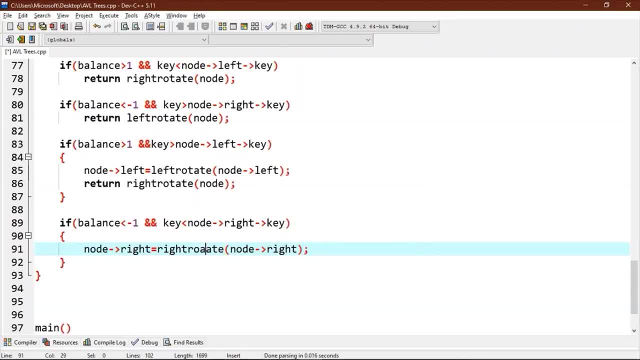 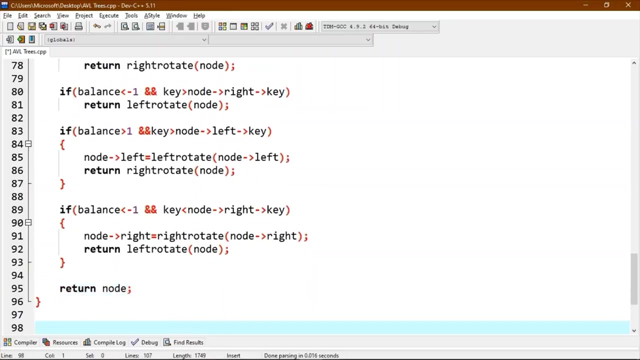 Now we will return left rotate node. Now we will return left rotate node. Now let's return the unchanged node pointer. So return node. Now let's write a function to find minimum value node. So node star: Min value node. 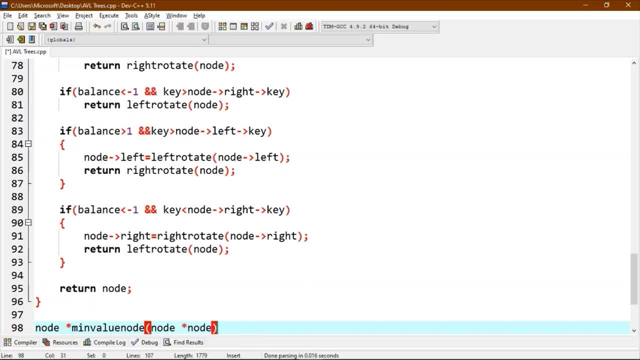 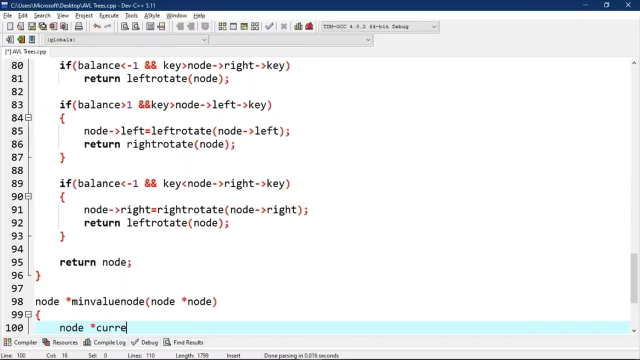 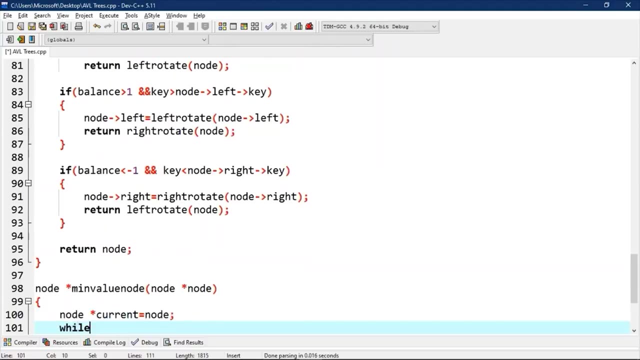 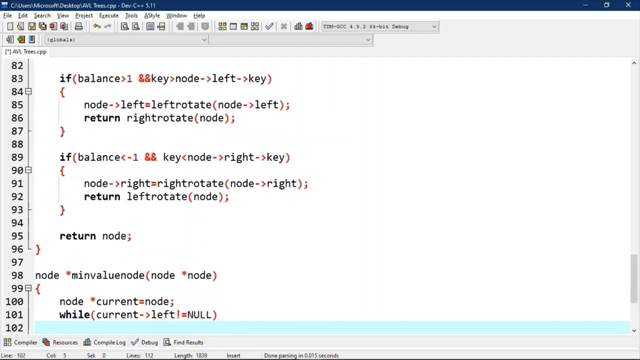 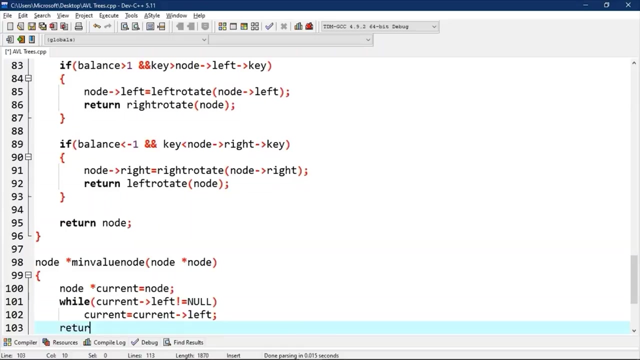 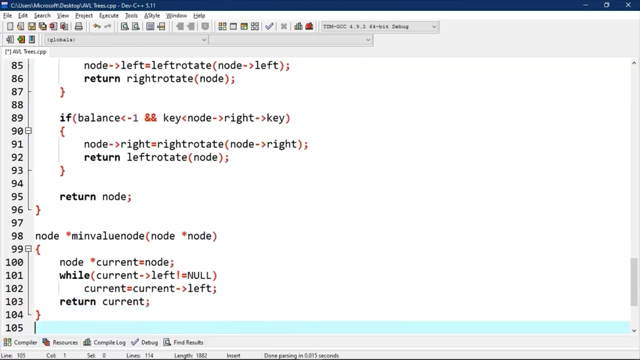 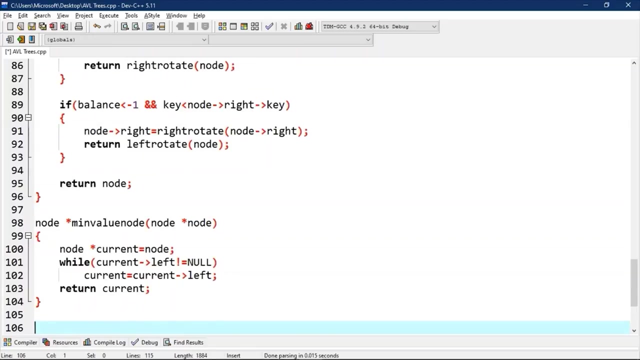 Node star, node. So node star, current equals to node. So, while current Left is not equals to null, Current is equals to current at left. Now we will return current. Now we will write a recursive function to delete a node with the given key from sub-tray with the given root. 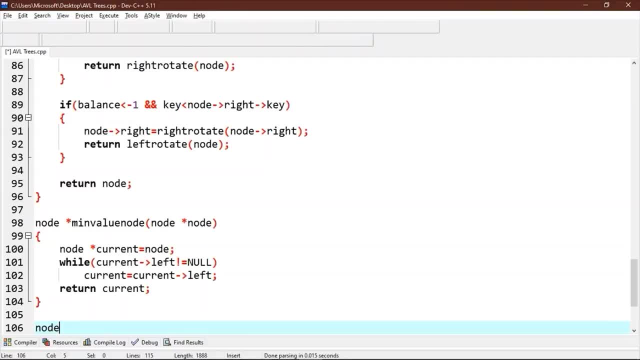 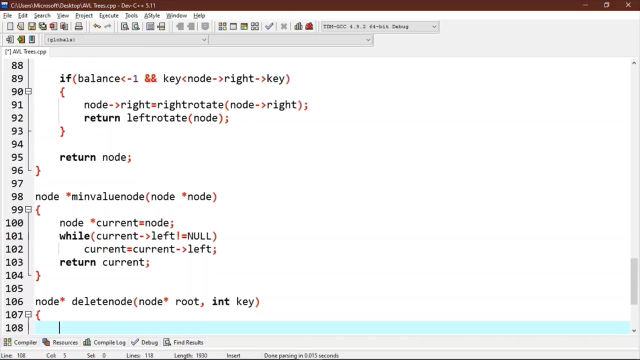 So node star delete node. Its arguments are: node pointer root, comma, int key. So node star delete node. So node star delete node. It has standard defaults like t defining node So and s and s t Ans. So node star delete node equals to the correct bears deal, a single node. 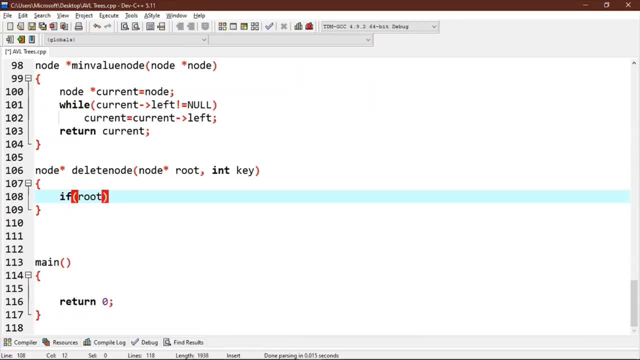 So if we are not Wrested with node extraordinaryWe will perform ST standard BST delete. For starters we will perform standard BST delete. So if root is equals to null, then we'll return. So if root is equals to NULL, then we will returnazi Columbus root. Root equals null. If unAll b videos, Then we will return root dividing. If we are sorry, but we are late for a couple seconds. So if we have 에 and an English language, you can pretty easily. Oh, I don't even know, I could have gotten it, but I have to go through it myself. 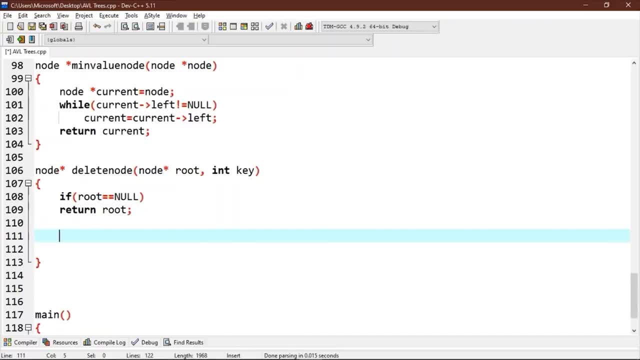 Oh, and I have to go Lewis and U out. okay. Now if the key to be deleted is smaller than the root key, then it lies in the left subtree. So if e is less than root e, then root left will be equals to delete node root to the. 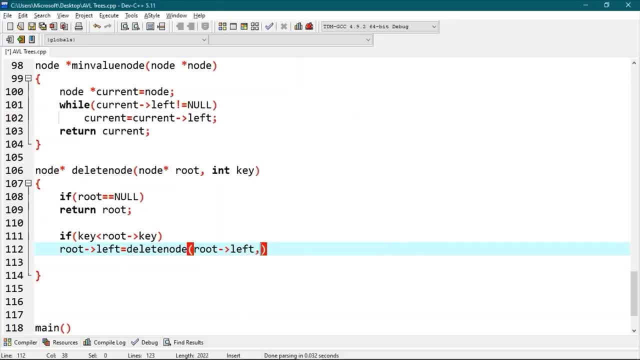 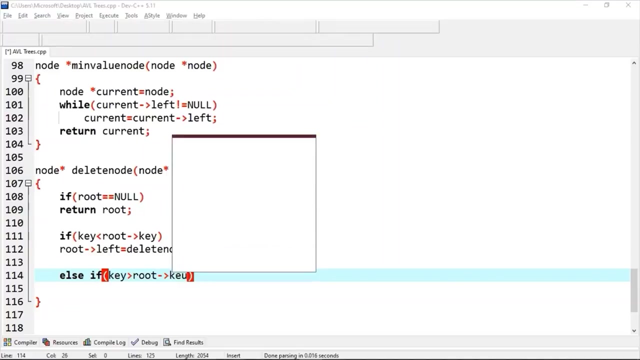 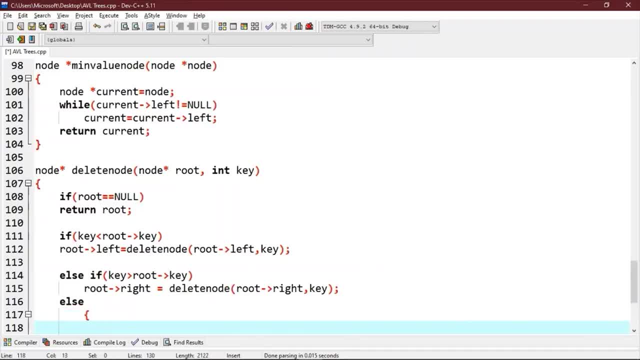 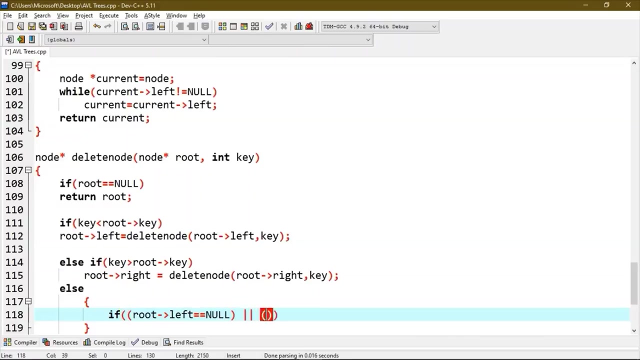 So if e is greater than root e, then root root right equals to delete node root right. So if fu $ $ e to the left is greater than fr $, $ is equal to $$, $, $, $, $r, $$$, $, $$ and. 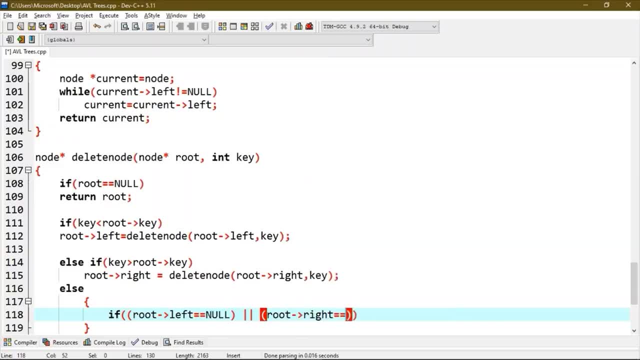 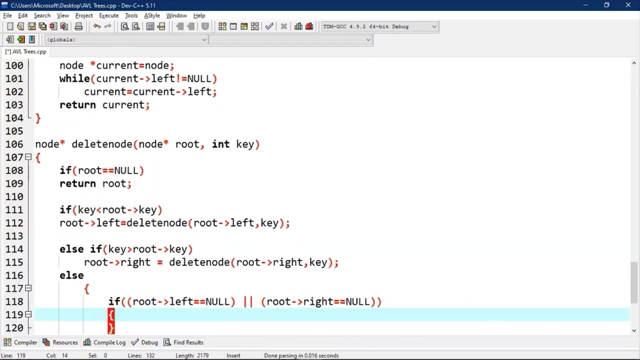 root root to the right is equal to tr$cz% in the right. So if f$$, $$$яз32$$$, $$, $$fob Xbox n to the right is greater than equals to null, then node star temp is equals to root left. 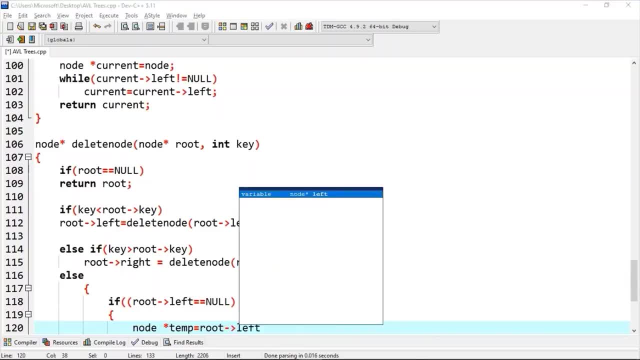 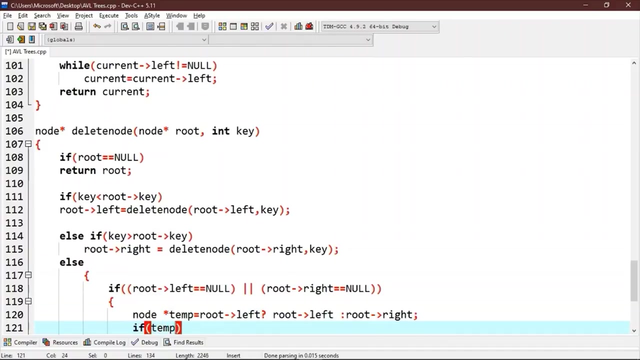 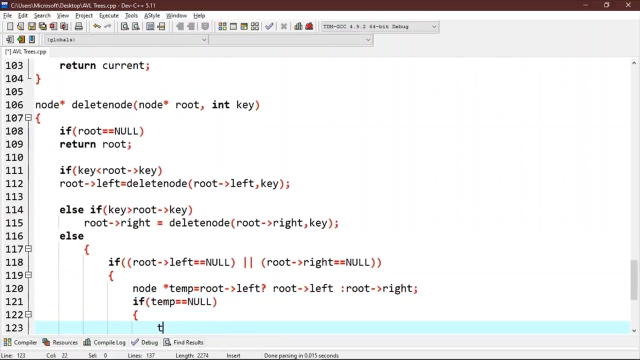 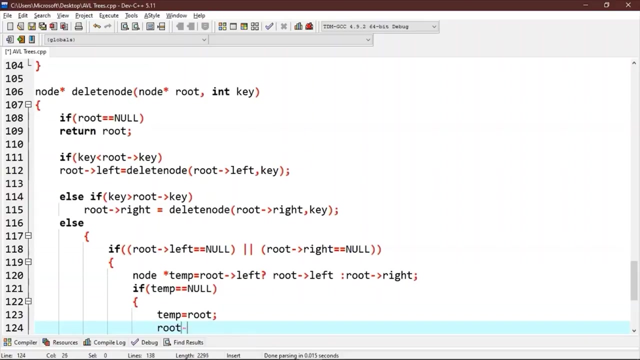 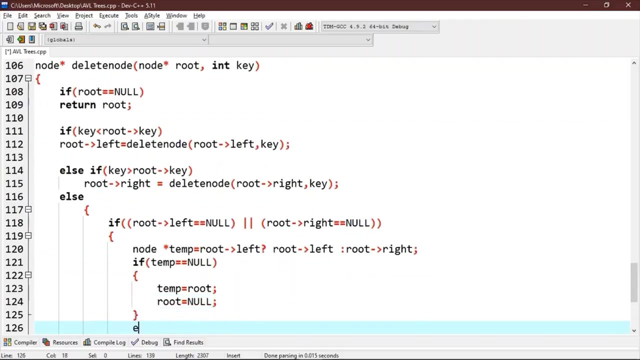 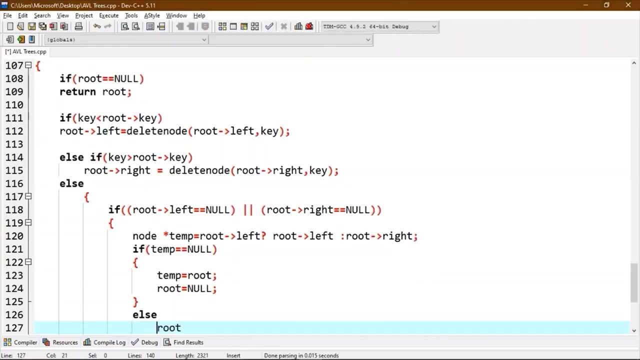 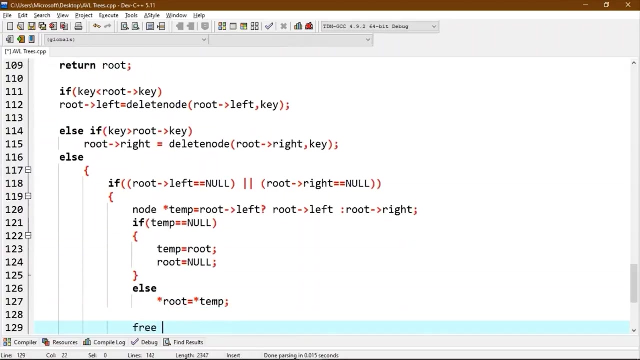 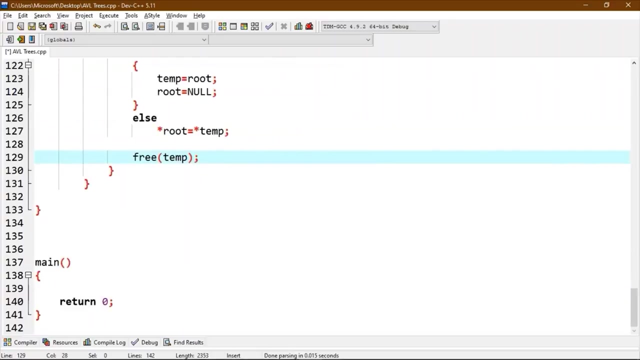 then node star temp is equals to root. right now, if temp is equals to null, then temp will be equals to root and root will equals to null as the result of the query. hence, root will be equals to star temp and free temp. so node: star temp is equals to min value. node. 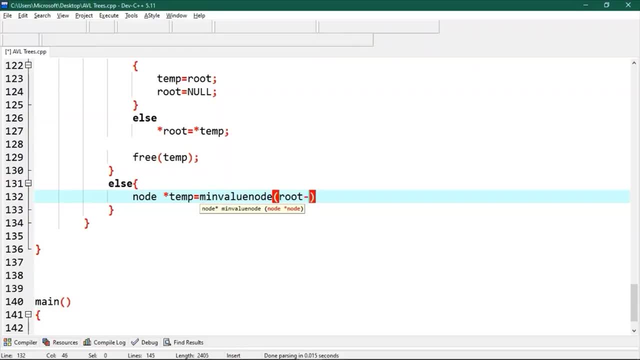 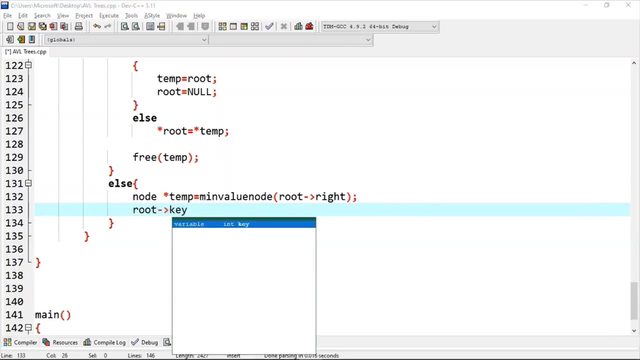 root. Now we will copy the inorder successors data to this node. So root key is equals to temp key. Now we will delete this inorder successor. So root write is equals to delete node root comma temp key. Now, if root is equals to null, then we will return root. 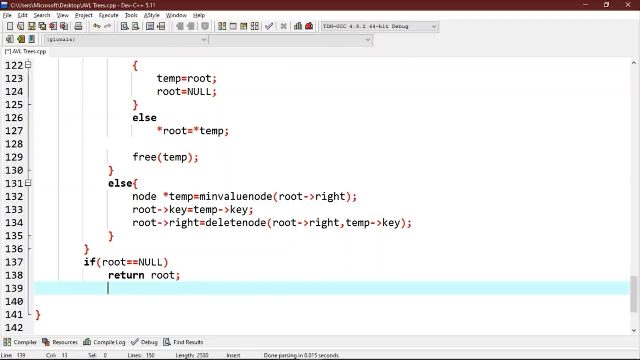 Now we will update the height of the current node. So root height is equals to 1 plus max of height of roots. left comma: height of roots. So now we will get the balance factor of this node. As we can see, we will define root of root height. 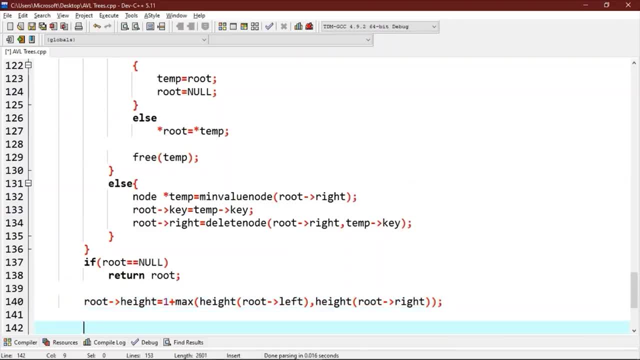 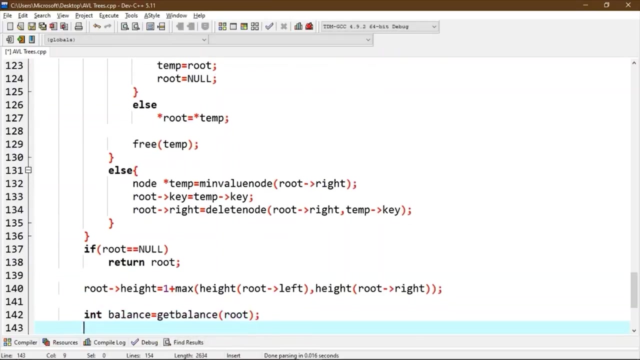 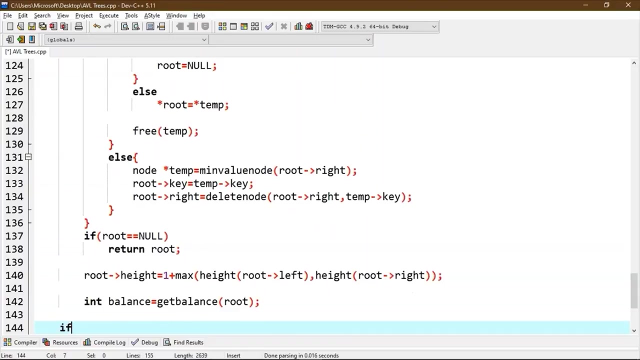 Now we will get the balance factor of this node. Now we will get the balance factor of this node. so int balance is equals to get balance root. if this node becomes unbalanced, then there are four cases. first up ll case. so if balance is greater than one and get balance of roots, left is greater than equals. 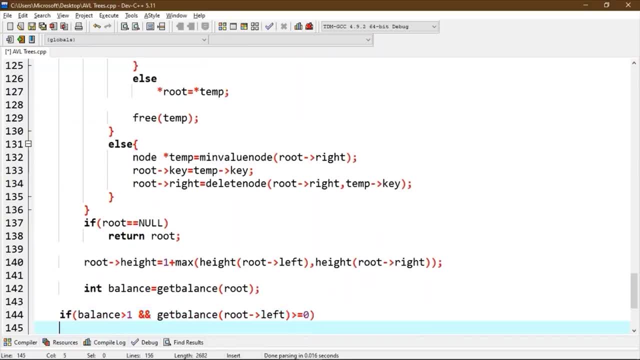 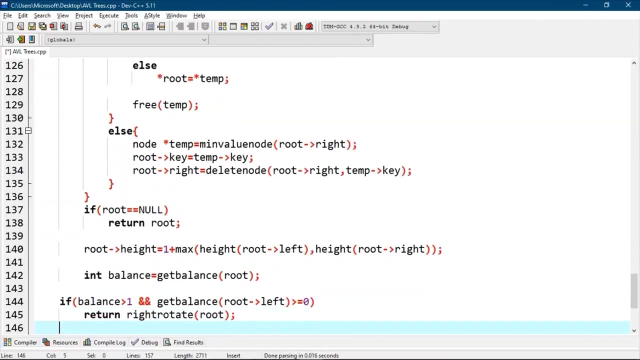 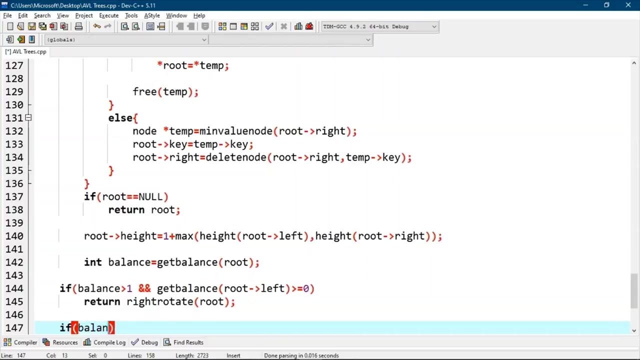 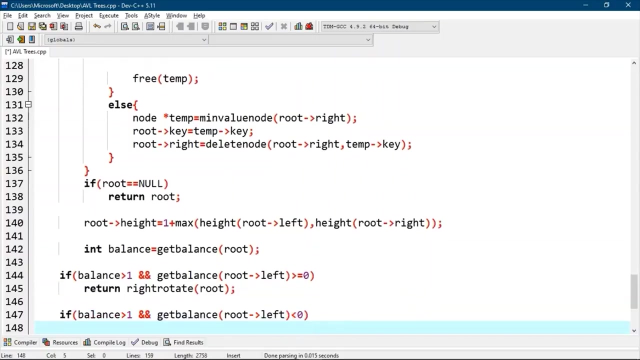 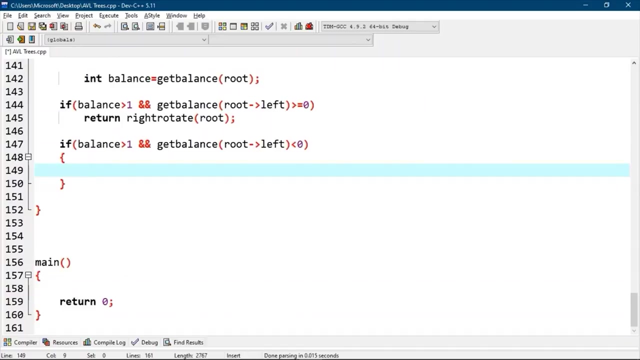 to zero. get balance of roots left is greater than equals to zero, then we will return rightRotate now. if balance is greater than 1 and get balance of root left less than 0, then root left will equals to leftRotate root left. now we will return. 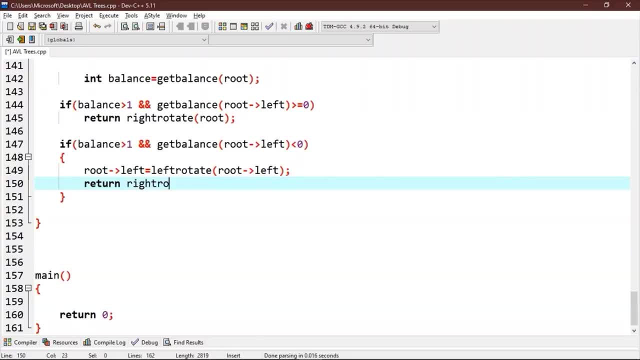 rightRotate root root. now let's write rightRotate case: if balance less than minus 1 and get balance is less than 0 and get balance is less than or equal to 0 and get balance is less than or equal to 0, then we will return. 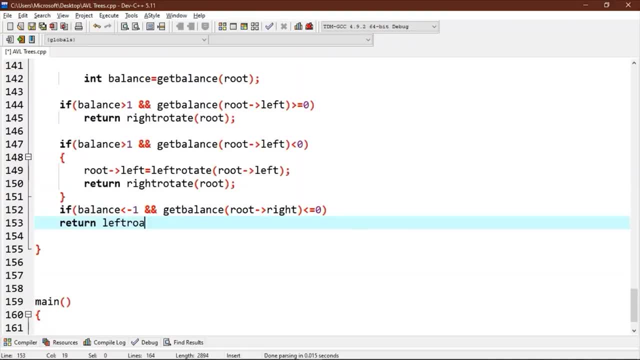 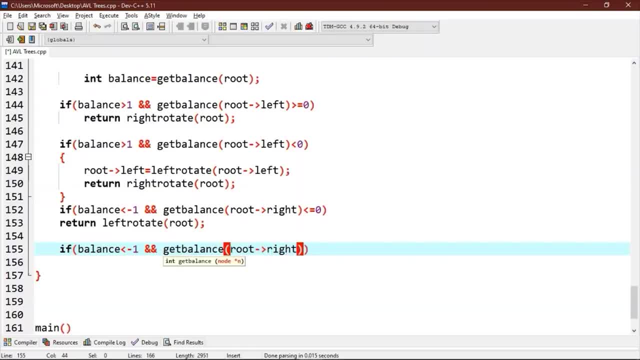 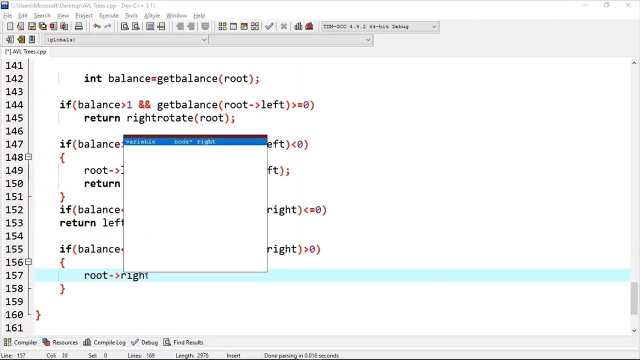 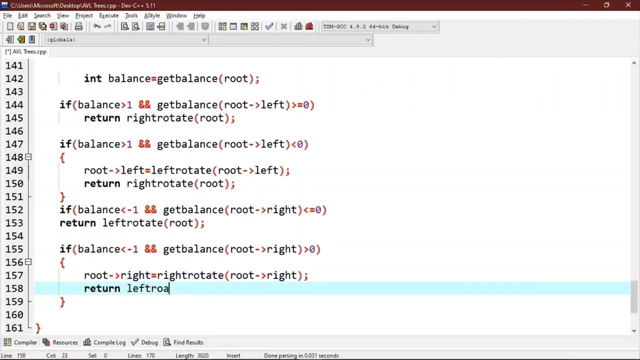 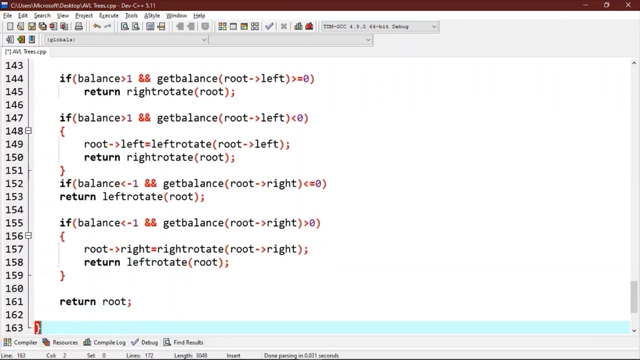 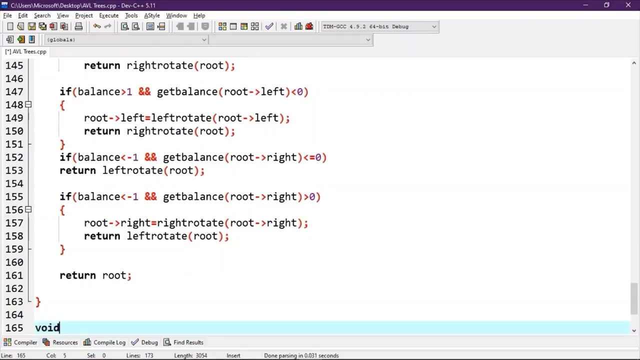 route right right of it's greater than zero, then root right is equals to right rotate of root right now we will return left rotate and we will return the suit now. let's write a function to print pre-order traversal of this tree. so void pre-order traversal of this tree. so void pre-order. 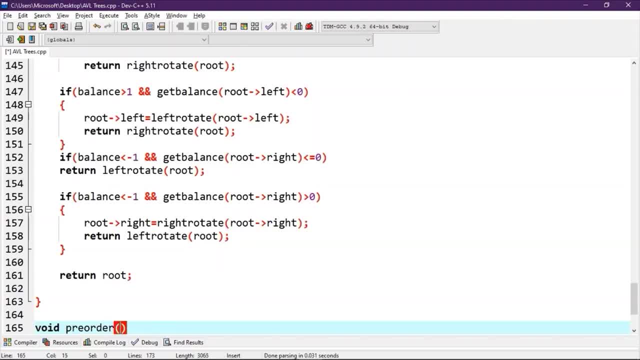 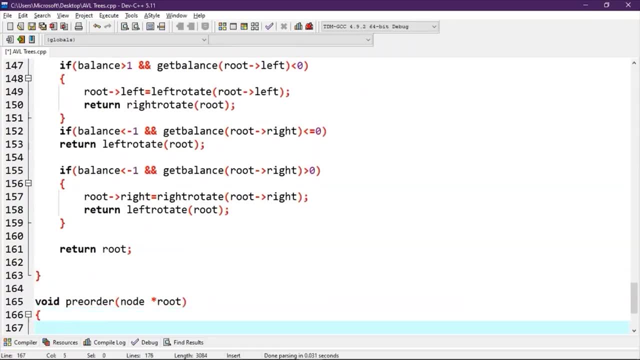 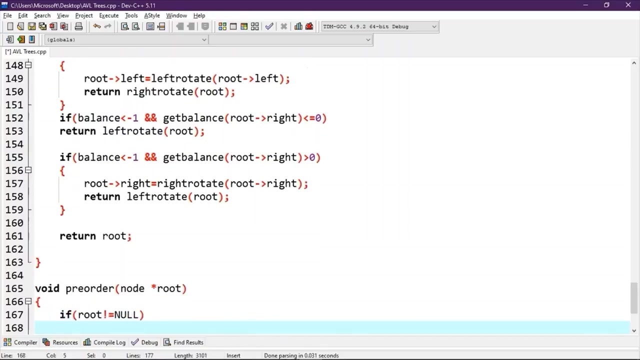 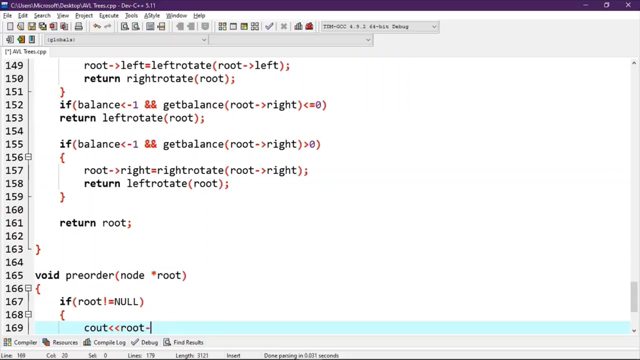 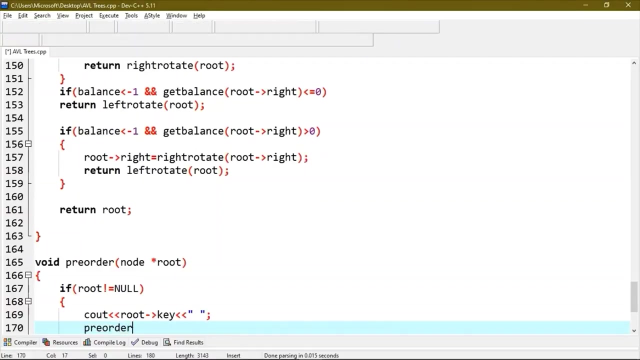 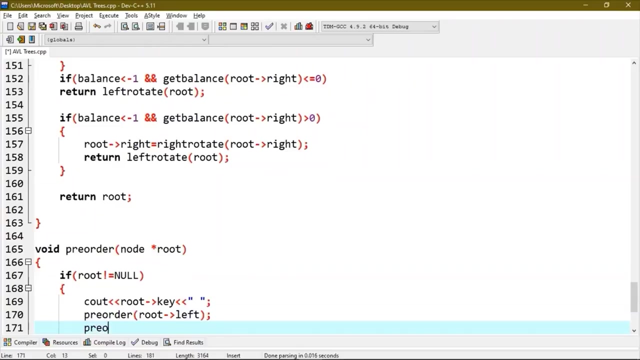 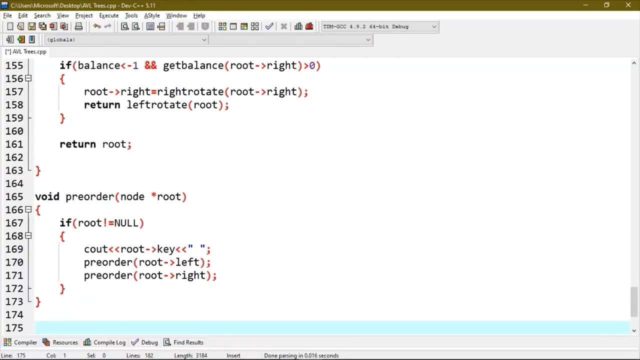 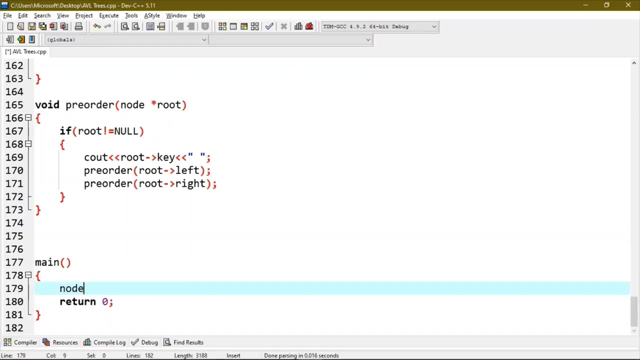 forward star. so if root not equals to null and cout root not equals to null and cout root key, pre-order root duct and pre-order root, write pre-order. now let's write a code for the main block. we will start with an empty tree, so node root. 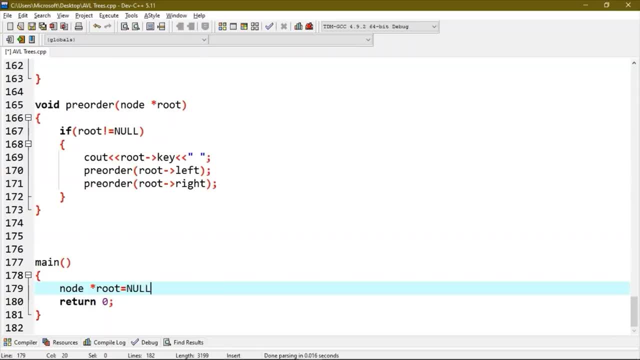 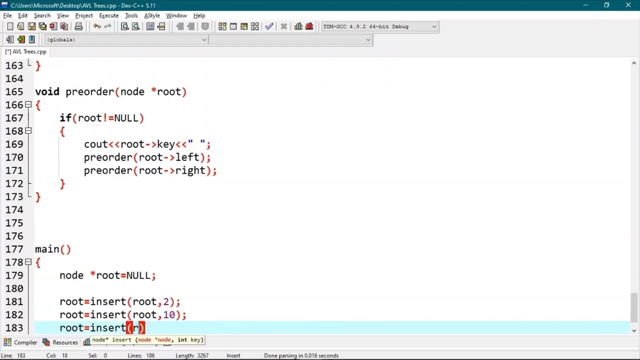 is equals to null. now, root is equals to insert root. comma two: root is equals to insert root. comma ten: root is equals to insert root. comma nine: root is equals to insert root. comma seven: root is equals to insert root. comma five: root is equals to insert root. 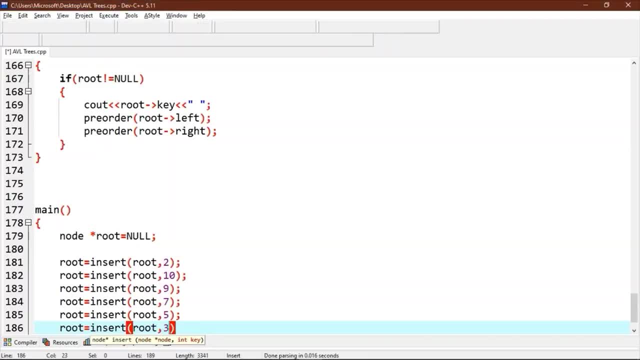 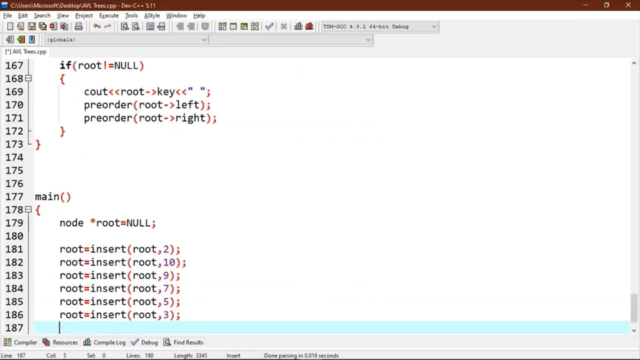 comma three: root comma three, root comma three. now let's try and print this: of avial tree so cout, so cout created avial, avial created preset. so mikk t an an render lé will delete a node. so root is equals to delete node root, comma 10. now let's 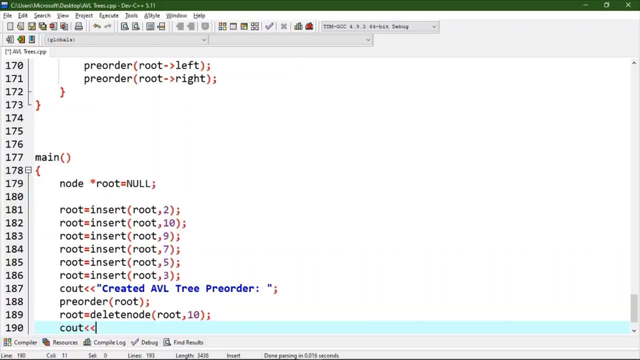 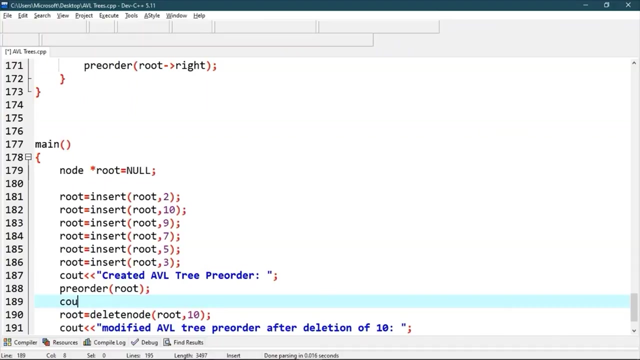 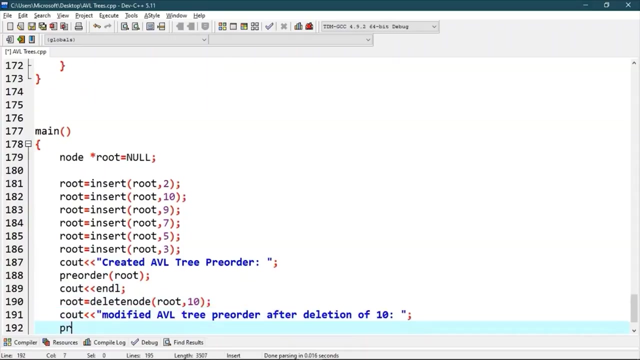 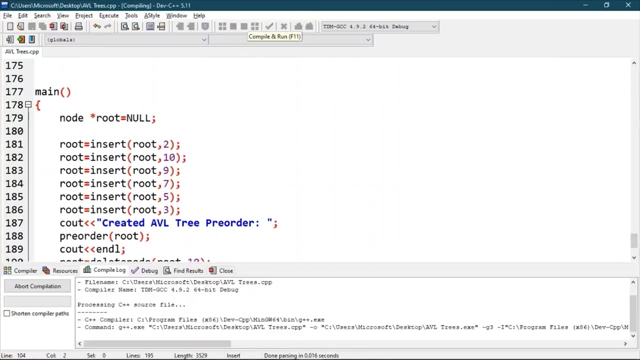 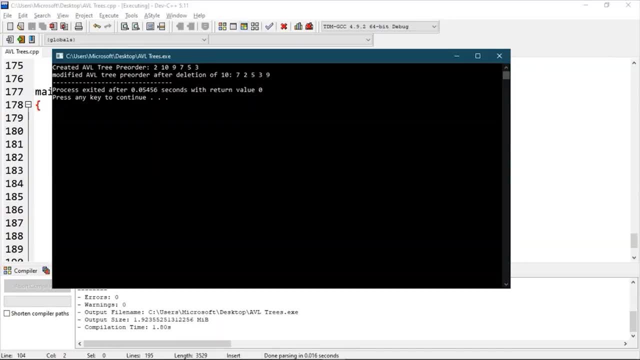 as you can see, our deletion function is. as you can see, our deletion function is working perfectly, working perfectly, working perfectly. now let's get back to our slides at last. now, let's get back to our slides at last. now, let's get back to our slides at last. let's sum up what we have learned from. 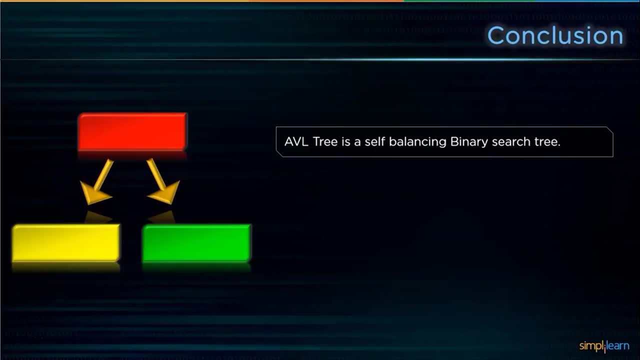 let's sum up what we have learned from. let's sum up what we have learned from this session, this session, this session. first up avial trees is our self-balancing first up avial trees is our self-balancing first up avial trees is our self-balancing binary search tree. 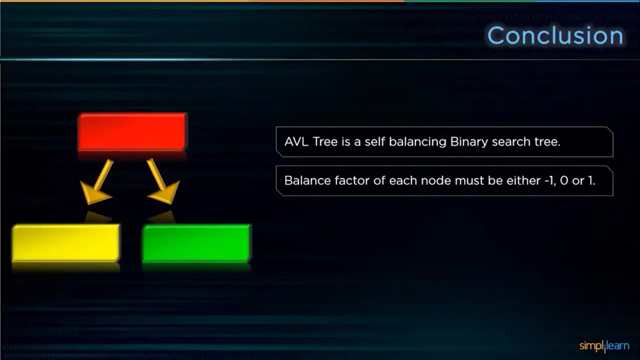 binary search tree. binary search tree. next, every node must have a balance. next, every node must have a balance. next, every node must have a balance factor of either factor of either minus 1, 0 or 1.. Next, after every rotation, we must verify if each node is balanced or not. 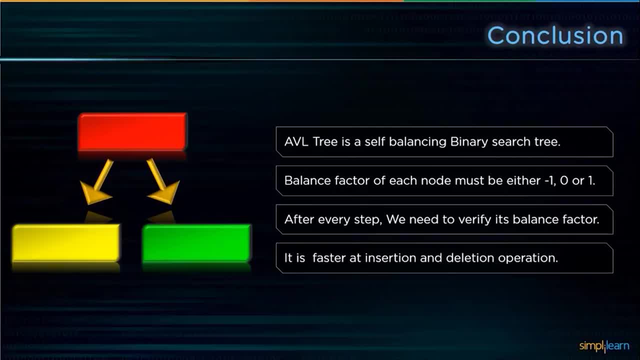 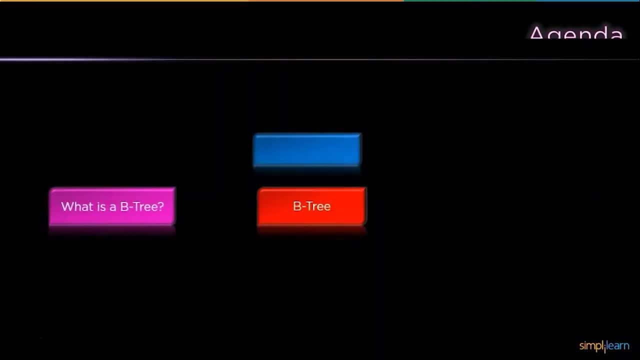 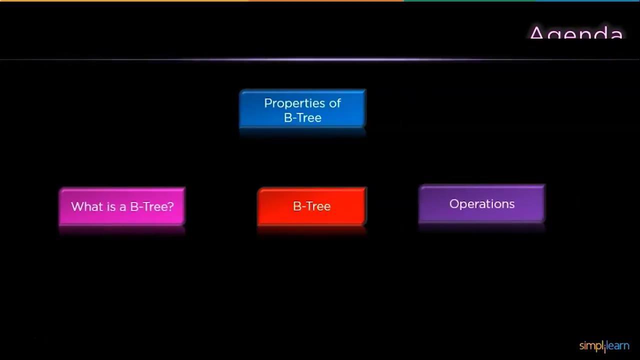 Finally, AVL trees offers fast insertion and deletion operations. B-trees: We shall begin by introducing B-trees, Then we will discuss the properties of B-trees. After that we will try various operations on them, like searching, insertion and deletion. 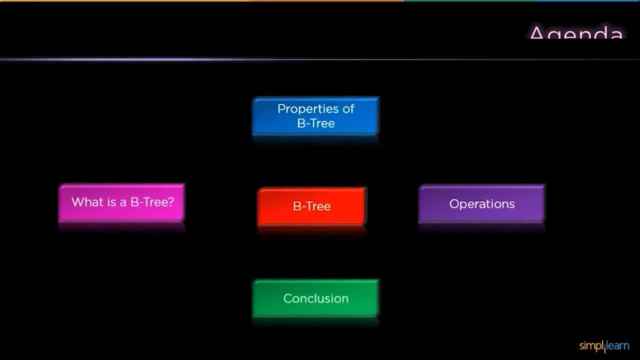 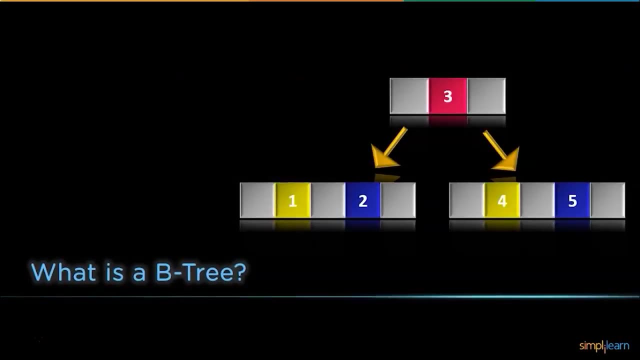 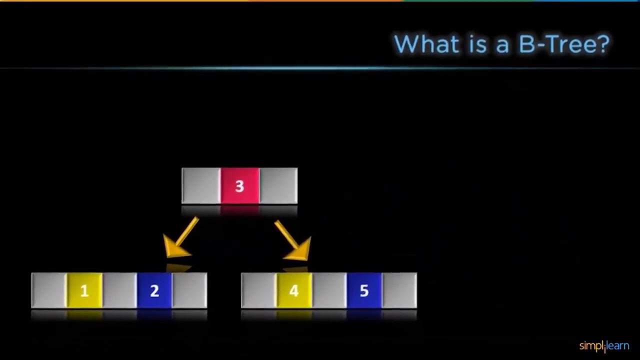 Finally, we will sum up what we have learned from this session, But before we begin, make sure you have subscribed to our YouTube channel and clicked on the bell icon below So you never miss an update from Simply Learn. So, without any further ado, let's get started with. what is B-tree? 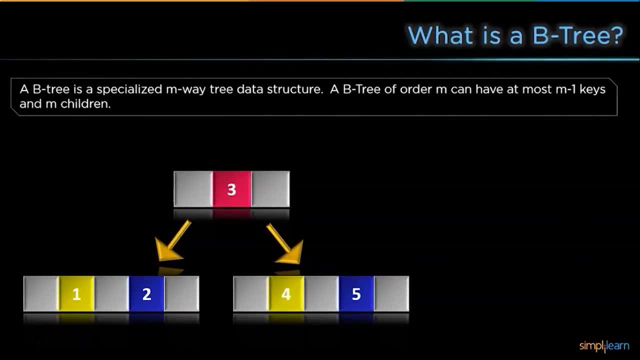 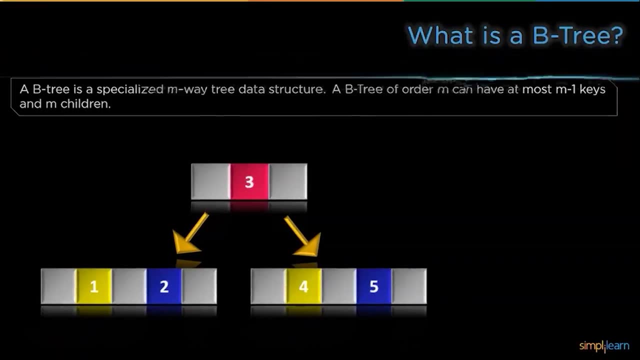 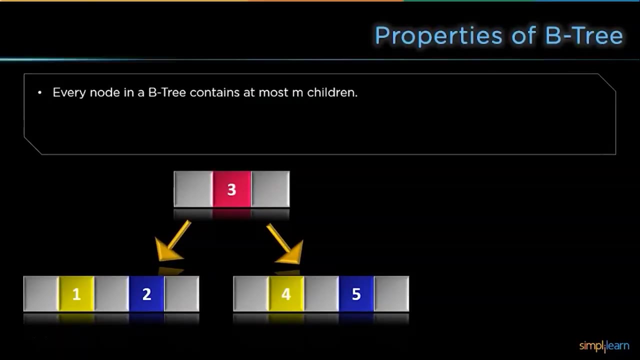 B-tree is a special M-way tree data structure. A B-tree of order M can have at most M-1 keys and M children. Now let's discuss some properties of B-trees. First up, every node in a B-tree can have at most M elements. 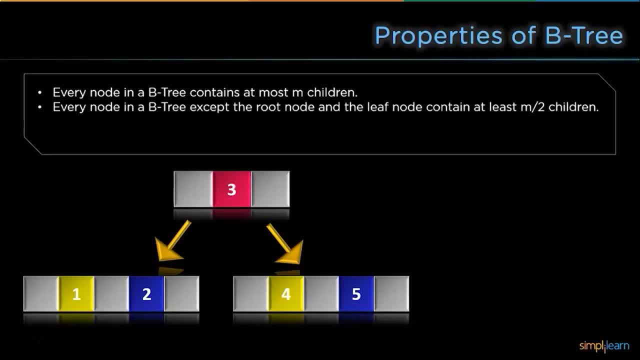 Next, every node, except the root and the leaf node, must have M by 2 children. Next, a root node must have at least two nodes. At last, a leaf node must be at the same level. Now let's discuss what are the various operations we can do. 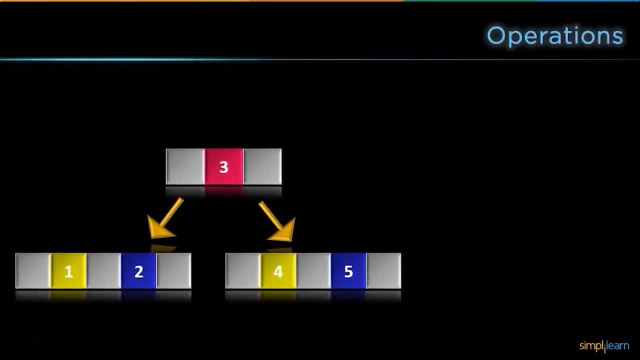 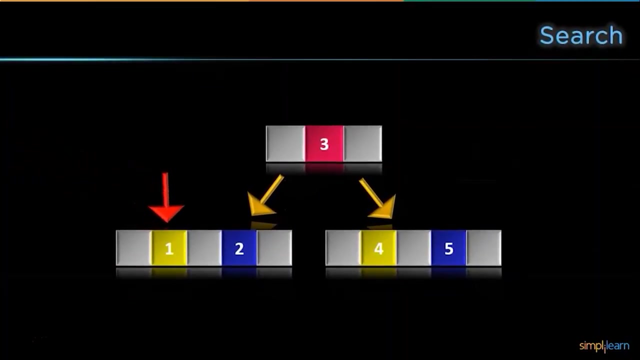 First, we can perform three operations on a B-tree. We can perform three operations on a B-tree, That is, searching, insertion and deletion. Let's discuss these in detail. First up, searching. In this we will traverse the complete B-tree until we have found a key. 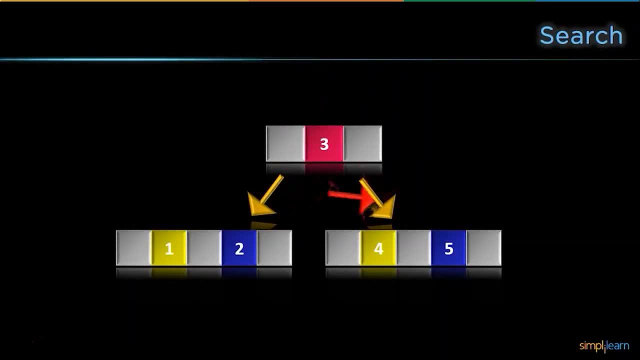 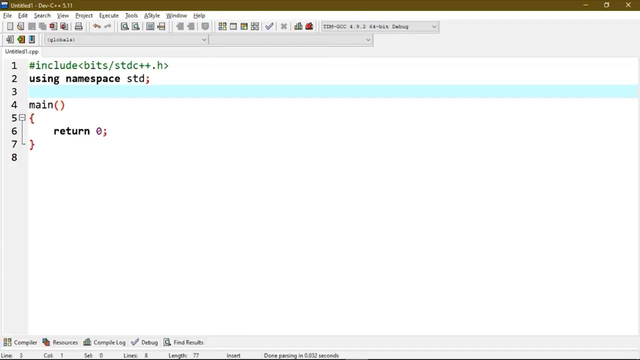 We will start from the left side to go all the way up to the right side. Now let's try this in a code editor. We will first start by creating a B-tree node. To do that, we will use class B-tree-node. 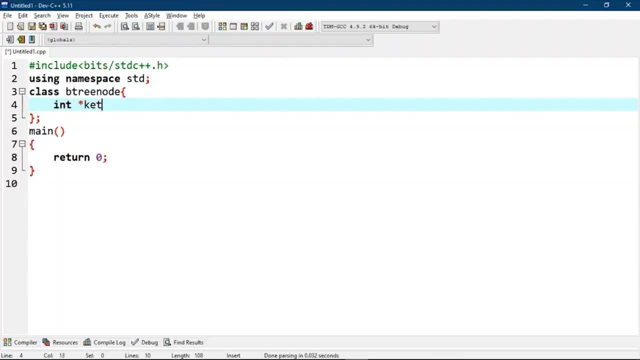 int keys- It is an array of keys. Then int t. This will define the range of the number of keys. Then we will create a child pointer, B-tree-node-tree. It is an array of child pointer, Then a variable to check the current number of keys. 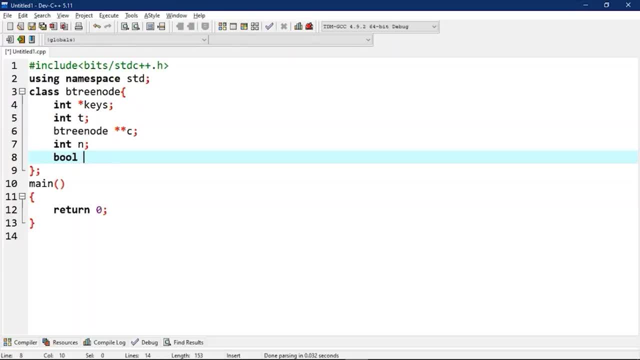 And a boolean variable, which will be true when the node is leaf. Now define some functions in public: First constructor, Then the function to insert a new key in the sub-tree void. Insert Non-full Argument as int k. 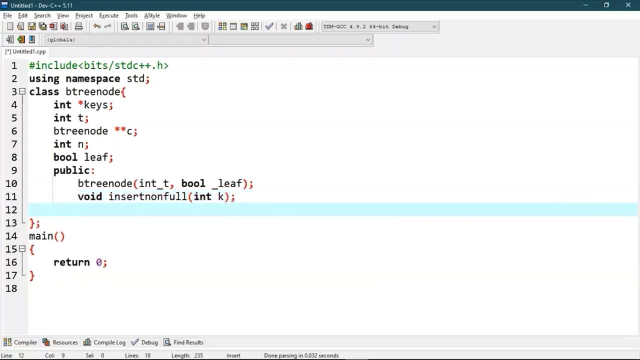 In this case we will use a function to insert the key, Then a function to insert a new key in the sub-tree. Next, a utility function to split the child y of the node, That is, int i, comma a, btree node pointer y, a function to traverse the btree. 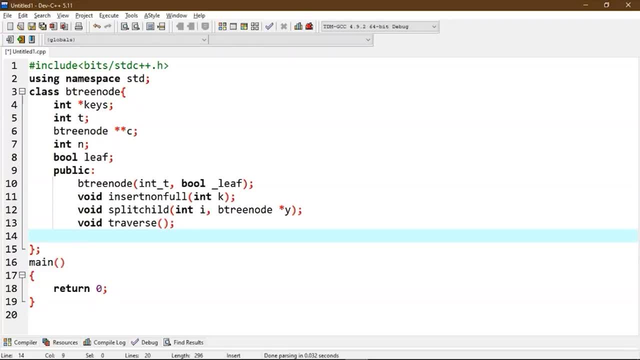 and a function to search a key in the subtree. It will return null if key is not present. Now we will create another class, btree, and make it a friend of this so that we can access private members of this class in btree function. 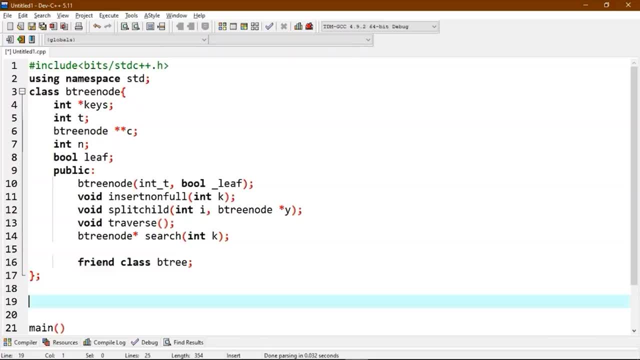 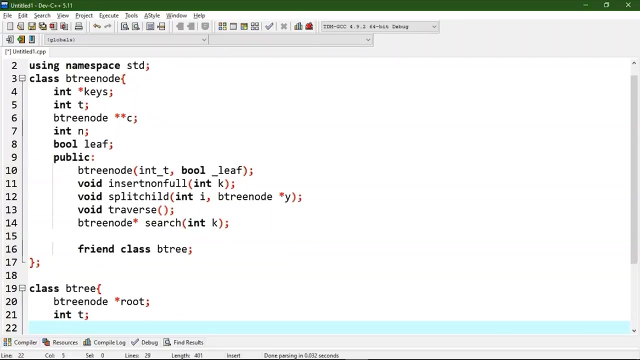 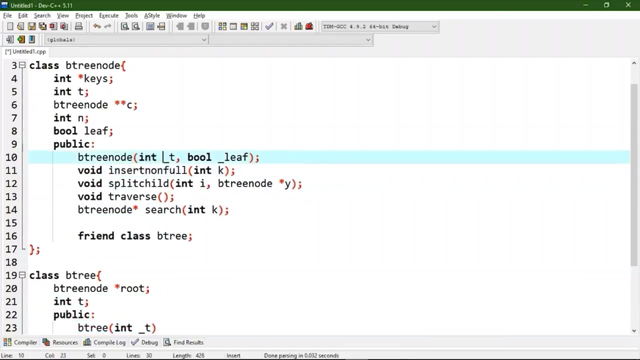 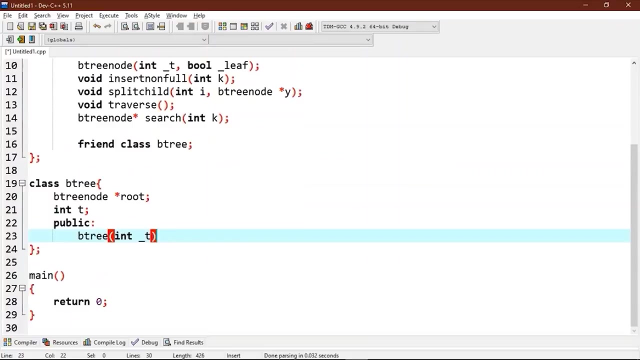 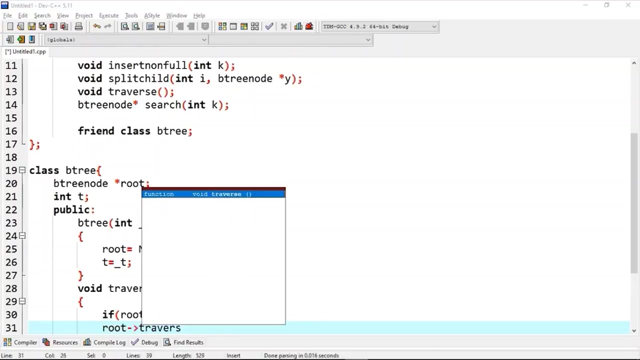 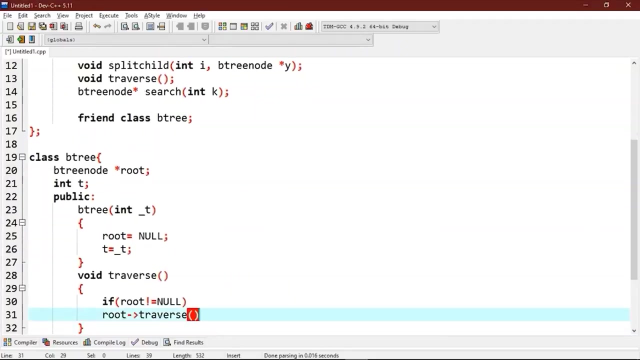 Now we will create a pointer, root gradient, minimum degree, then public a constructor btree. root equals to null and t is equals to t. Now we will write a function to traverse this tree, So it traverse, if not null, then root traverse. 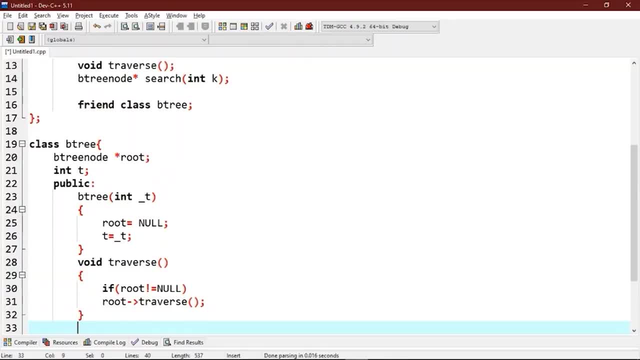 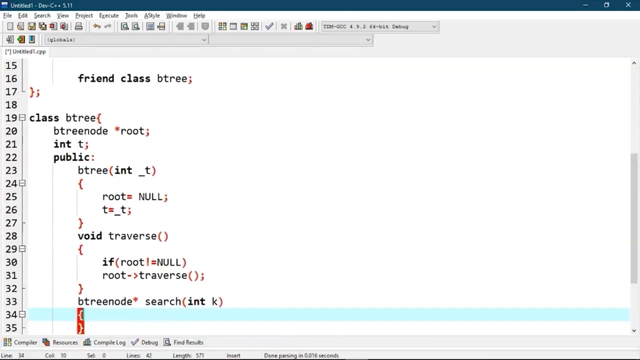 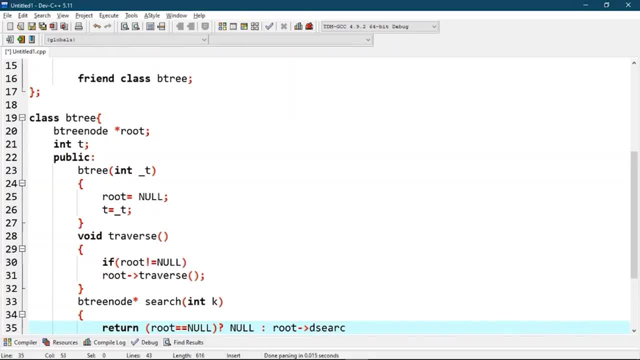 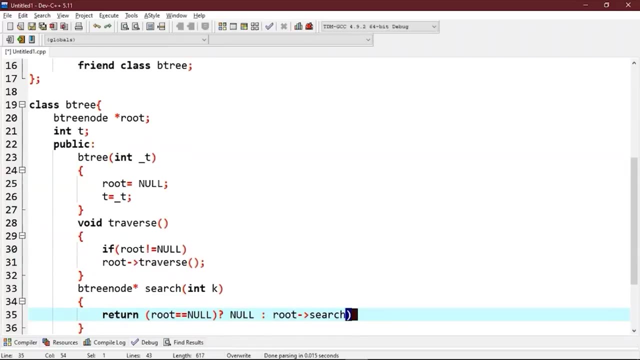 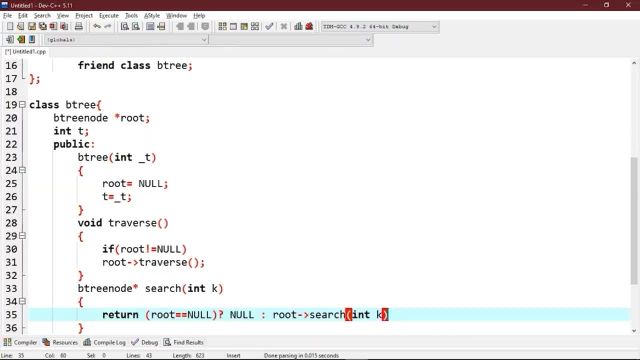 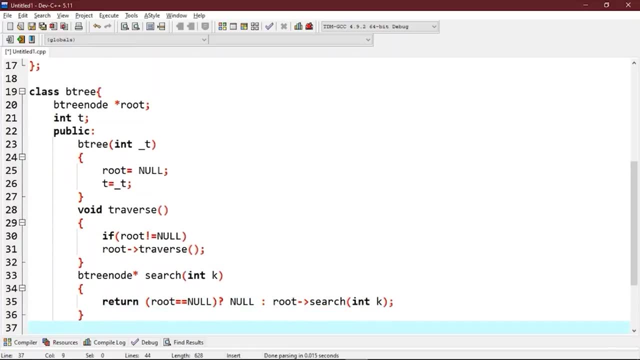 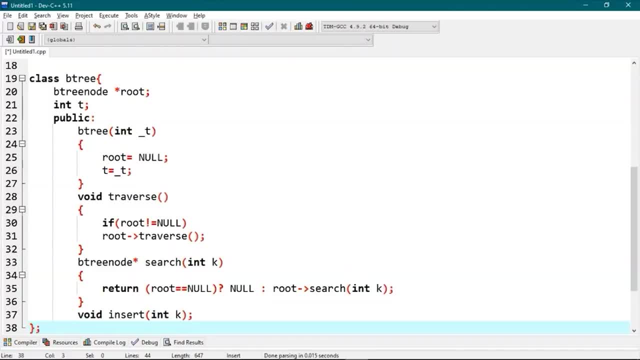 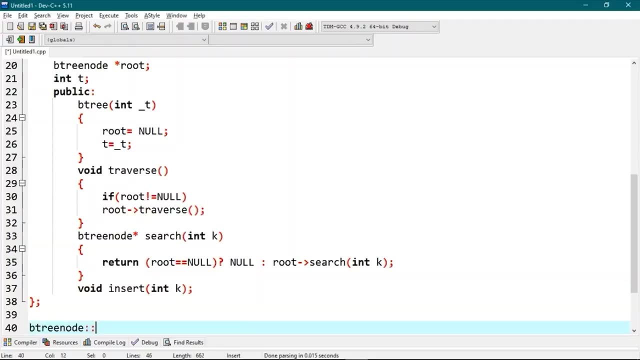 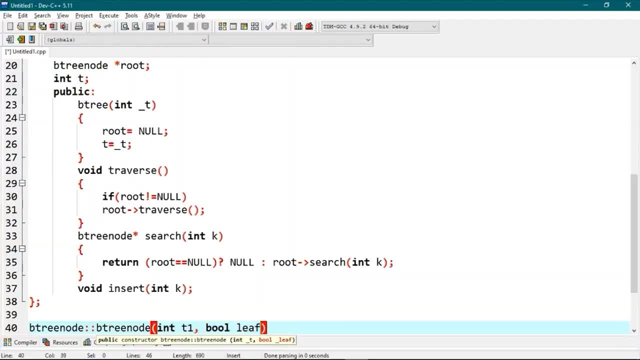 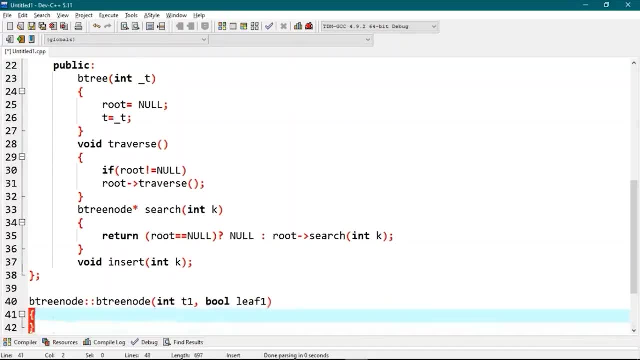 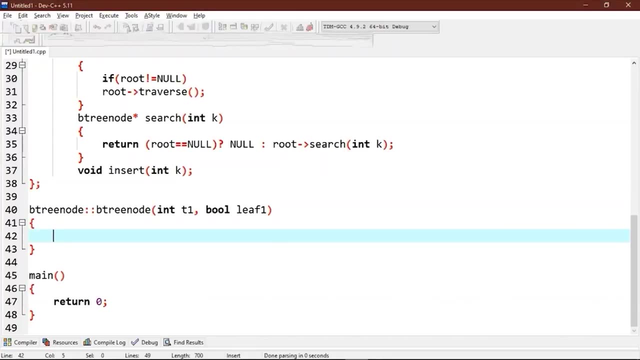 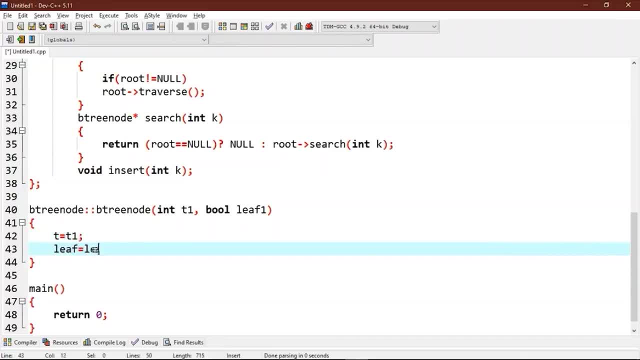 return, return, return, return. Now we will allocate the memory of the maximum number of possible keys and the child pointer, and c equals to new btree code: star bracket 2, star t. Now we will initialize the number of keys as zero. Now let's write the function to traverse all nodes in the sub-tree rooted with this. 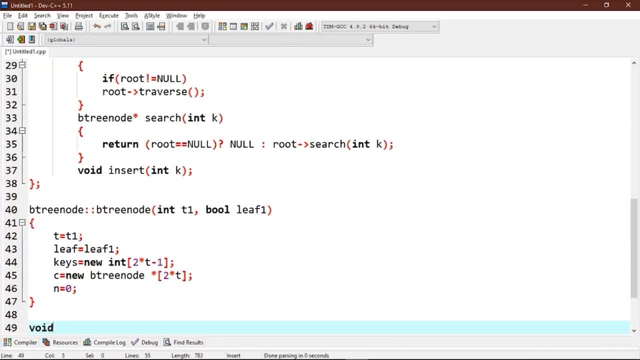 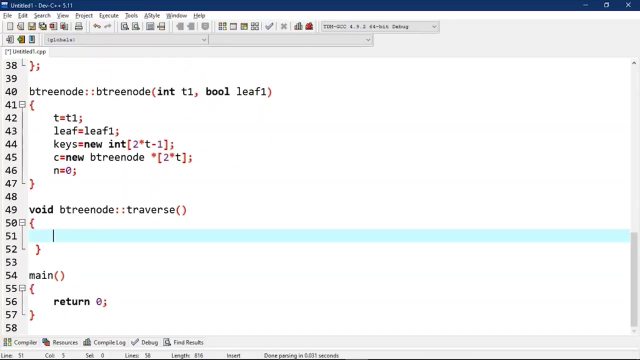 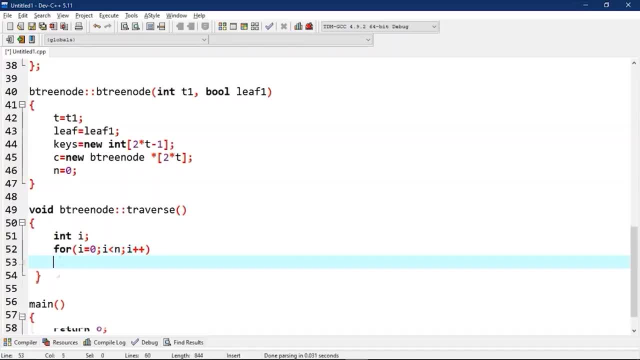 n? i plus plus, If this is not leaf node, then before printing key traverse the subtree rooted with child c i. So if leaf is equals to false, then c bracket i L equals to traverse, else cout case. Now we will print the sub-tree routed with the last node. 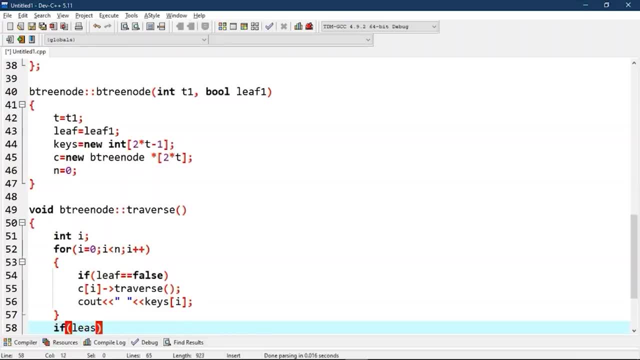 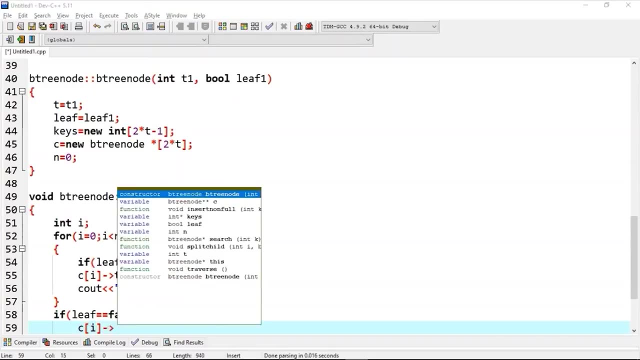 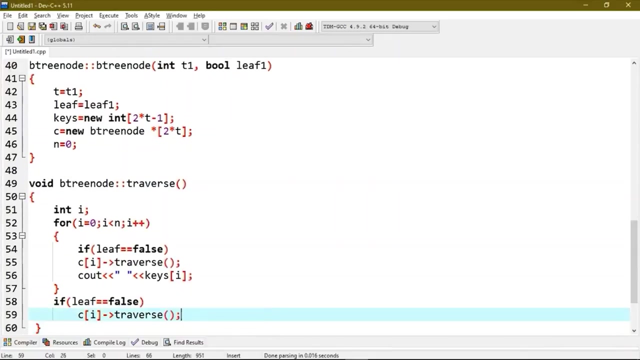 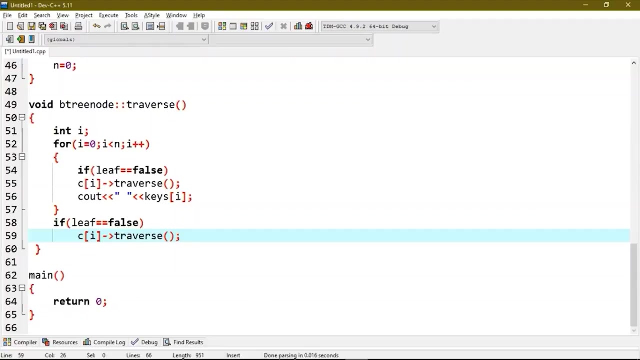 So if leave equals to false and c i traverse and c i traverse and c i traverse. Now we will write the function to search key k in sub-tree routed with this node. So btreeNode or btreeNode is search int k. We will first find the first key greater than or. 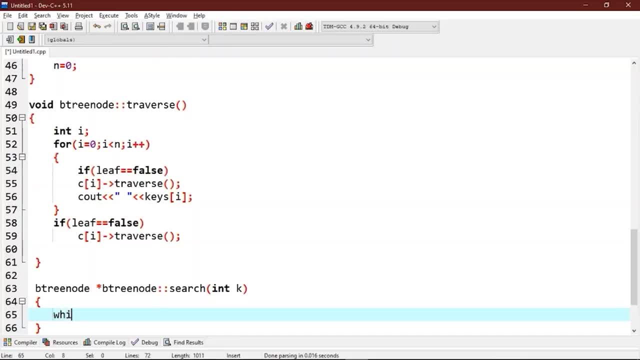 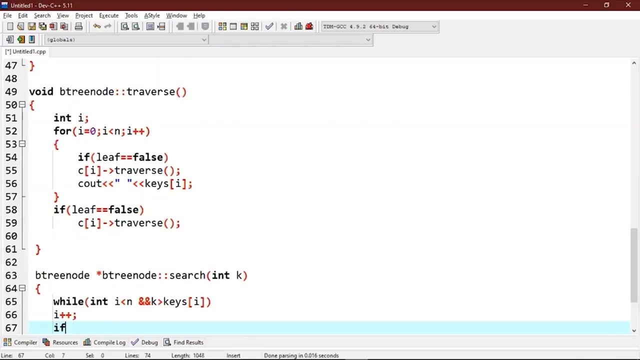 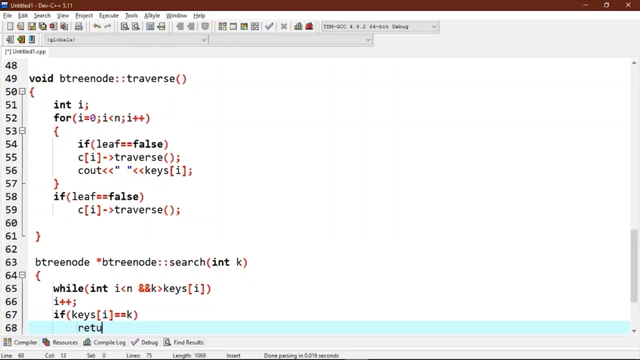 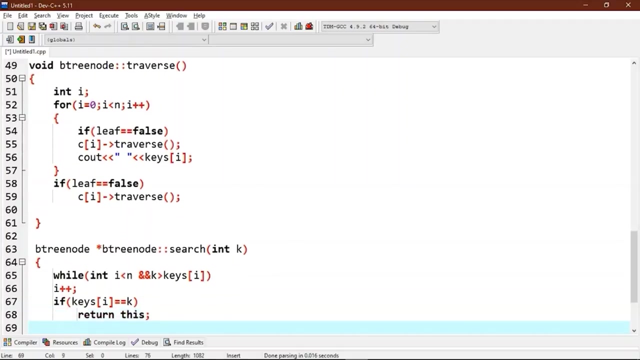 equal to k. so while int i is less than and and K is greater than, is bracket I, then I++. Now, if we found the key is equals to K, then we will return this node. if bracket I is equals to K, then we will return K. if key is not found here- and this is a leaf- 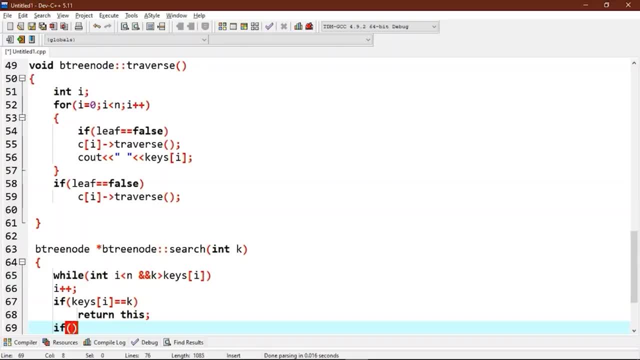 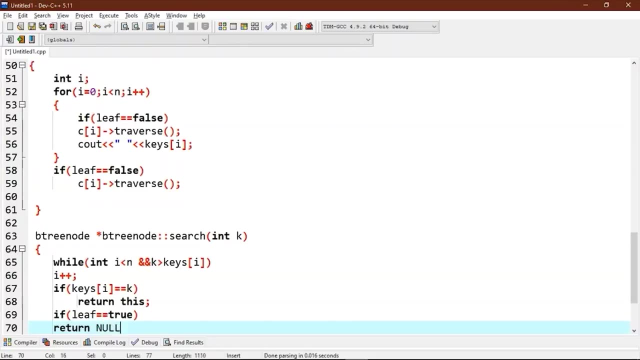 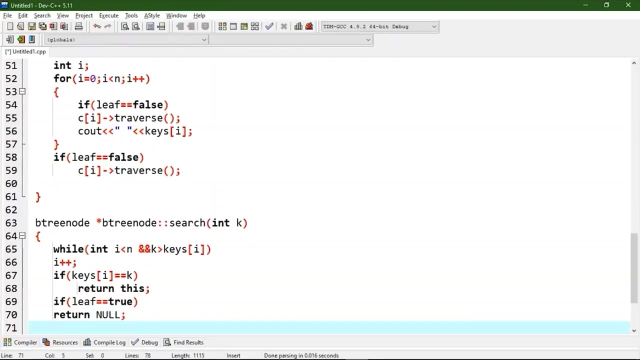 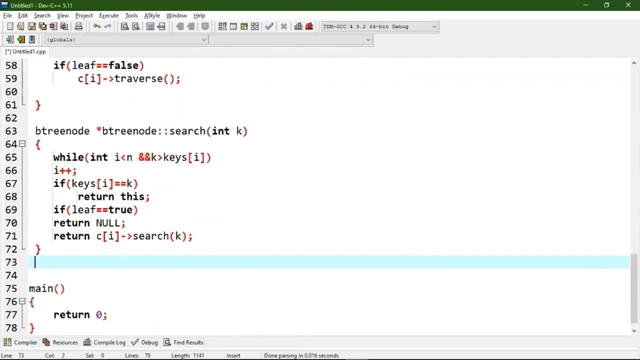 node, then if leaf is equals to true, then we will return L. Now we will try to go to the appropriate child, so we will use return C, bracket I arrow search. now we will write the bean function that insert the new key in this B tree. so void B, tree insert and K. so if root is equals to NULL, then we will return. 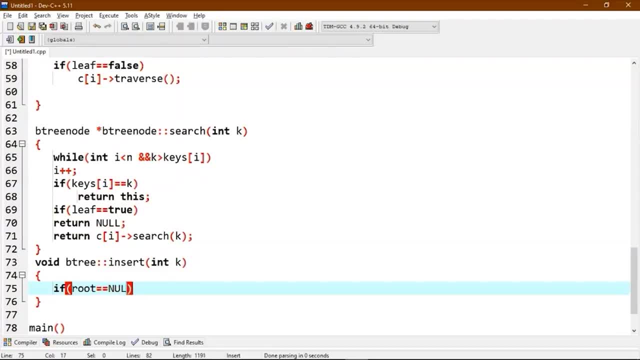 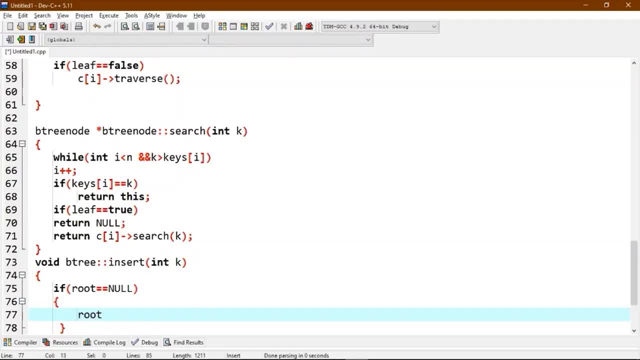 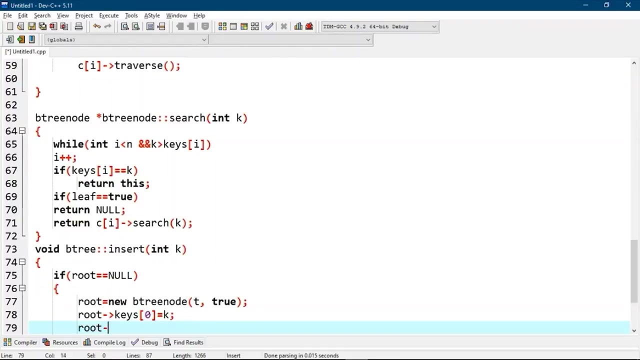 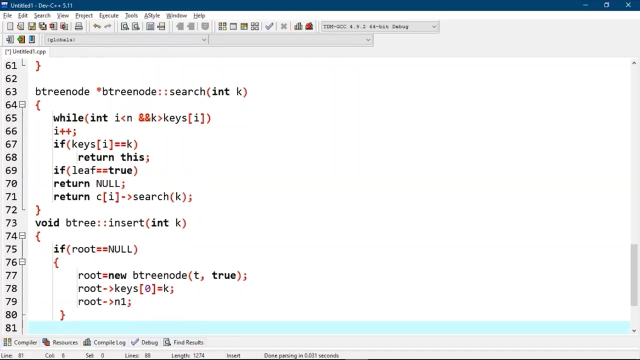 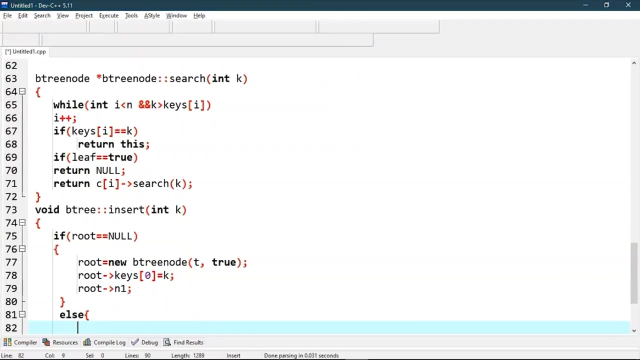 Then we will relate the memory of for root. Thank you Now root keys. bracket zero is equals to K. Now we will change root. Here we are updating the number of keys in this root Now. if else else, if tree is not empty, then if root is full, then tree grows in height. 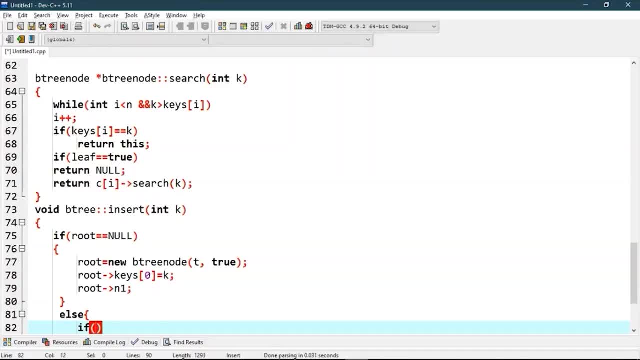 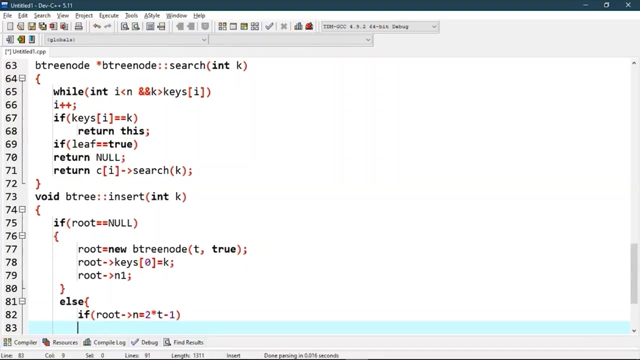 So if root arrow N Is equals to 2 star T minus 1.. Then we will allocate the memory for the new root B tree Rote star S equals to new B tree node T, comma false. Now we will make the old root as child of the new root. 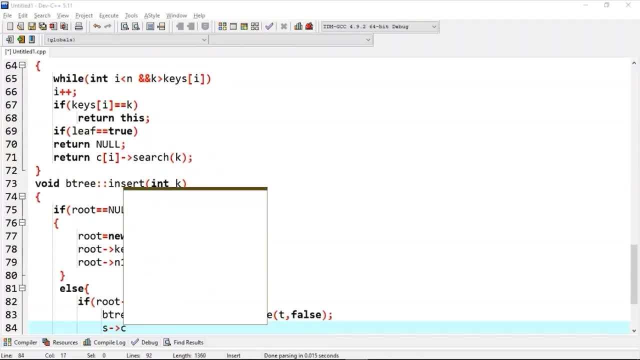 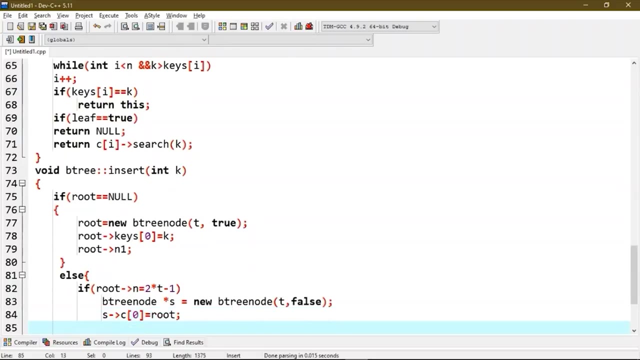 So S arrow C bracket zero Is equals to root. Now we will split the old root and move one key to the new root. So S split child Zero comma root. Now new root has two childrens. We have to decide which of the two children is going to have a new key. 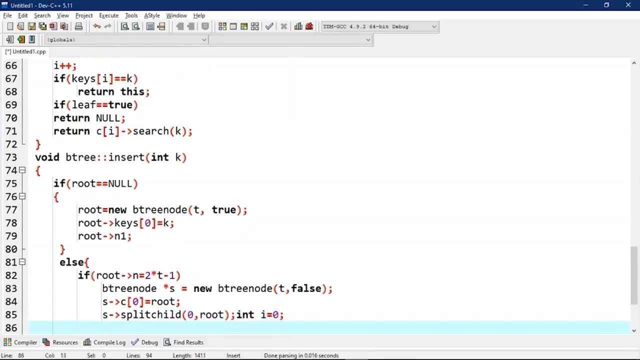 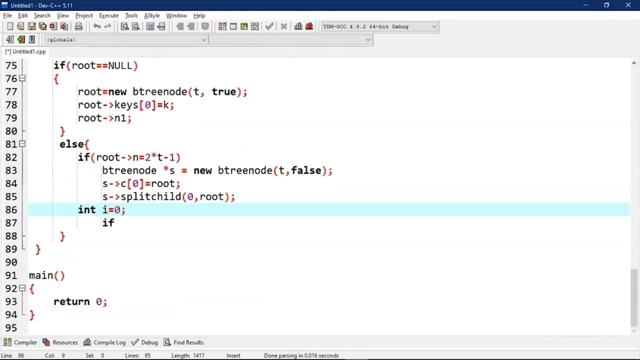 So int I is equals to 0.. If, If As Add a new name As Not And The key is 0 is less than k, And then i++ and s arrow, c bracket i arrow insert known full k. 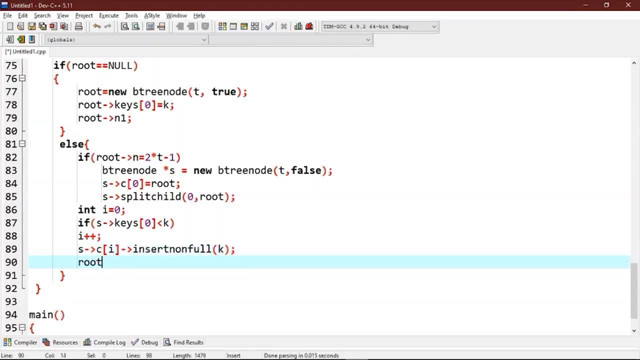 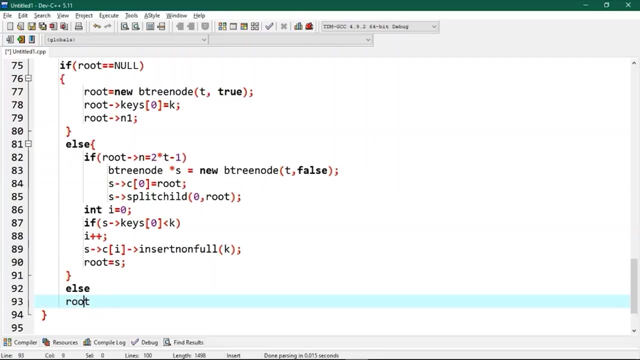 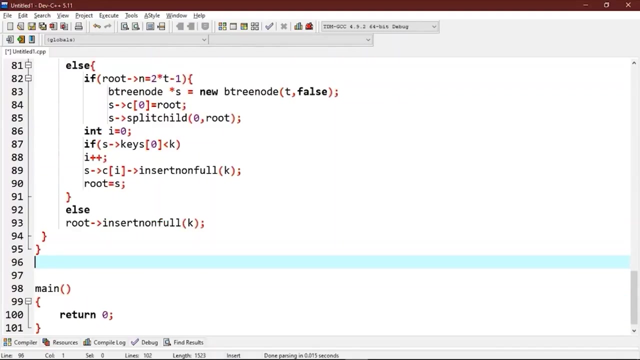 Now we will change the root equals to s. else if root is not full, we will call the insert known full k. Now we will write a function insert for known full k. we will initialize: int. size equals to n-1 if it equals to true. 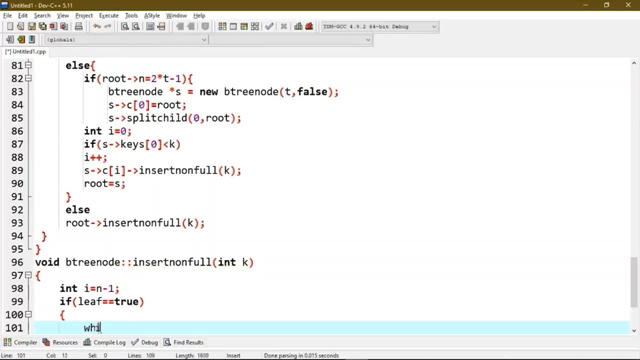 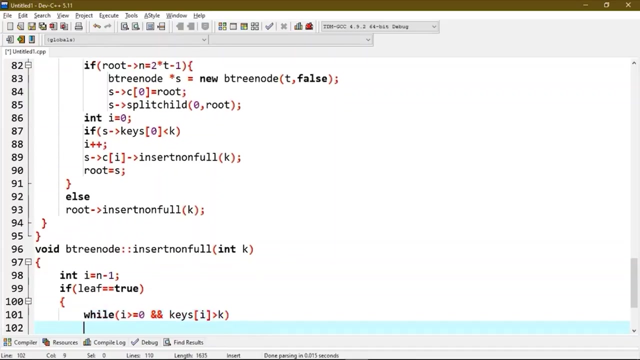 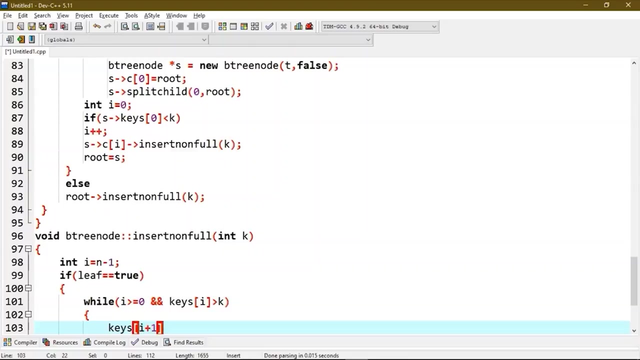 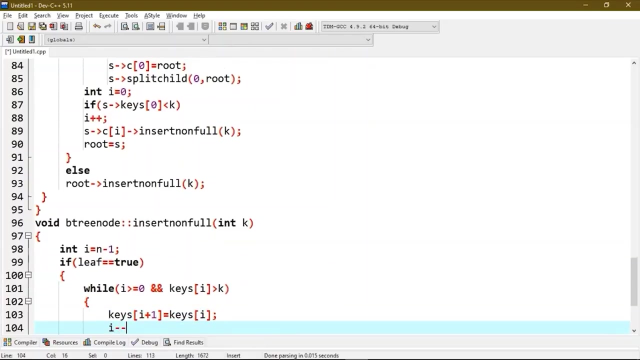 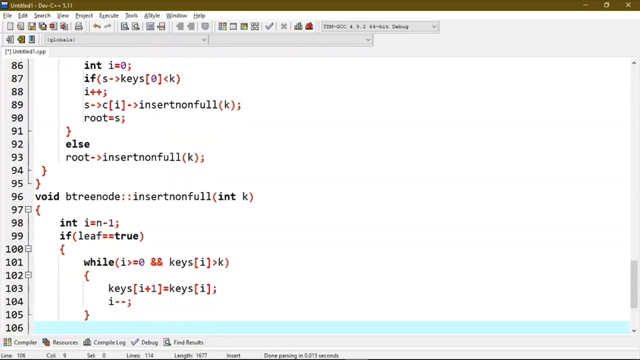 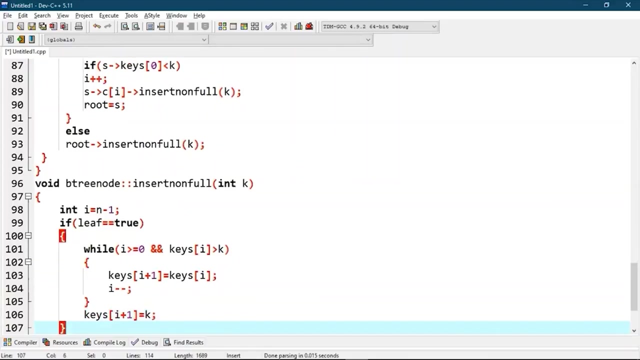 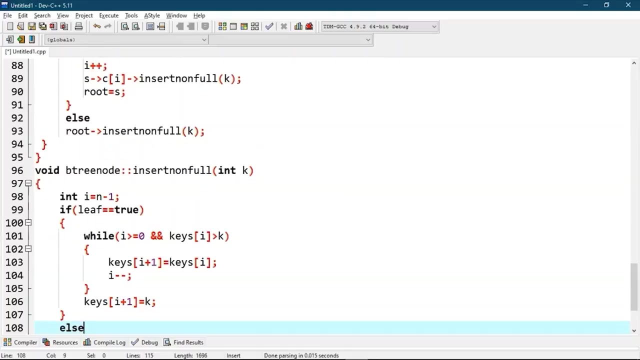 than, while i is greater than or equals to 0 and keys is greater than k, then keys i plus 1 will be equals to keys i and i minus minus. now we will insert the new key at the found location. else, while i is greater than, equals to 0. 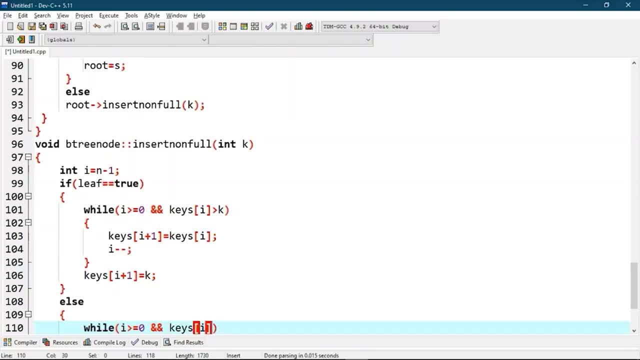 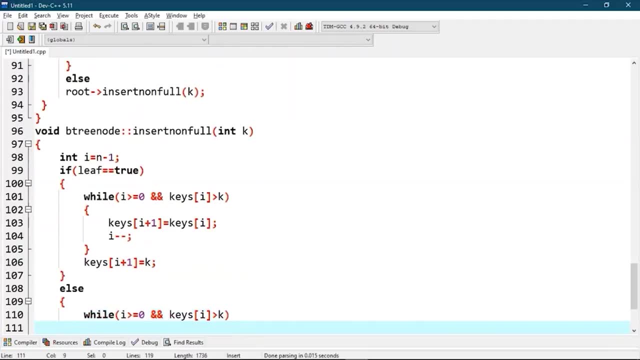 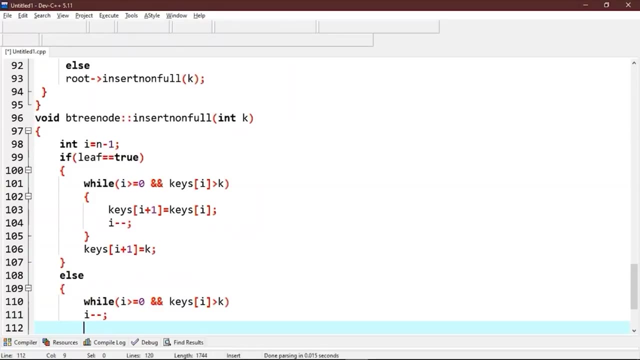 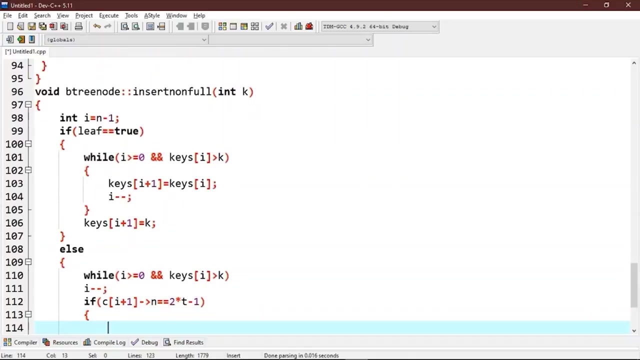 keys i is greater than k, then i minus minus. now we will see if the found child is full. if c bracket i plus 1 l is equals to 2 star t minus 1, then we will use split child: i plus 1 comma c, i plus 1. 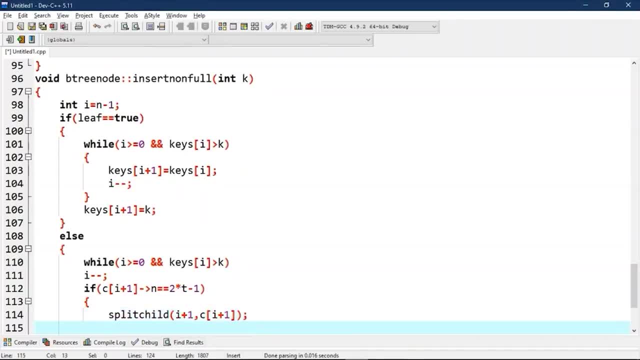 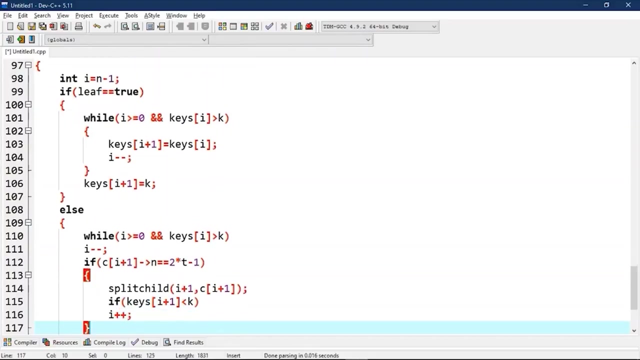 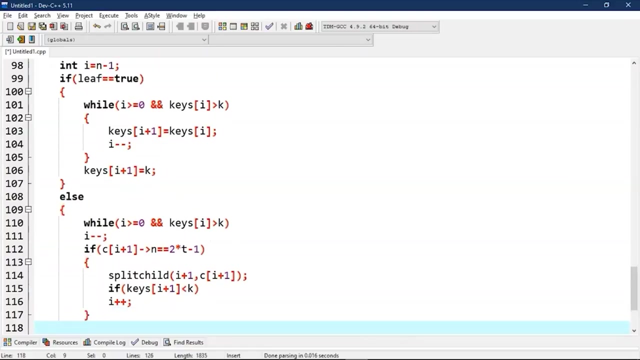 they will be equal to key 1, 3, 4, 5, 6, 7, 8, 9, 11, 2, 3, 1, 2, 1. keys bracket: i plus 1 is less than k. then i plus plus c, i plus 1. 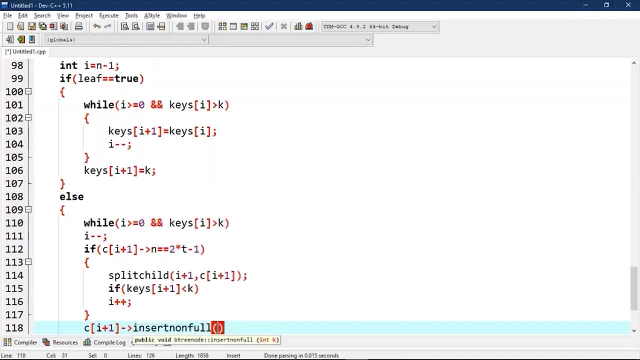 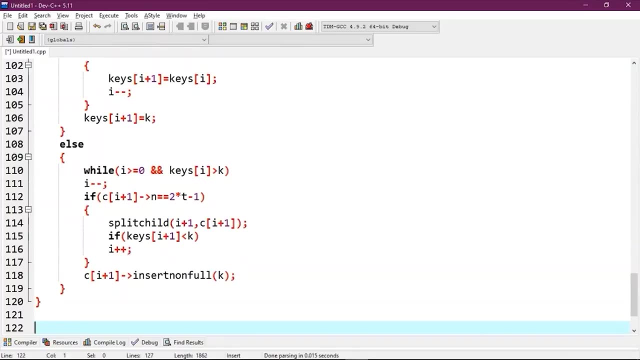 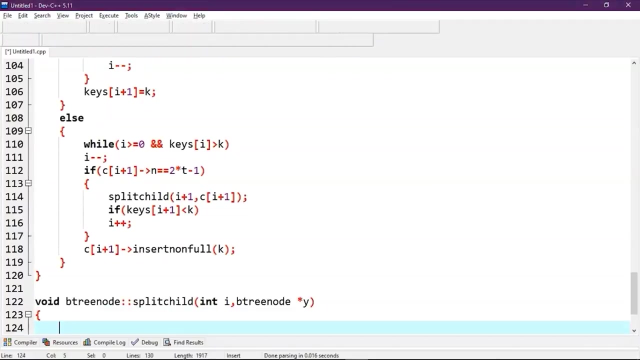 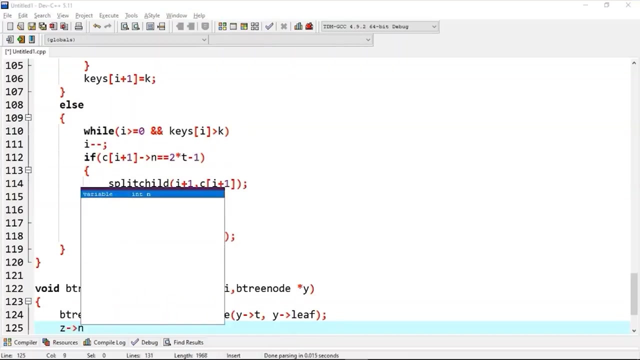 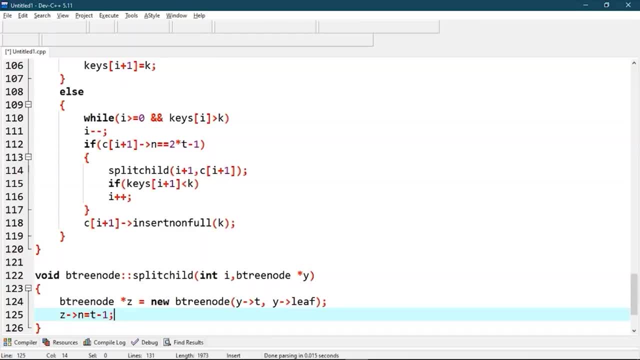 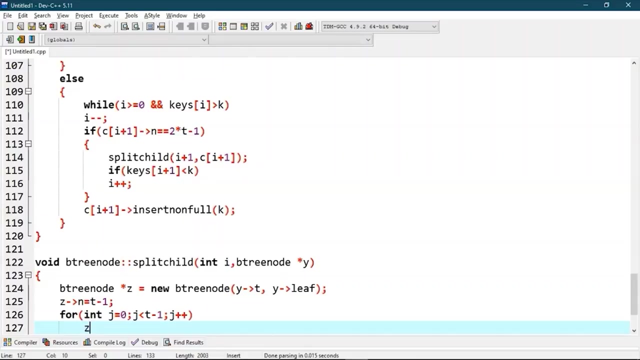 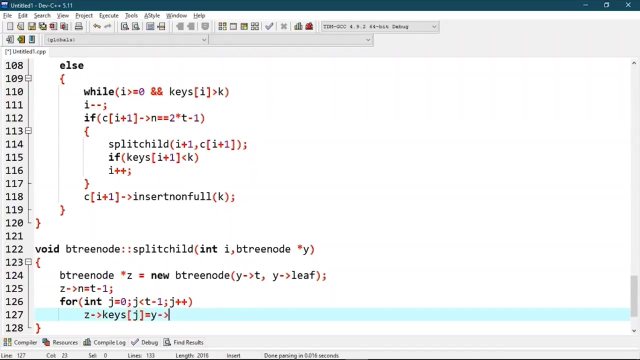 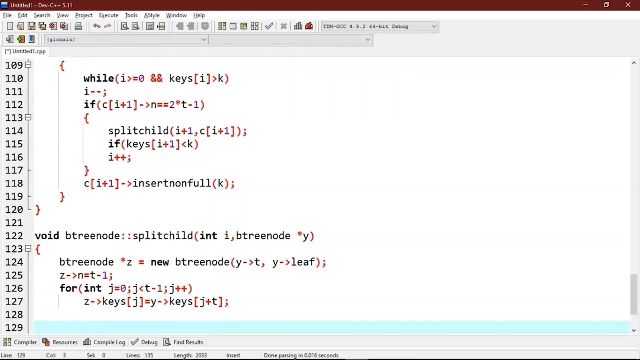 t minus one now for do and J is equal to 0, J less than T minus 1. J plus plus Z equals to a. equals to Y. equals to a, equals to. now we will copy the last T childrens of Y to Z if Y leaf. 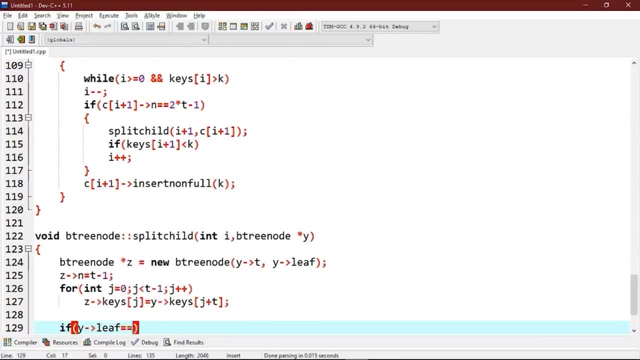 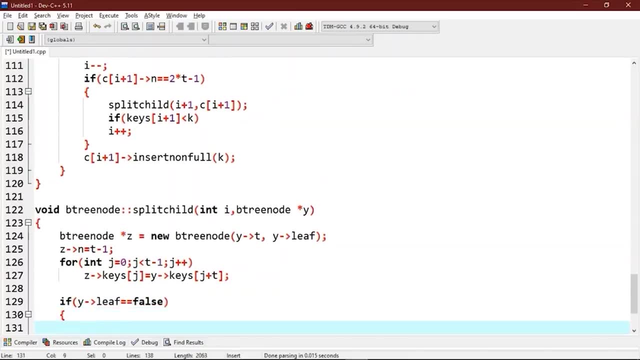 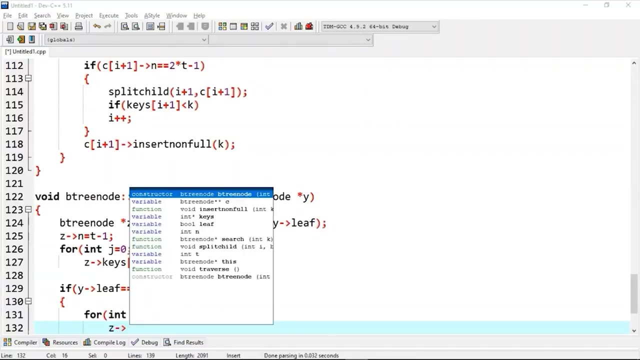 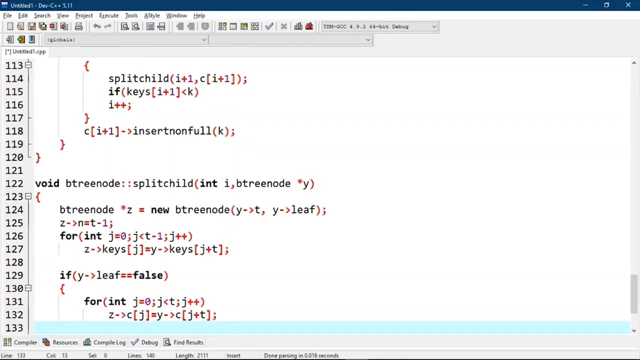 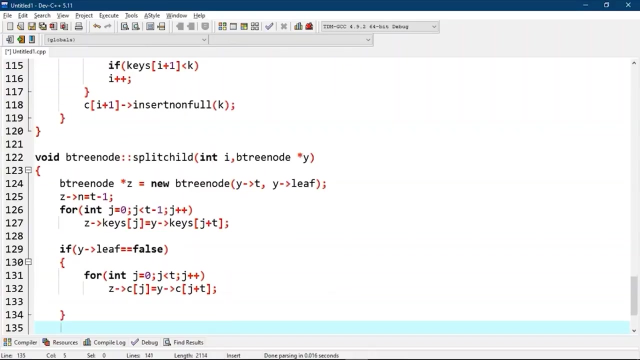 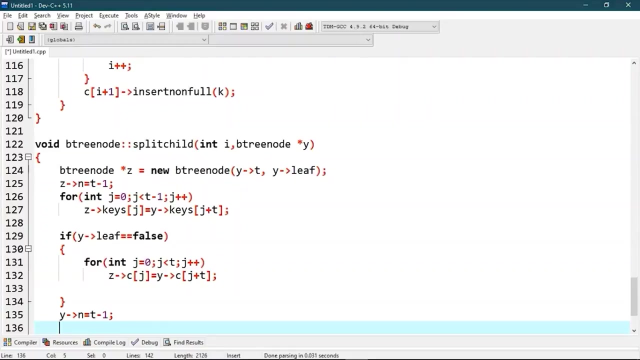 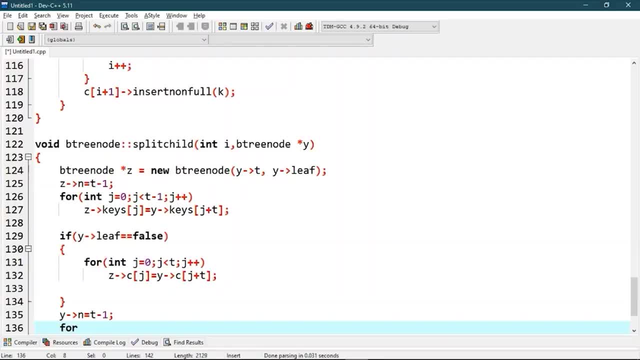 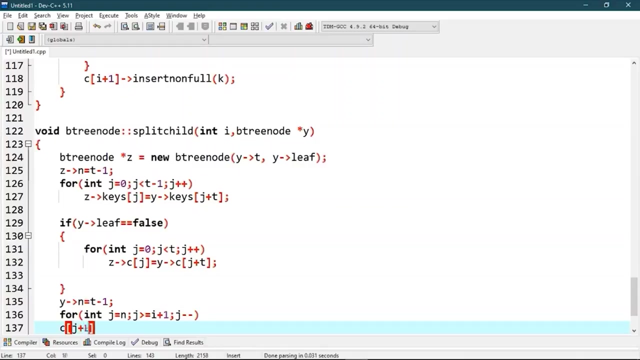 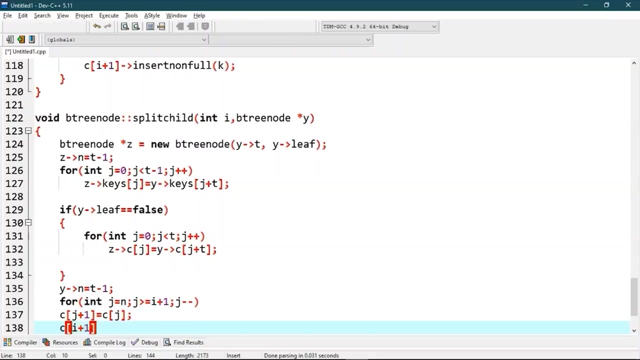 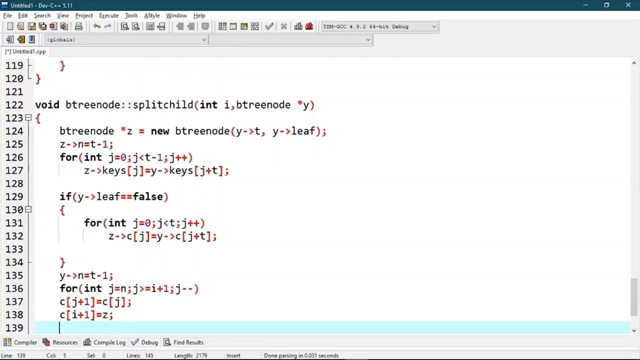 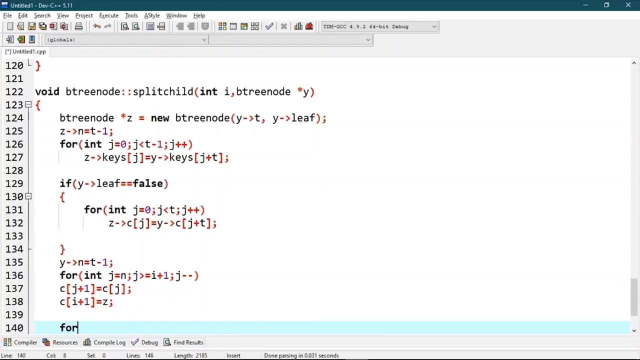 for Network: int j Tran j12 jullen j聖 j' jn 0 0 0 0. Now we will link the new child to this node. Now a key of y will move to this node and find the location of new key and move all. 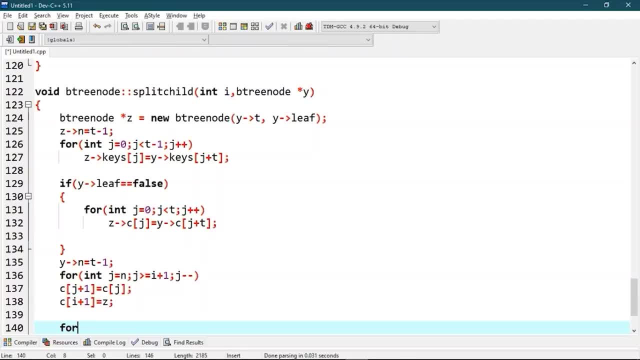 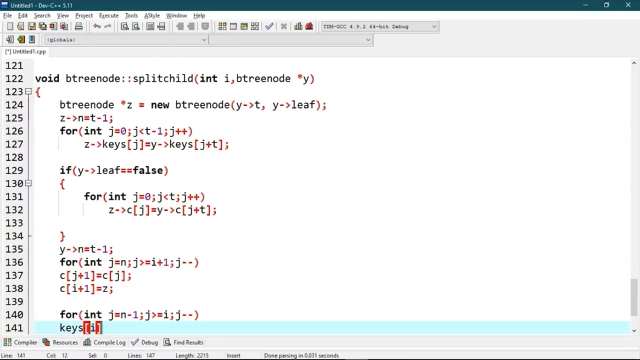 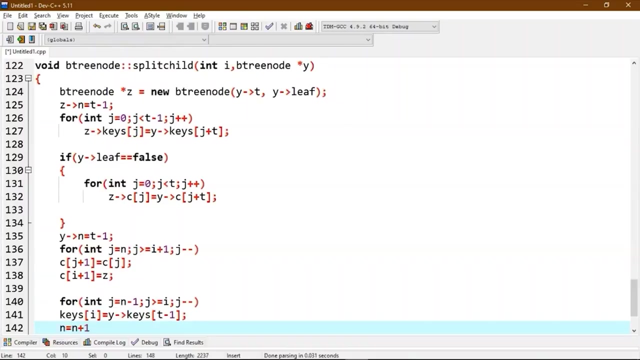 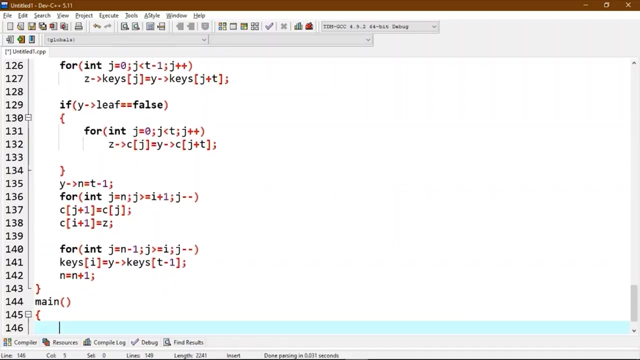 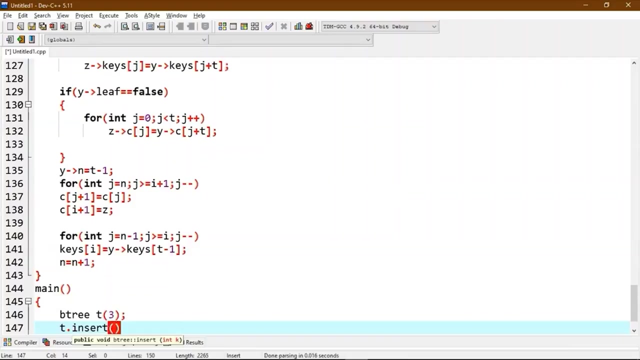 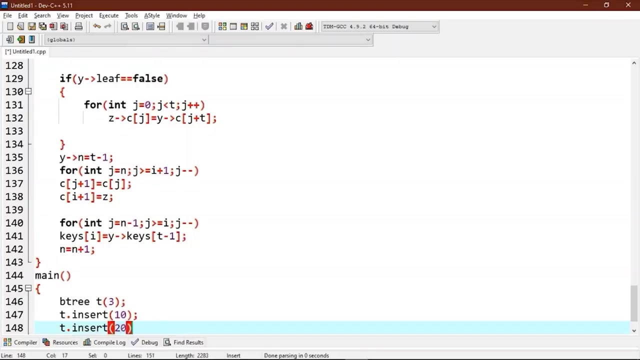 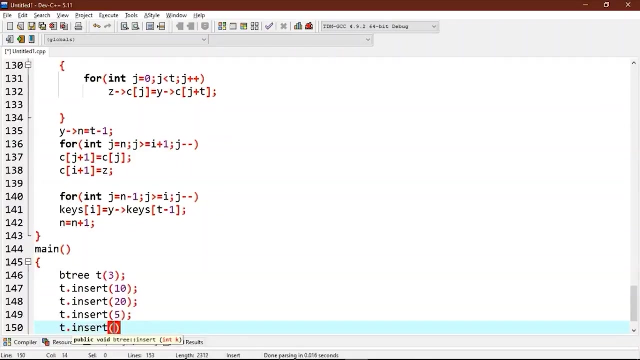 greater keys one space ahead. Now we will increment the count of keys in this node. Now let's write the main block. We will define a b tree with minimum degree 3.. Now t dot insert 10,. t dot insert 20,. t dot insert 5,. t dot insert 6,, 7,, 8,, 9,, 10,, 11,, 12,, 13,, 14,, 15,. 16,, 17,, 18,, 22,, 23,, 24,, 25,, 26,, 27,, 28,, 59,, 31,, 32,, 32,, 33,, 32,, 33,, 4,, 34,. 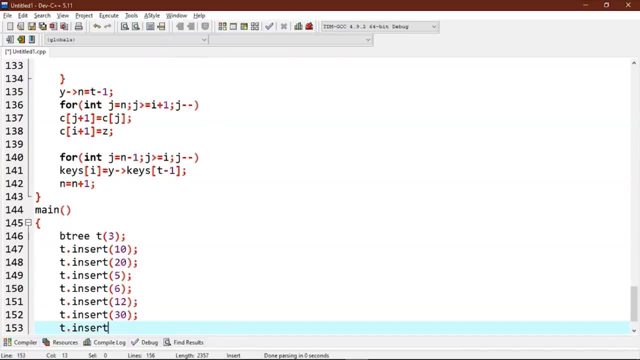 15. 24. 20. T dot insert 12, t dot insert 30. T dot insert 7. and t dot insert trade 17. now let's try to traverse this cout traversal of p3 and t dot traversal. 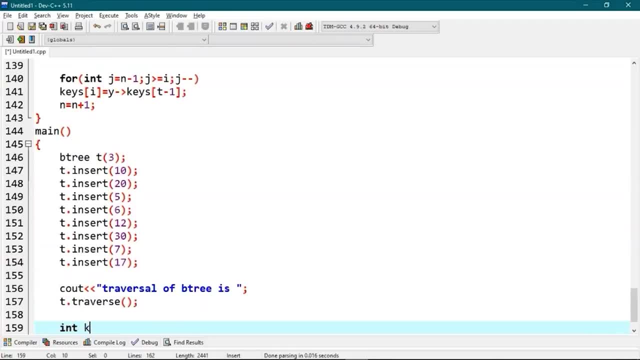 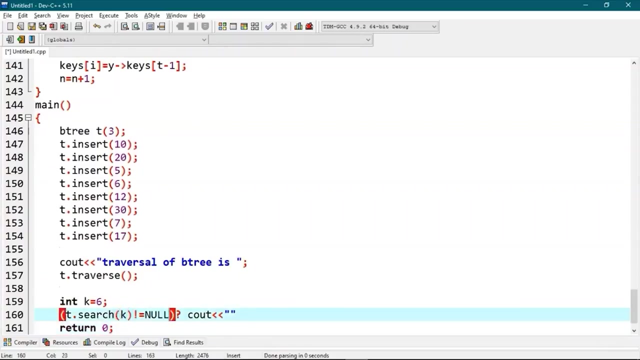 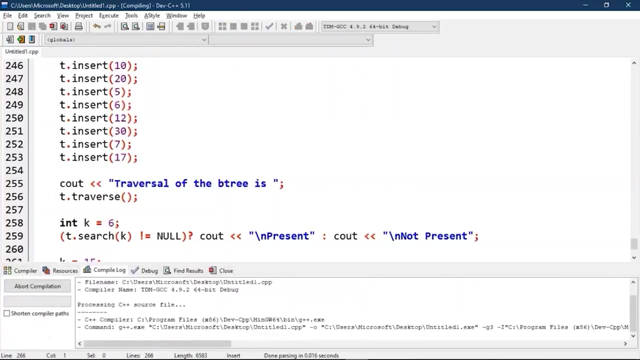 now let's search some keys. so let's state: int k is equals to 6. so if t dot search k is not null, then cout, else cout not present, not present. let's try this function one more time with k is equals to 15. let's execute this: 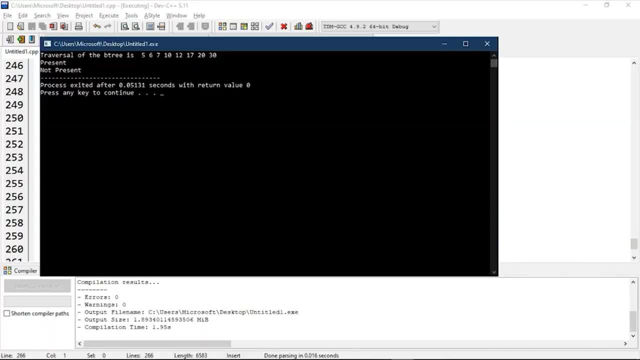 as you can see, we have successfully traversed this b-tray and we have checked two keys if they are present or not. the k is equals to 15 was not present and k is equals to 6 was present. let's get back to our slides. 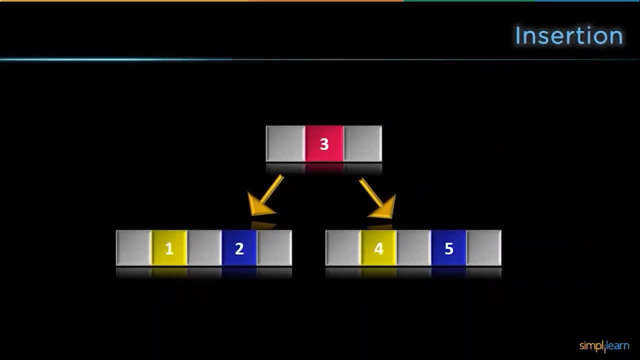 next up, insertion. we have to insert an element in such a way so that we won't disobey any properties of b-trays. now let's try this operation in a code editor. we will start by creating a node. to do that, we need to create a node and we need to create. 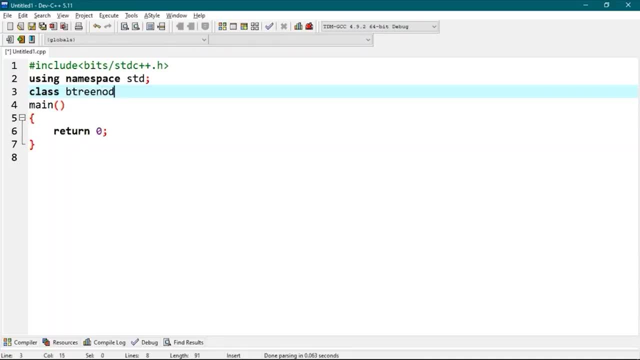 a class. for that we will use class b-tree node. then we will create an array of keys- minimum degree- an array of child pointers and a key- current number of keys- and a boolean variable- leaf. This variable will tell if that node is leaf or not. 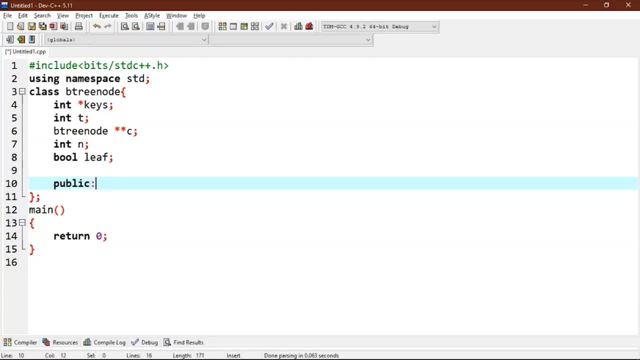 Then we will define some public functions. We will start with constructor. Now we will create a function to insert a new key into the non-full node, A utility function to split the child, A function to traverse the tree, A friend class, btree. 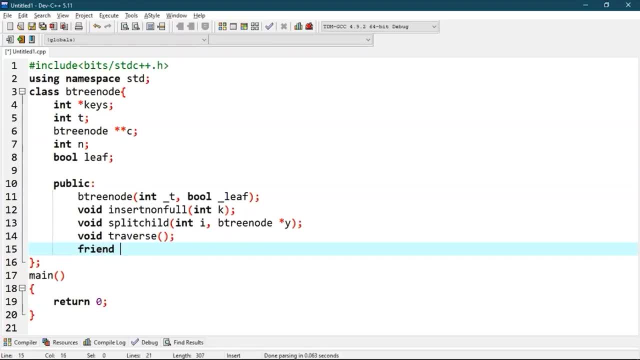 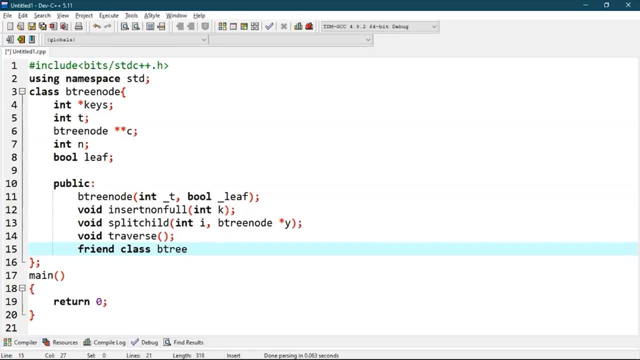 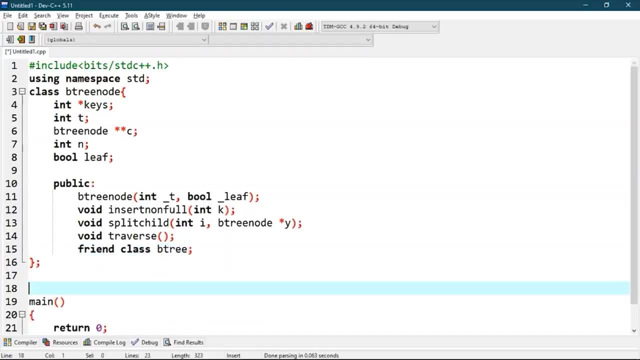 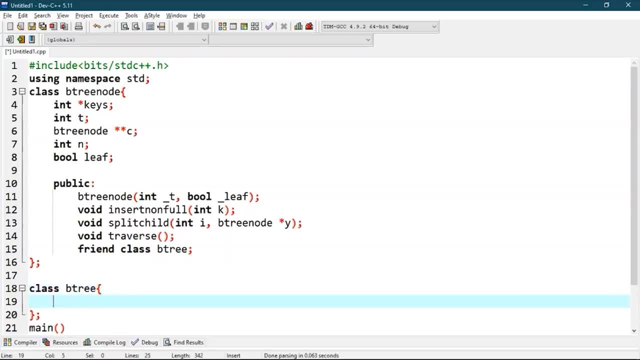 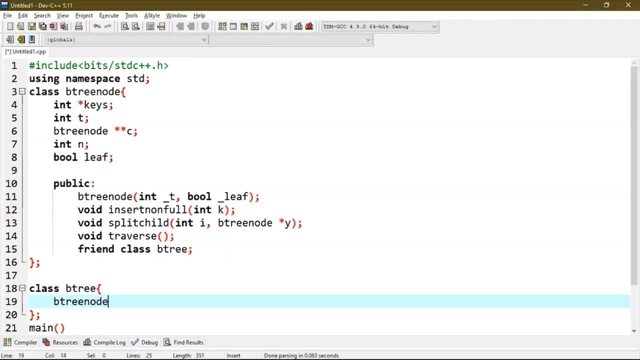 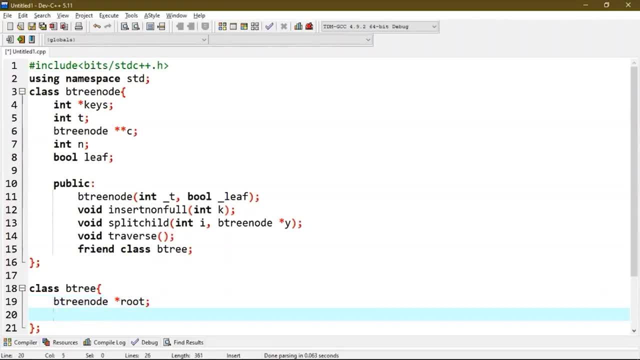 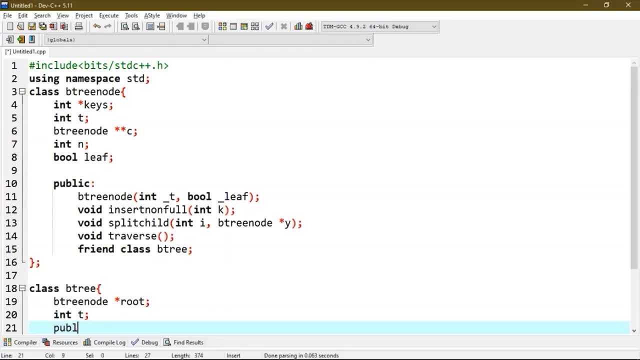 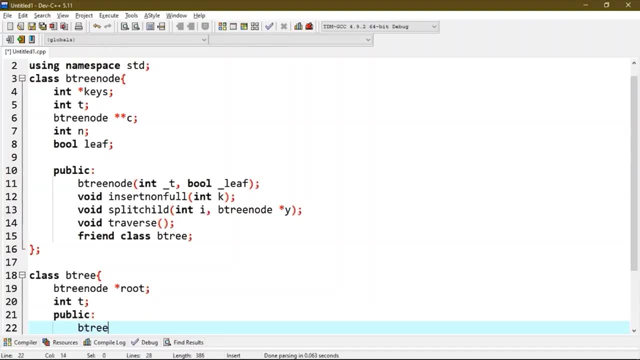 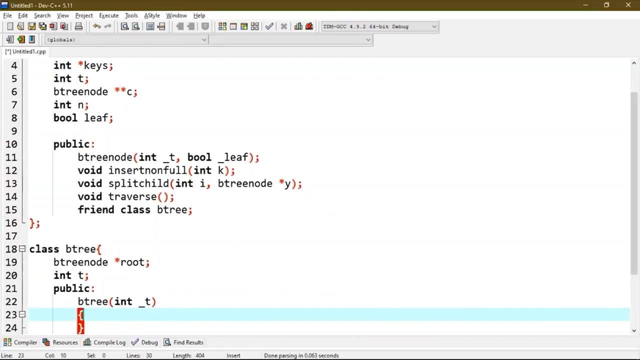 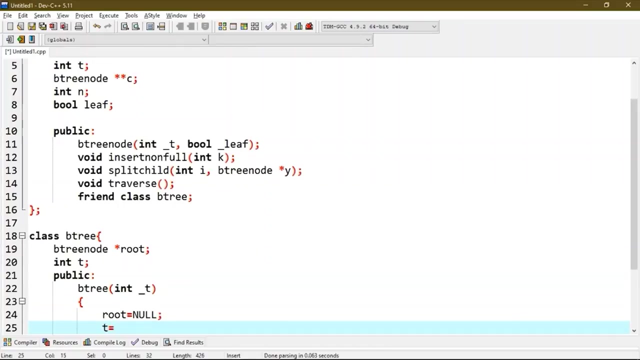 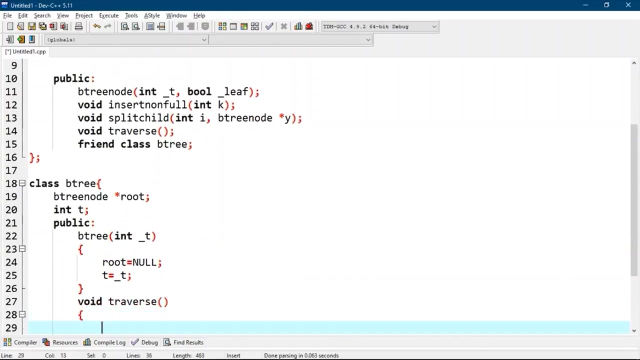 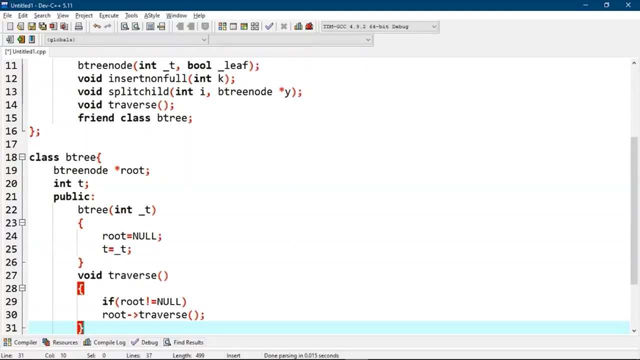 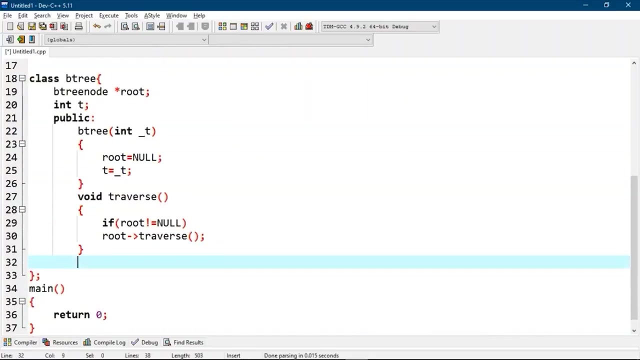 A function to cross the tree. A function to cross the tree. A function to cross the tree, public functions. first, constructor: root equals to null and T equals to underscore. T now void traverse. now, if root is not equal to null, then root arrow traverse. now we will define a main function that 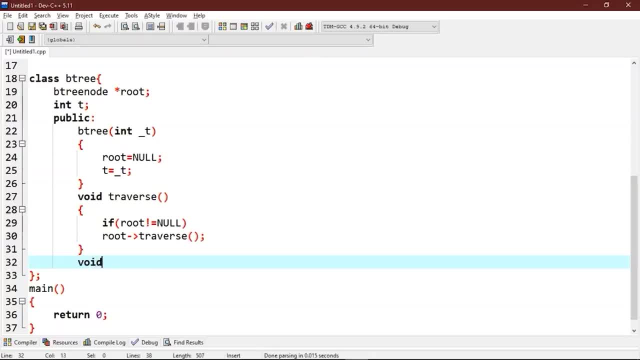 inserts a new key in this B tree. now we will write the constructor for the B tree dot class class. now we will write the constructor for the B tree dot class. and T 1 comma boolean leaf 1. and T 1 comma boolean leaf 1. 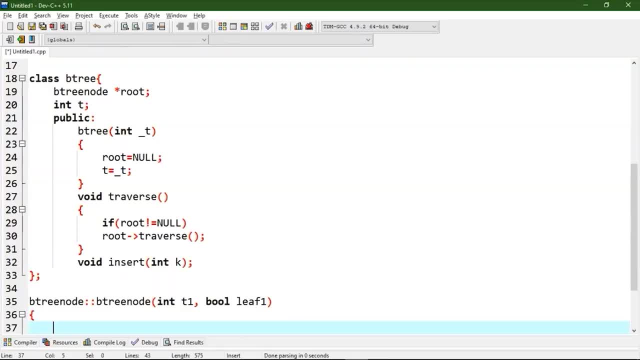 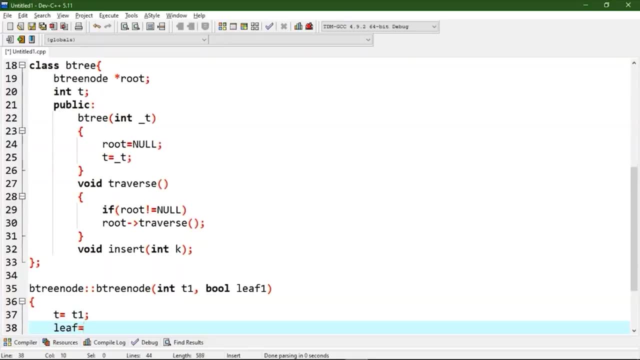 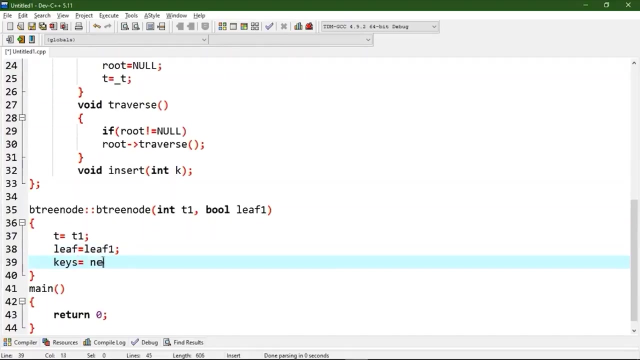 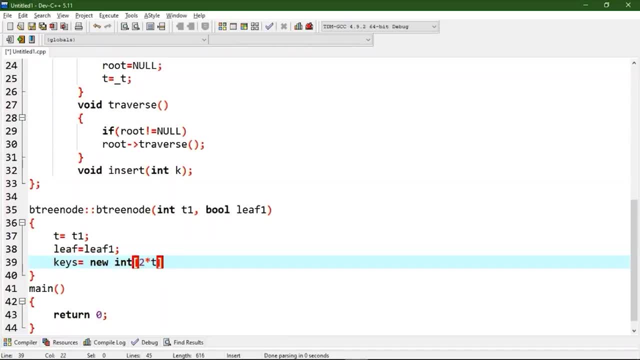 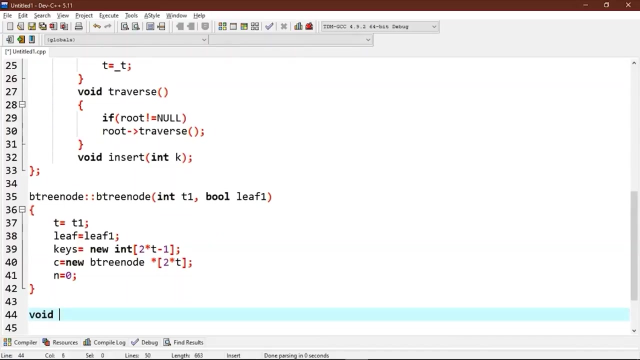 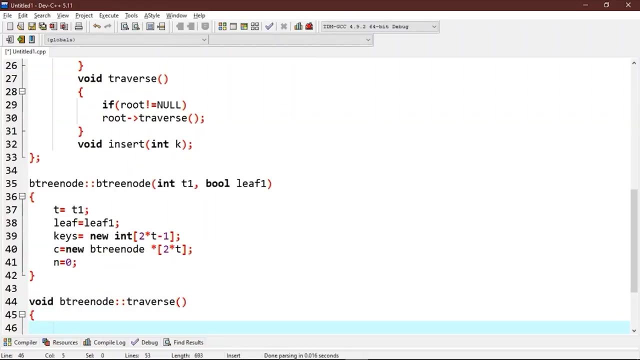 now we will allocate memory of maximum number of possible keys and child pointers. Now we will initialize the number of keys as 0.. Now let's write a function to traverse all nodes in the subtree. Now there are n keys and n plus 1 children. 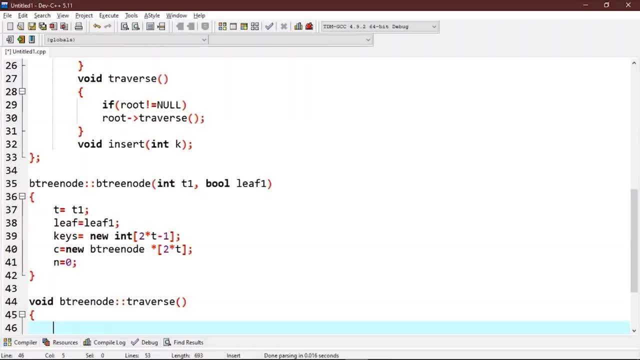 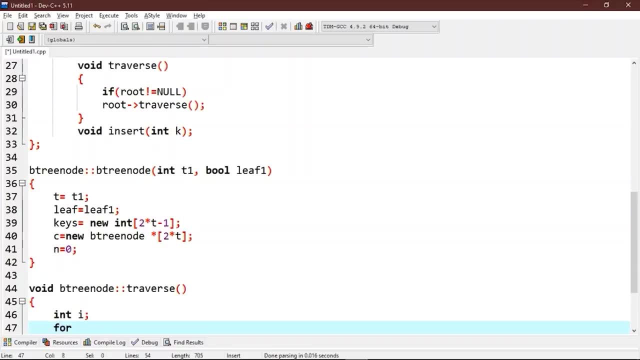 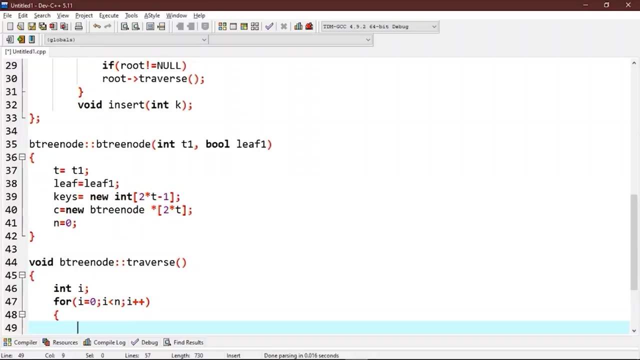 So we will traverse through n keys and first n children. So int i for loop, i is equal to 0, i less than n and i plus plus. Now suppose if this is not leaf, then before printing key we will traverse the subtree rooted with this child. 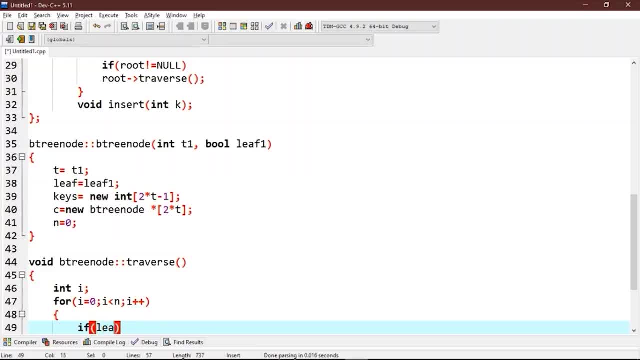 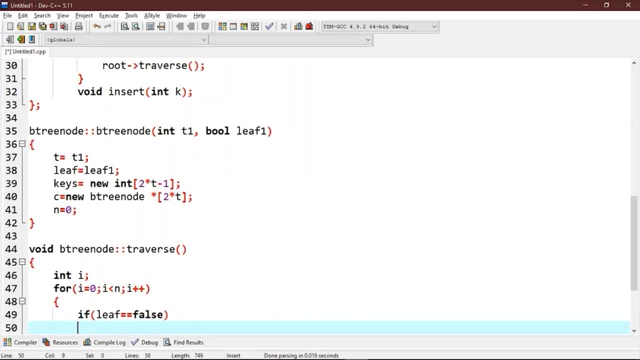 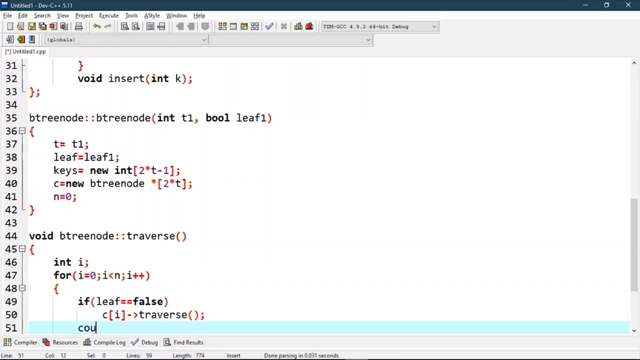 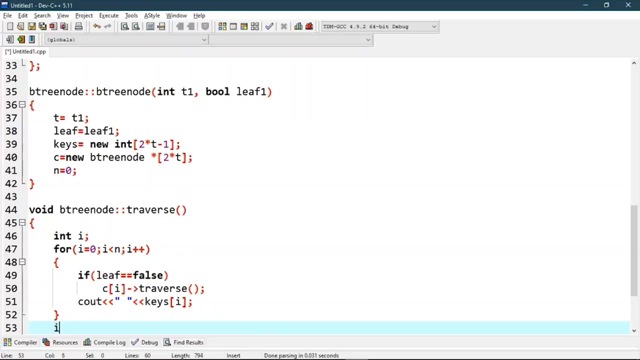 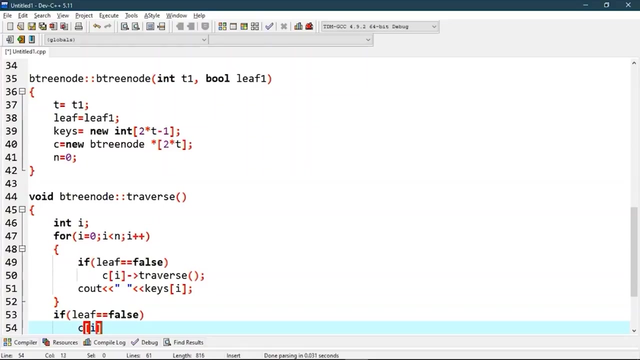 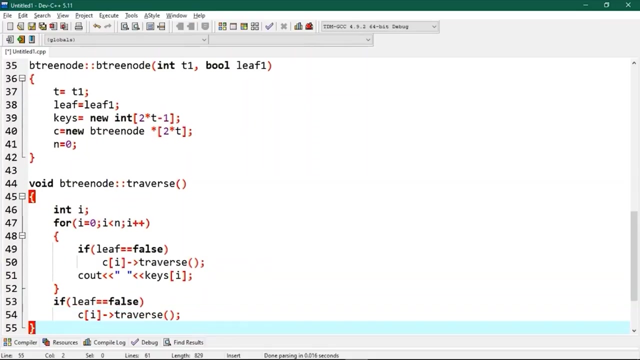 So if leaf is equals to false, Then see i arrow traverse. Now we will print these keys. Now we will print the subtree rooted with the last child. So if leaf is equals to false, Then see i arrow traverse. Then see i arrow traverse. 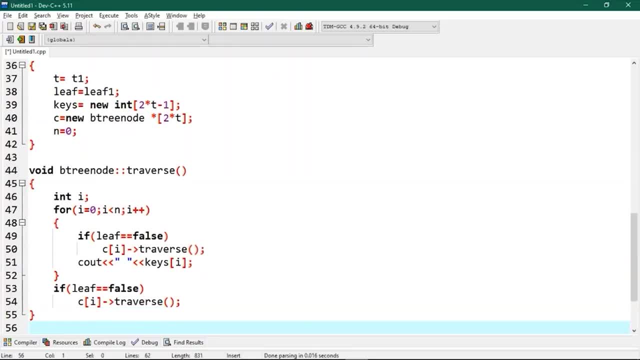 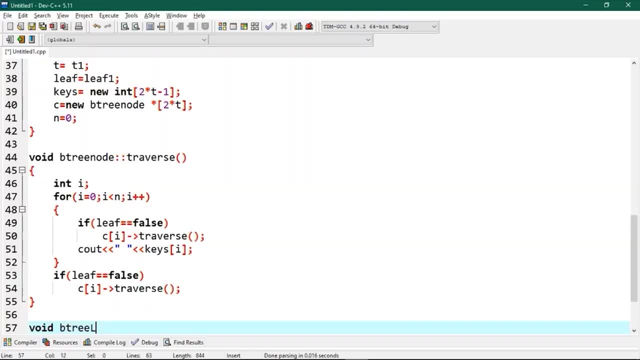 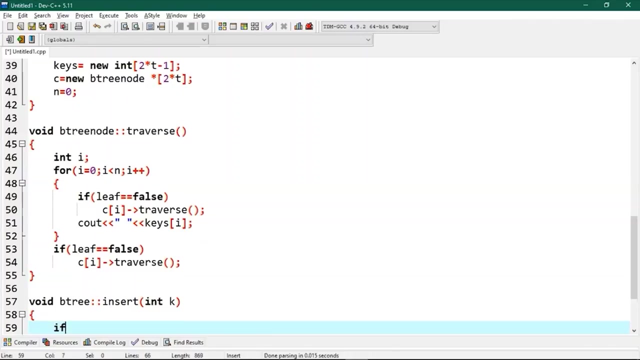 Now we will write the main function that inserts a new key in this btree. Now we will write the main function that inserts a new key in this btree Now. if btree is empty, Then we will allocate the memory to root. So root is equals to new. 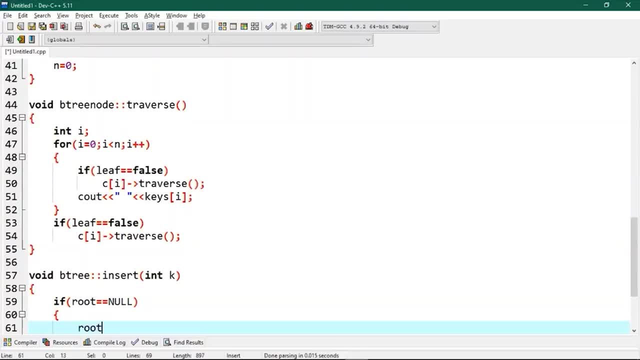 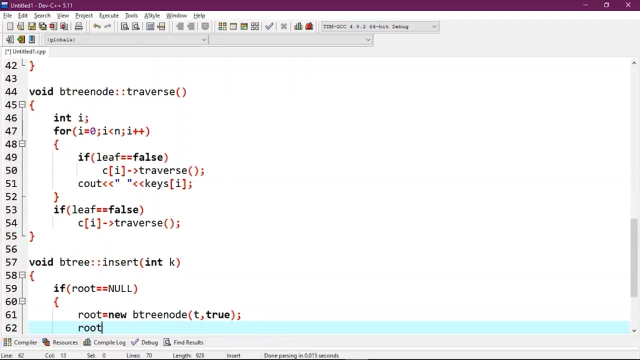 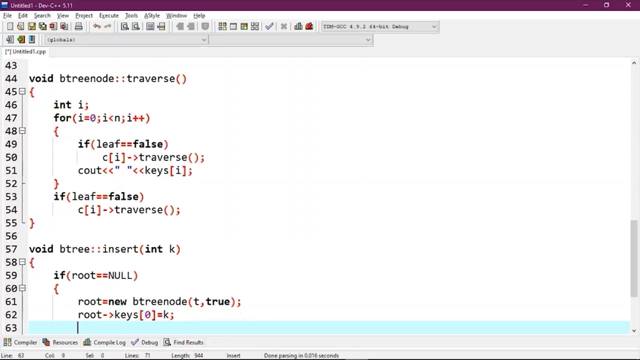 And we will add the memory to root. Now we will find the number. So we will add the memory to root. btray node key comma: true. now we will insert the key root arrow keys equals to k and we will update the number of keys in root. 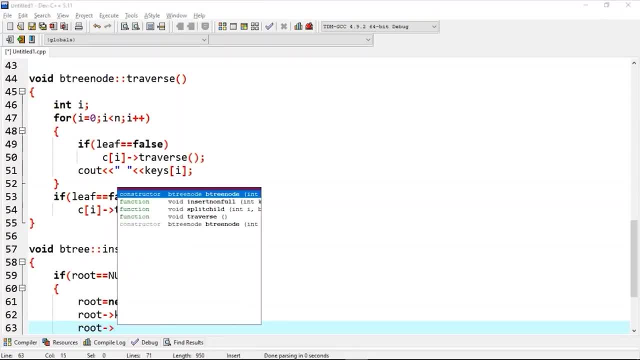 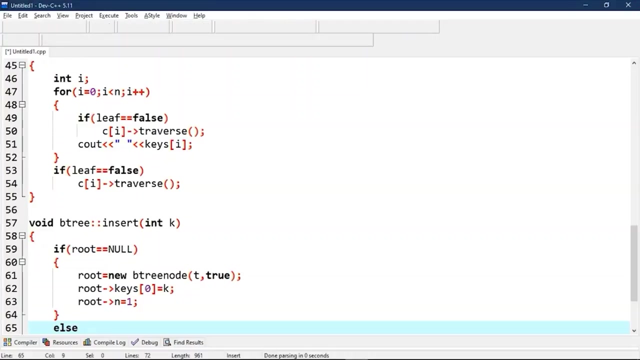 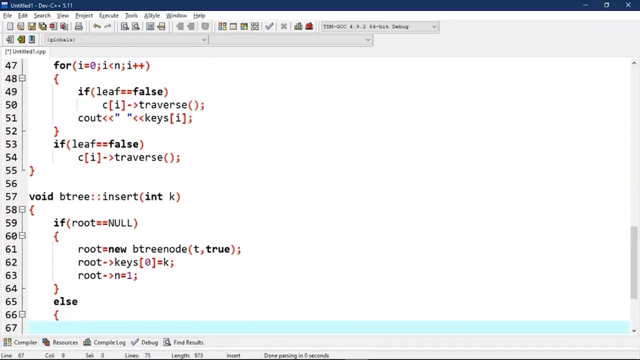 so root arrow n equals to 1 and we will update the number of keys in root. and we will update the number of keys in root. else, if tree is not empty and if root is full, then tree will grow in height. if root arrow n is equals to: 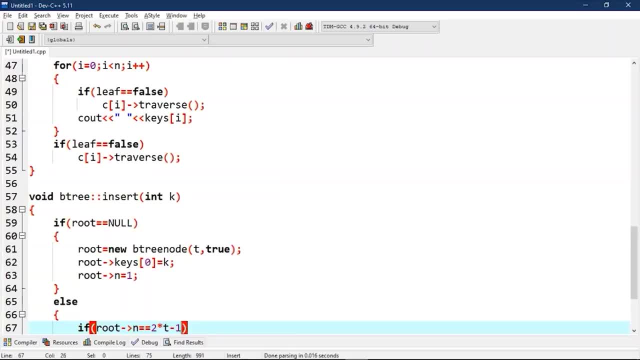 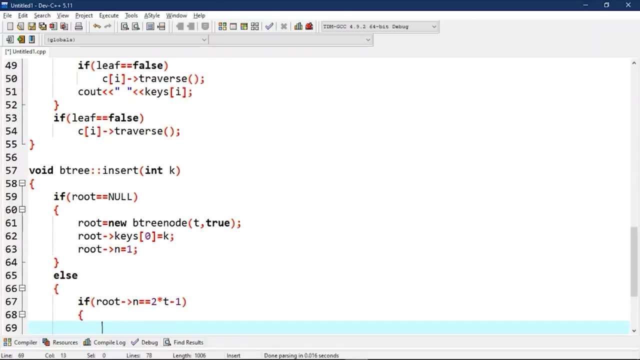 2 star t minus 1 and we will update the number of keys in root. and we will update the number of keys in root. and we will update the number of keys in root. now we will allocate the memory of new root. now we will allocate the memory of new root. 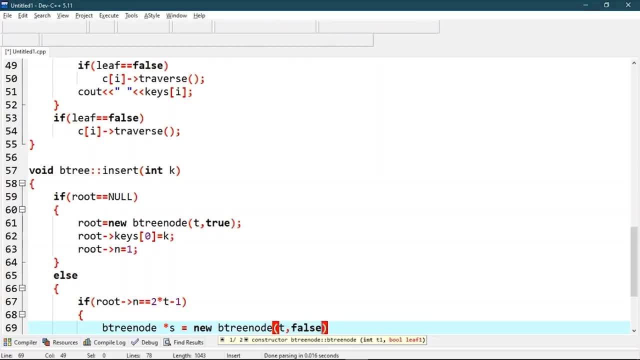 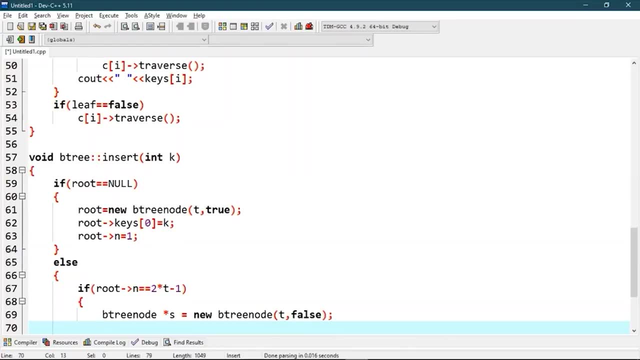 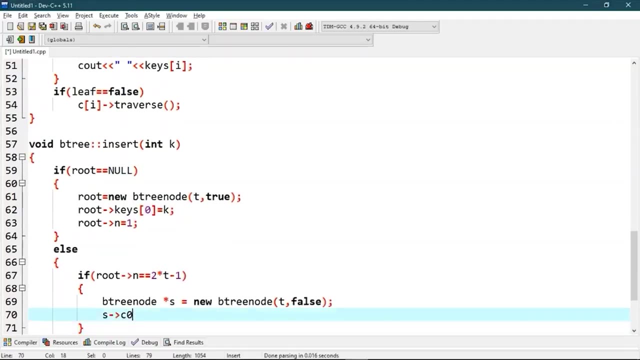 now we will allocate the memory of new root. now we will make old root as child of new root. now we will make old root as child of new root equals to root. root equals to root. Now we will split the old root and move one key to the new root. 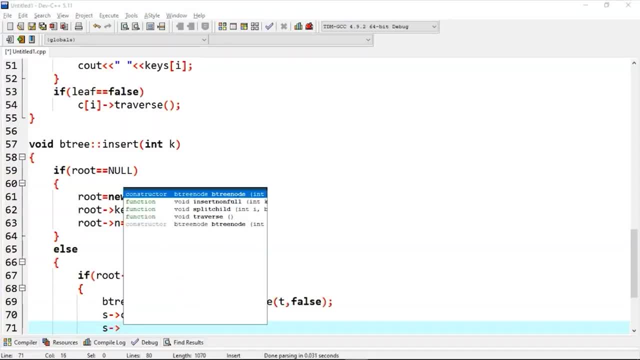 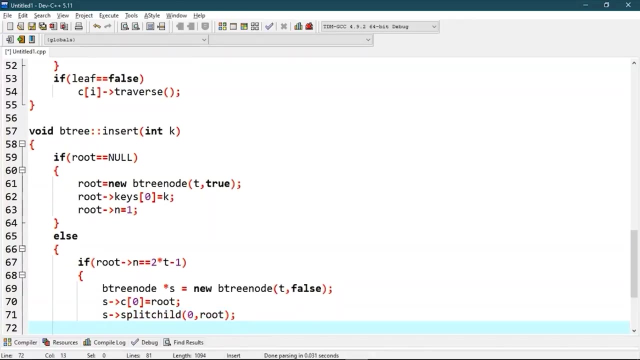 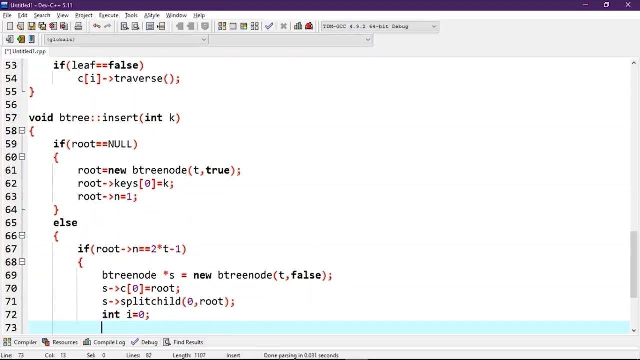 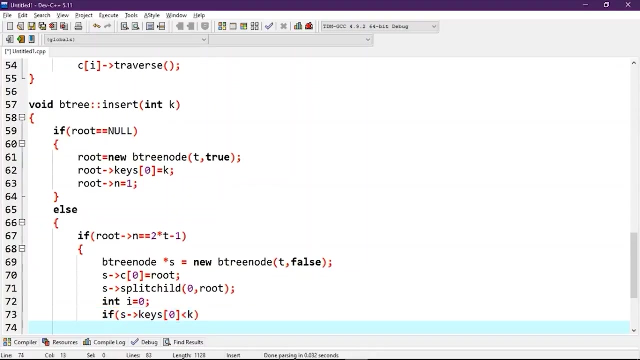 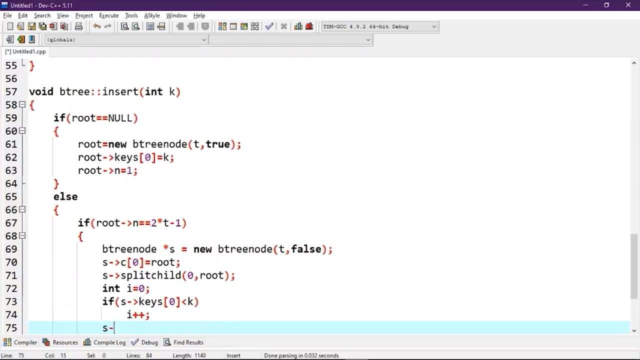 So to do that we will use split child function: 0 comma root. Now new root has two childrens. now We have to decide which of the two children is going to have new key. So to do that we will use int. i is equal to 0. if s keys 0 is less than k, then i++ and s. 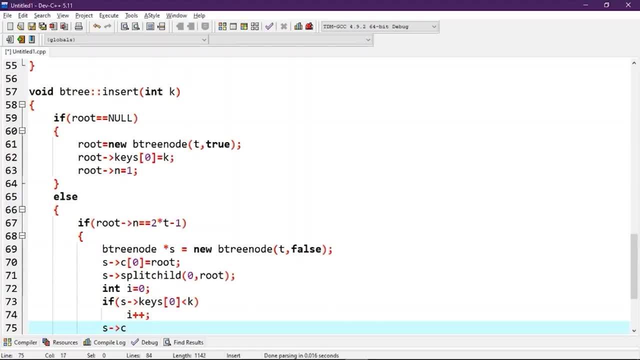 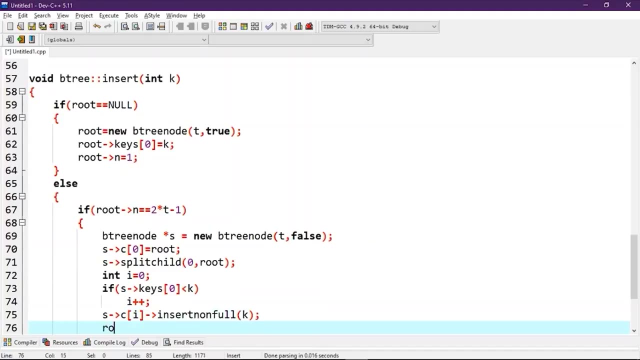 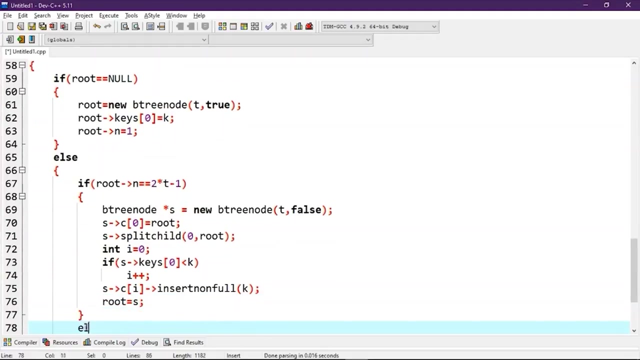 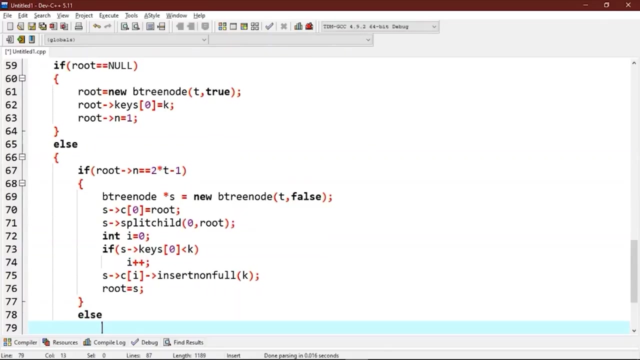 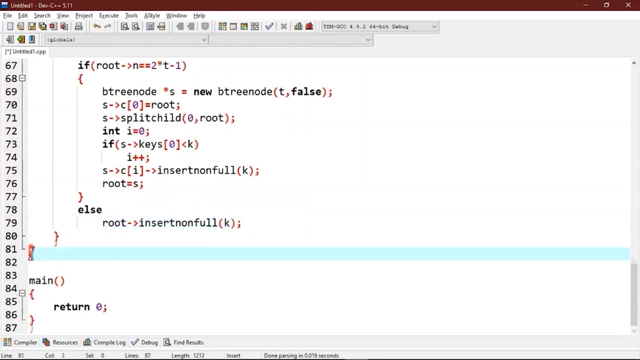 arrow c. Now we will change the root i but non full. Now we will change the root Else. Now we will write a utility function to insert a new key in this node. We will assume the node must be non-full when this function is called. 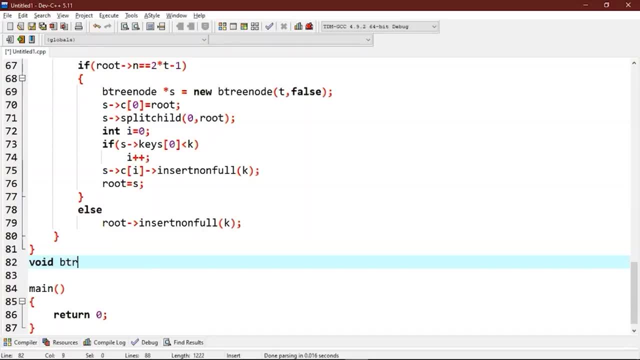 So void btreeNode. insert non-full int k. We will initialize index as index of rightmost element. So int i is equals to n-1. Now if this is a leaf node, then the following loop does two things: a- finds a location of new key to be inserted or move all greater keys to one place ahead. 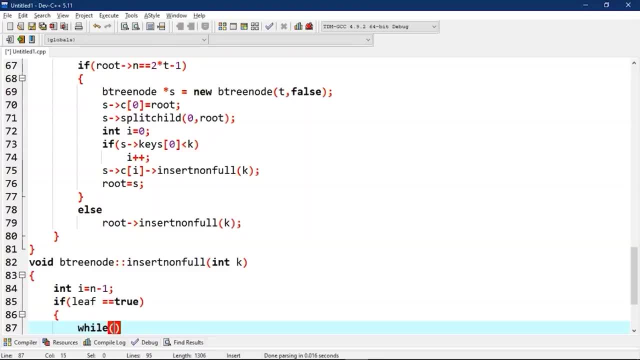 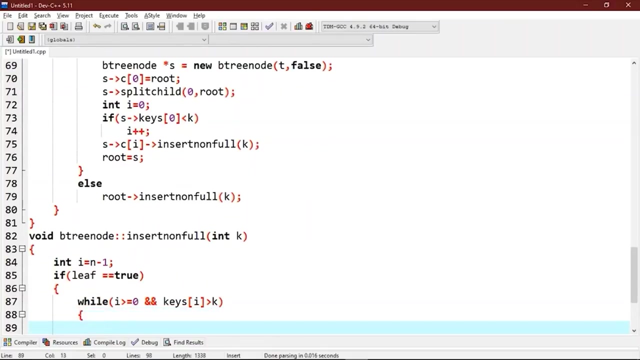 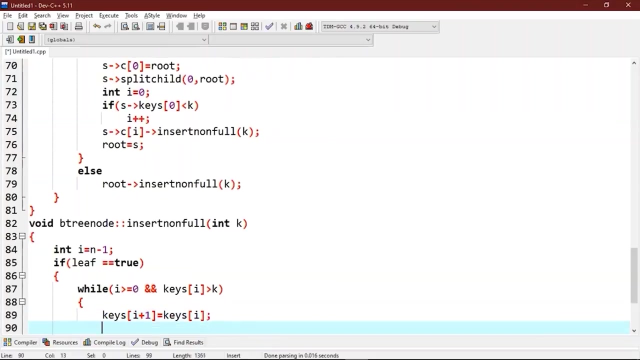 So, while i is greater than equals to zero and t is i is greater than k, Now t is i plus 1.. Now t is i plus 1.. Now t is i plus 1. will be equals to keys at i and i- 😉. 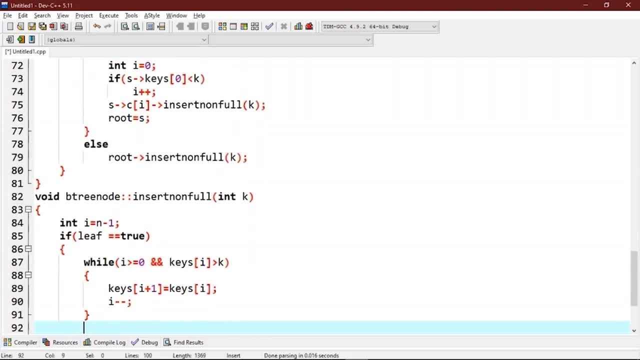 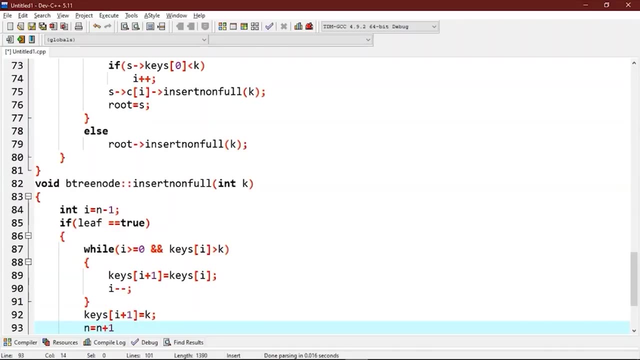 Now we will insert the new key at the found location. So keys at i x 1 will be equals to k and N equals to N x 1.. So key n1n1 will be equal to n1.. So we must insert the new key at the found location. 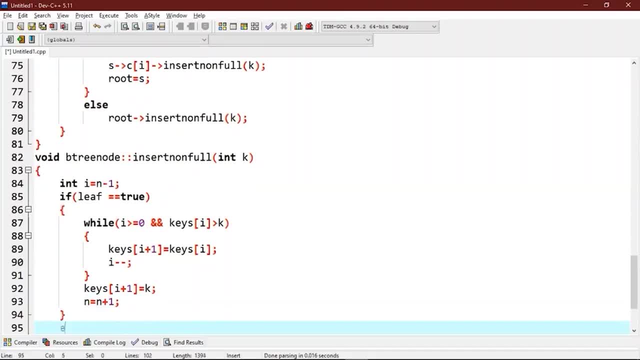 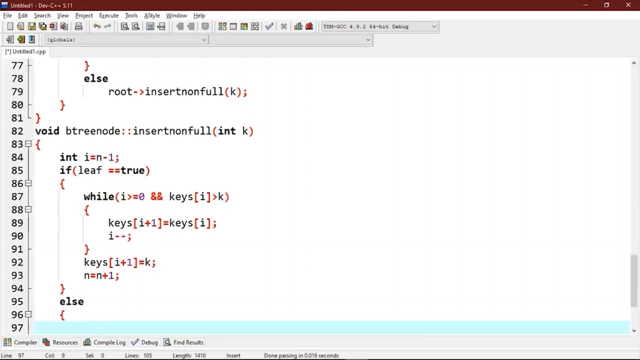 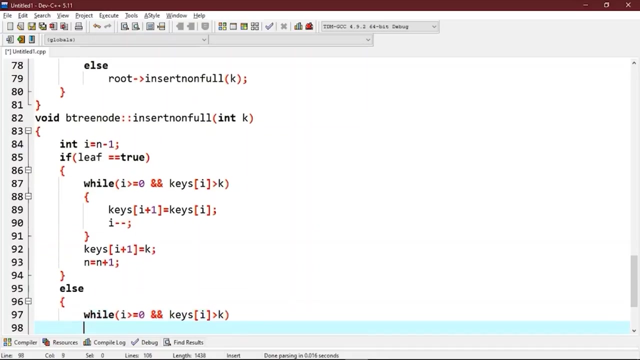 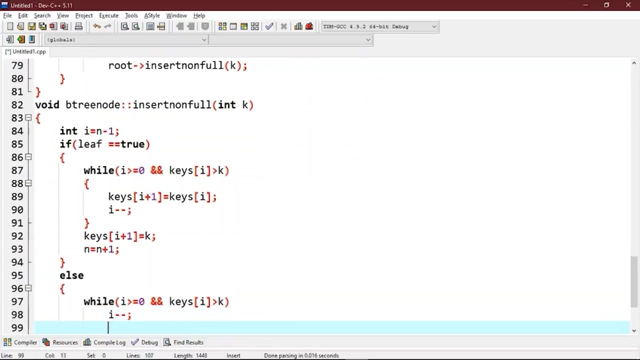 So keys at i, x, 1.. Now else, if this node is not leaf, then we will find the child which is going to have the new key. So while i is greater than equals to 0 and t is i is greater than k, then i minus minus. 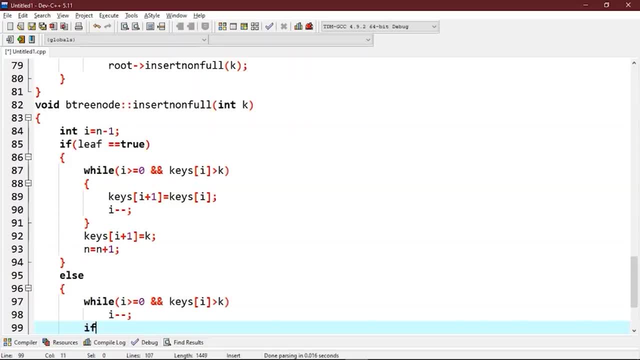 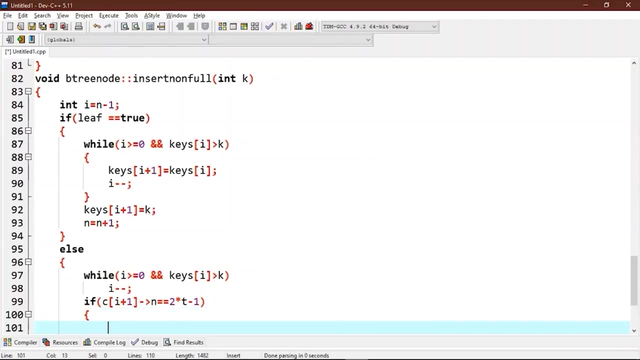 Now we will see if the found child is full. So if i is greater than c, i plus 1 arrow n is equals to 2 star t minus 1.. Now if the child is full, then we will split it. So split child at i plus 1 comma c, i plus 1.. 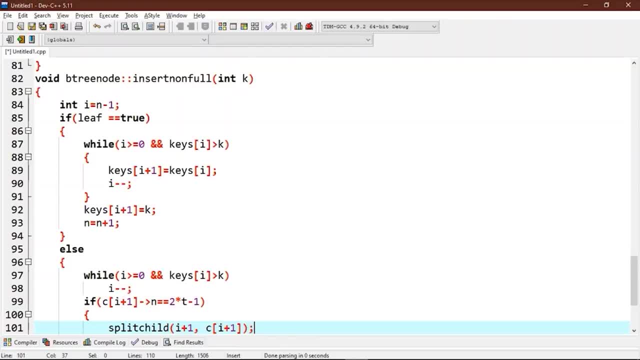 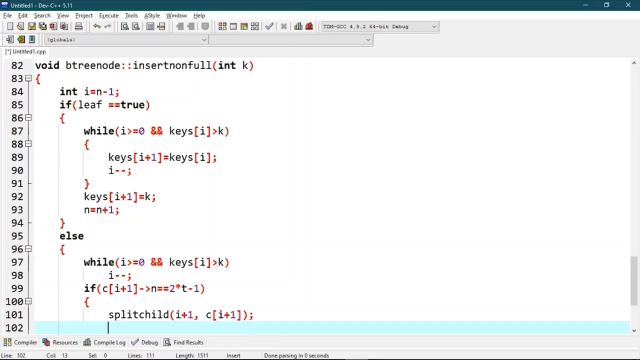 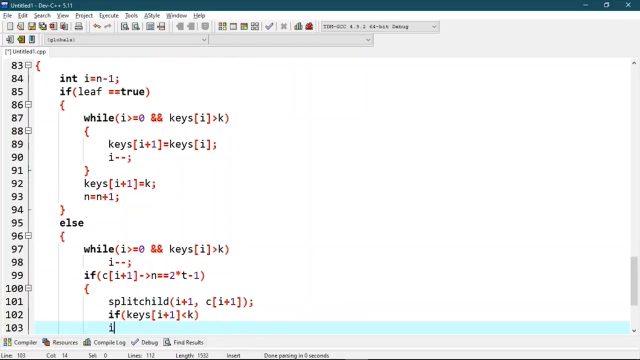 After split, the middle key of c i goes up and c i is split. Now we will see which of the following will have the new key. F key is: i plus 1. is less than k than i plus plus c. i plus 1, insert non-full k. 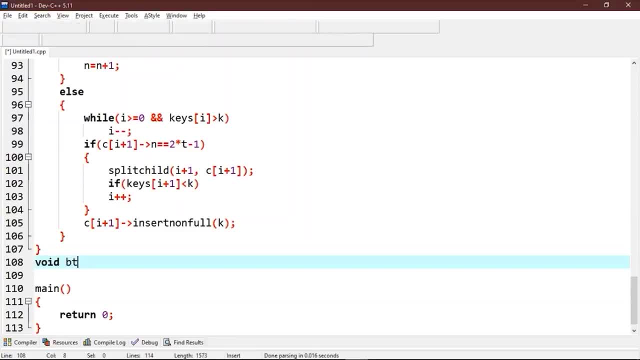 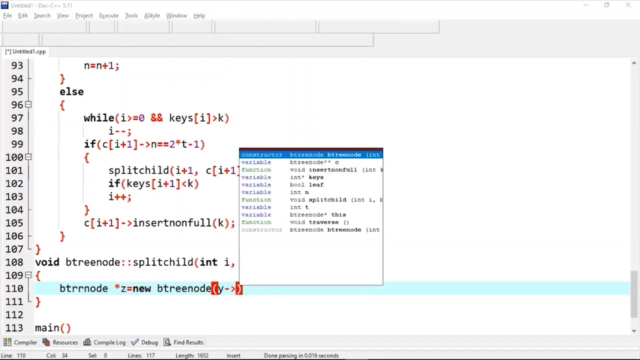 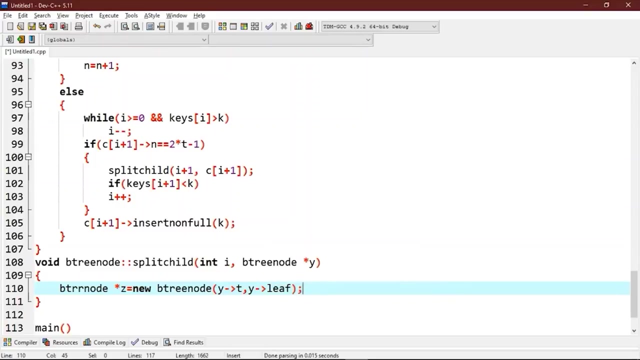 child end i a tree node. now we will create a new node which is going to store T minus keys of Y. so btree node star z equals to new btree node y arrow, t comma, y arrow leaf. now z arrow n is equals to t minus one. 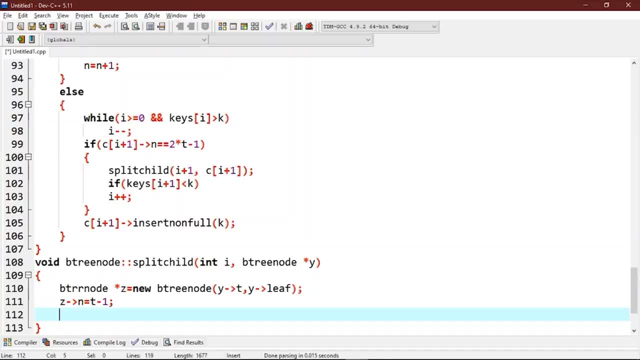 now we will copy the last t minus one keys of y to z. so for loop. now we will copy the last t minus one keys of y to z. so for loop. now we will copy the last t minus one keys of y to z. now we will copy the last t minus one keys of y to z. 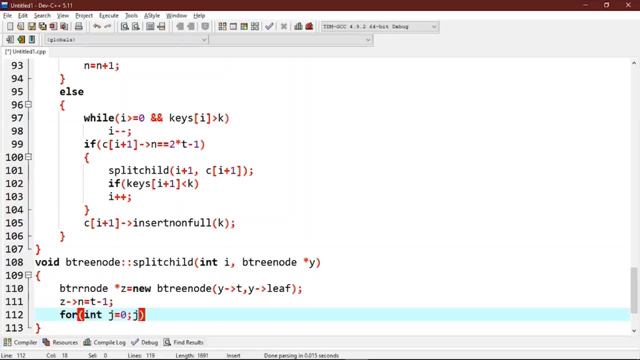 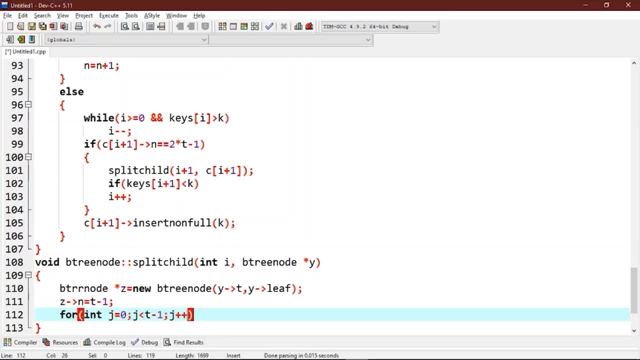 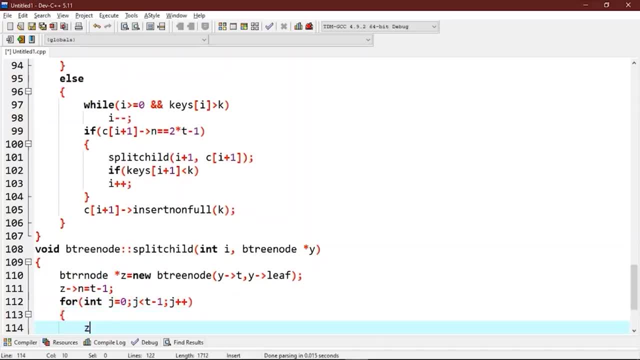 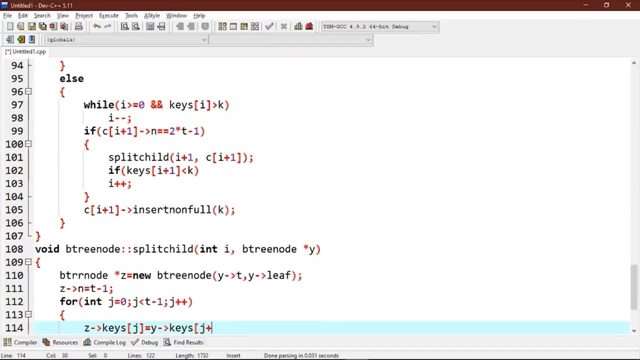 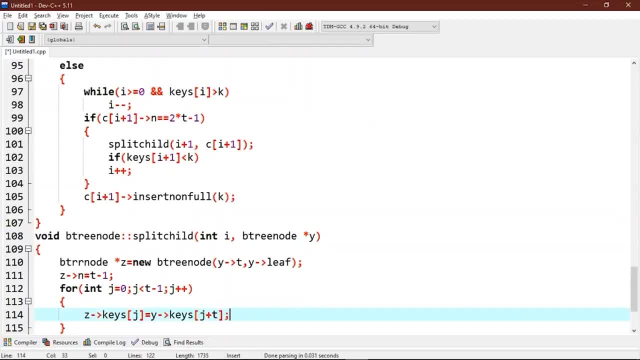 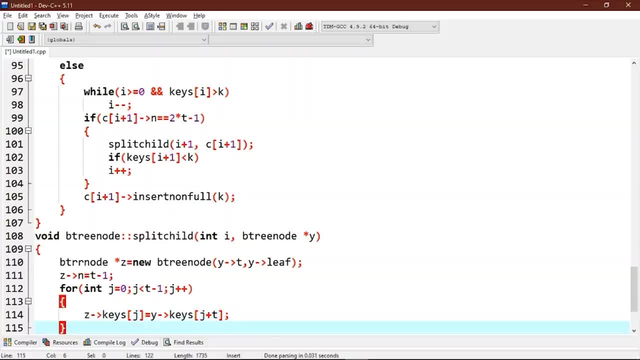 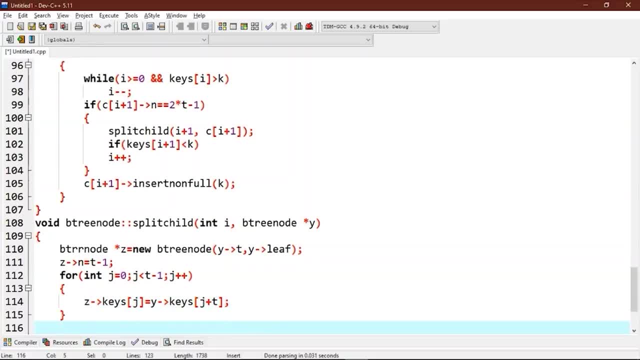 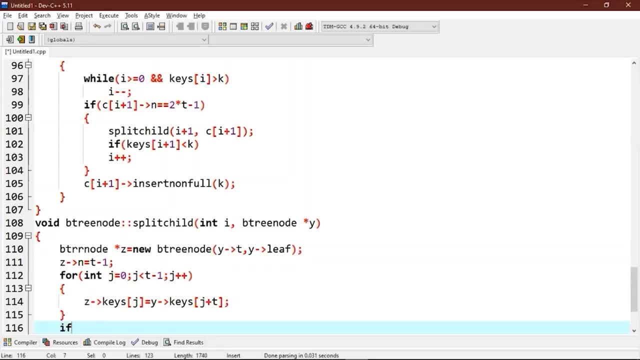 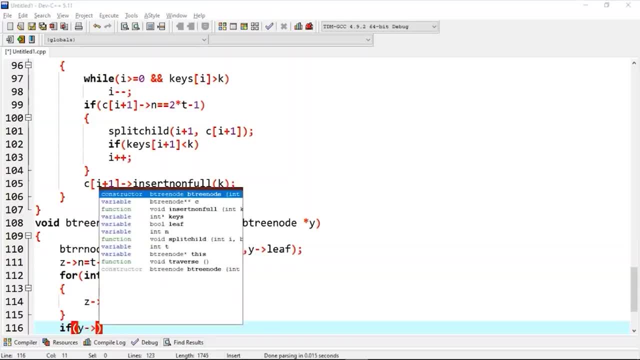 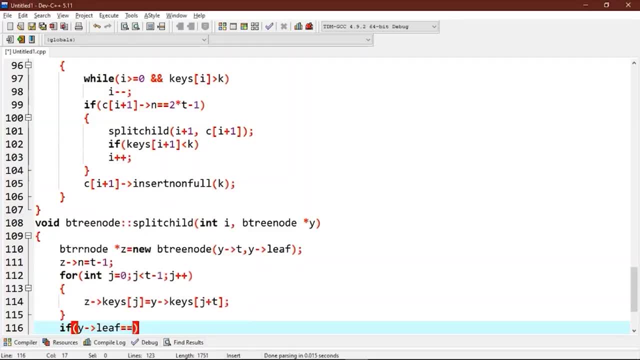 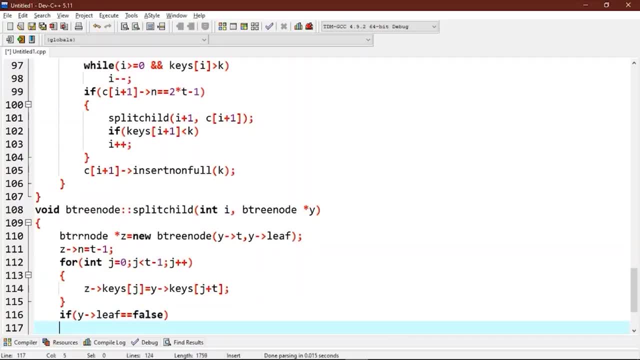 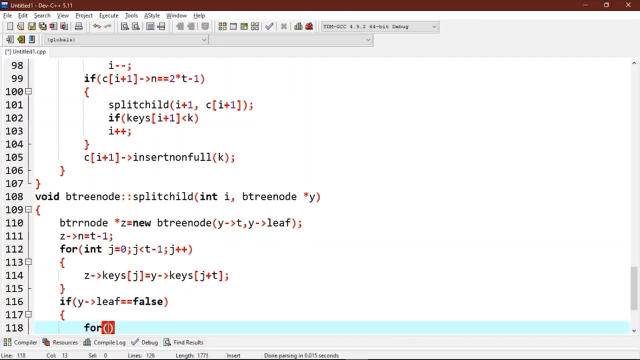 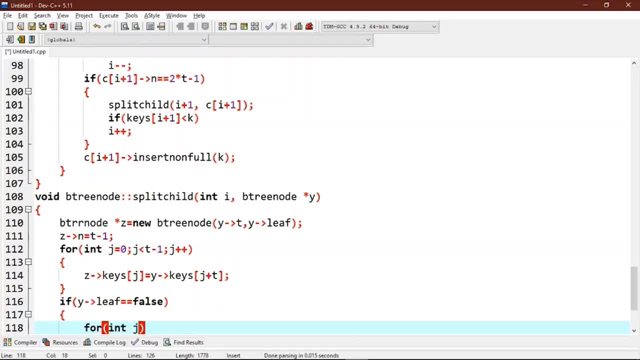 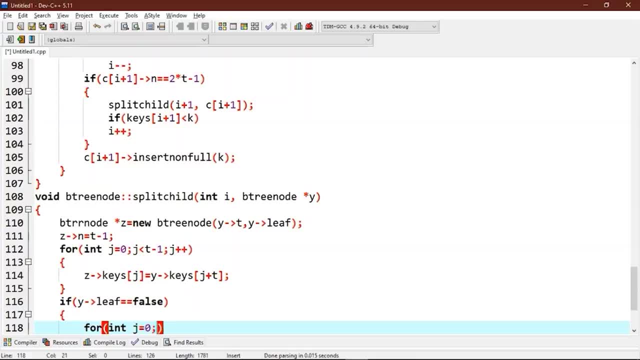 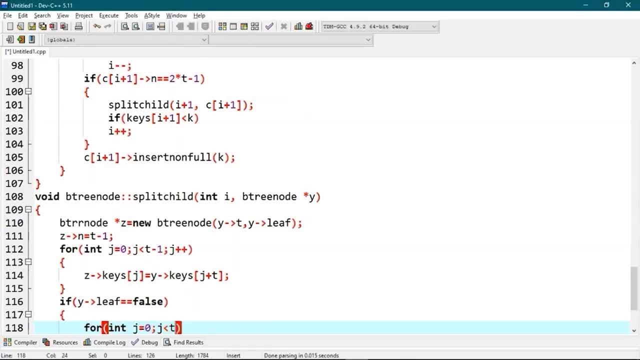 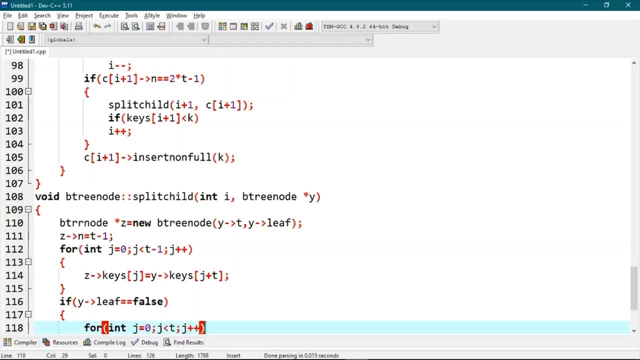 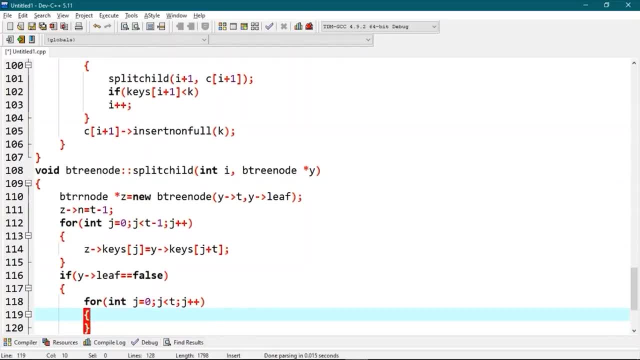 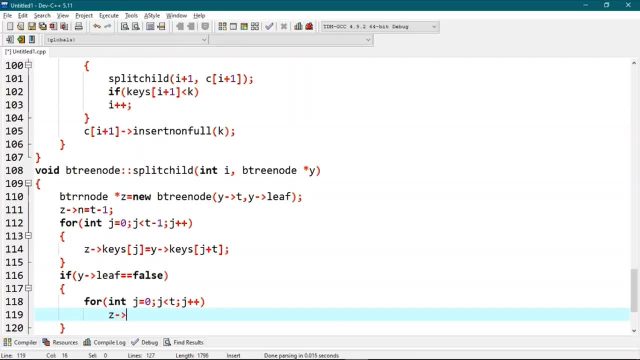 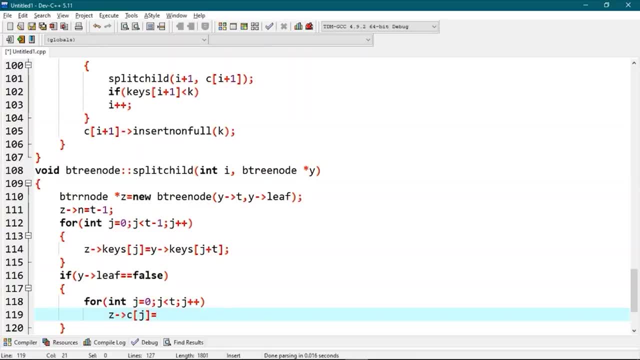 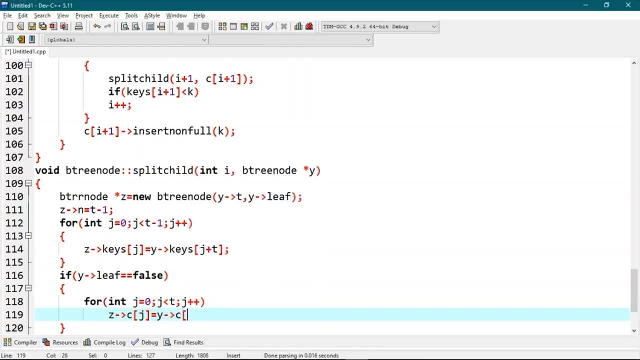 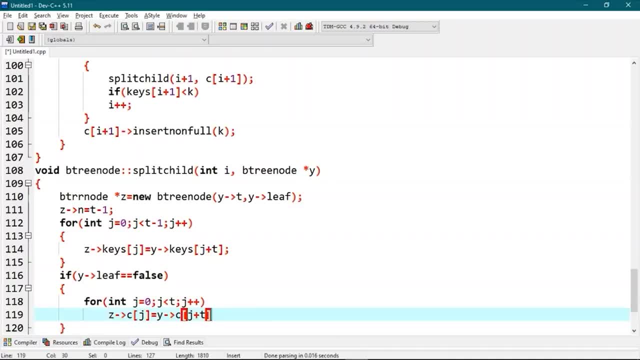 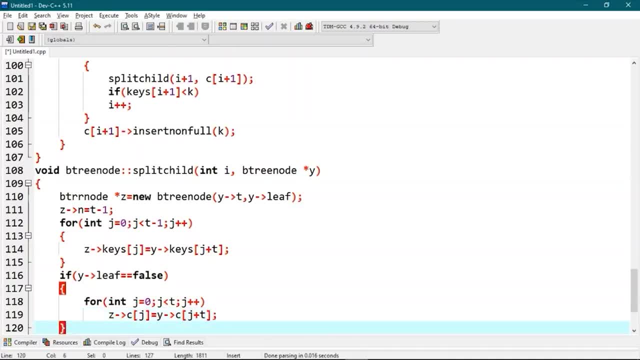 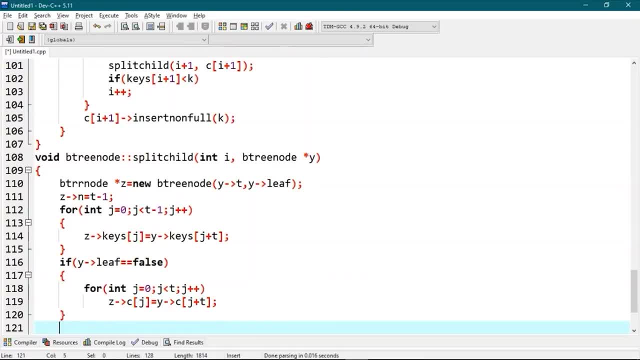 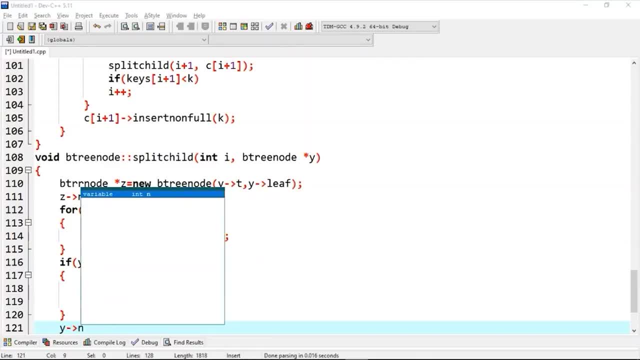 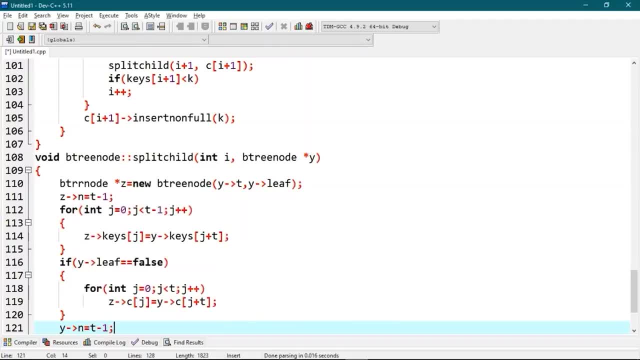 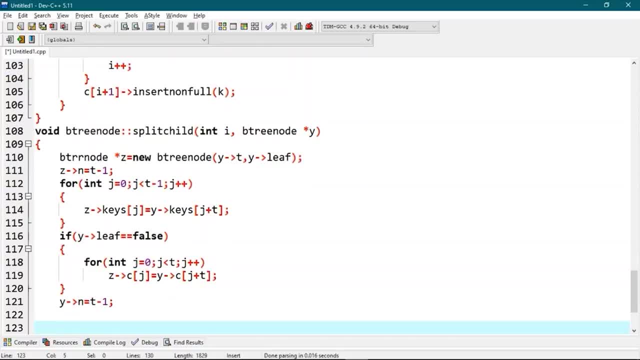 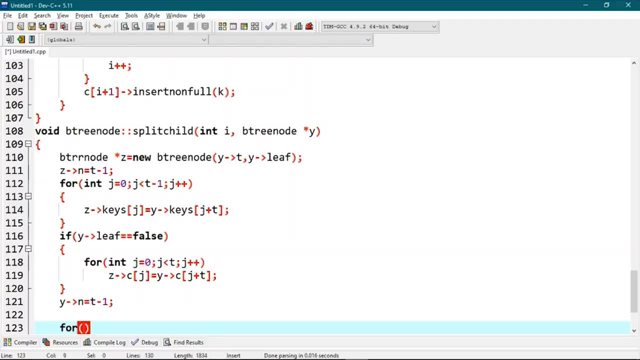 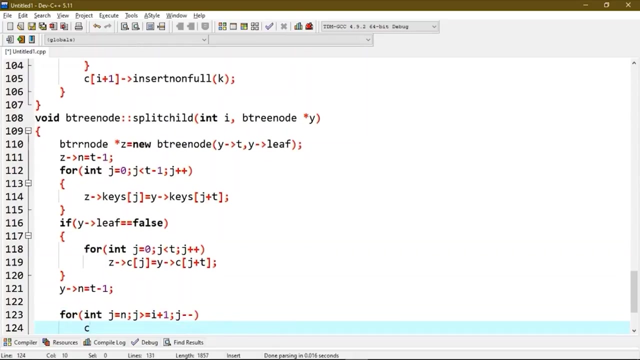 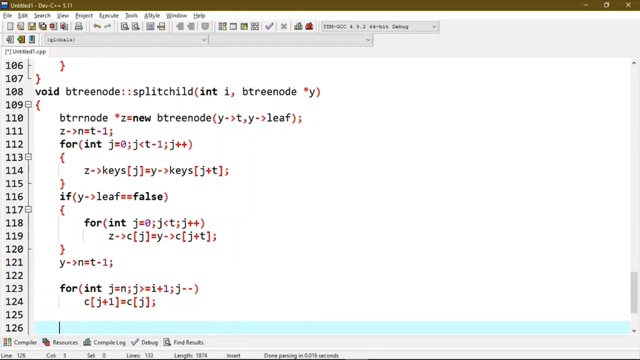 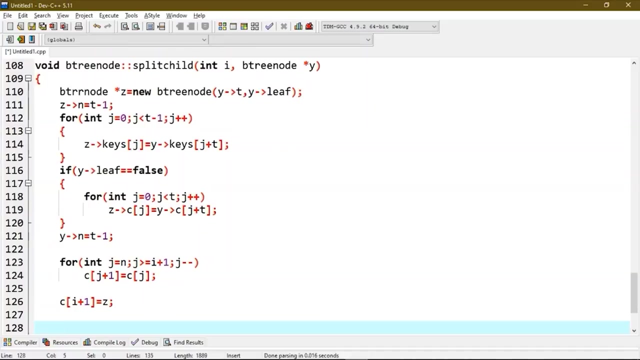 child. so for int j is equals to n and j is greater than equals to i plus 1 and j minus minus c j plus 1 will be equals to c j. now we will link the new child to this node, so c bracket i plus 1 equals to z. now a key of y will move to this node, so we will find the location. 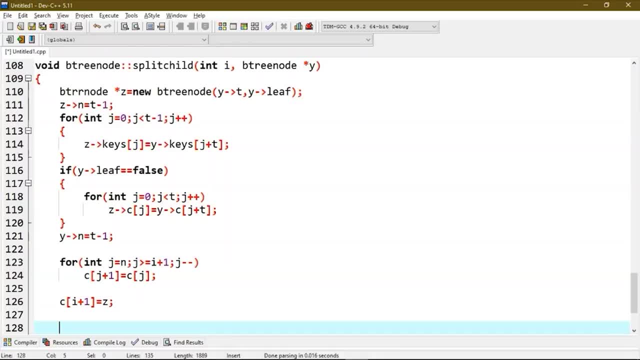 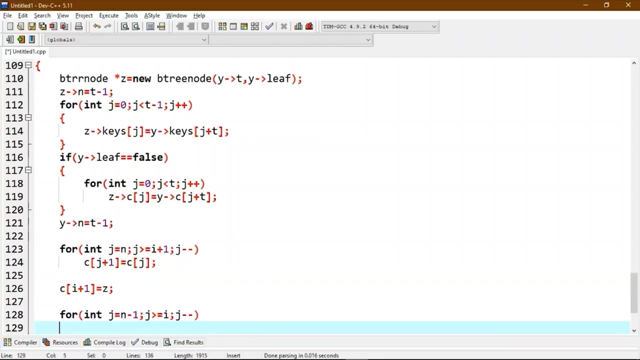 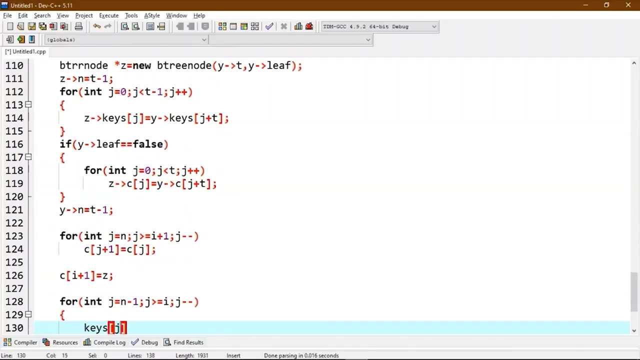 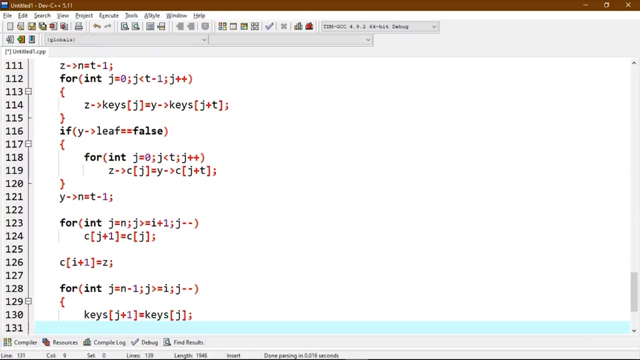 of new key and move all greater keys one space ahead. so for int j is equals to n minus 1, j greater than equals to i. j minus minus is j plus 1 equals to keys j. now we will copy the middle key of y to this node, so key is bracket. i is equals to y arrow. 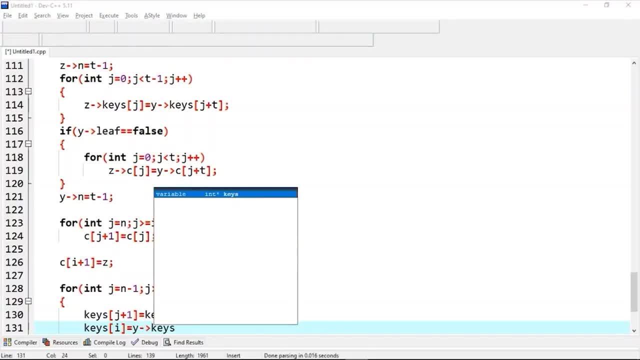 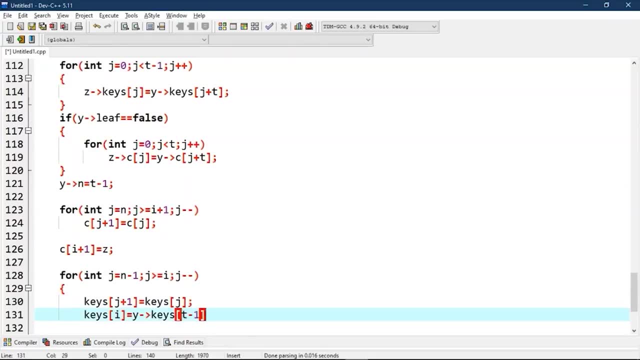 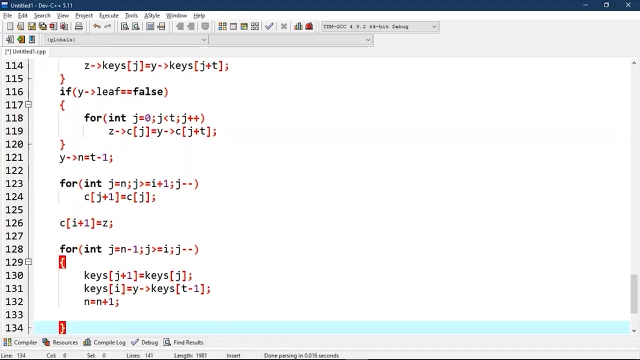 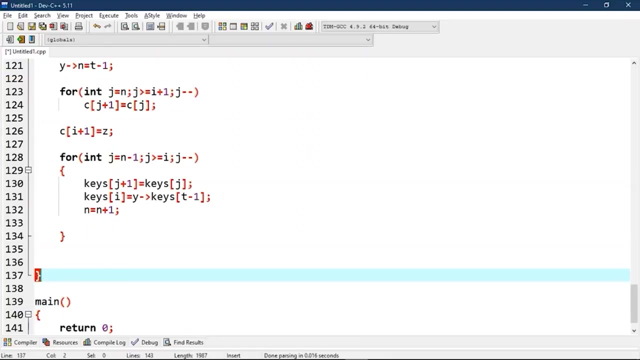 is at t minus 1. now we will increment the counts of key in this node. so n equals to n plus 1. now we will write a driver program to test above functions. now we will start the root function as Jewish. now we will write the main block. 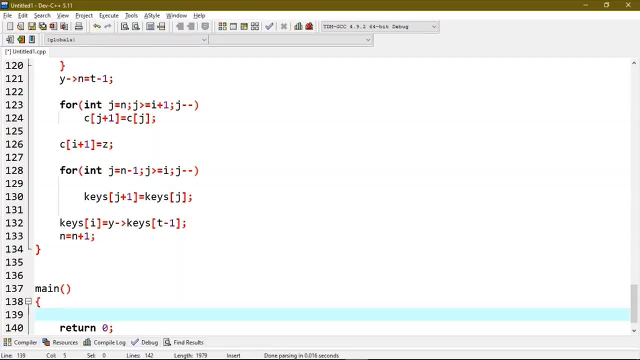 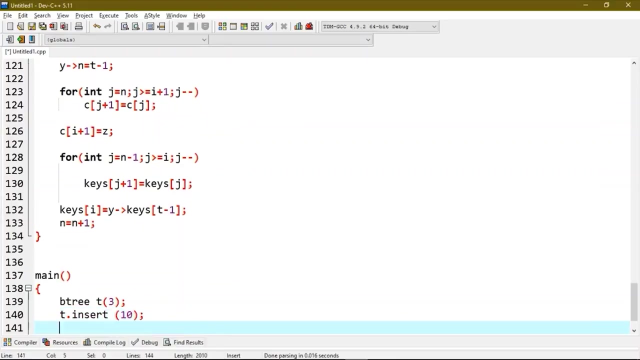 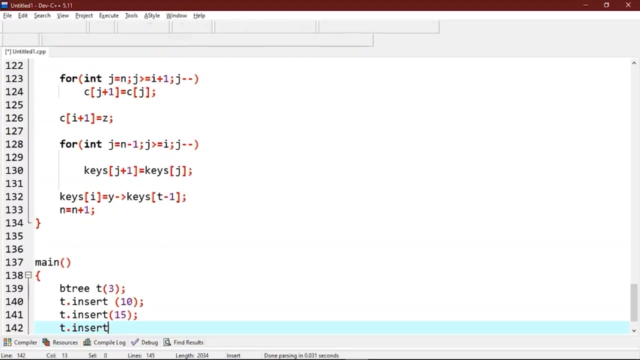 we will start with the B tree with Ne of degree three Soon. let us review some examples. after introducing barrier, what you are looking for Now? we will insert keys in this tree. so tinsert 10, tinsert 15, tinsert 5, tinsert. 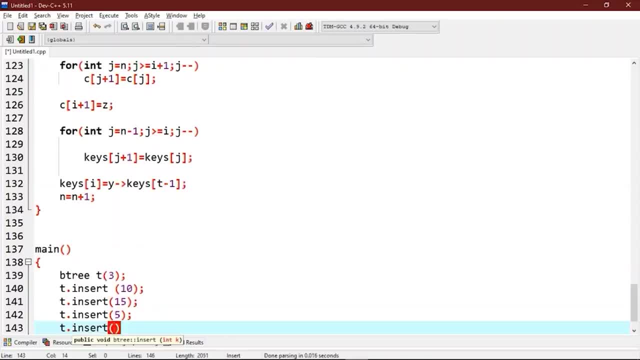 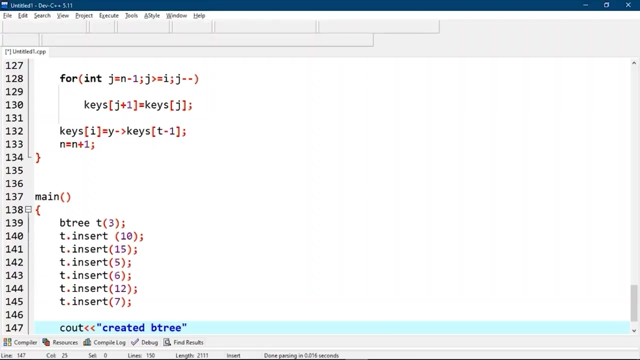 tinsert 6, tinsert 12, tinsert 7, tinsert 8, tinsert 9, tinsert 10.. Now let's print this constructed tree. so cout created btree s, Now tinsert. 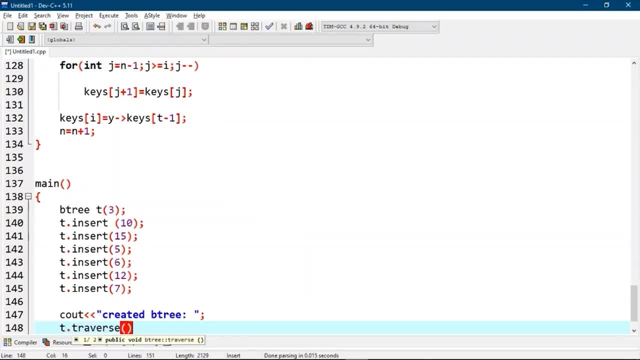 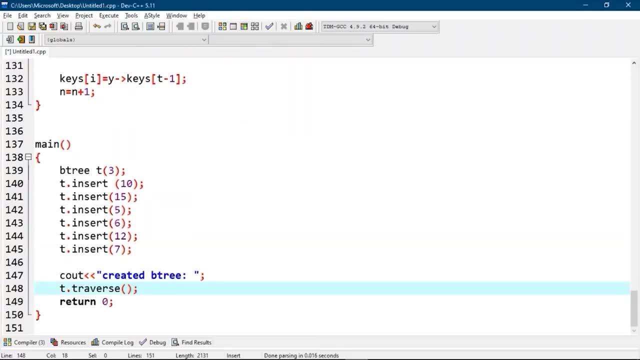 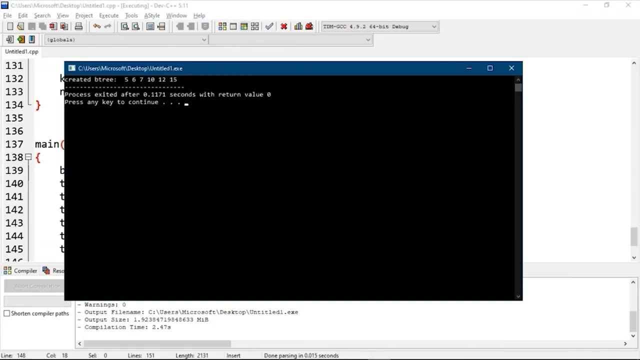 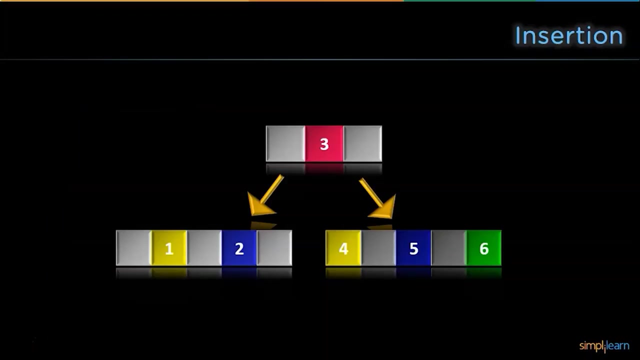 Traverse. Now let's execute this. As we can see, we have created btree of order 3.. Let's get back to our slides. Finally, deletion. While deleting any elements from btree, we have to be careful not to break any properties of the btree. 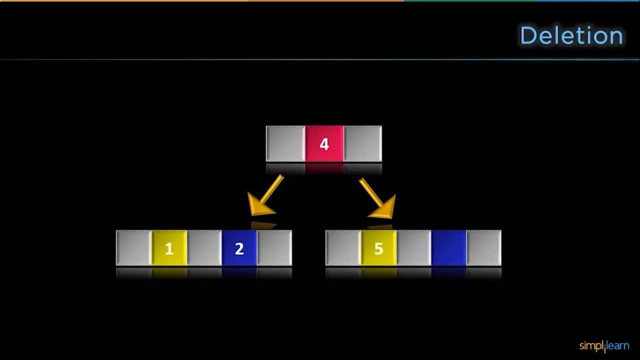 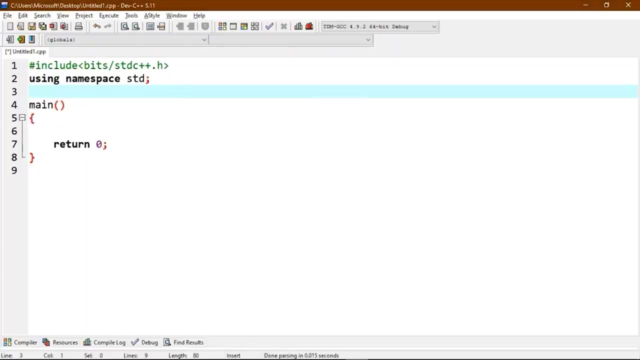 Like all, the leaves must be present at the same level or elements must be in ascending order. Now let's try this operation in a code editor. Let's start by creating a node. To create a node, we need a class. 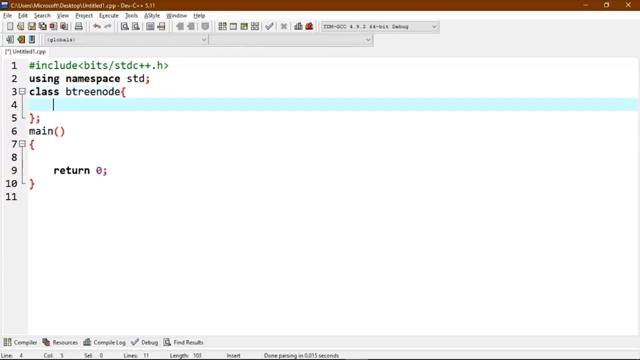 node: int startkeys. this is an array of keys: int t, a minimum degree. Now we will define an array of child pointers, so btreeNode. Now we will define an array of child pointers, so btreeNode. 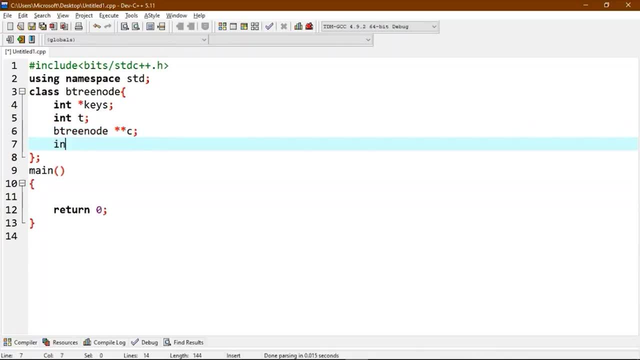 And a number of keys: int, n, A Boolean variable leaf to tell us if the node is leaf or not. Now we will define some public functions. We will start with the constructor of this class: btree node. int- underscore t comma boolean. 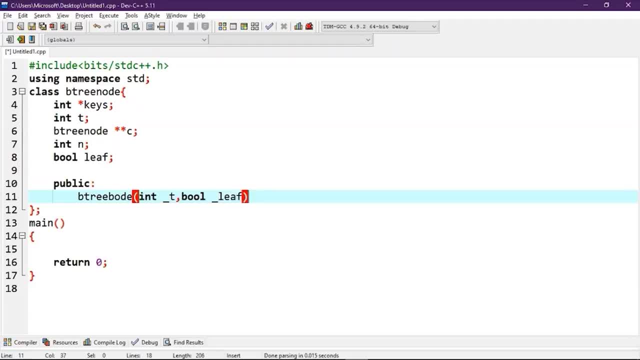 underscore leaf and a function to traverse all nodes in the sub-routed tree. so void, traverse. Now a function to search a key in the sub-tree. so btree node, star, search int k. This will return null if k is not present. Now we will write a function that returns the index of the first key that is greater or 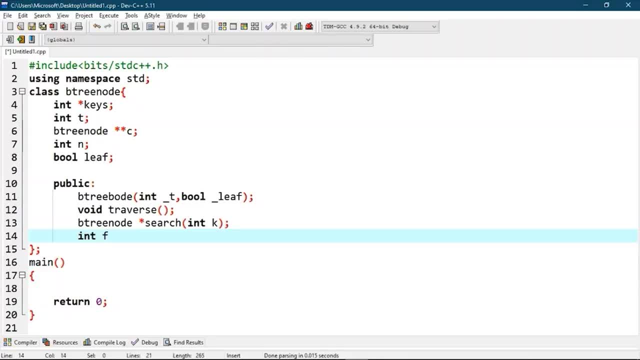 equal to k. so int point key: int- k. Now we will write an utility function to insert a new key in this sub-tree Rooted with this node. we will be assuming the node must be non-full when this function is called, So void insert non-full as argument as k. Now we will write a utility function to split. 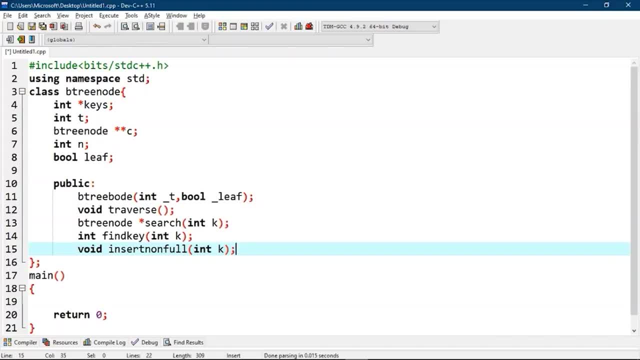 the child of y of this sub-tree. Now we will write a utility function to split the child of y of this sub-tree. Now we will create an entity of y of the sub-tree我要. We will say that the 2017 itsMultiple célint. 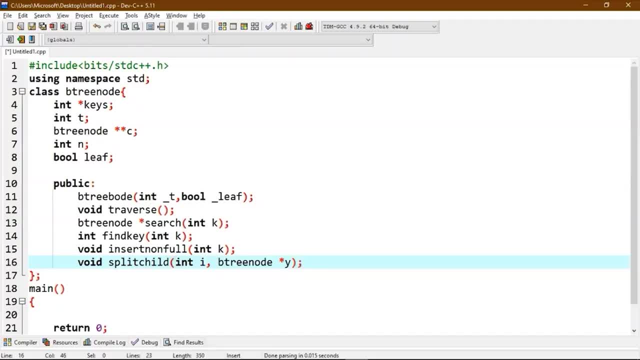 be called child. int i comma, btree node star y, Cheng y, R p, j. A wrapper function is to remove the keys k in substituted with this node. So void: remove int k. Another function: to remove a key present in the ith position in this node, which is a non-leaf. 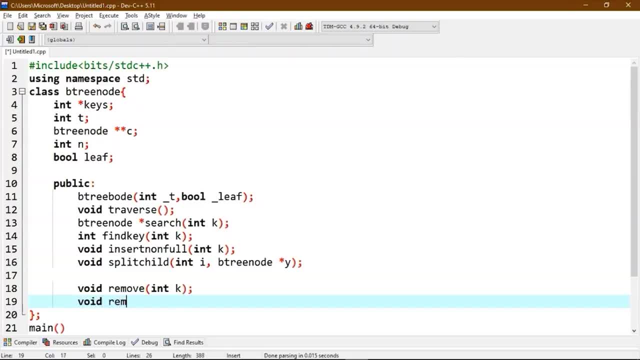 node. So void: remove from non-leaf int: idx. Now we will write a function to get the predecessor of the key where the key is present in the idx node. Now we will finish this simple function by removing the keys k which were present in. 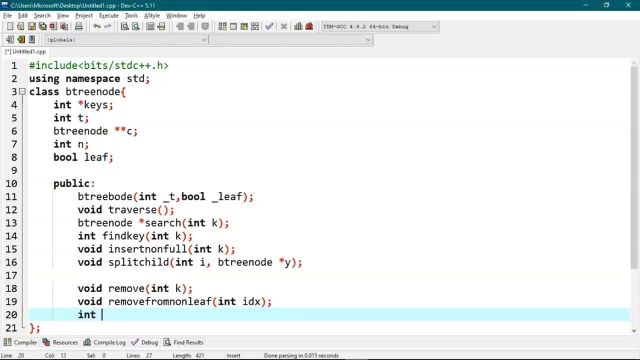 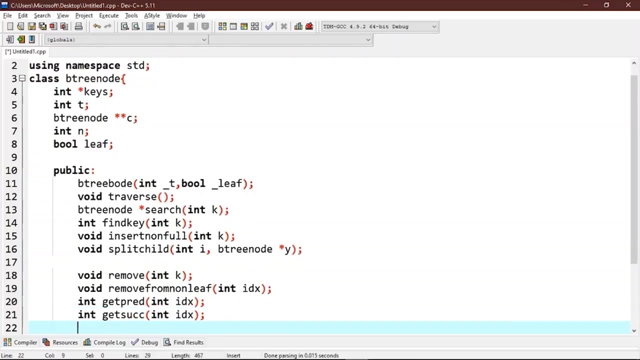 the for of this node. So void. remove from non-leaf int idx node. So attendees can now copying this line. We can hit O Demon, So it occurs. Now we will return this to our node: int getSuccessor int idx. Now we will write a function to fill up the child node present in the idx position in. 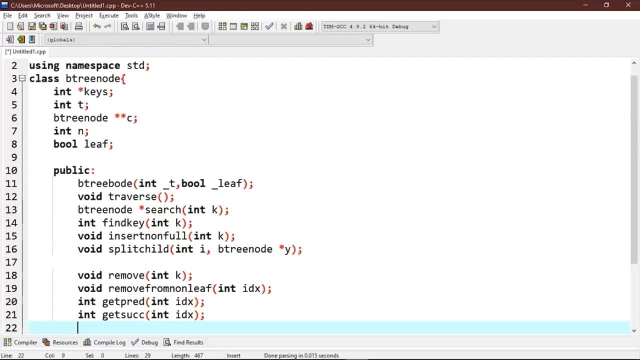 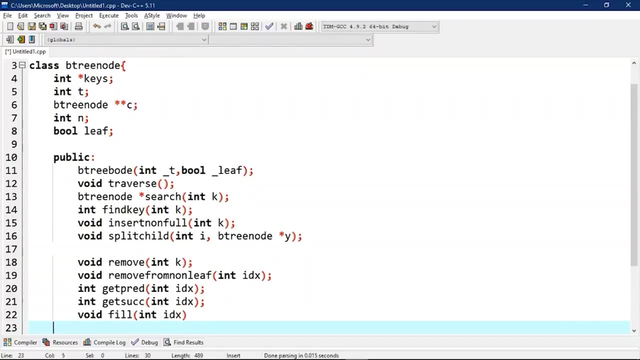 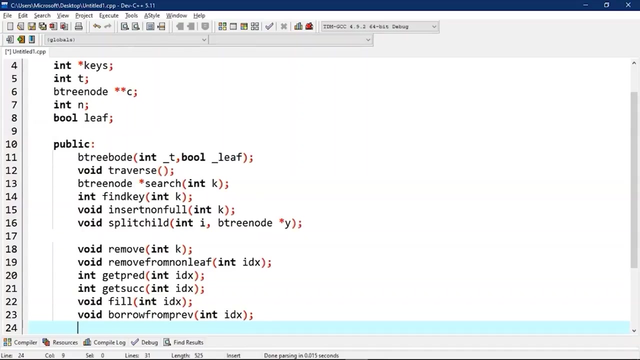 the C array if that child has less than t-1 keys. So void: fill int idx. Now we will write another function to borrow a key from the C node and place it in C node. So void: borrow from rev int idx A function to borrow a key from the idx plus one node and place it at the idx. 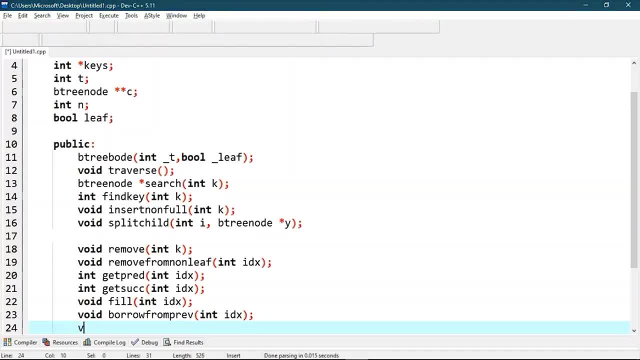 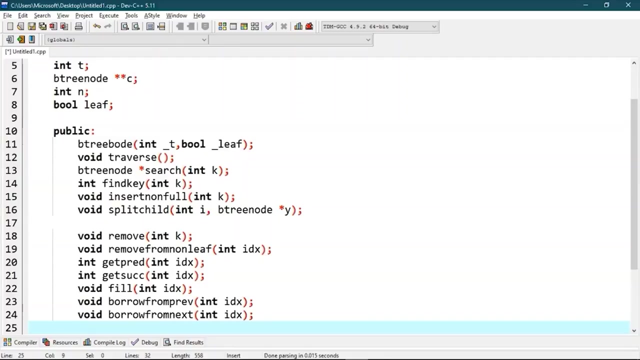 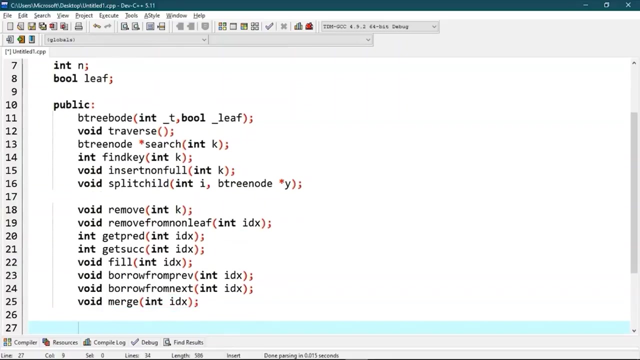 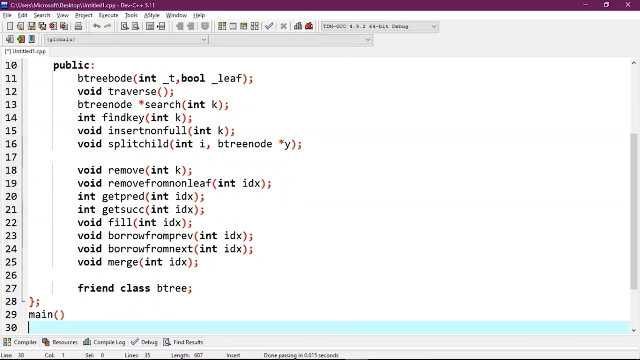 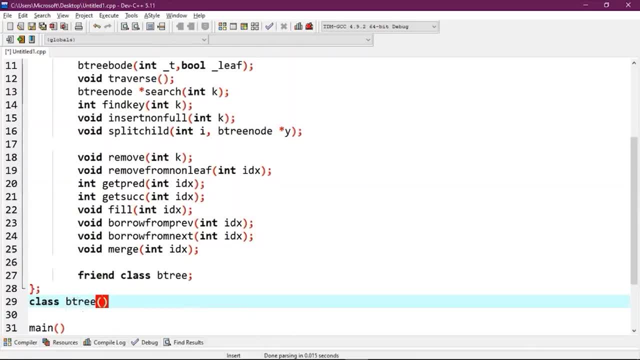 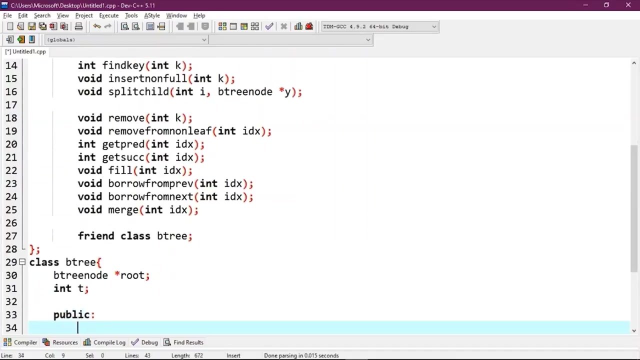 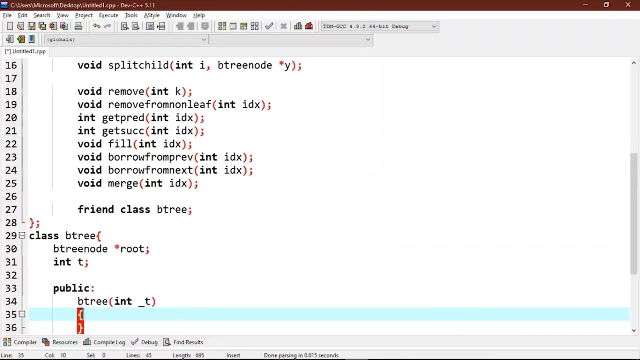 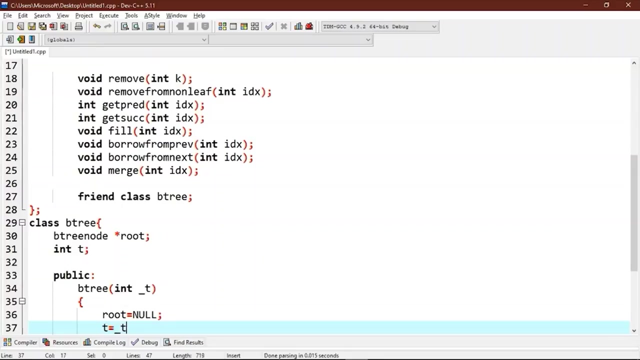 so class. we will start with the pointer to the root node. so btree node star, root, int t. now we will write some public functions: btree btree. we will start with the constructor. so btree int underscore t. so root is equals to null and t is equals to underscore t. 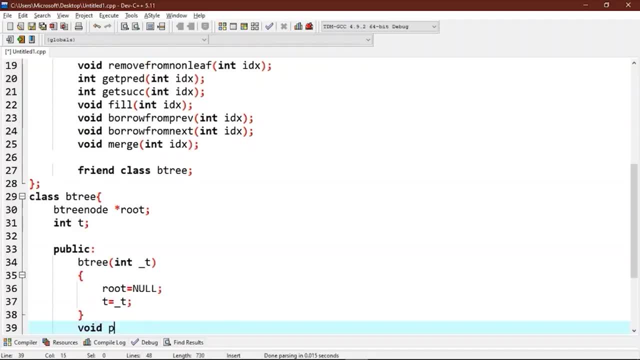 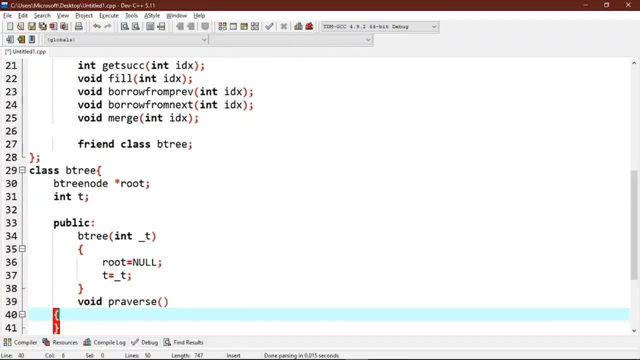 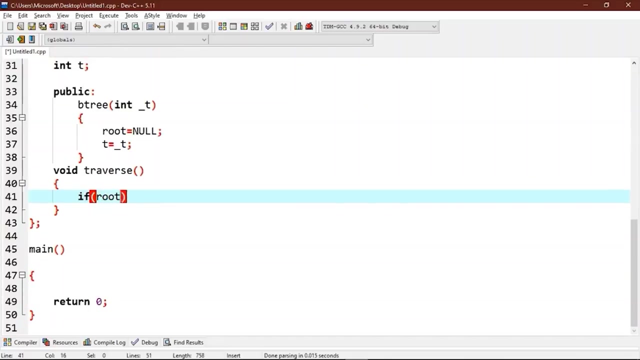 now a traverse function, void traverse. so we will check. if root is not null, then root arrow traverse. now we will write a function to search a key in this tree. so btree node search f and k, we will return. if root is equals to null, then we will return null, else root arrow search at key. 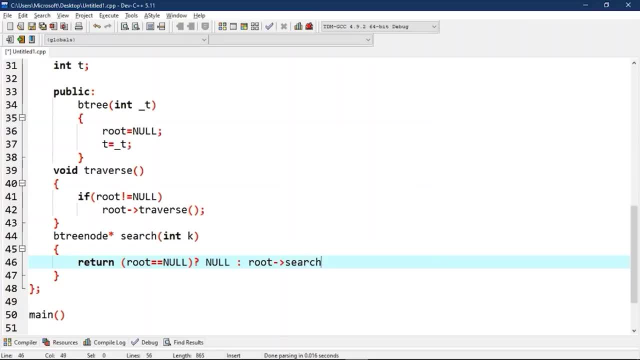 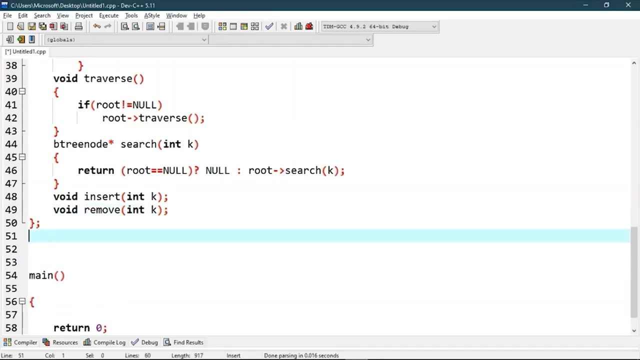 now we will write the main function that inserts a new key in this b-tree. so void: insert int k. now another main function that removes the new key in this b-tree. so void: remove int. now we will write the constructor for this b-tree: node us, us. 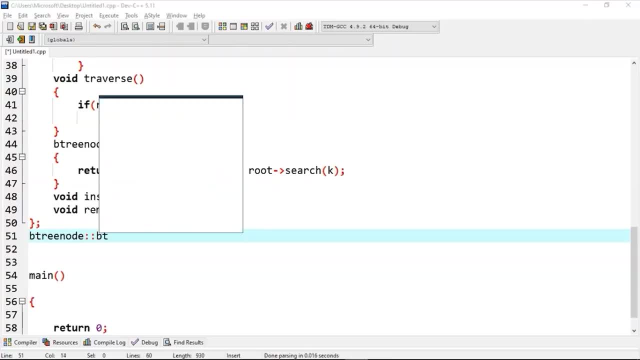 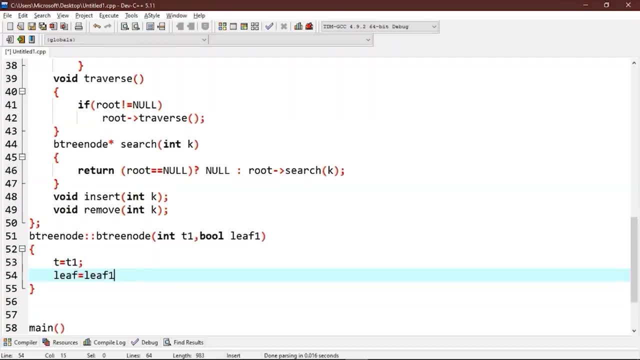 int t1 comma. int t1 comma. do now we will allocate memory for your maximum number of possible keys and child pointers. now we will allocate memory for the maximum number of possible keys and child pointers. so keys is пу như encode, guess, and equals to. 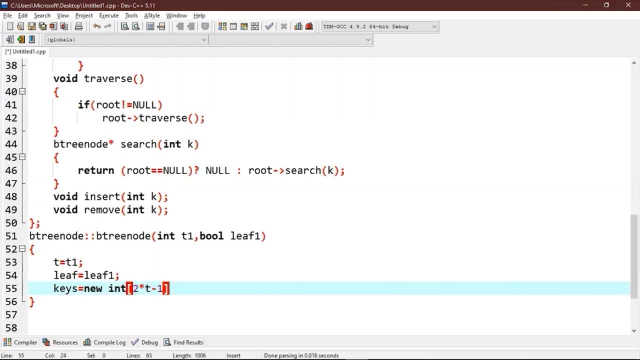 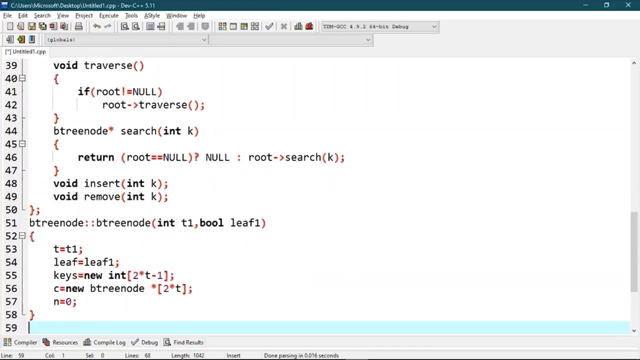 ashi minus 1 and child C is equals to new B tree node star bracket 2, star T. now we will initialize the number of keys as 0, so N is equals to 0. now we will write a utility function that returns the index of the first key that is greater than or. 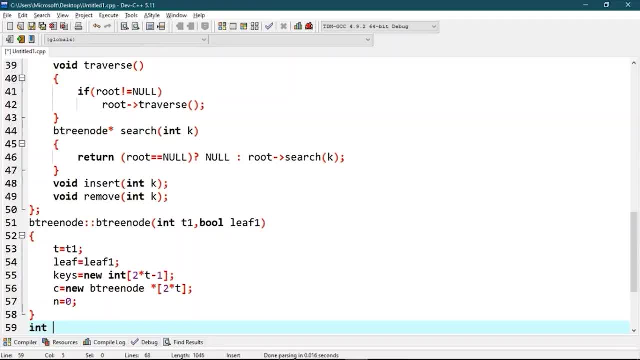 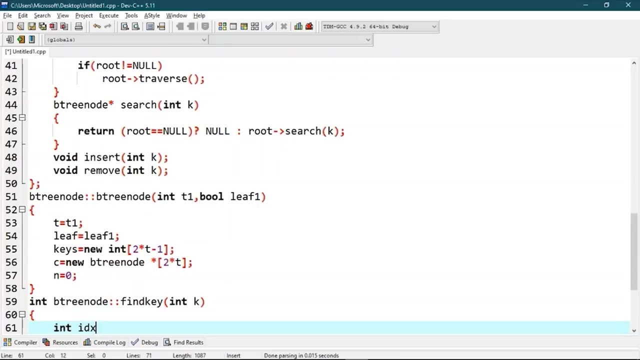 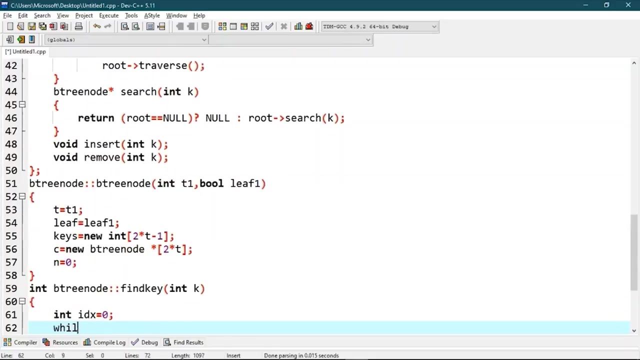 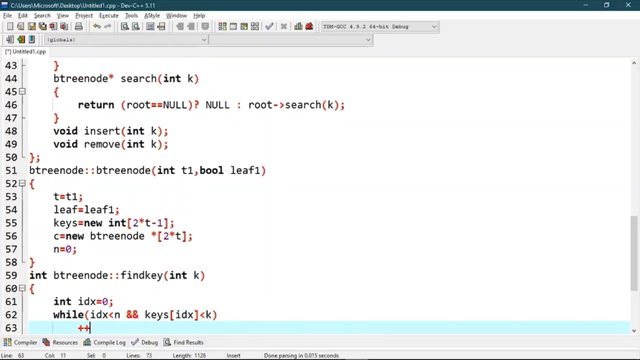 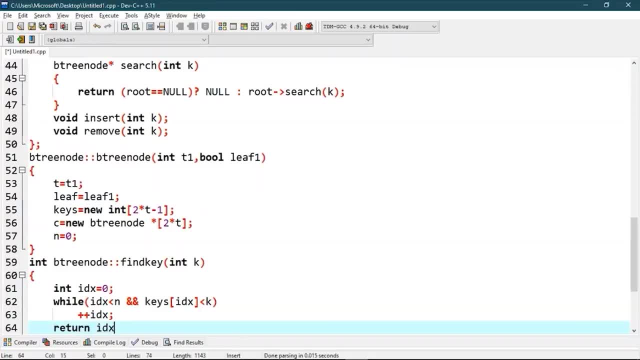 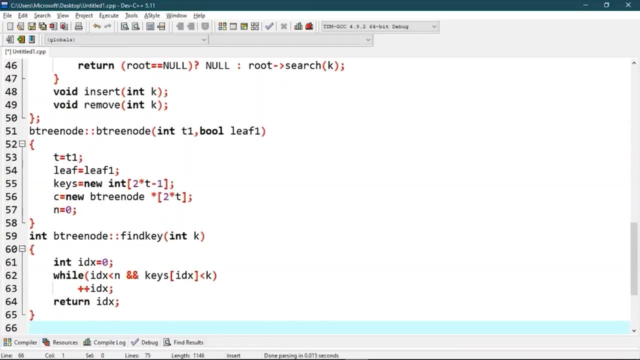 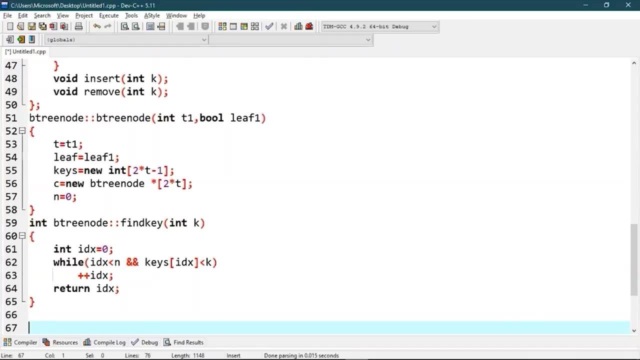 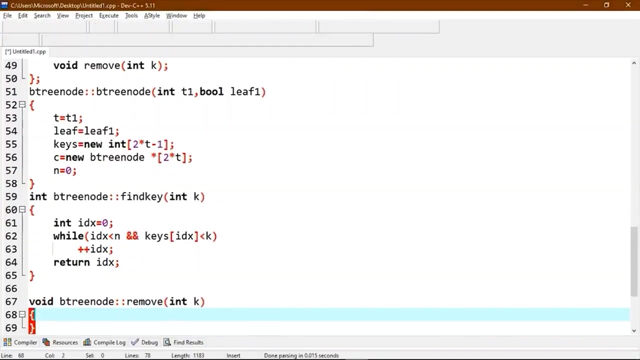 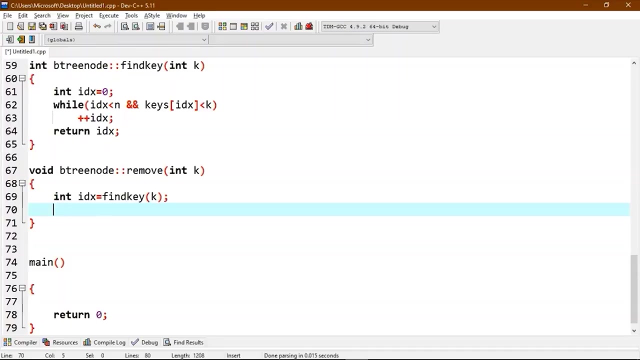 return idx. Now we will write a function to remove the key k from the subtree rooted with this node. So void btree node, remove int k. int- idx equals to find key k. if the key to be removed is present in this node, then if idx is less than n. 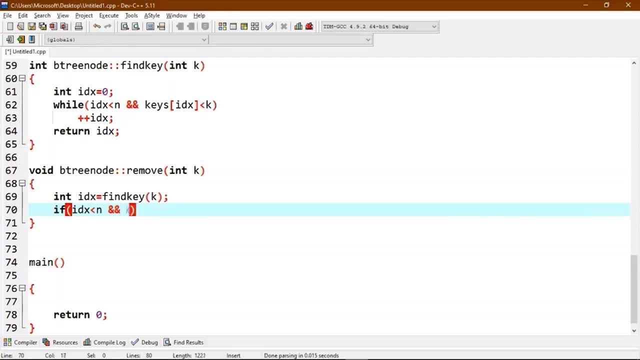 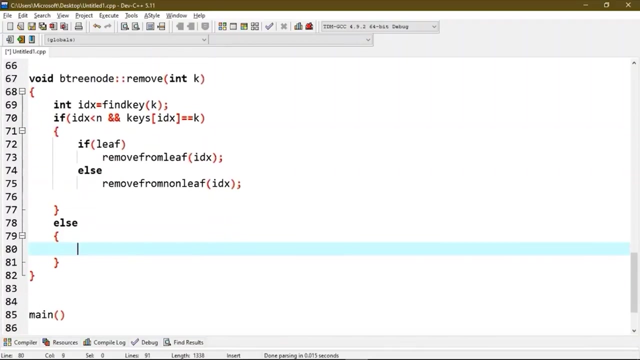 and keys at idx is equals to k. now if node is leaf node, then we will remove from leaf node is called. otherwise remove from non leaf function is called. so if leaf, then remove from leaf idx, else remove from non leaf idx. ев, idx, surface SI idx. 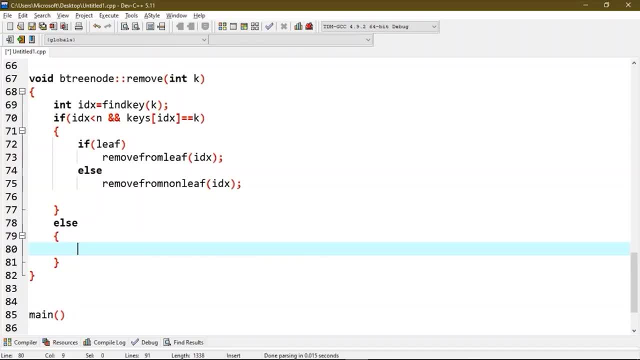 if this node is leaf node, then k is not present in the subtree. so if leave sealed is, does not exist, industry and return and return and return. so the key to be removed is present in this subtree rooted with this node. the flag indicates whether the key is present in this subtree rooted. 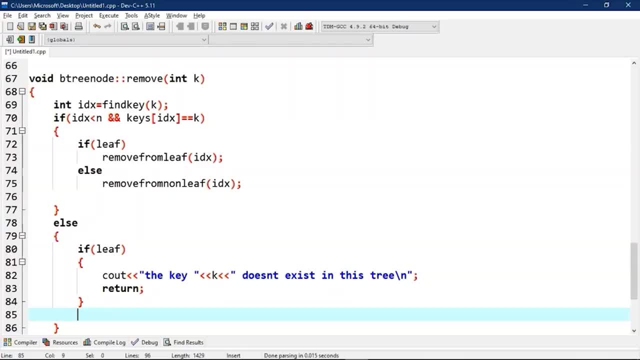 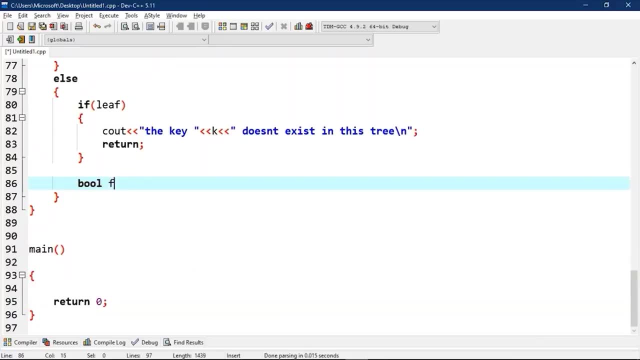 with the last child of this node. so surprised guilty flag is equals to IDX, equals to n if it is true, else false. if the child where the key is supposed to exist has less than T keys, then we fill that child. so if C at IDX and it's less than T, then fill IDX. 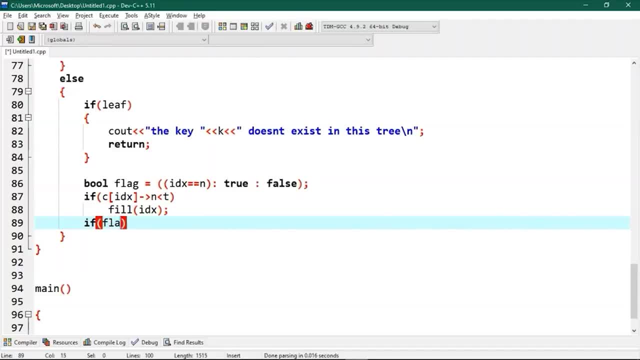 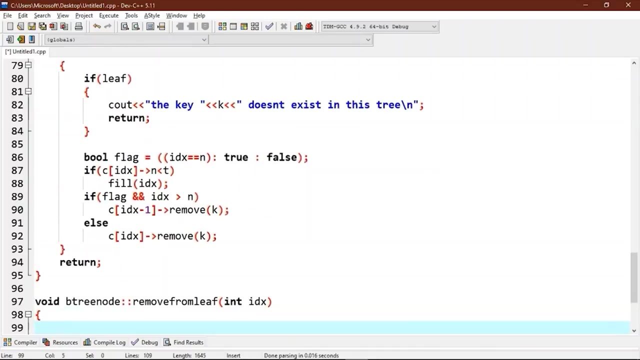 now, if flag and IDX is greater than n, and see IDX minus one, remove a, else else see IDX. remove a return. return string. string void from B tree node. remove from leaf. from leaf. Now we will move all the keys after the idx position, one place backward. 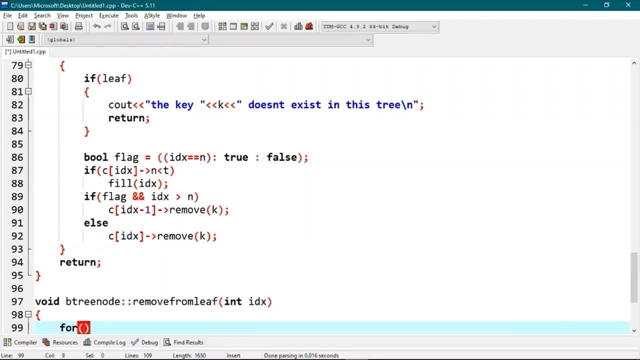 So for loop int i is equals to idx plus one. idx plus one. i less than n, i plus plus. So for loop int i is equals to idx plus one. idx plus one. i less than n, i plus plus. So for loop int i is equals to idx plus one. idx plus one: i less than n. i less than n, i plus plus. 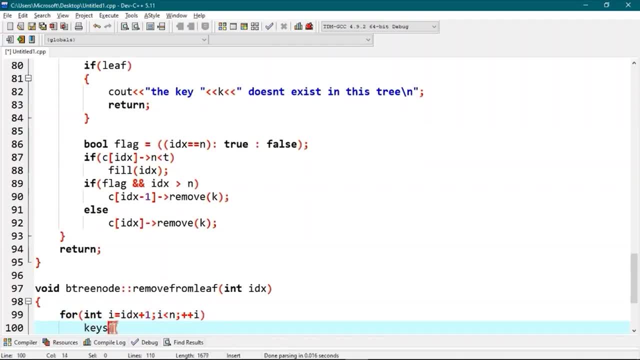 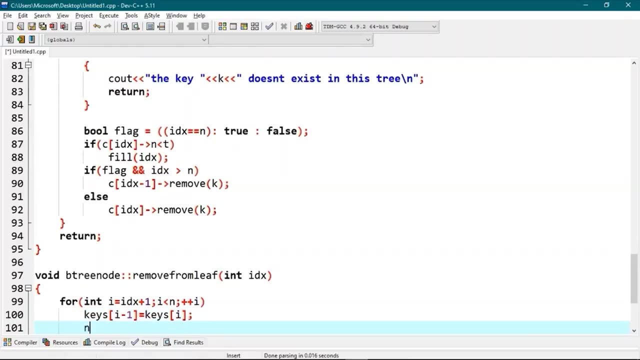 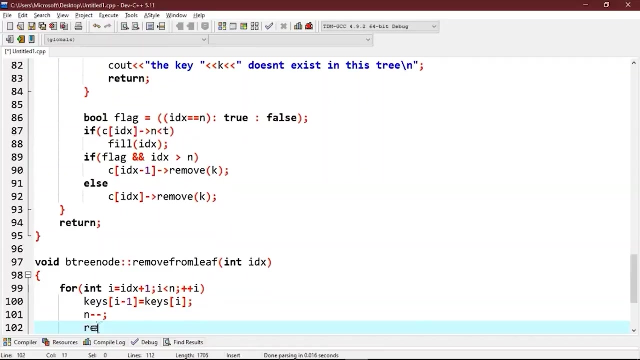 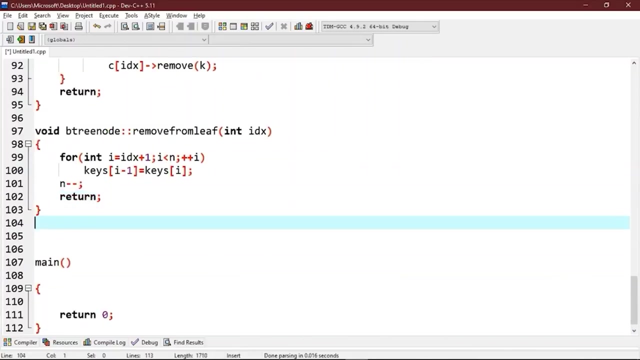 So keys at i minus one should be equal to at i And we will reduce the count of keys, So n minus minus, Then return. Now we will write the function to remove the idx key from the node which is non leaf node. 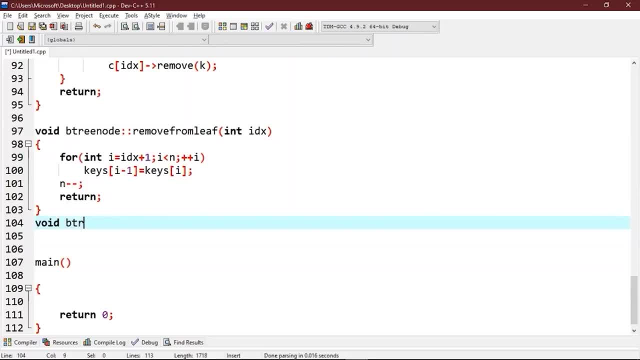 So void btree node: remove from non leaf int: idx. int k is equals to keys at idx. So we will write the function to remove the idx key from the node which is non leaf node. Now we will write the function to remove the idx key from the node which is non leaf node. 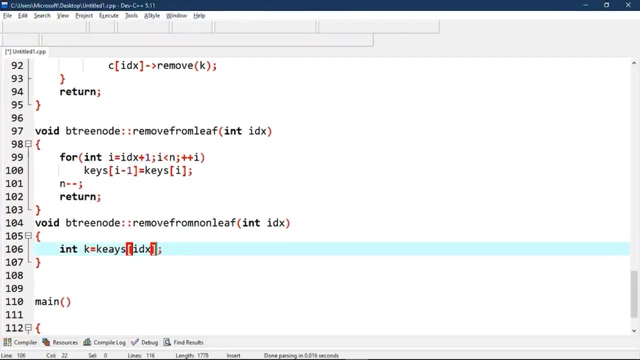 So void: btree node: remove from non leaf node. So we will write the function to remove the idx key from the node which is non leaf node. If the child that precedes k at CIDX has at least t keys, then we will find the predecessor. 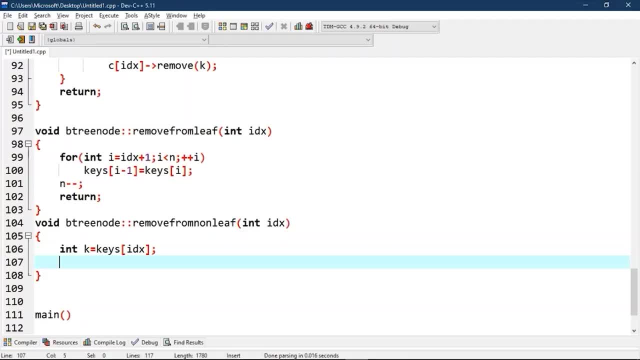 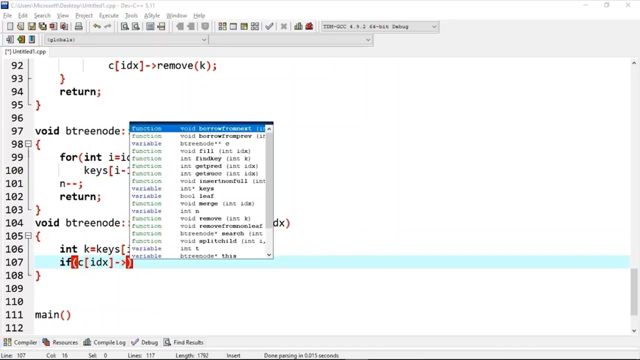 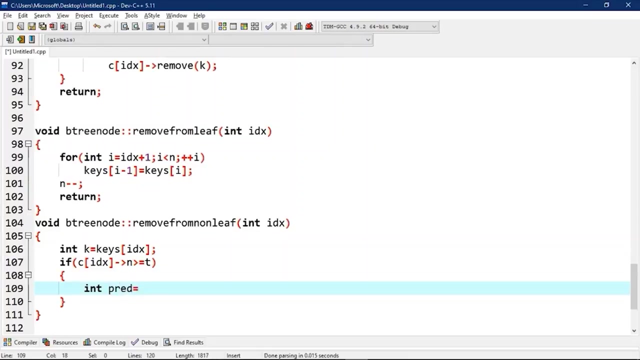 pred of k in the sub-tree rooted at CIDX. We will replace k by predecessor recursively and delete pred in CIDX. So if So. if So, if idx arrow n is greater than equals to t, then int thread equals to get thread. idx keys. idx equals to thread. 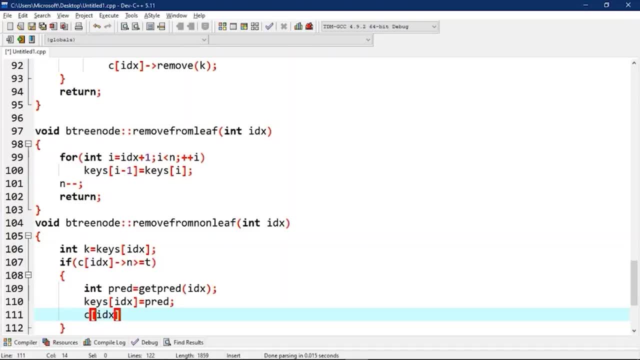 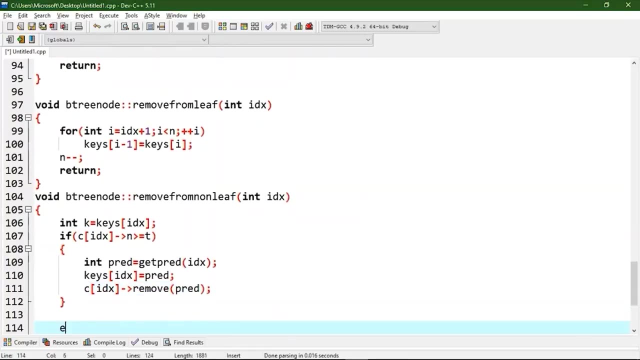 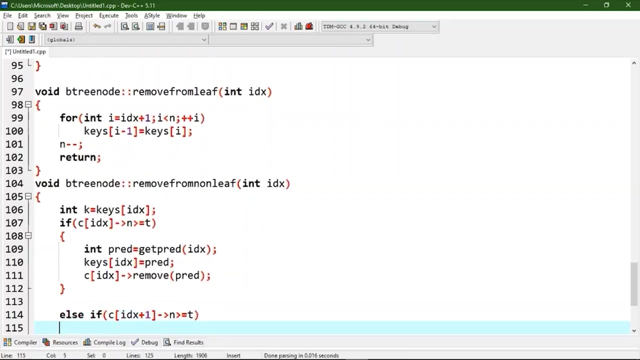 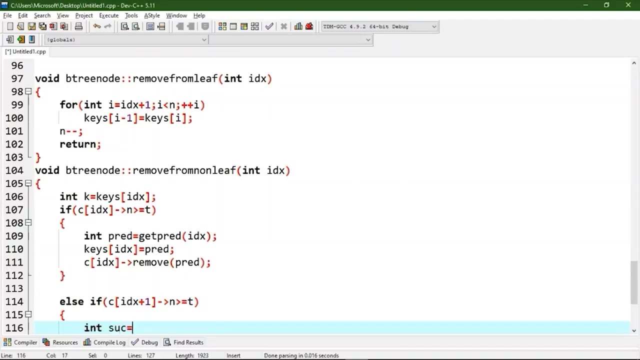 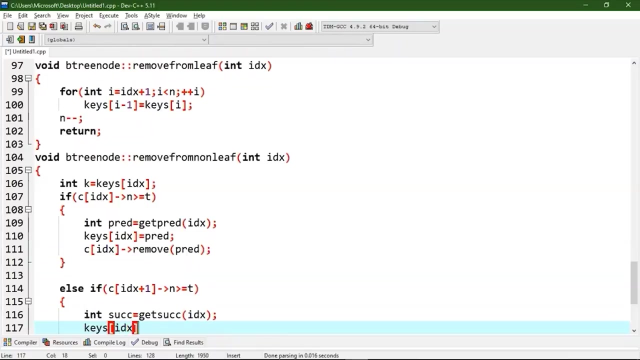 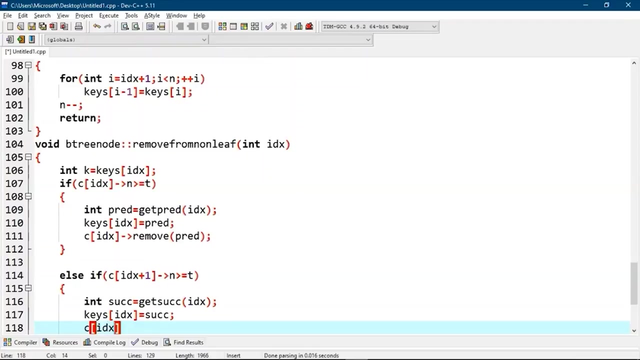 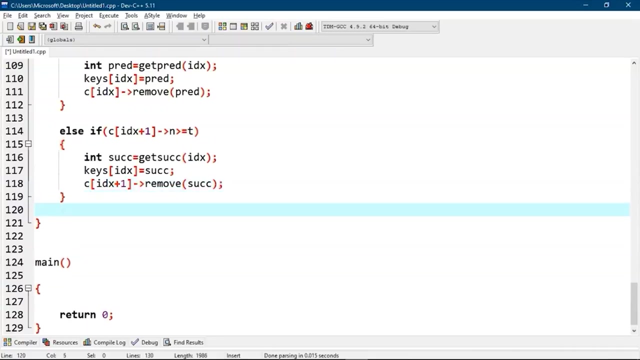 c- idx- remove thread. else, if c at idx plus one arrow n is greater than equals to t, then int suck is equals to get suck. idx of keys at idx is equals to suck c at idx plus one uses. remove suck, else will merge idx and c at idx will. 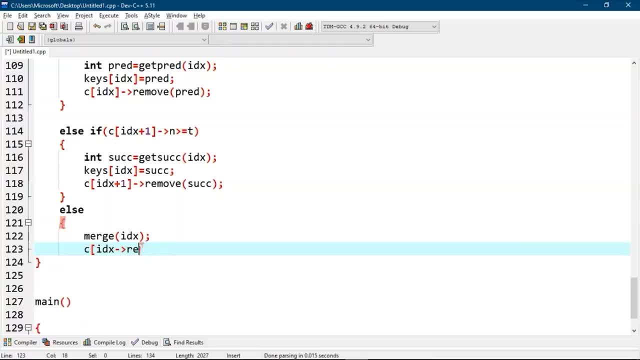 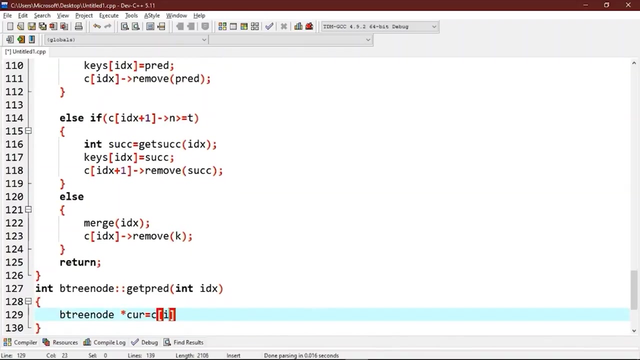 call remove oof suck idx is equal to error At idx. we will call remove. Now we will write a function to get predecessor of keys idx. so int vtreeNode getPred int suck. repeat int idx. vtreeNode startCurl is equals to c at idx. 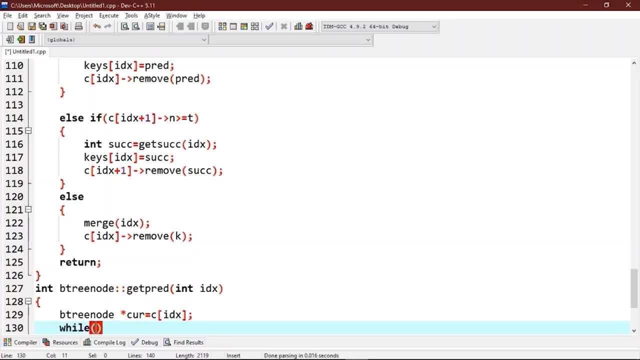 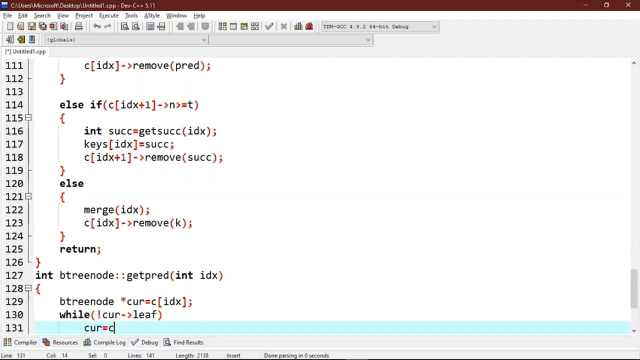 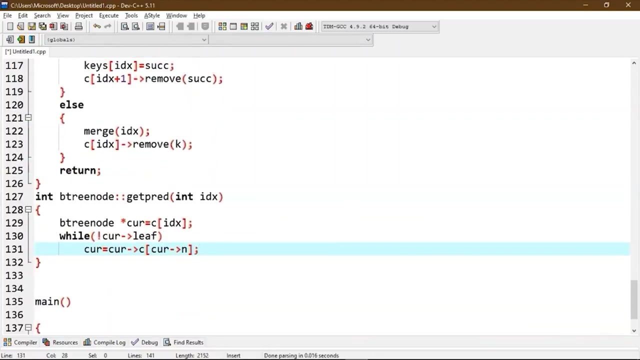 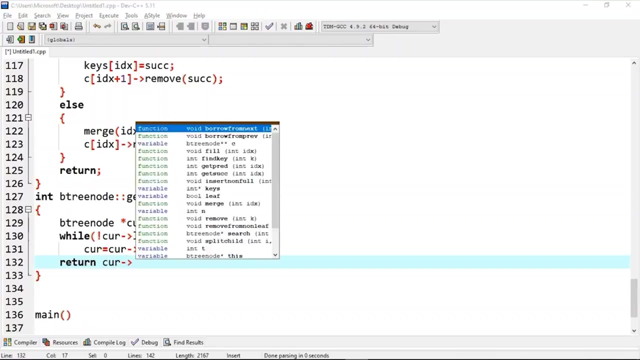 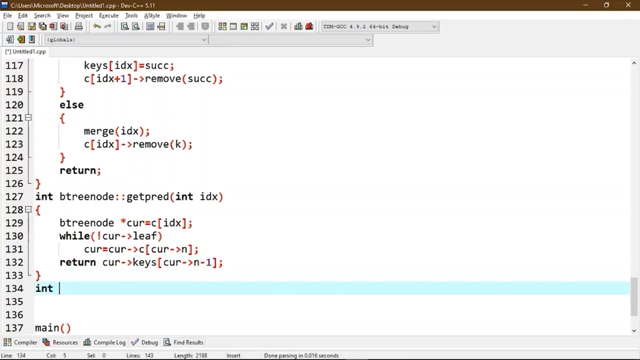 while vtreeNode startCurl is equal to c at idx, when r is not a leaf, r is not a leaf, then r will be equals to c arrow c. c arrow. arrow. c calls n. Now we will return Curve key. Now we will write int btree. 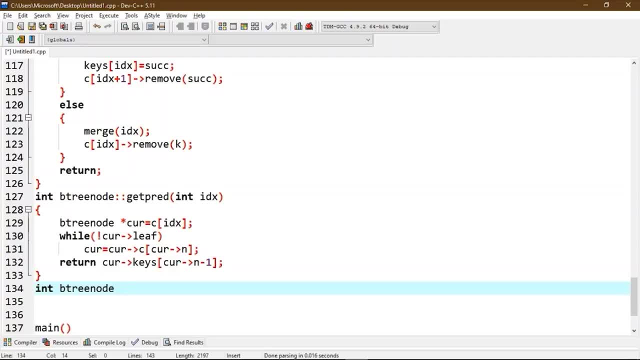 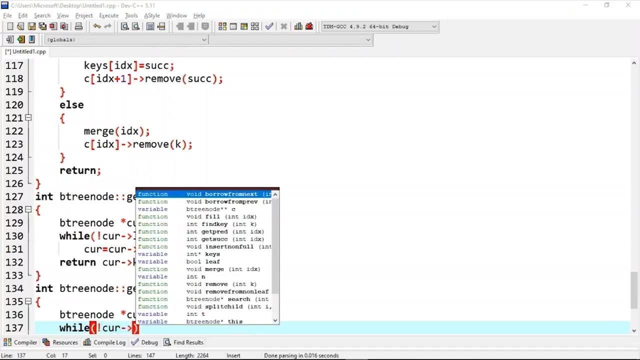 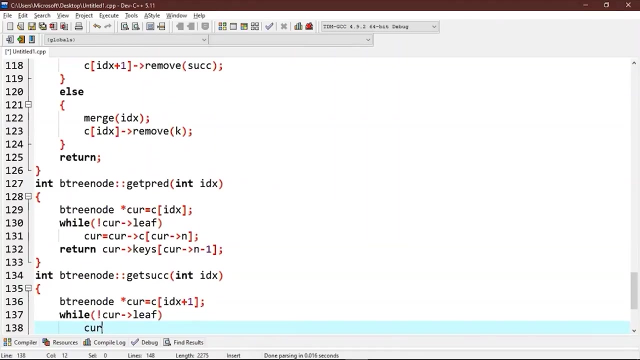 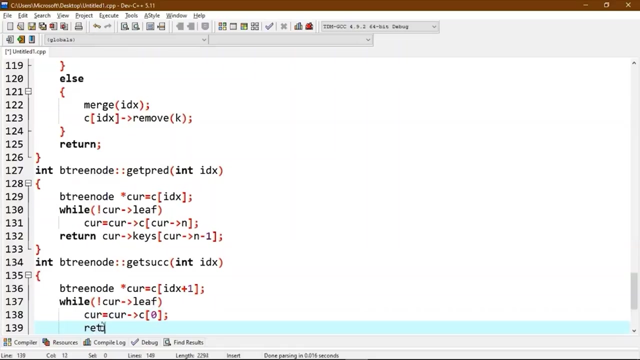 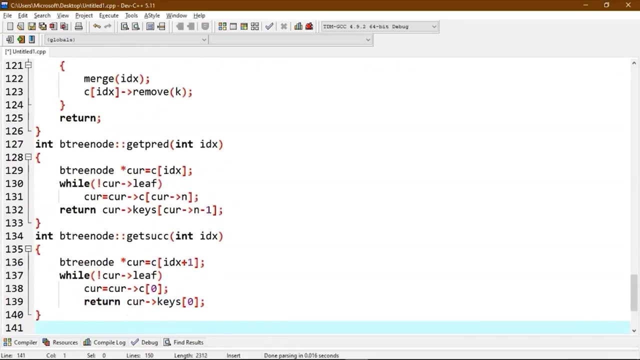 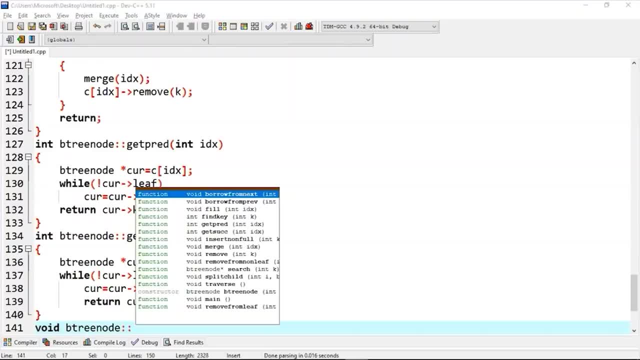 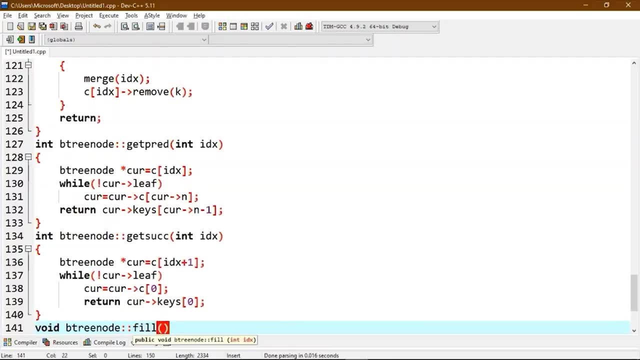 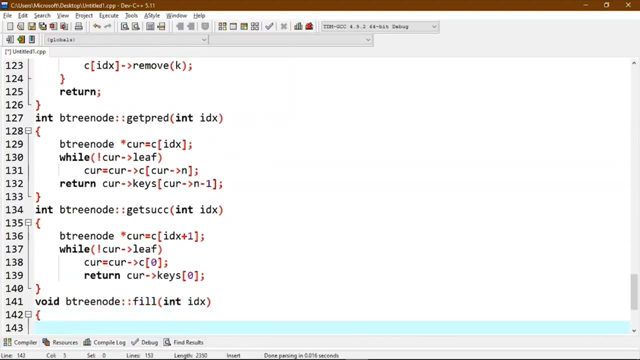 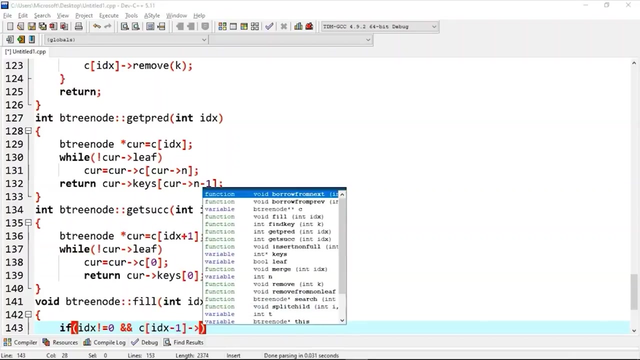 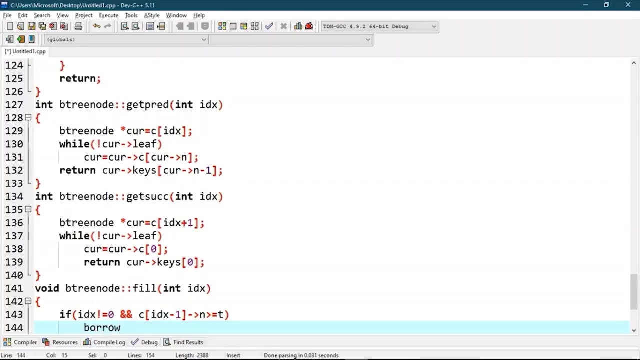 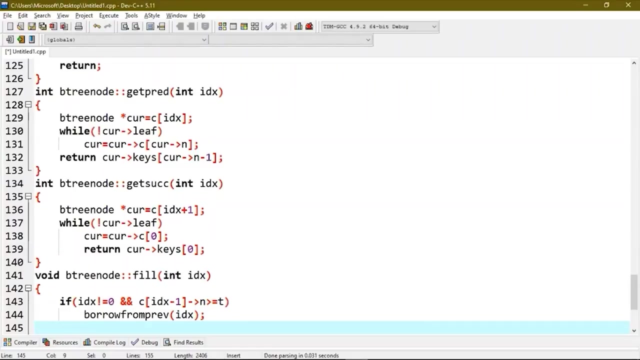 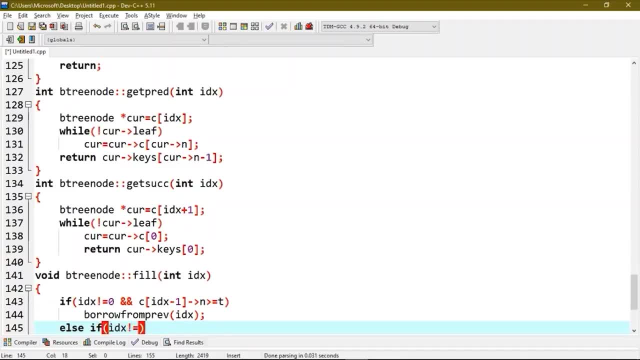 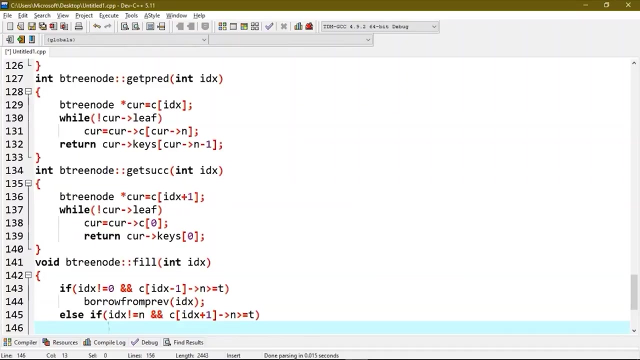 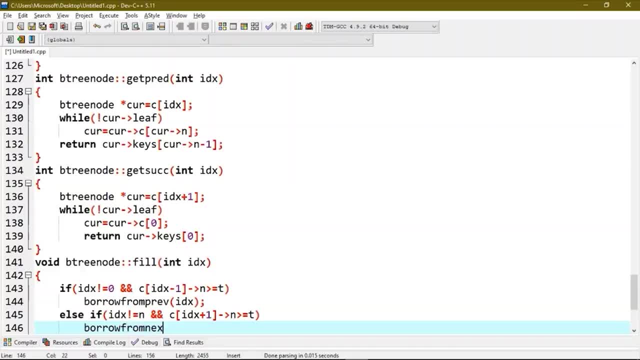 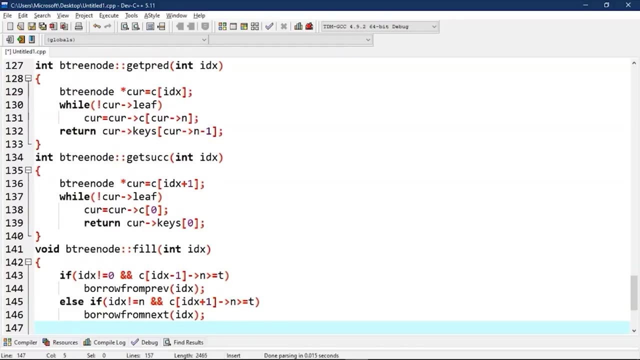 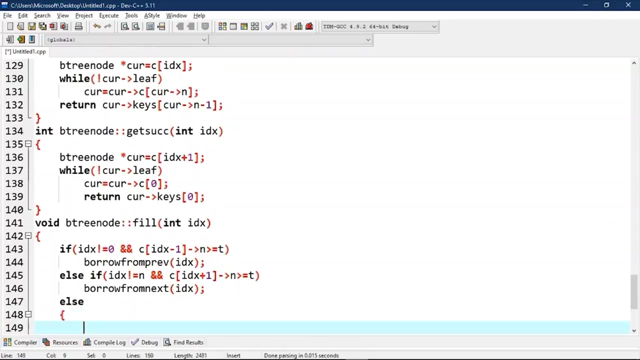 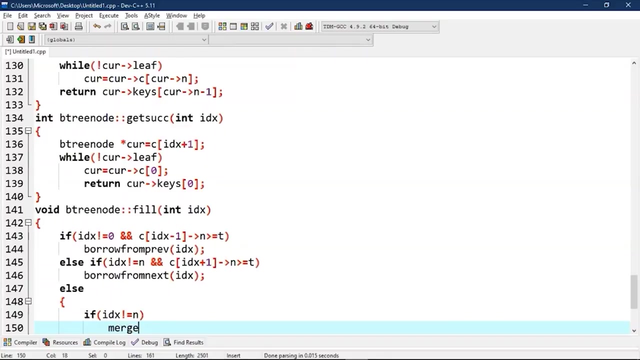 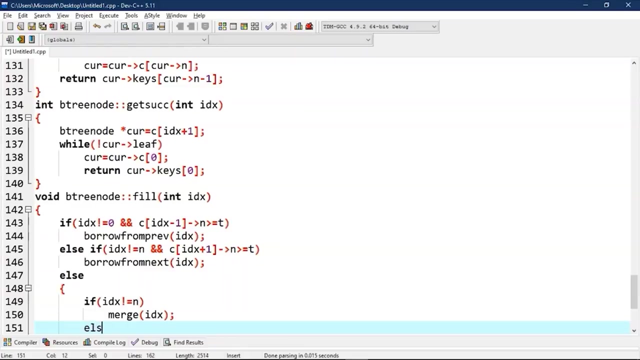 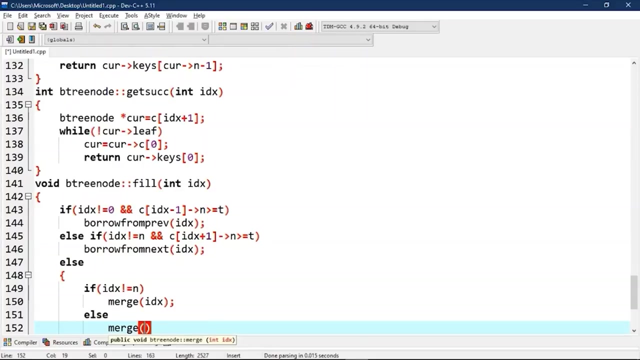 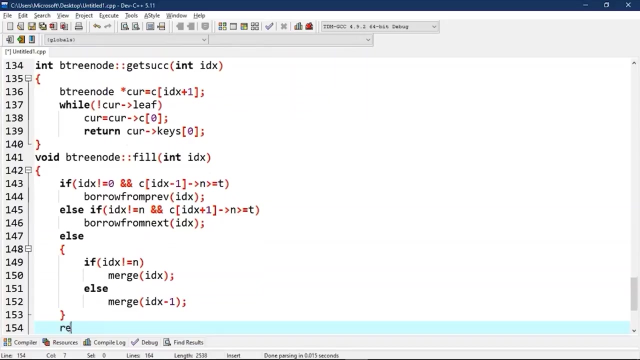 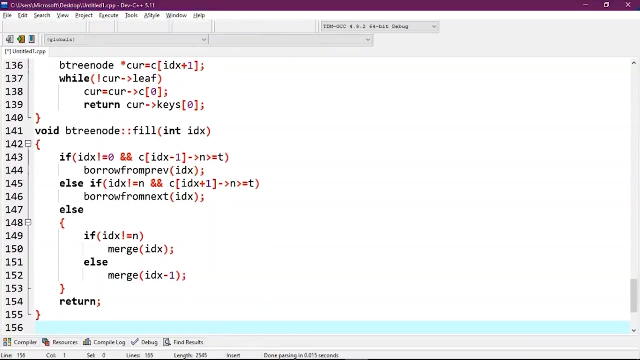 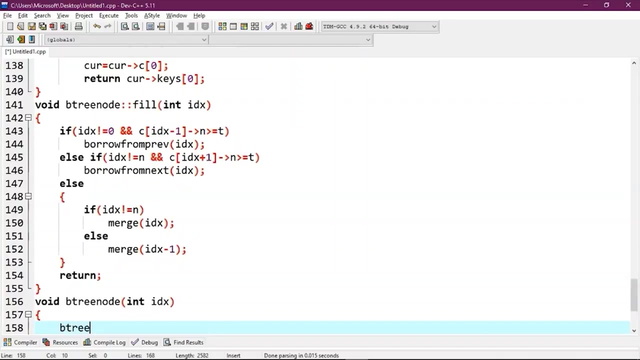 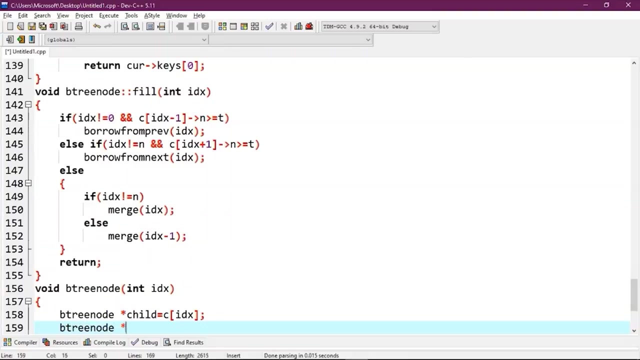 from next at IDX. else, if IDX is not equals to N and we will merge idx is merge IDX minus one. return. now we will write a function borrow from prev. at node star child is equals to C IDX. a train node star sibling is equals to C IDX minus one. 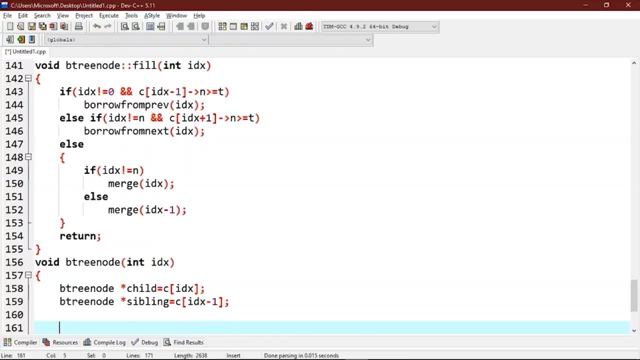 now the last key from C IDX minus one goes up to the parent and key IDX minus one from parent is inserted as the first key in C IDX. thus the losses sibling one key and child gains one key, moving all keys in C IDX one step ahead. so for loop. 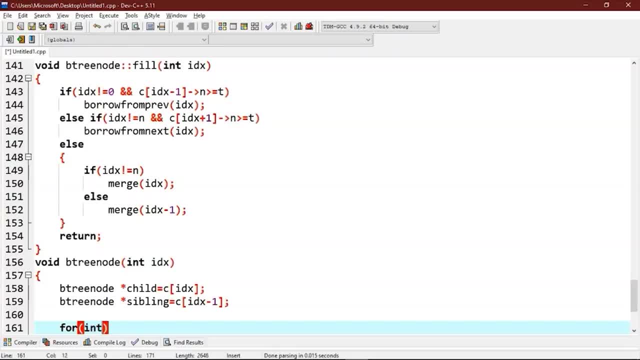 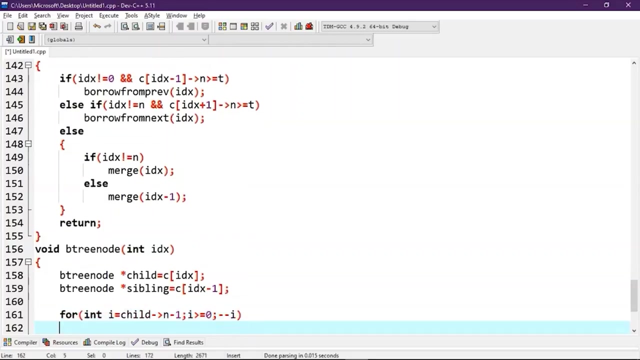 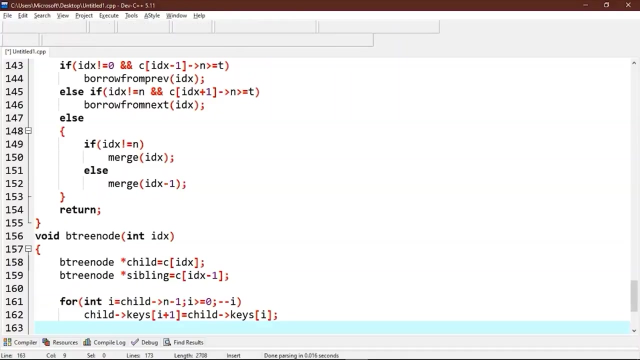 int. I is equals to child. at N minus one. I greater than equals to zero. and I minus minus, minus minus I I'll. I'll. calls keys at I plus one equals to child. calls keys at I I. now, if C IDX is not a leaf, then we'll. 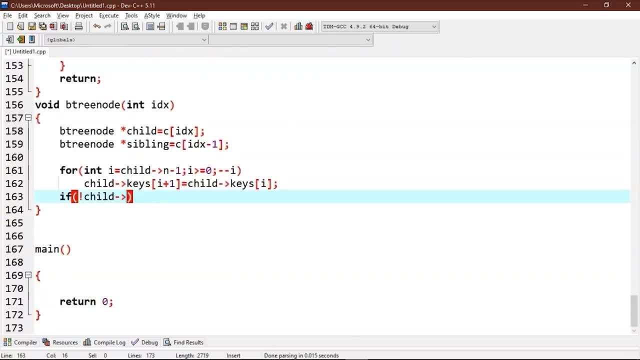 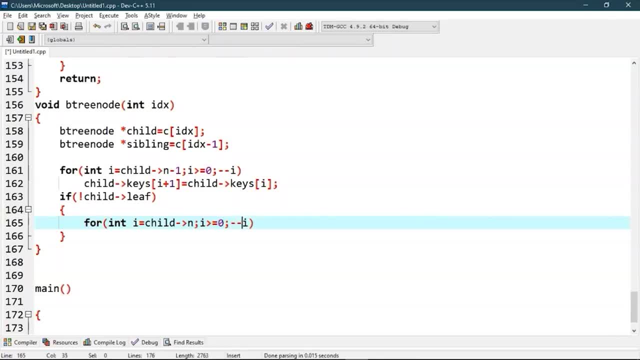 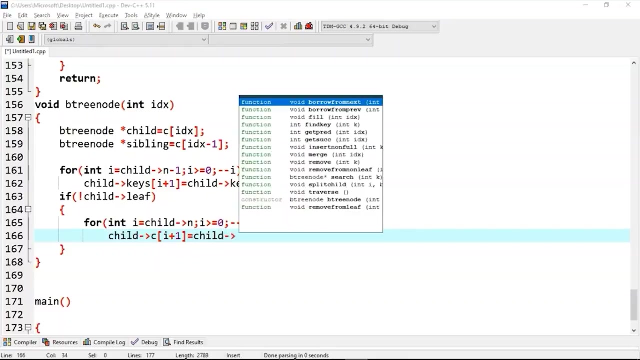 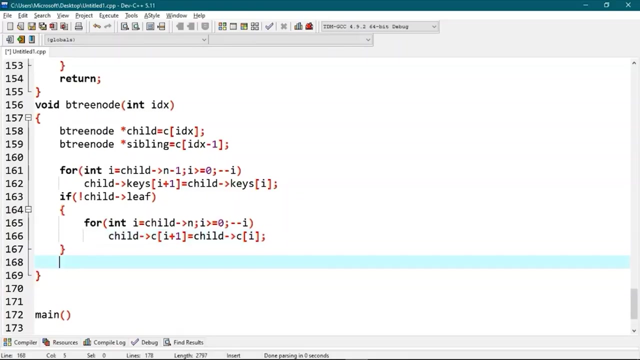 And when we look at this letters I would be very confused at this point. object: object: object: child at C bracket I plus 1 equals to child C bracket I. Now we will set the child's first key equal to the key at IDX minus 1 from the current node. 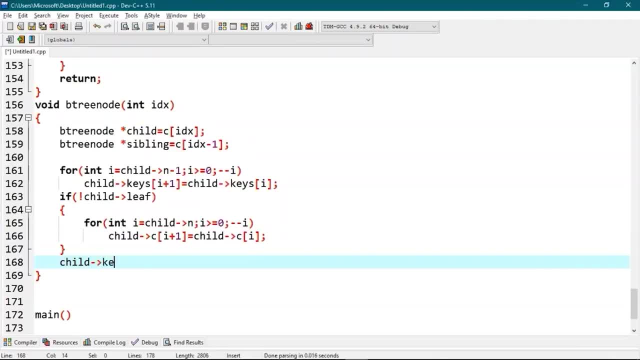 So child is at 0 is equals to keys at IDX minus 1.. Now we will move siblings. last child as CIDX is first child. So if child is not leaf and child arrow C bracket 0 is equals to sibling at C. sibling calls N. 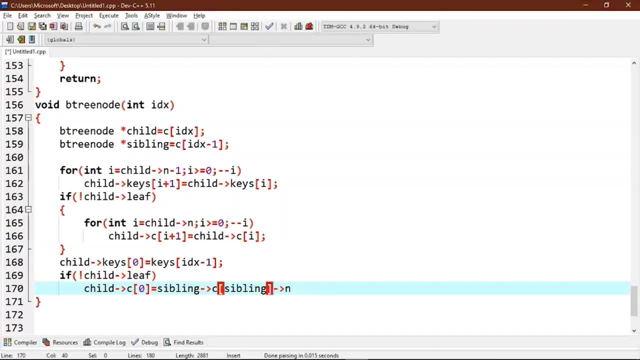 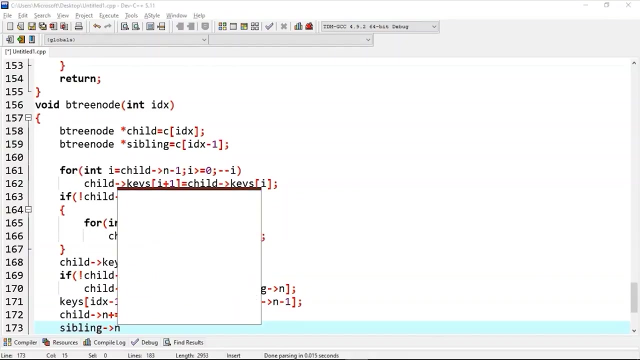 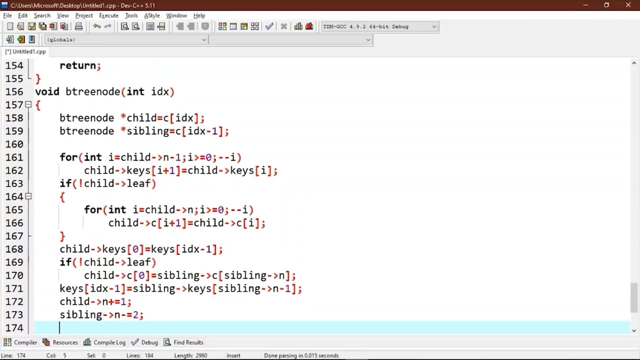 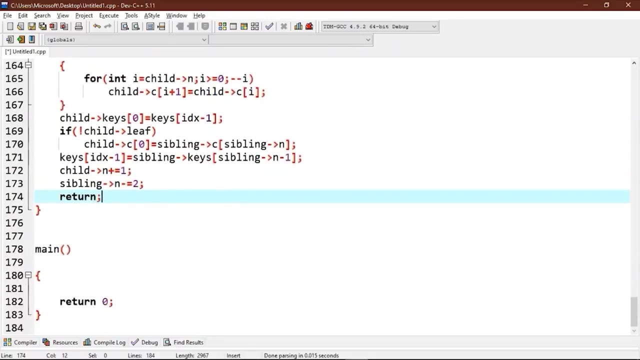 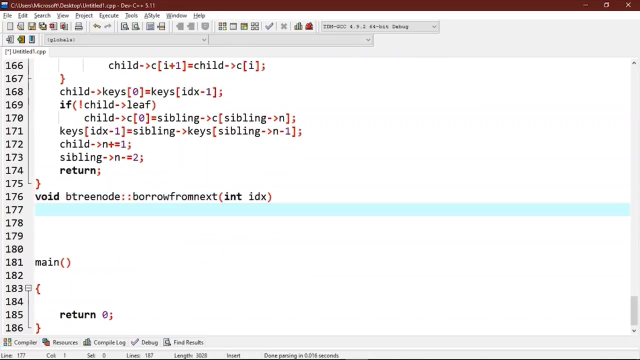 Now keys at id x minus 1 will be equals to sibling keys, sibling, all equals and minus one. now, child at n will be plus, equals to one and sibling and sibling will be equals to minus, equals to one. return void b, tree node and project and lichen. 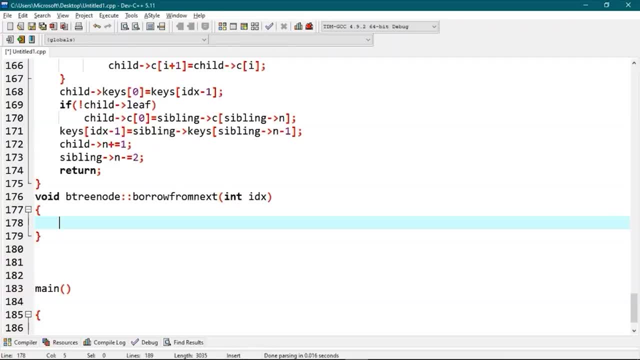 in presentation or in. Now. we will start by btree node child is equals to c at idx and btree node sibling is equals to c at idx plus 1.. Now key idx is inserted as the last key in the c idx. So child keys. 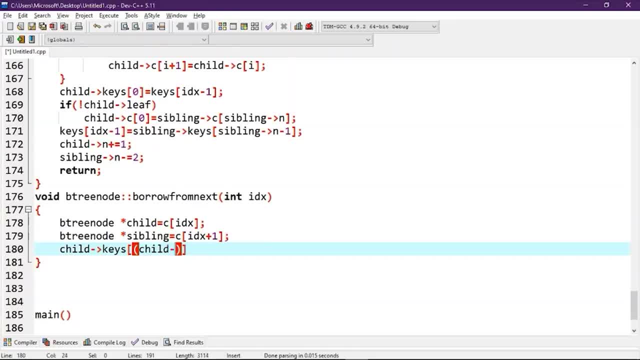 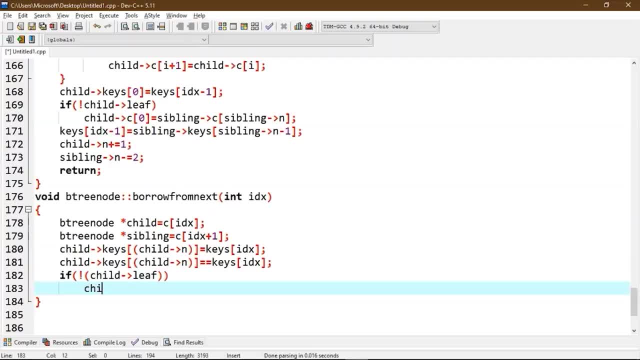 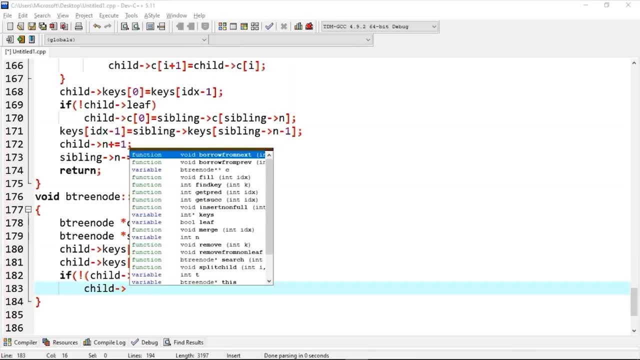 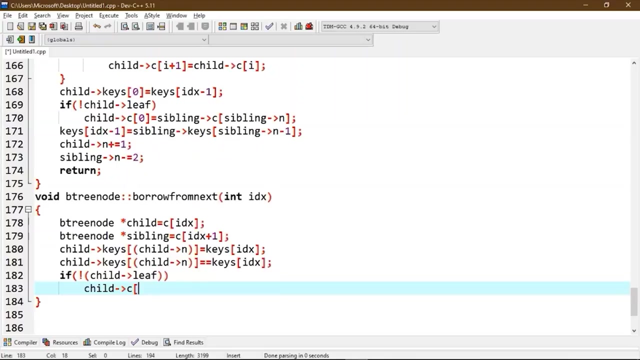 If child is live. Let's see Now. the first key from sibling is inserted into key IDX. So key at IDX Is it: I is equals to sibling, Key is 0 for loop and I is equals to 1.. I is equals to sibling. 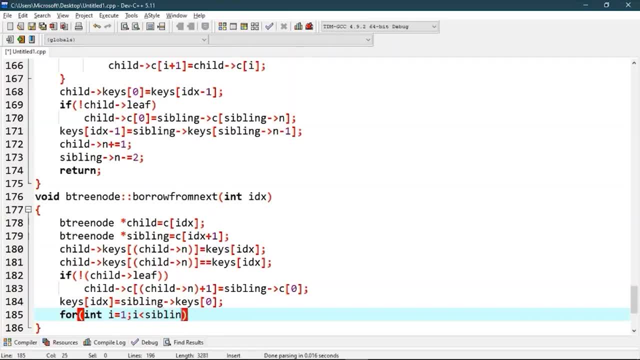 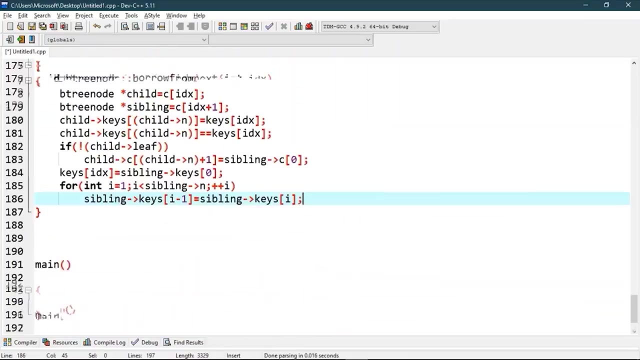 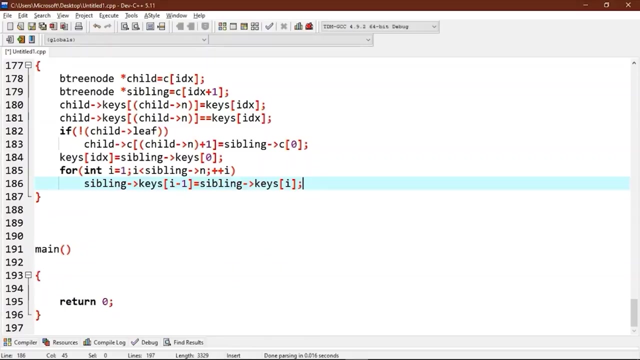 I less than sibling at N, plus plus I sibling, I minus 1.. I is equals to sibling Now, if sibling is not leaf, If sibling is not leaf, If sibling is not leaf, i equals to 1, then equals to sibling. calls n. 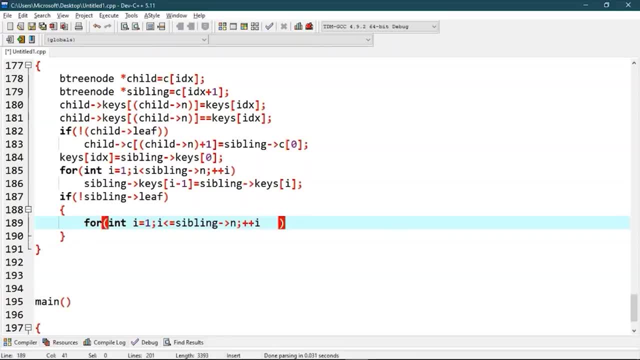 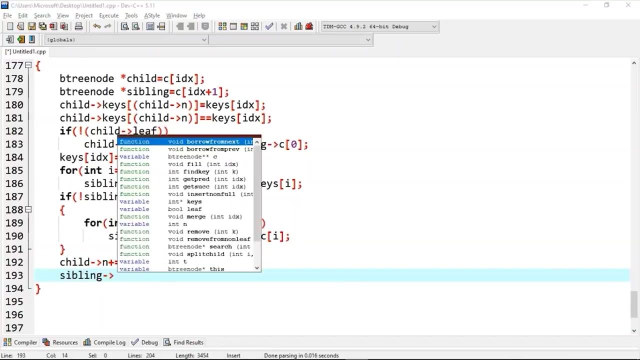 plus. plus i equals to sibling calls c at i-1 equals to sibling calls c at i. Now we will be increasing and decreasing the key count of CIDX and CIDX plus 1 respectively. So child at n is plus equals to 1.. Sibling calls n minus equals to 1.. 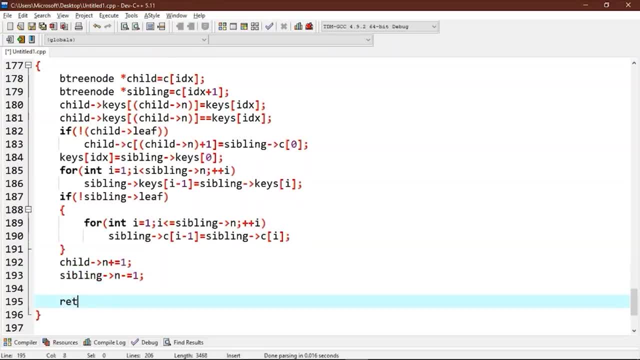 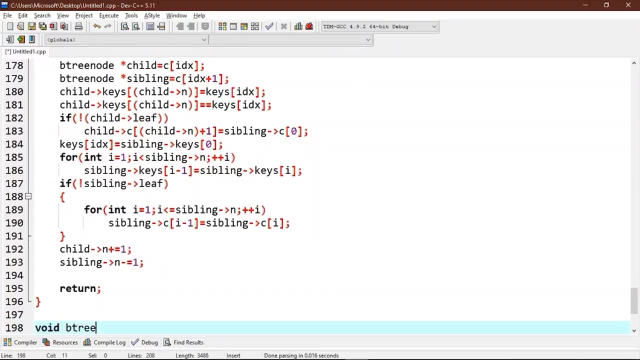 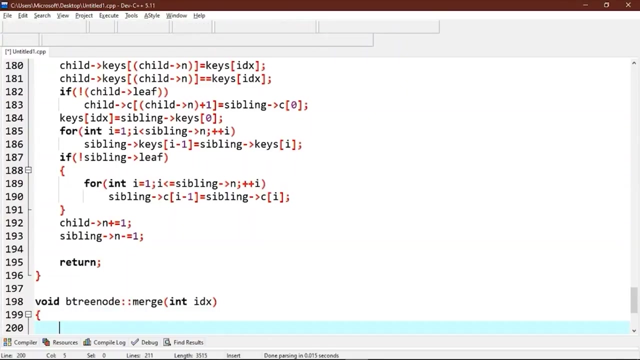 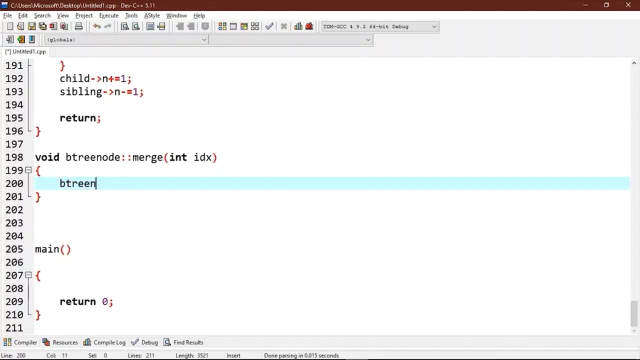 Return. Return Now. void: btree node merge with argument as int. idx. btree node star child is equals to CIDX. btree node- star sibling. btree node star sibling is equals to C at idx plus 1.. Now we will be pulling a key from the key node and inserting it at t minus 1th position in CIDX. 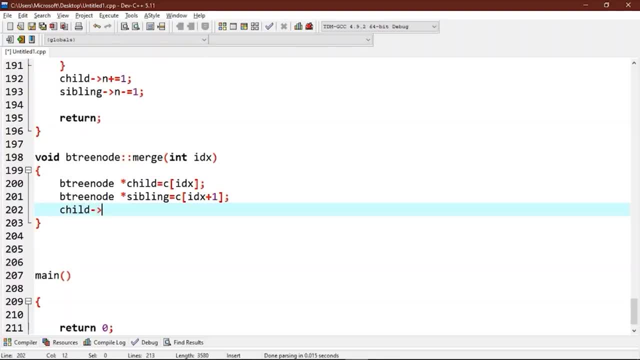 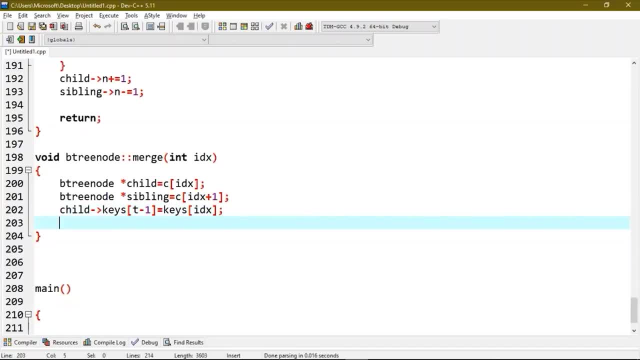 Now we will be copying keys from CIDX plus 1 to CIDX at the end. So for int, i is equals to 0, i less than c is equals to 0, iless than i, then sibling of n, and plus plus I. so 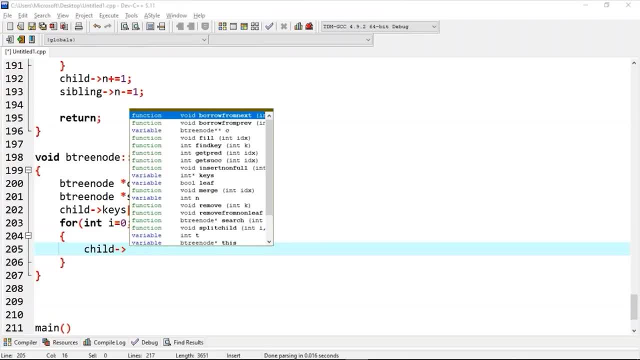 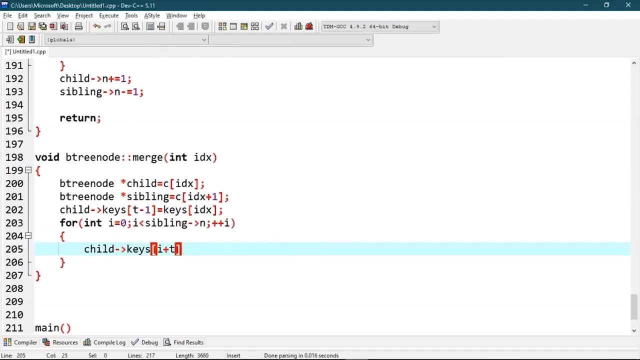 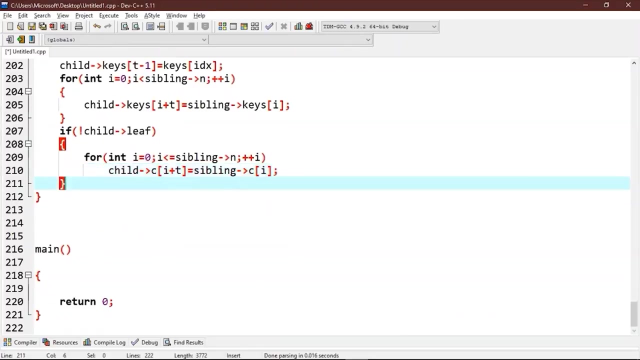 child. I plus T equals to sibling I. you. if our child calls leave for I, is equals to zero, I less than equals to sibling calls s plus I child. what's see record: I plus T was to sibling cause I. I I now for, and I is equals to IDX plus one. 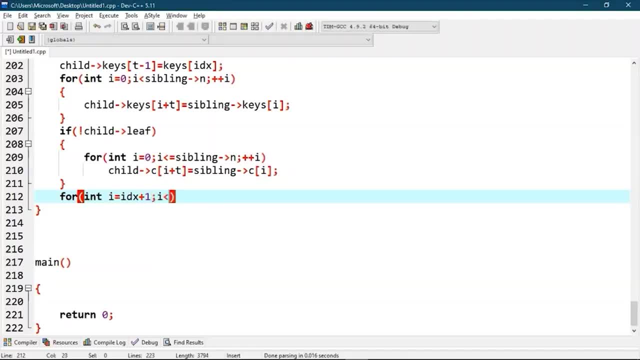 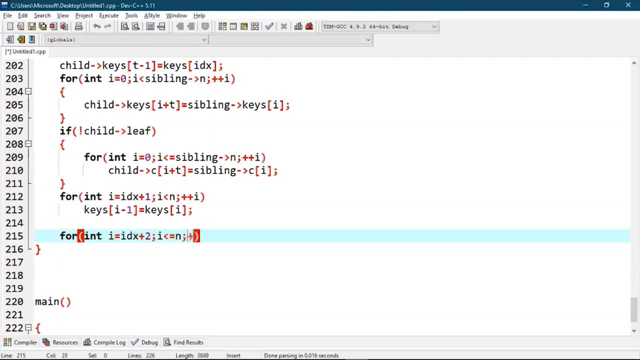 and plus plus i For int c at i minus 1 is equals to c at i. For int c at i is equals to idx plus 2, i less than equals to n and plus plus i For int c at i plus equals to c at i. 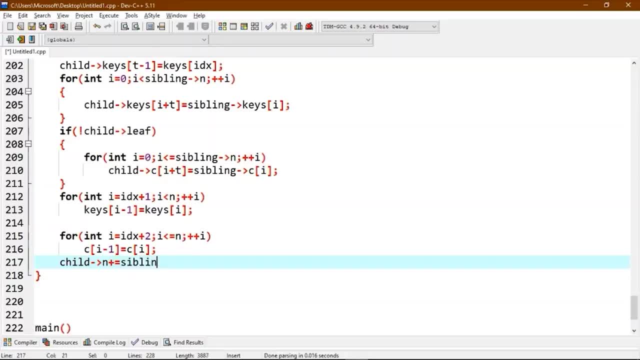 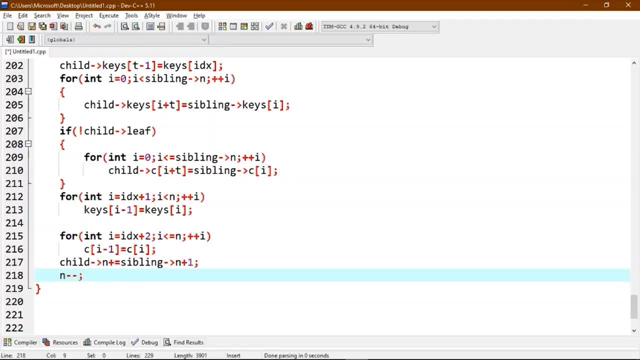 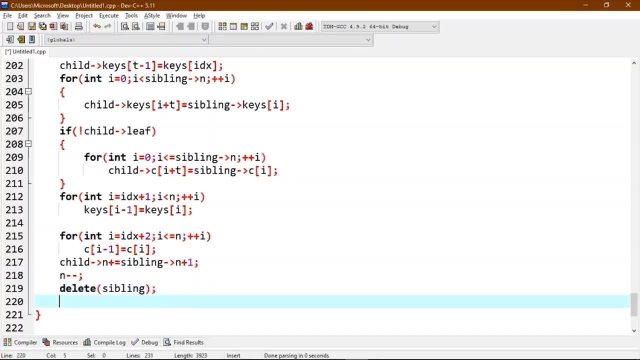 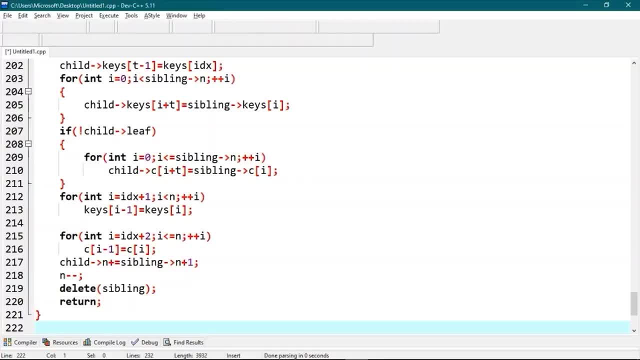 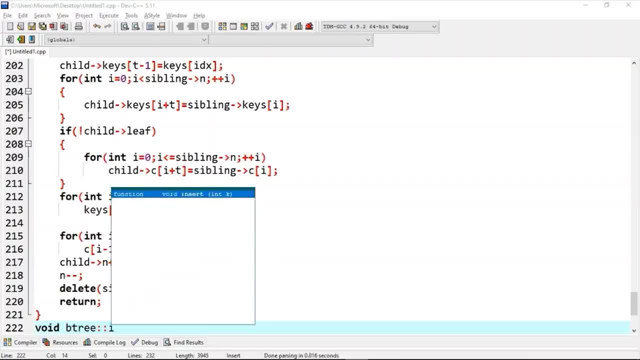 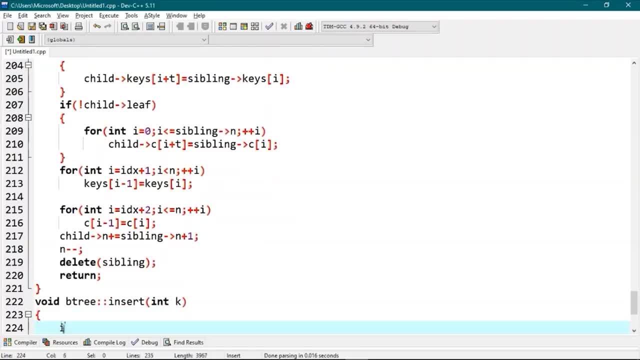 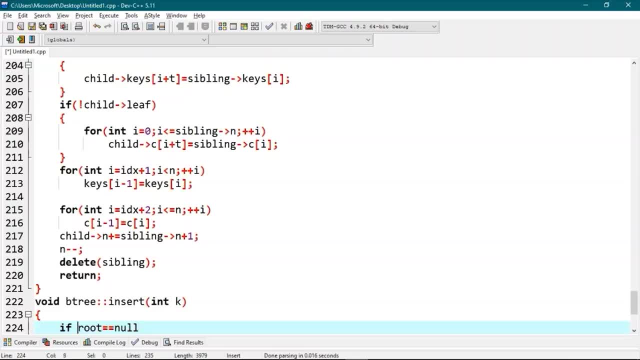 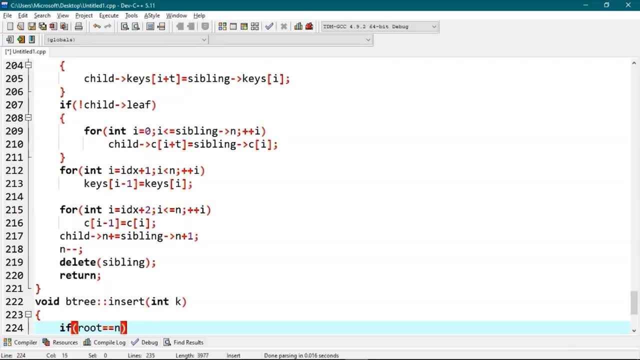 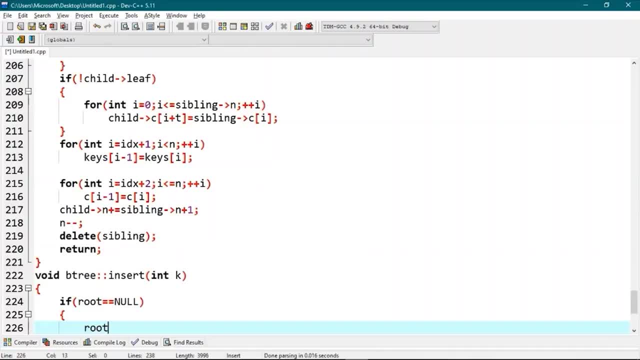 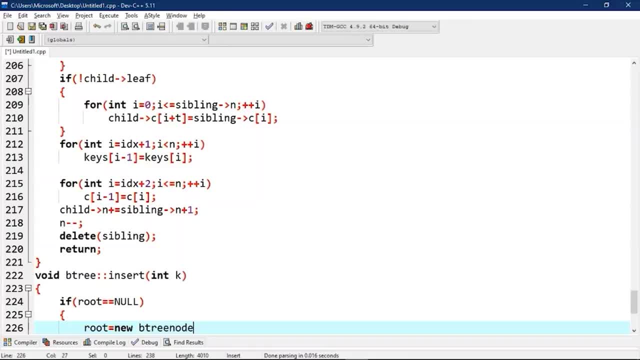 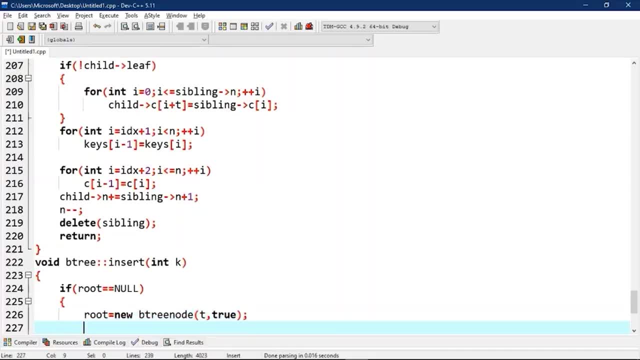 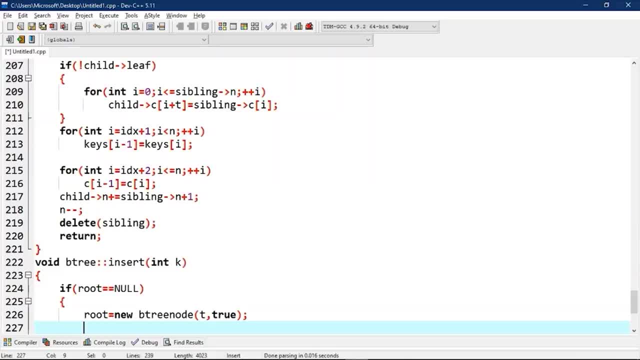 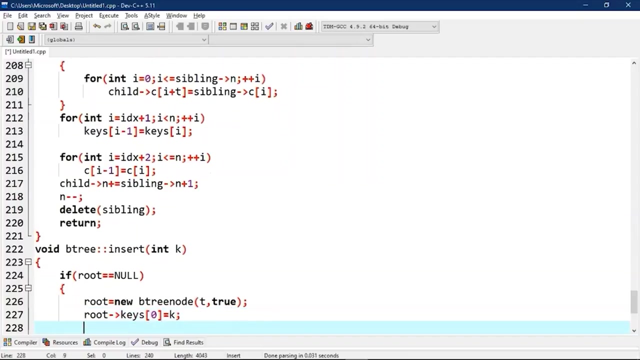 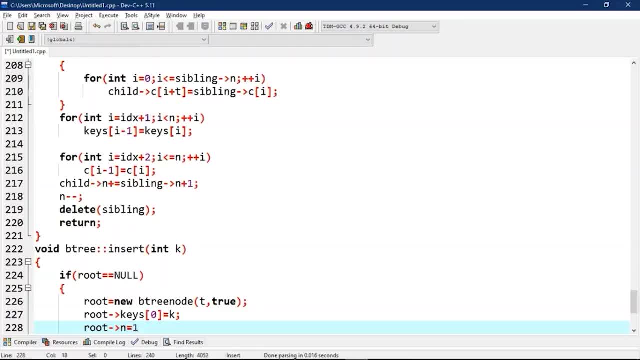 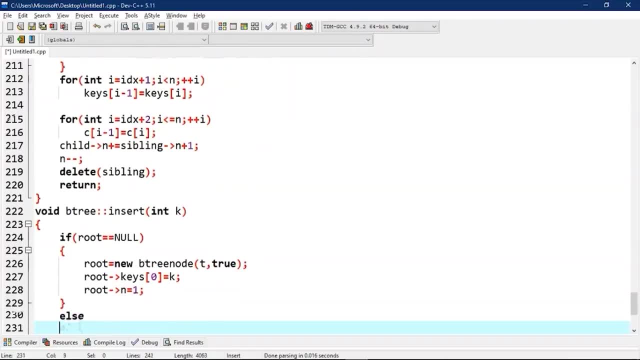 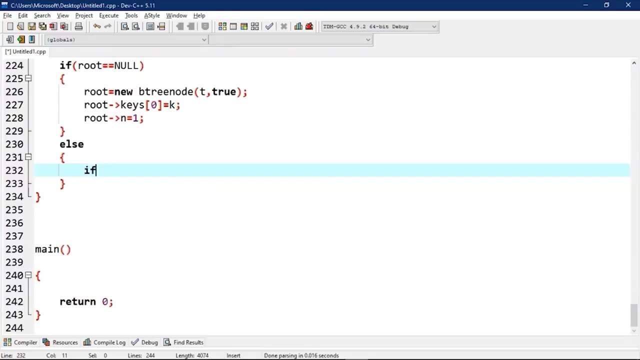 sun. else if root calls is equals to 2 star t minus 1. so btree node star s is equals to new btree node e comma false. now s c bracket 0 is equals to root s split side 0 comma root and i equals to 0. 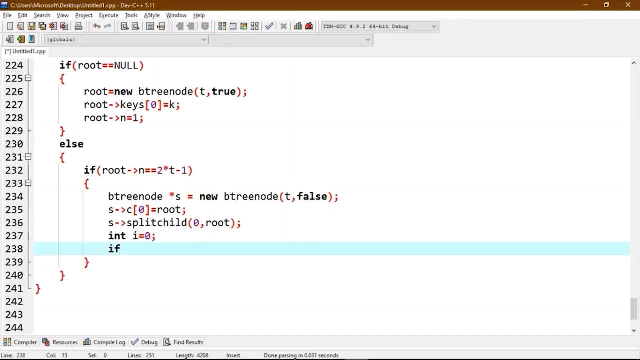 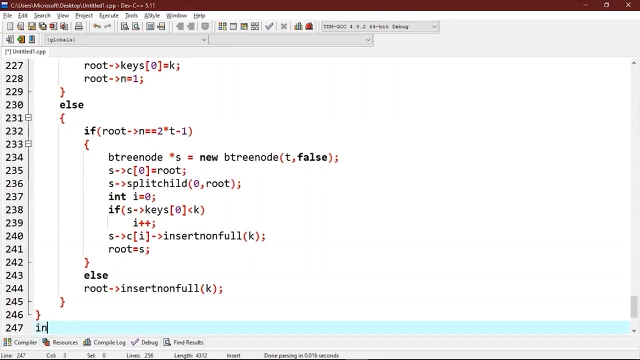 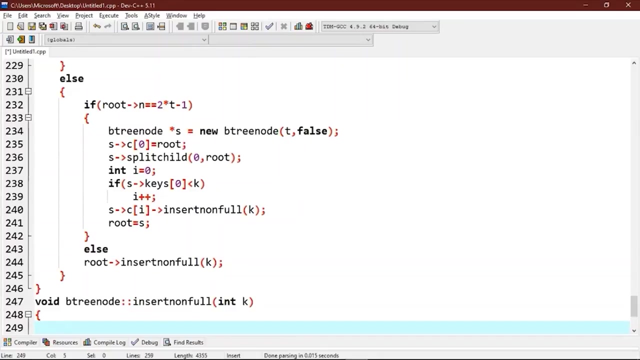 f s keys. bracket s s zero, less than K I plus plus s. see bracket I. insert nonpol K. now we will change the route to s else. root calls: insert nonpol at K, a utility function to insert at nonpol node. int I is equals to n minus 1 if leaf. 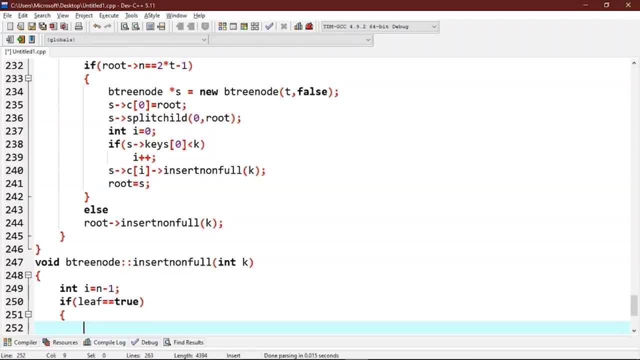 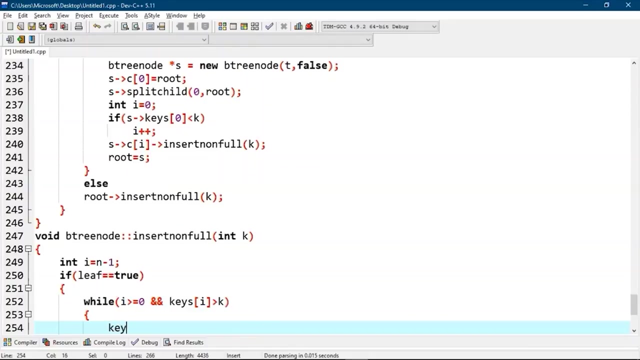 equals to true. the following loop does two things: finds the location of key to be inserted or moves all greater key to one place ahead. so while I is greater than equals to 0 and keys at I are greater than K, then keys at I plus 1 will be equals to keys. 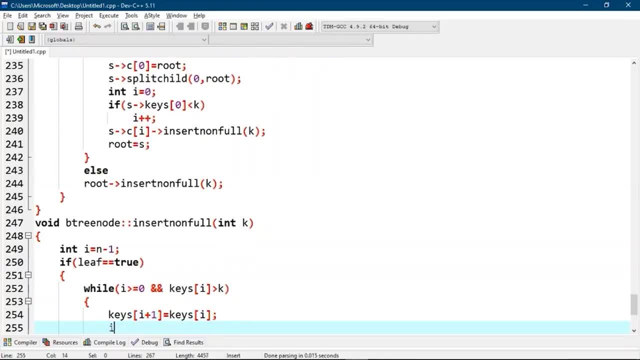 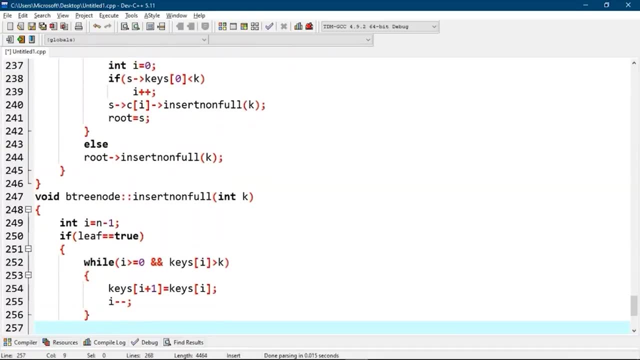 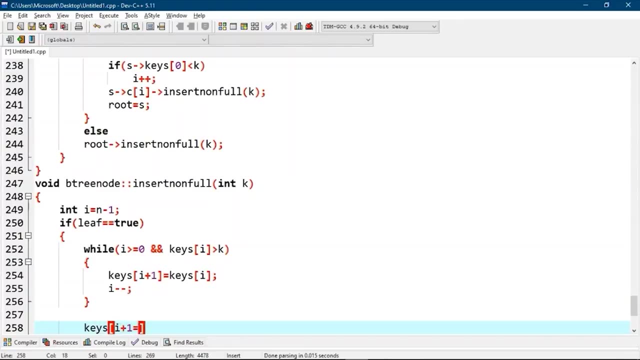 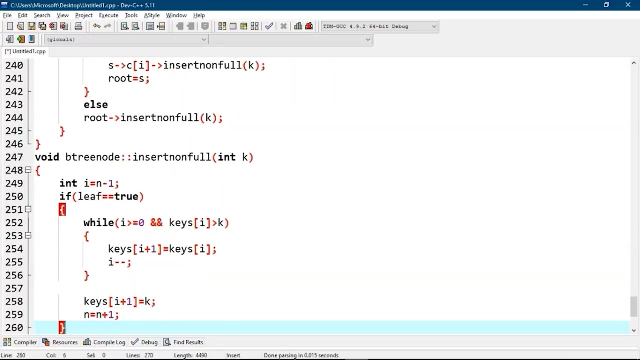 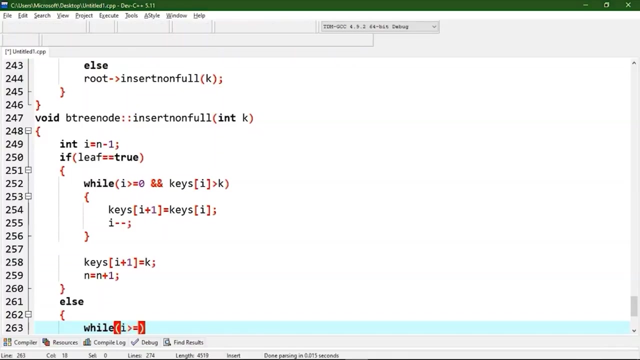 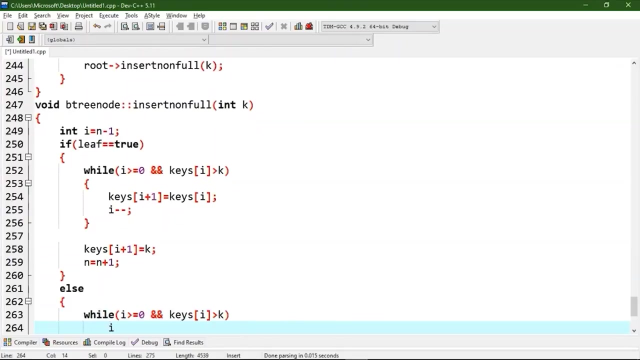 at I and I minus-minus, keys at I plus one will be equals to A and n will be equals to n plus 1, and keys and I will be equals to A once and else, while i is greater than equals to 0 and is at i greater than k, i minus minus. 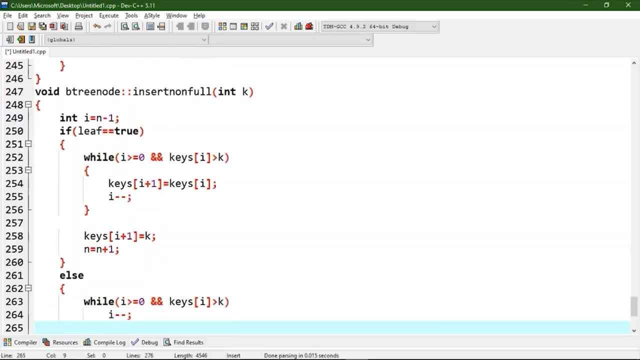 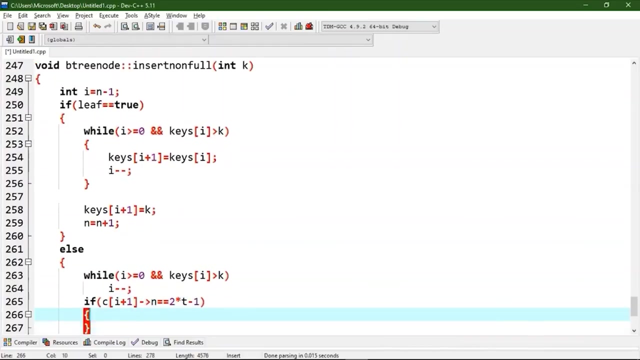 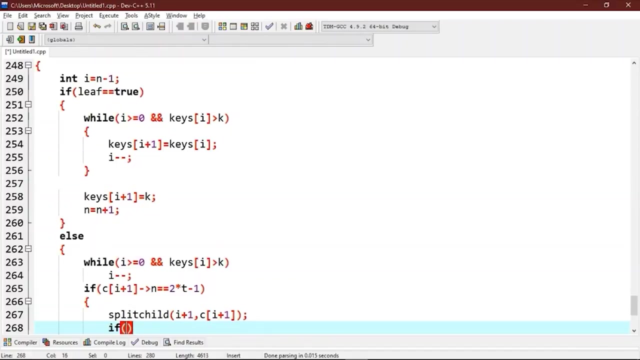 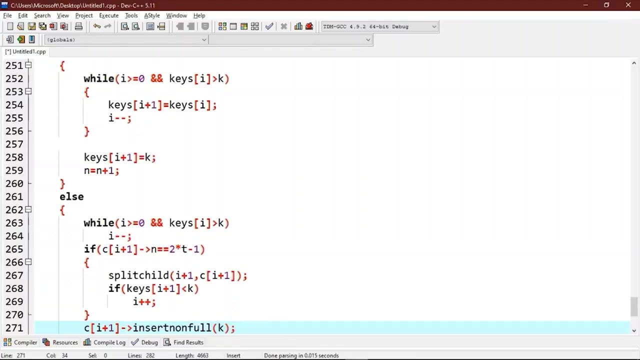 f. c bracket i plus 1 at n equals to 2 star t minus 1 child. i plus 1 comma c. i plus 1. f is bracket i plus 1. k. i plus plus c bracket i plus 1. insert non-full k void. 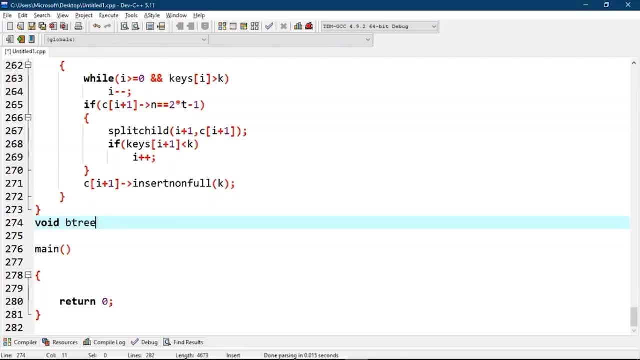 b3 node int i comma. b3 node star y. b3 node star z is equals to new b3 node argument as y calls t is equal to b3 node argument as y calls t is equal to b3 node argument as y calls t argument as y calls t. 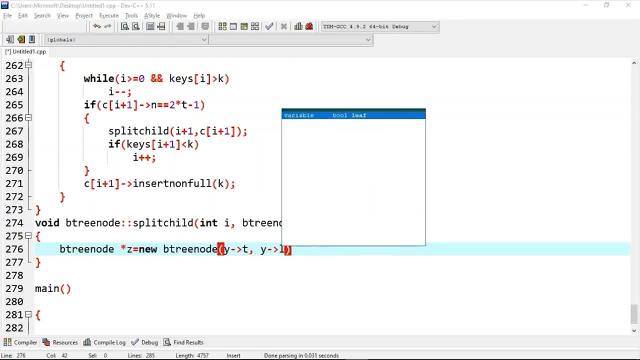 and y calls: leave now. z calls n equals to t-1. now we will copy the last t-1 keys of y to z. so for loop int: j is equal to 0, j less than t-1, j++. so z keys: j is equals to y at keys. 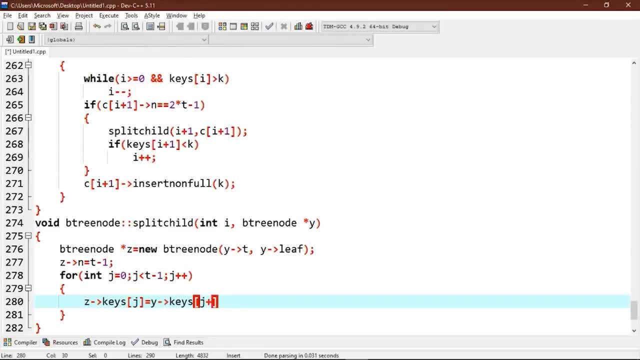 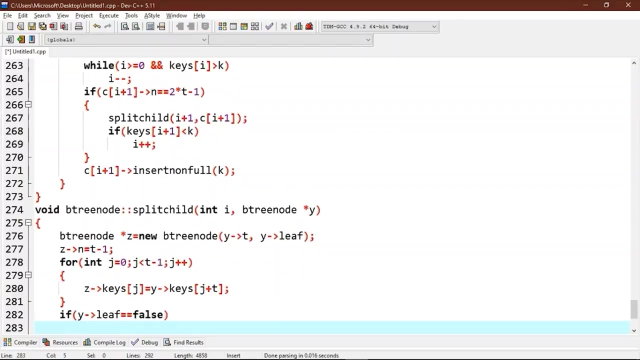 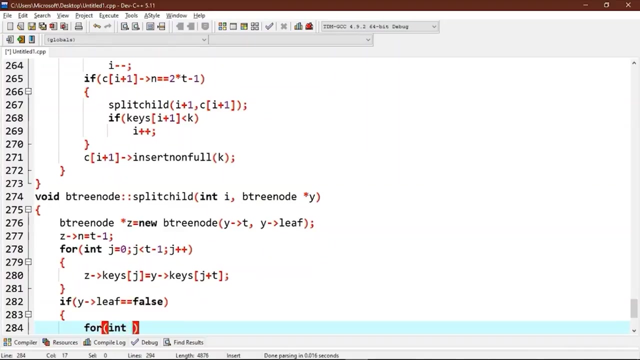 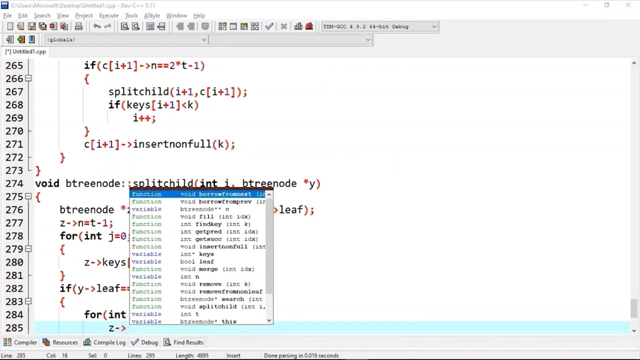 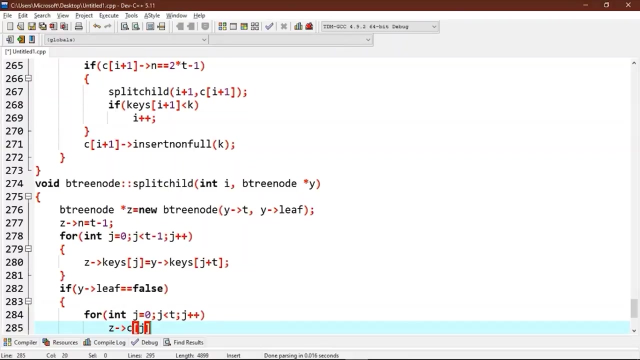 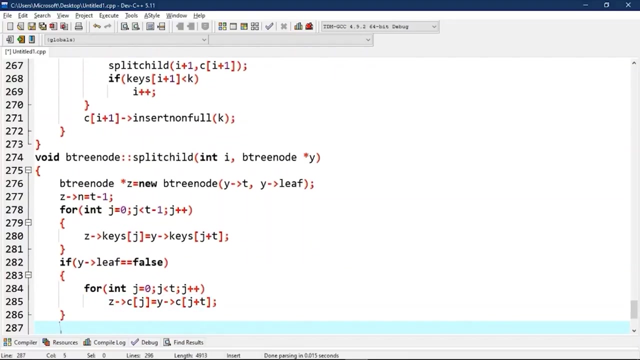 j plus t. so if y, if equals to, calls 0 for int, j is equals to 0, j less than t, j++ j, c bracket i is equals to y, calls c bracket j plus e. now, y, calls n, equals to t-1. now, since this node is going to have a new child, 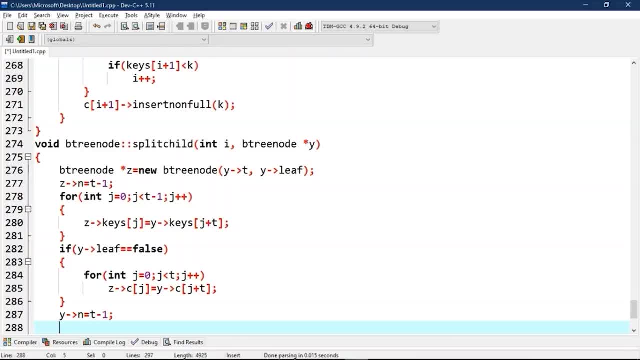 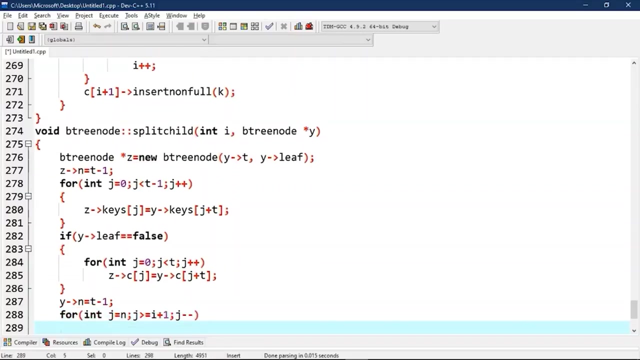 we will create space for the new child. so for loop int j is equals to n. j greater than equals to i plus 1. j minus minus c. greater than equals to i plus 1. j minus minus c. greater than equals to i plus 1. C bracket J plus 1 equals to C bracket J. 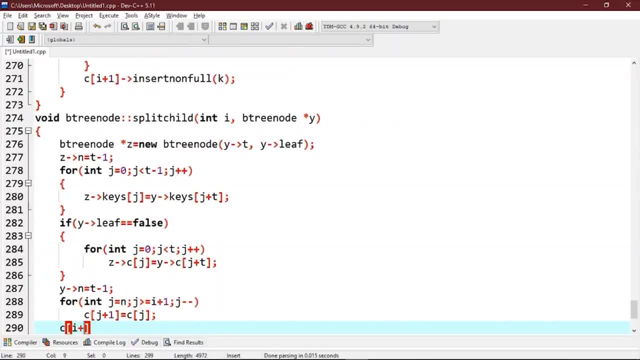 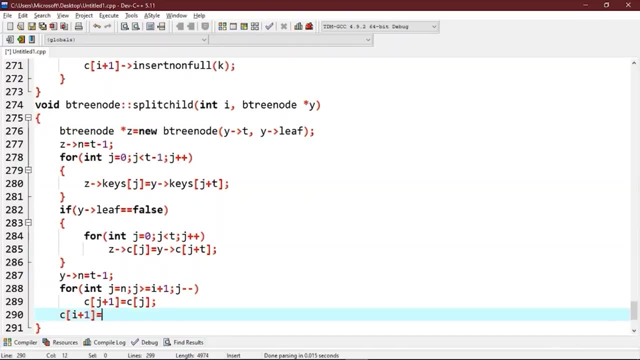 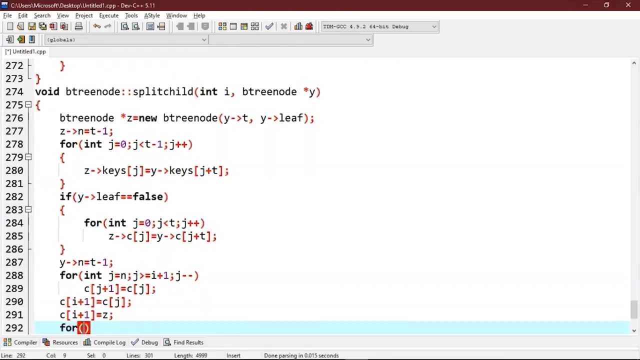 of C bracket I plus 1 is equals to C bracket. J of C bracket I plus 1 Is equals to Z For loop, and j is equal to N minus 1 J greater than equals to i. j minus minus 2 minus 1 j greater than equals to i j. 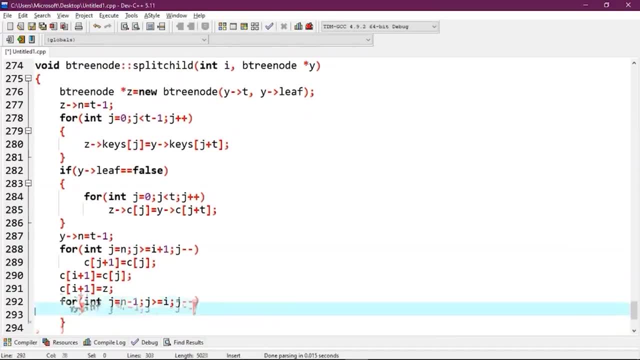 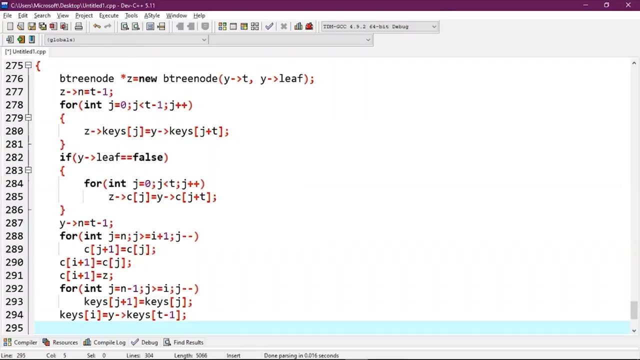 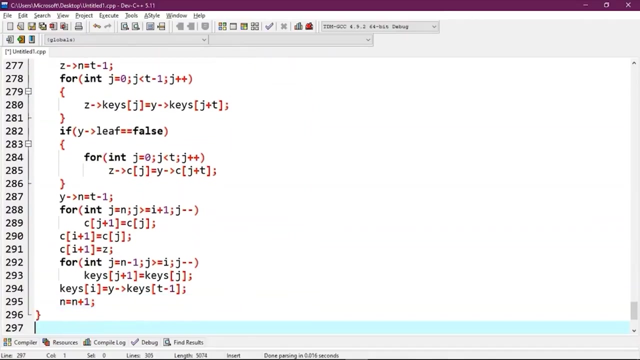 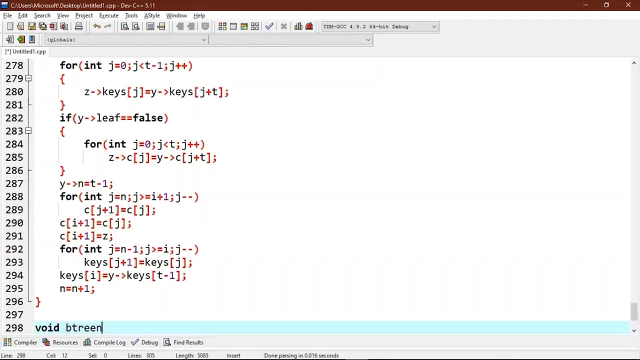 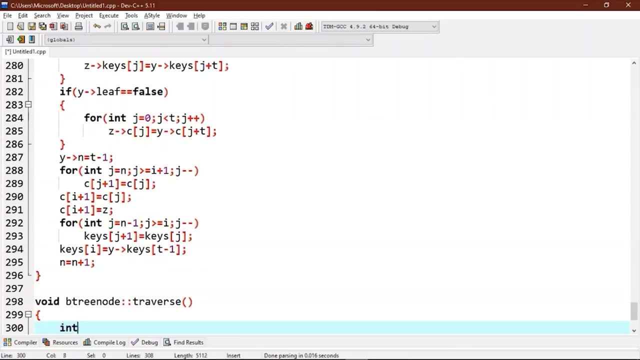 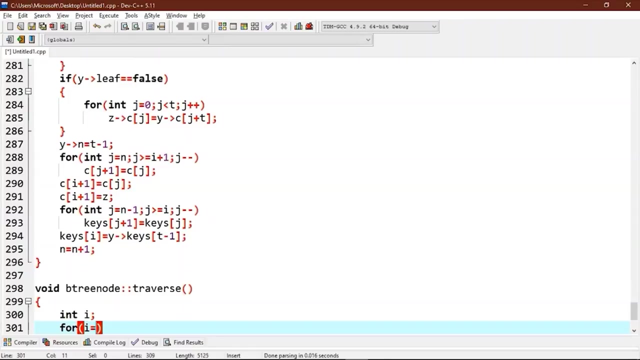 is bracket J plus 1 equals to keys at J, is I equals to Y, is bracket T minus 1 and is equals to n plus 1. now we will write function for traverse. so void B, tree node, traverse and I for loop. I is equal to 0, I less. 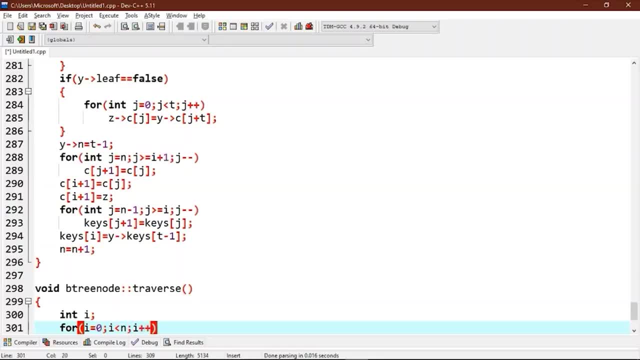 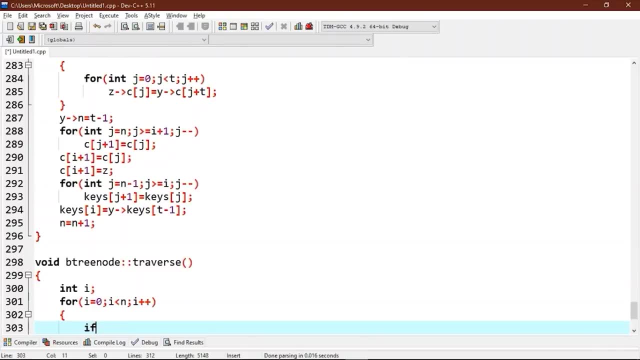 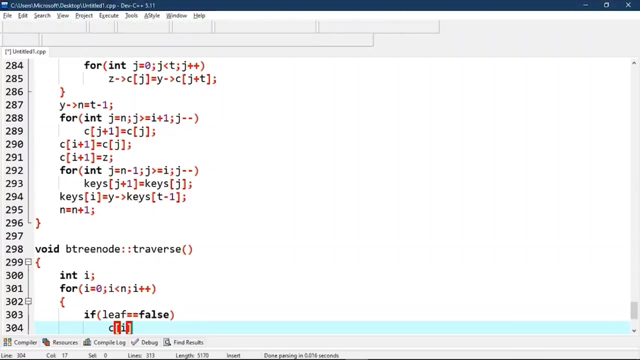 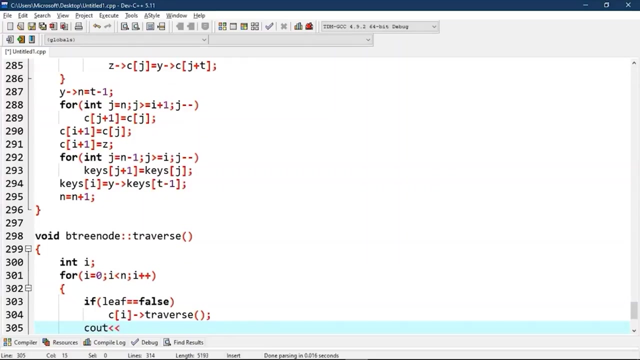 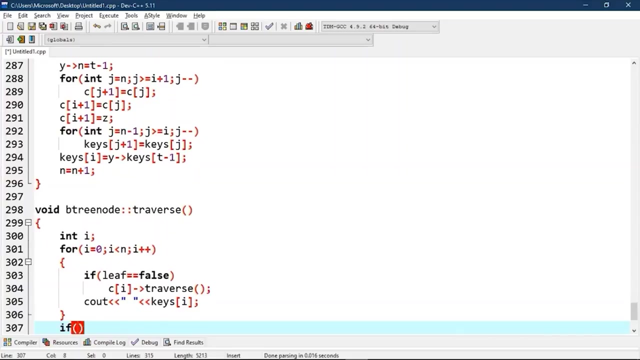 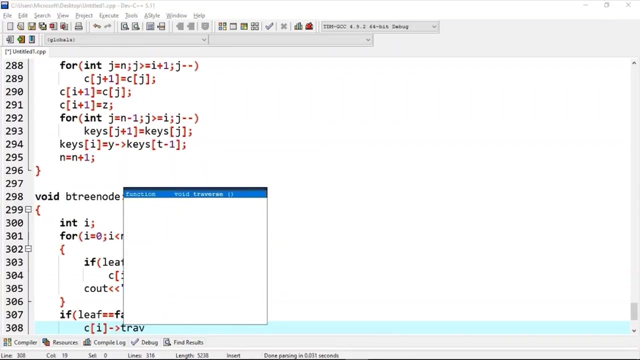 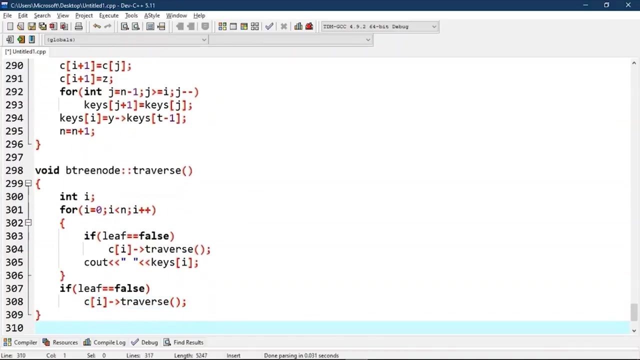 than n, I plus plus. if leaf equals to false and see bracket, I will traverse you. if if is equals to false and see, I will call this function. if if is equals to false and see, I will call this function. will pose traverse function. now we will write the function to search. 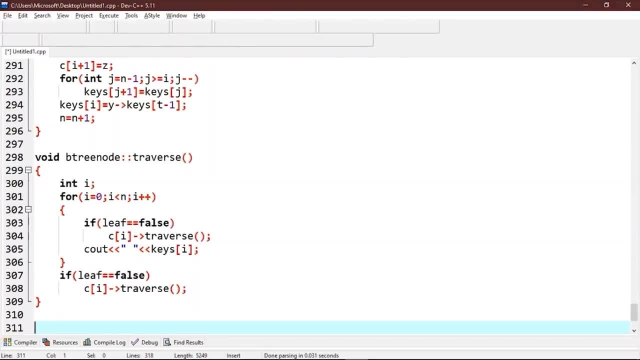 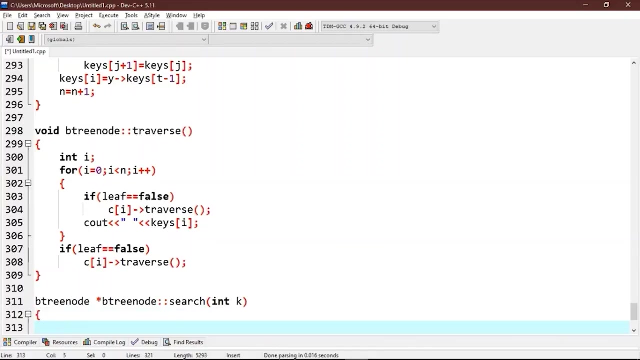 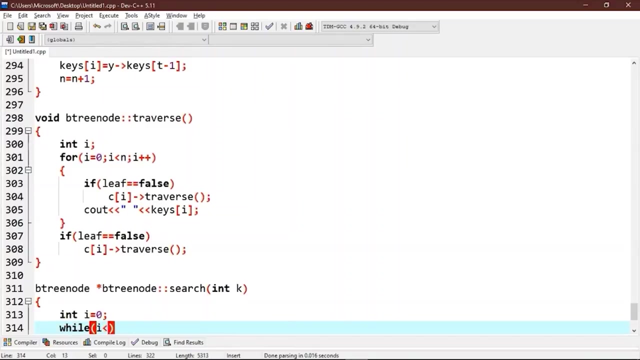 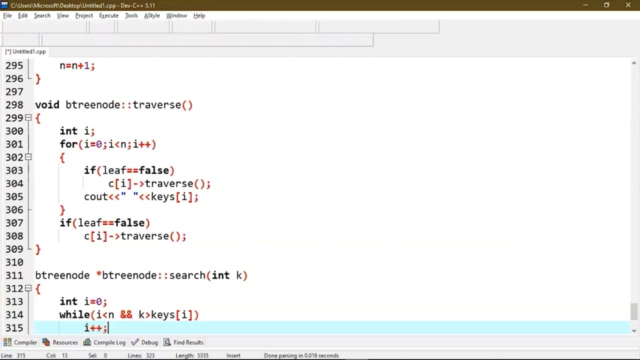 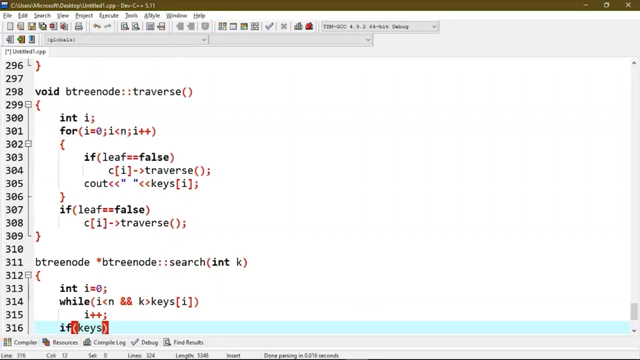 key in the subtree routed with this node for be tree, node star B tree. Now search int k. int i is equal to 0, while i is less than n. Now if m% k is greater than keys i, i++. Now if keys i is equal to k, i++. 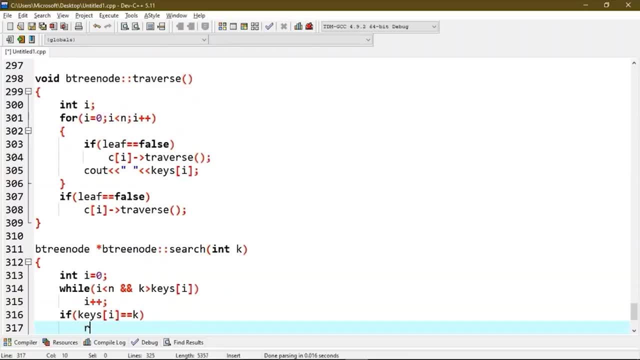 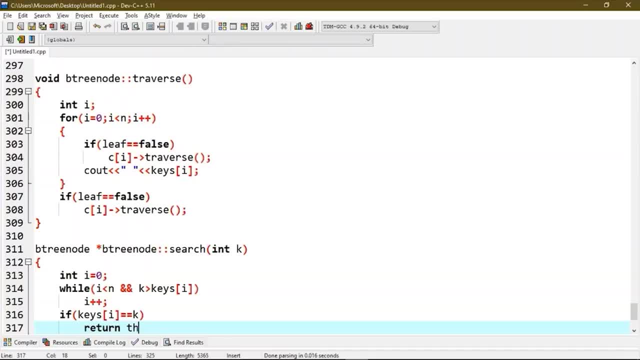 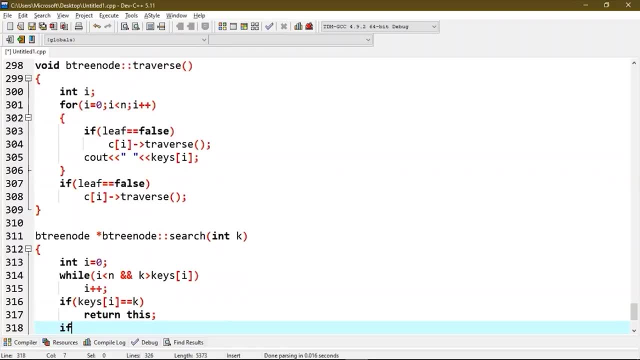 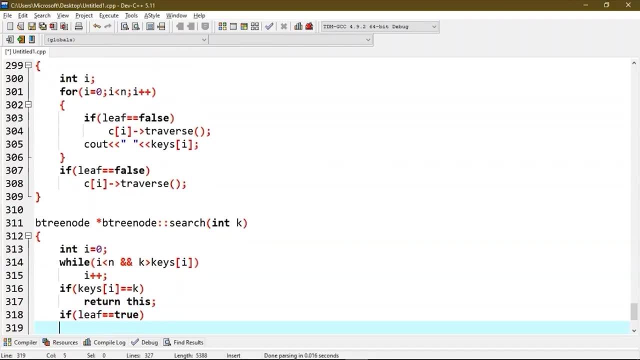 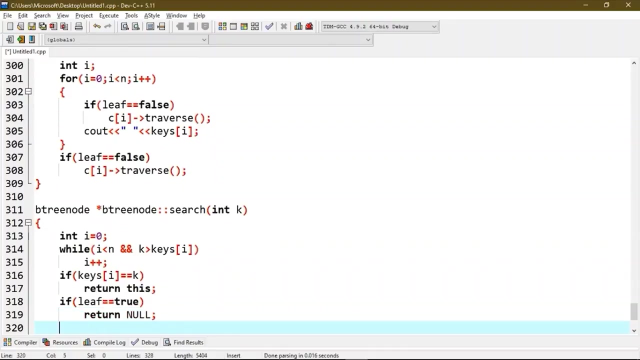 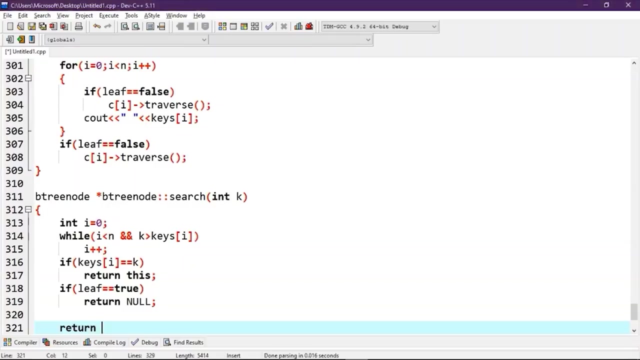 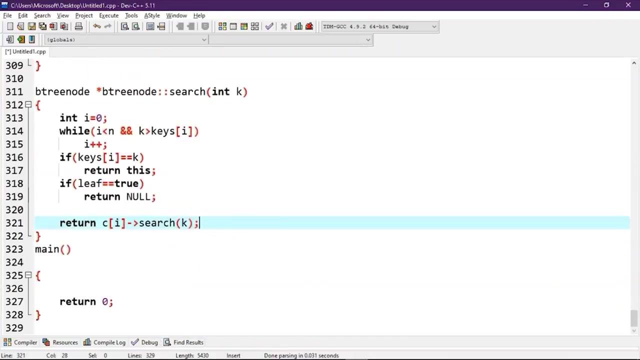 Now return this. Now, if Keith is equal to true, Then return null, otherwise return c bracket. i calls search for k. now we will write the utility function to remove. so void e tree. remove int, k, f, not root, and c out. the tree is empty. 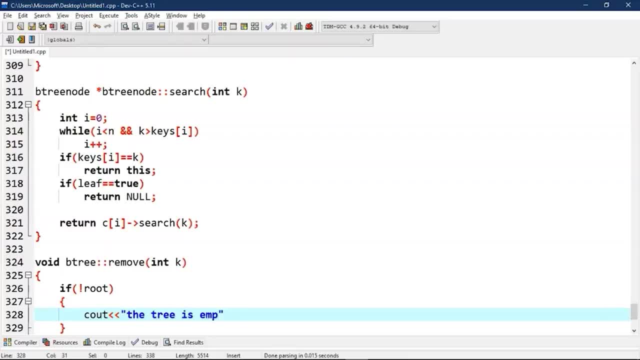 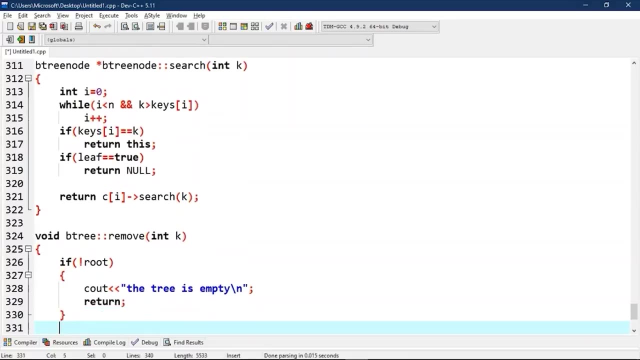 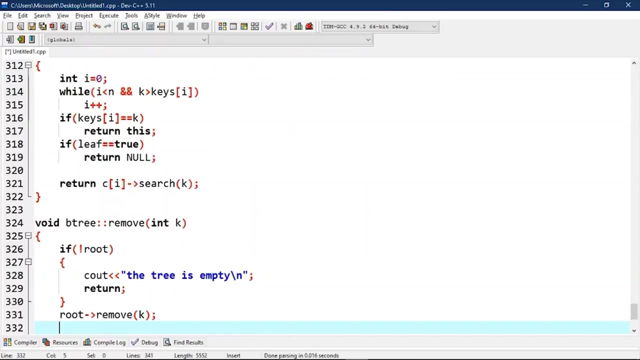 return. return. now we will call the reboot. repeat. then will we call the remove function for root. so for pudding root, call remove k. now. if root has zero keys, then we will make it's first child as a new root. if it has a child otherwise, which it says, 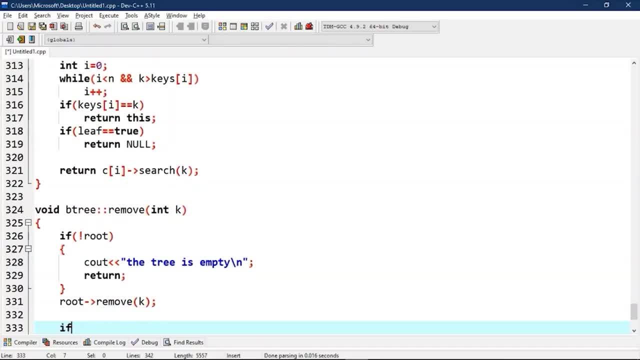 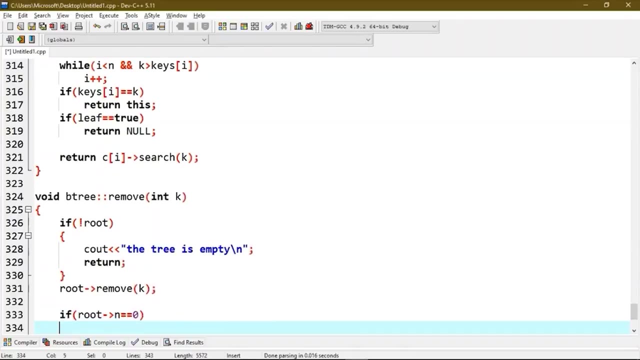 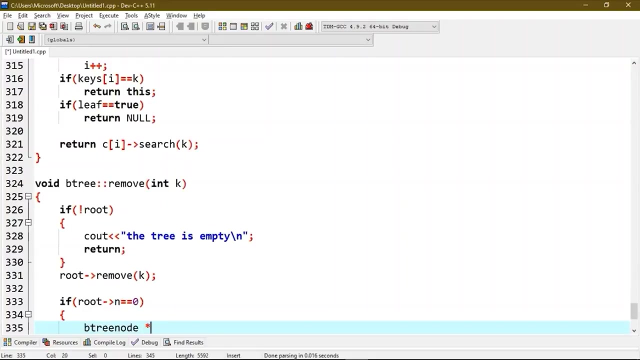 root as null. if root has zero keys, then will we calls it's is an old child title. if a child is aAGKthen we calls the root as new root, then will we calls for kão ngute. so if root n is equals to zero, then btree, node, star, tmp equals to root. 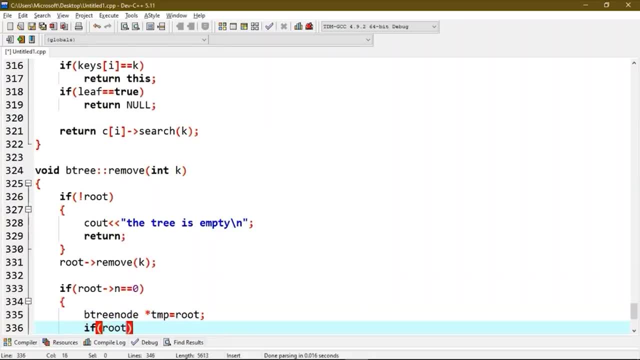 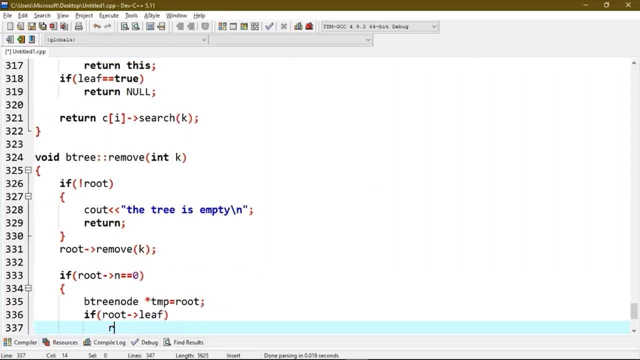 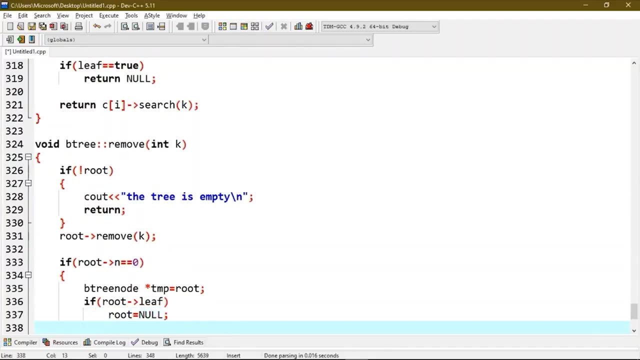 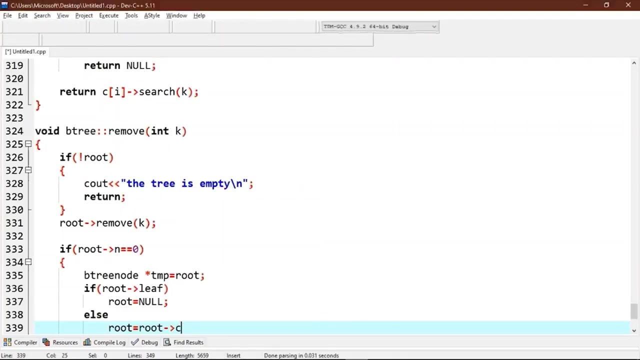 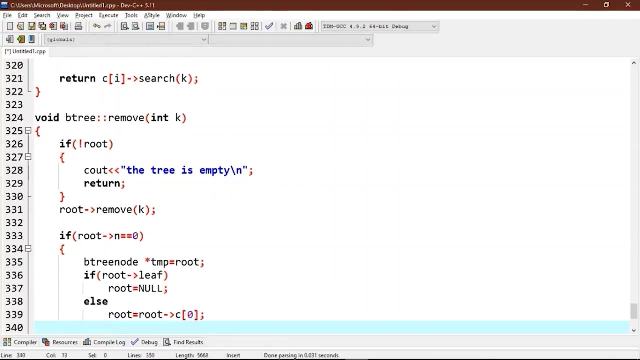 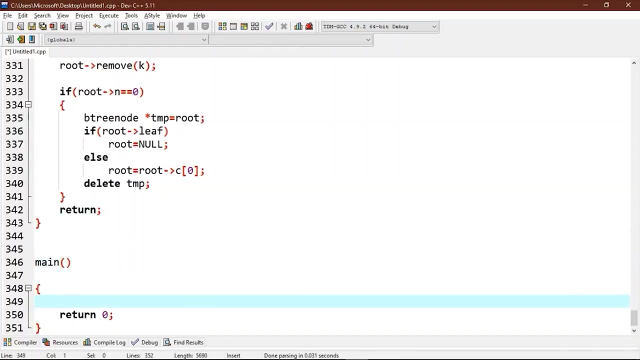 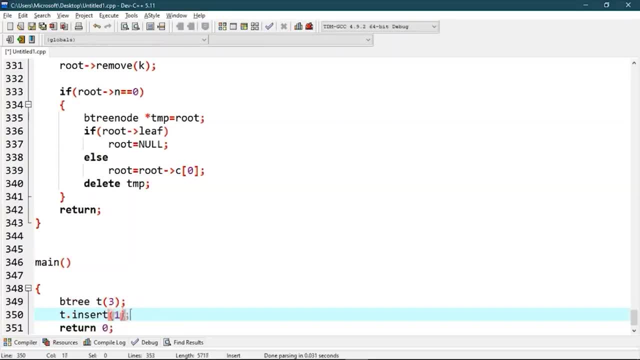 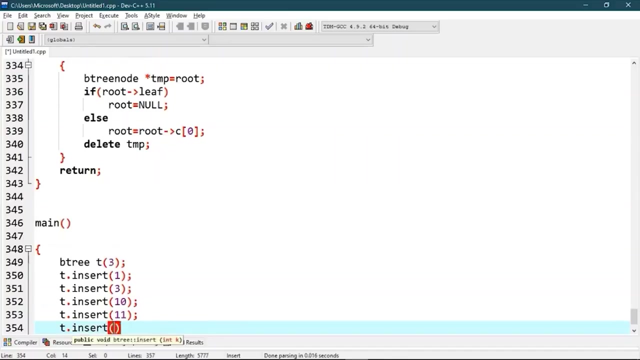 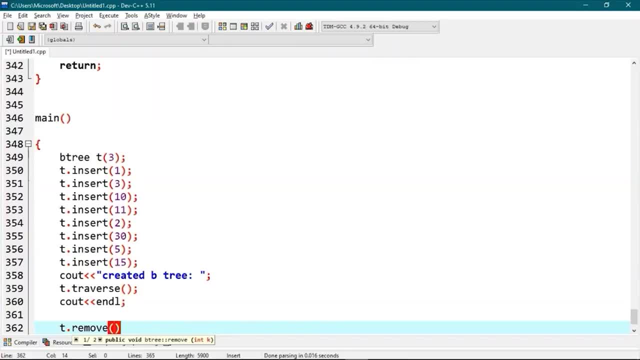 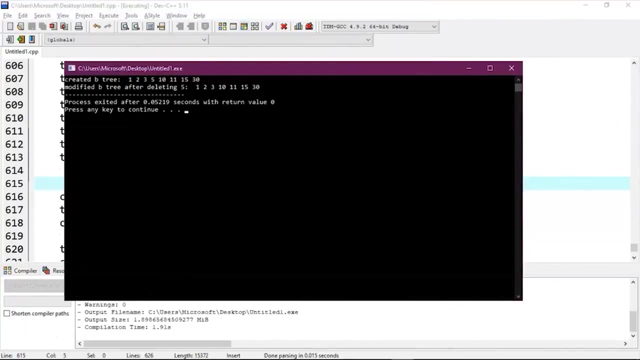 Now we will use tremove To remove 5.. Now see out Modified t tree after deleting 5. ttraverse: As you can see, we have successfully deleted 5 from our b tree. Let's get back to our slides. 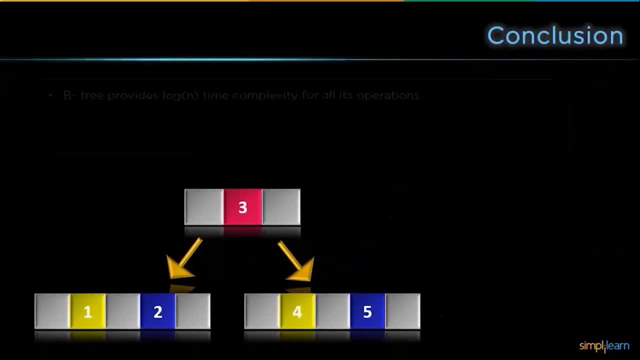 At last. let's sum up what we have learned. Let's sum up what we have learned. Let's sum up what we have learned In this session. first up, all the operations on b tree have time. complexities of log n. Next, all the leaves must be on the same level. 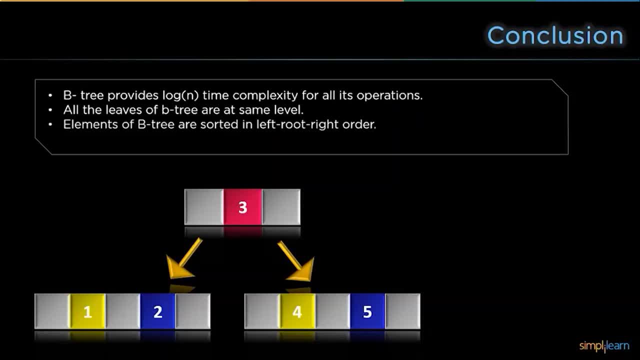 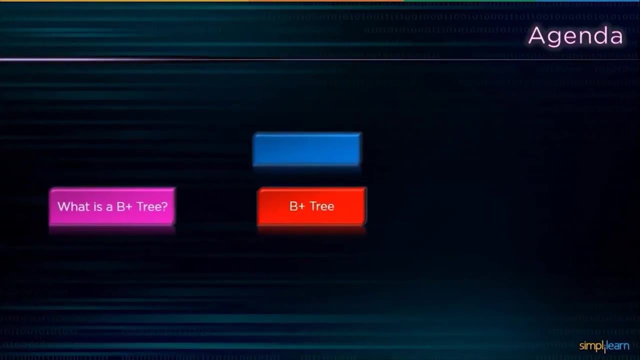 Next elements of b tree are sorted in ascending order from left to right. Finally, every node contains one more pointer than the number of elements of the node, b plus trees. We shall begin by introducing b plus trees, Then we will discuss properties. 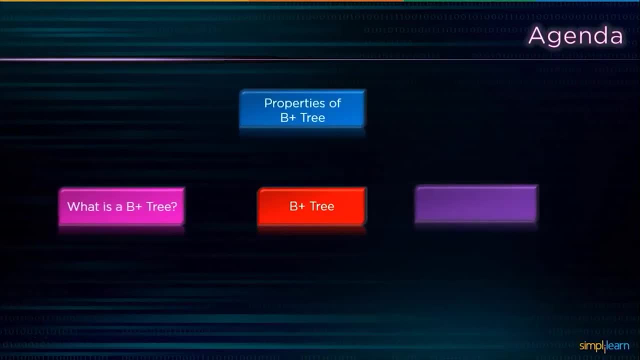 B plus. trees are an optional tree and there is an undetermined number, but there are some other properties that we want to talk about. First and foremost, we will try various operations on them, like insertion and deletion. Finally, we will sum up what we have learned from this session. 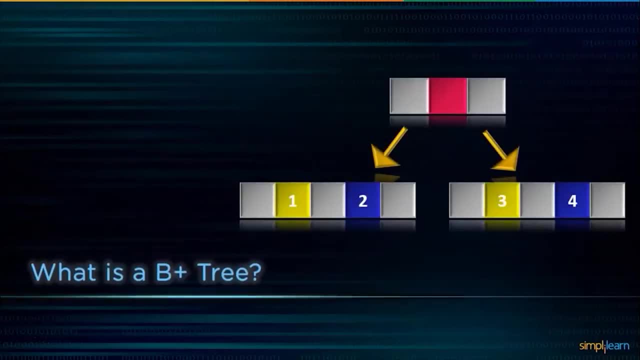 Finally, we will sum up what we have learned from this session. Before we begin, make sure you have subscribed to our YouTube channel and clicked on the bell icon to never miss an update from SimplyLearn. So, without any further ado, let's get started with what is a b plus tree. 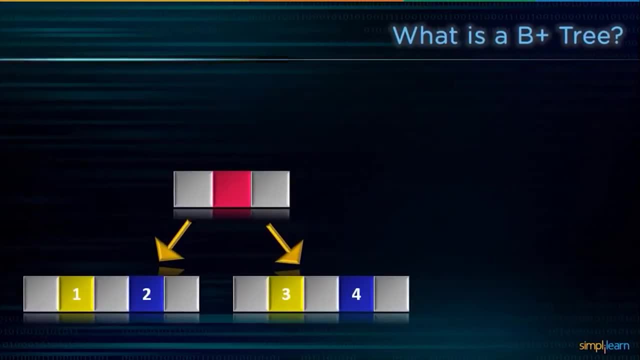 Let's get started with. what is a b plus tree? A b plus tree is, as explained in the previous slide, a special m-way tree data structure which makes it copocks value as if nobody wants it. but f is for all. now you can use tree. 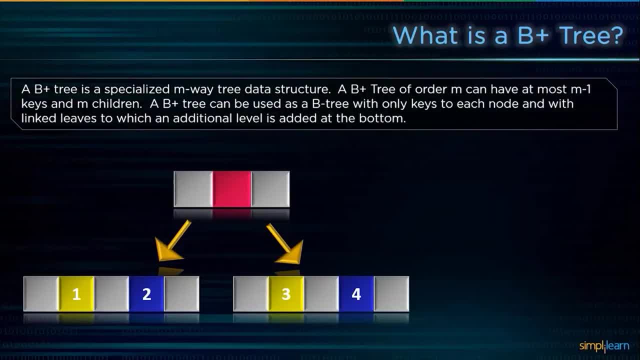 that loves trees. b plus trees have two categories: data structure: a, B plus tree of order m can have at most m-1 keys and m children. A B plus tree can be used as B tree with only keys to each node and with linked leaves to which an additional 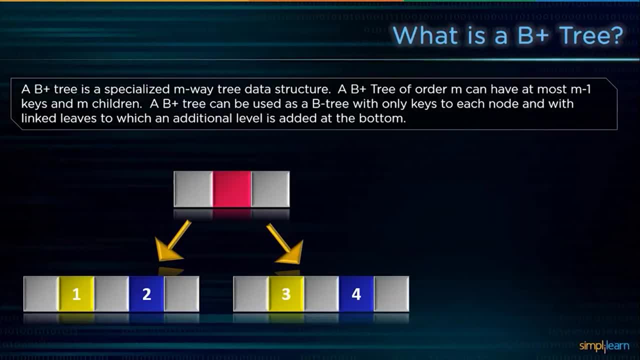 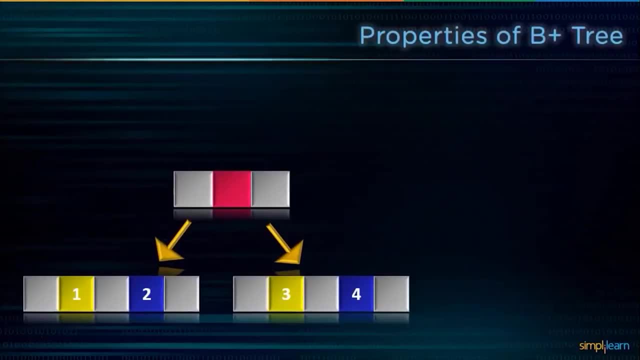 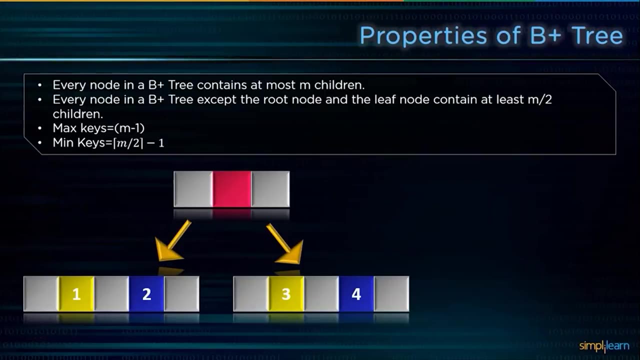 level is added at the bottom. Now let's discuss some properties of B plus trees. First up, every node in B plus tree can have at most m elements. Next, every node except the root and the leaf node must have m by 2 children. Next, maximum keys for any node is m minus 1.. 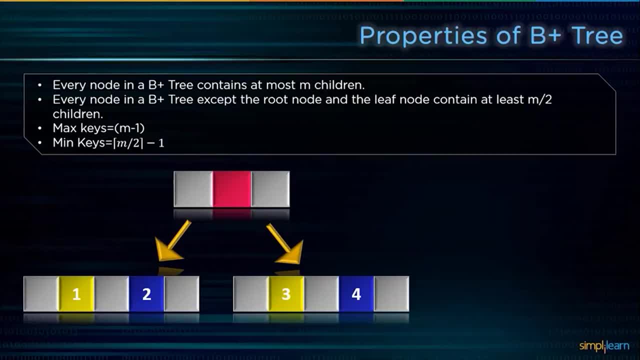 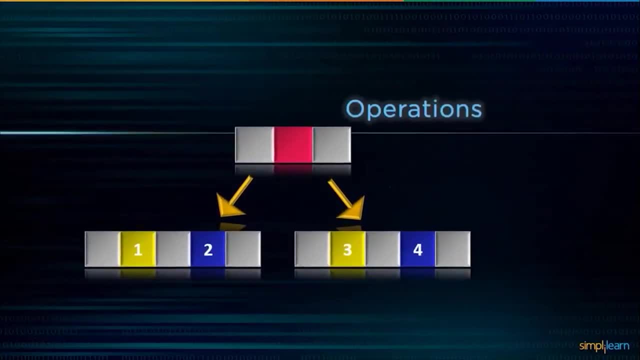 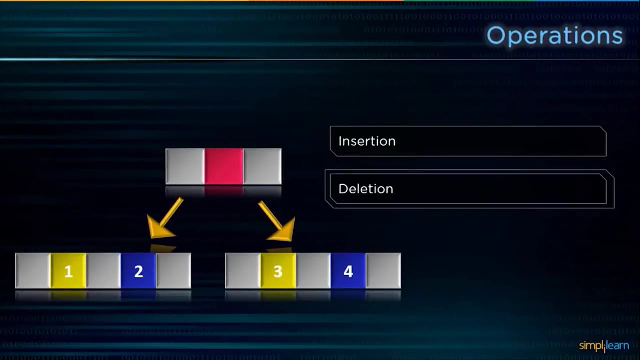 And at the last, minimum keys for any node is ceiling of m by 2 minus 1.. Now let's discuss what are the various operations we can perform on B plus tree. We can perform two operations on a B plus tree: First, up insertion, Second, deletion. Now let's discuss these in detail. 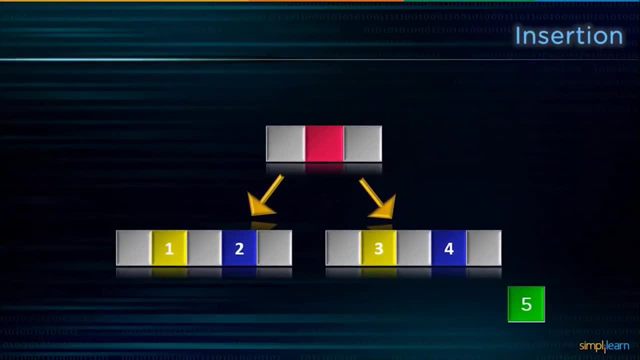 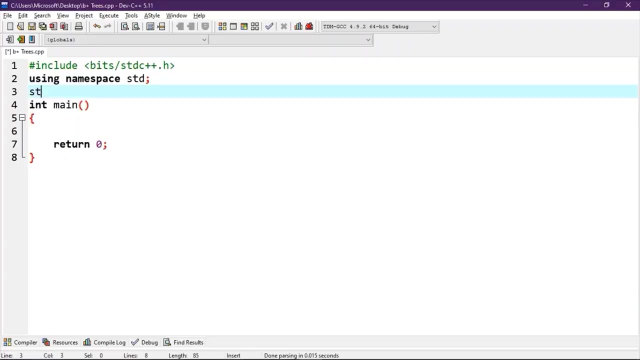 First up, insertion. We have to insert an element in such a way so that we won't disavow any properties of B plus trees. Now let's try this operation in a code editor. We will start by creating a node. To create a node, we need a struct. 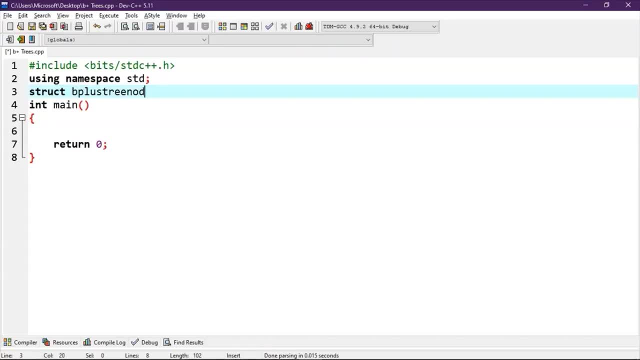 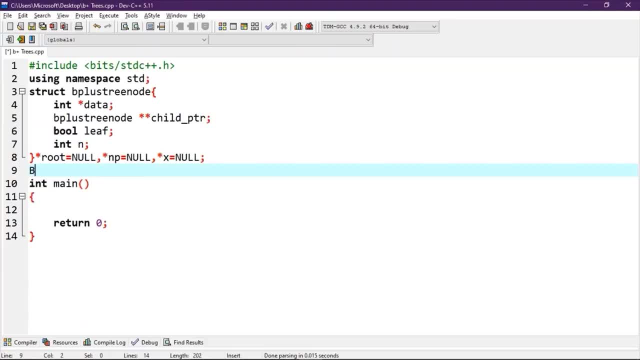 now we will write a constructor for it, so be free. node star in it. and i and p equals to new b plus tree node and p arrow data is equals to new space and bracket 5 and then p, child ptr is equals to new b plus tree node. 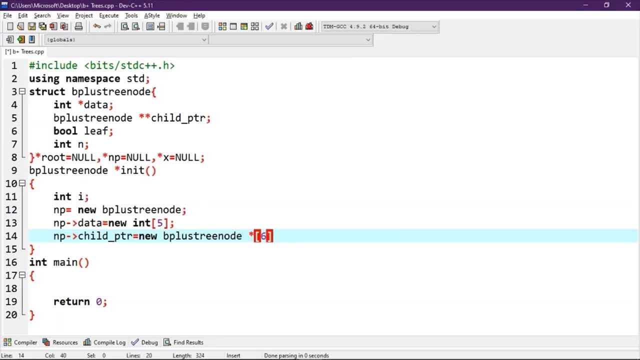 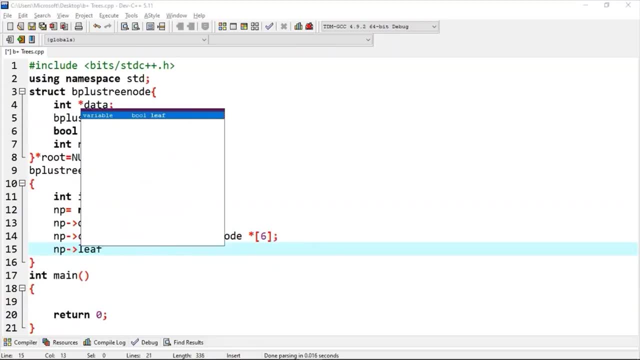 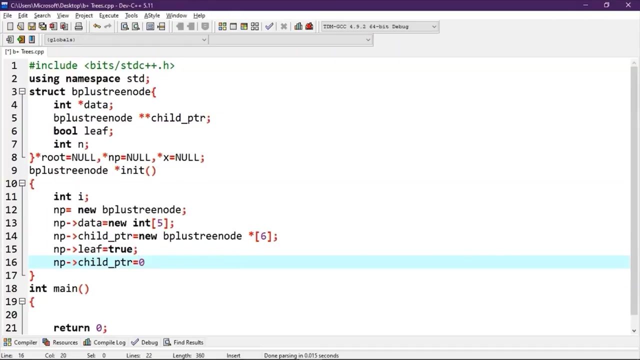 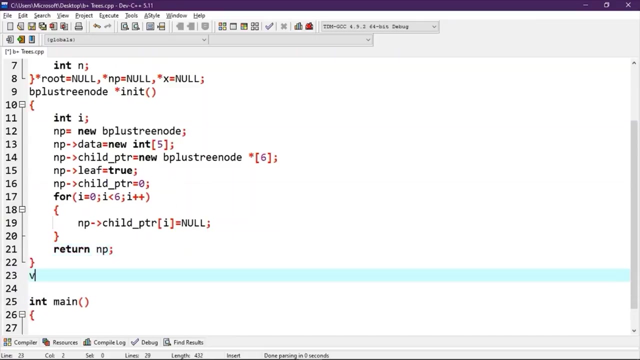 star bracket 6 and belief is equals to true and p at the n is equals to 0. now we will write a for loop: i is equals to 0, i less than 6, i plus plus and p child is equals to regard return traverse b plus 3. 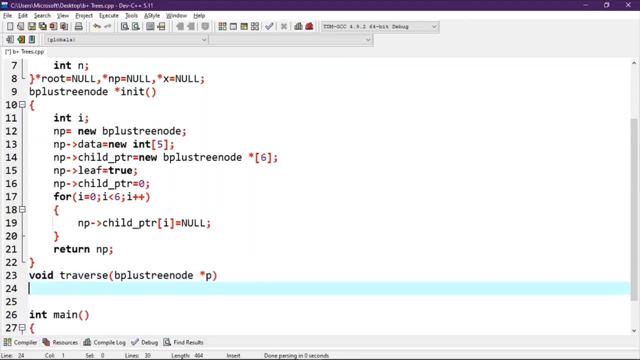 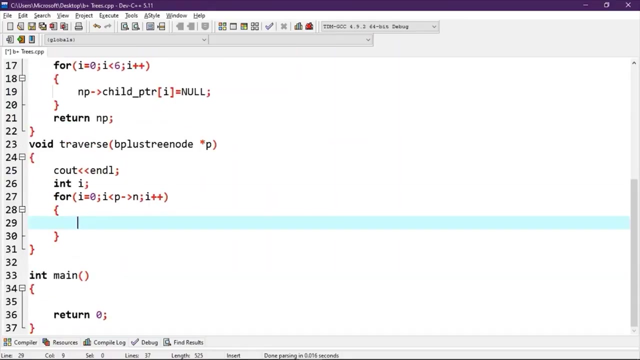 node star, p and am and I. again a for loop from my equals zero to I, less than P, at n, I plus plus. if P doesn't have leave, then we will traverse that child Travis, a child PTR bracket high. say out be daughter at I, I, I. 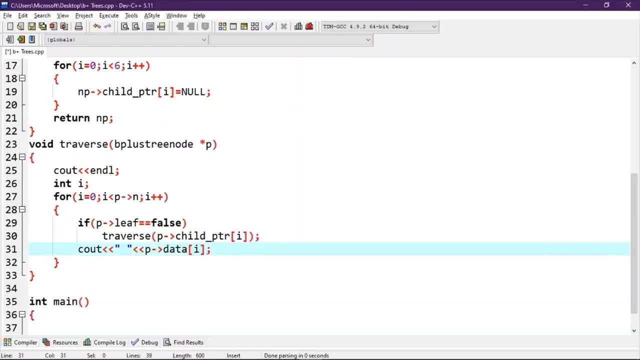 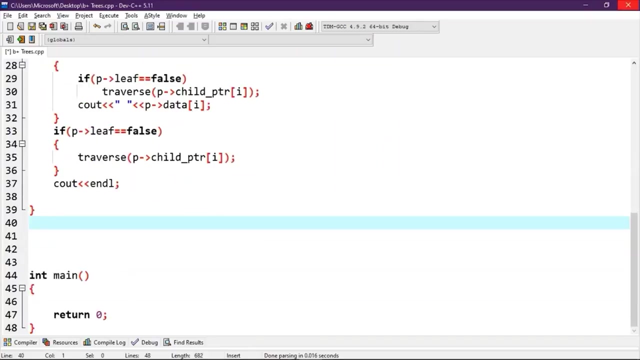 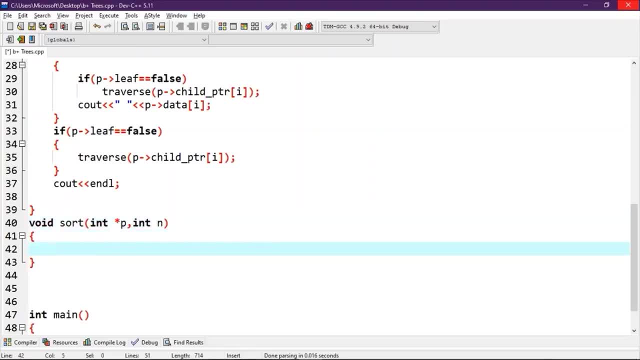 int. i comma j comma. temp for loop: j equals to i, j less than equals to n, j plus n plus. if P bracket I better than P bracket J, then we will swap these two. temp will store P at I and then P will replace its value with P at J. 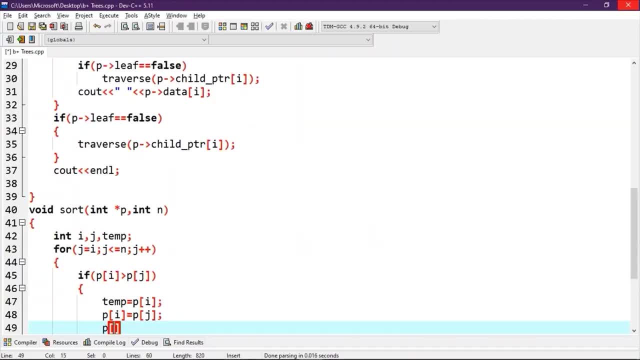 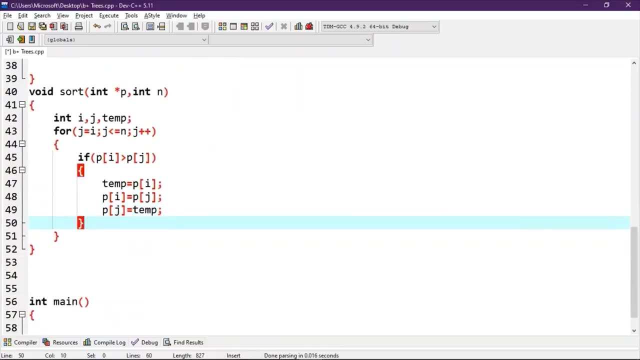 now we will store the temp value in the P of J you now let's write a function to split these child and set child E plus tree node star x, comma, int I, int J, mid child. we are gonna do Notice that we were found a crater. can. 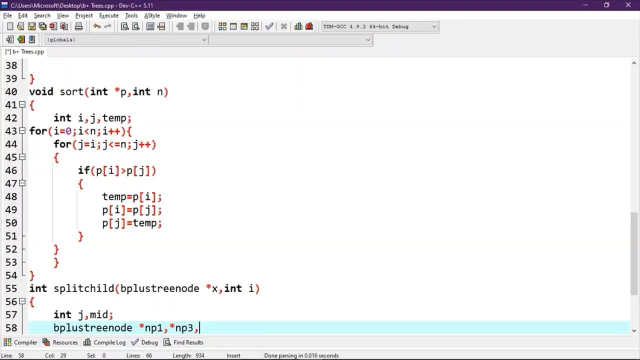 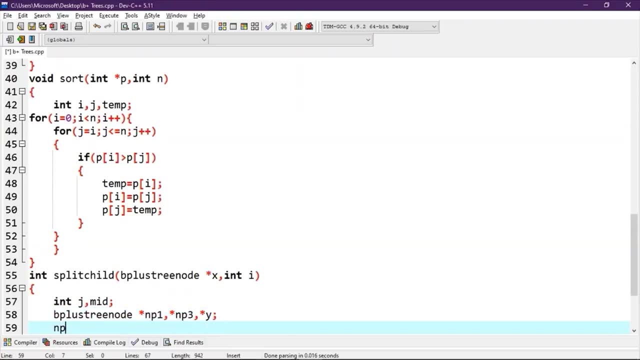 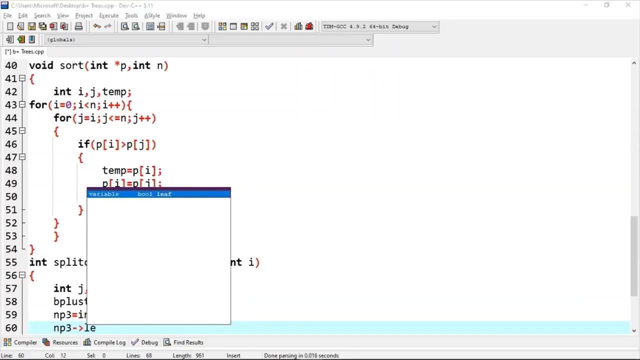 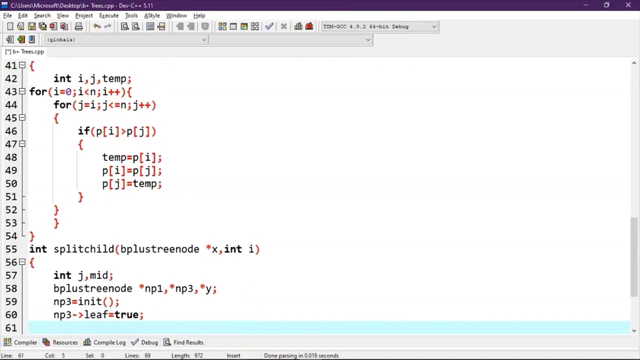 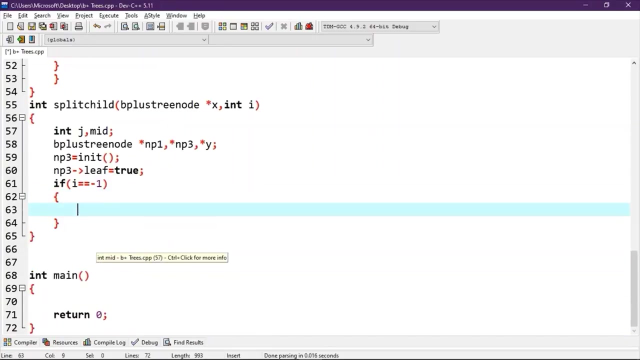 p1 comma star. I'm keeping three comma star 확인. a three is equals to a net and P3 equals to true. if pi is equals to minus 1 and if mid is equals to x tata bracket 2, x tata bracket 2 will be equals to 0. 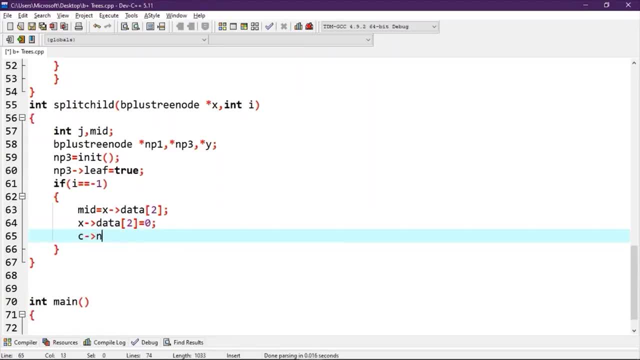 then x will store 10 and minus minus p1 is equal to INET. now when p1 leave will be equals to FALSE and X LEAVE is equals to TRUE. so for loop J is equals to 3, J less than 5, J++ J minus 3. 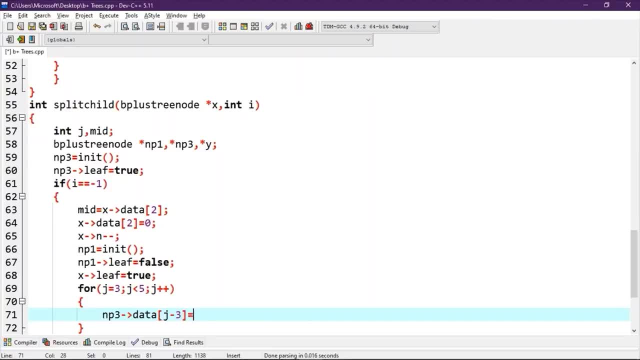 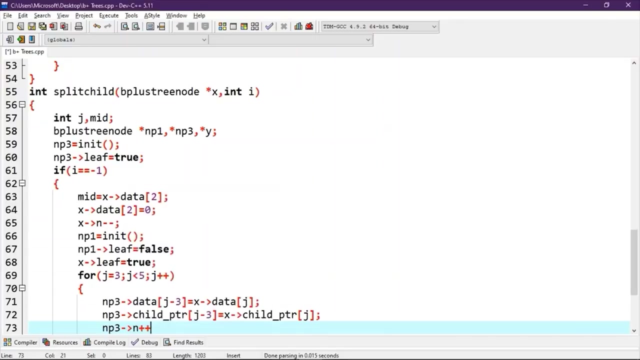 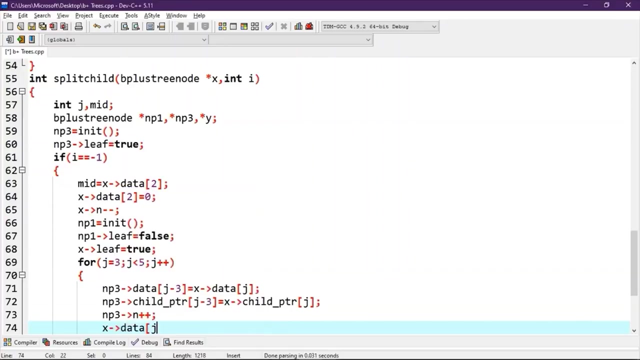 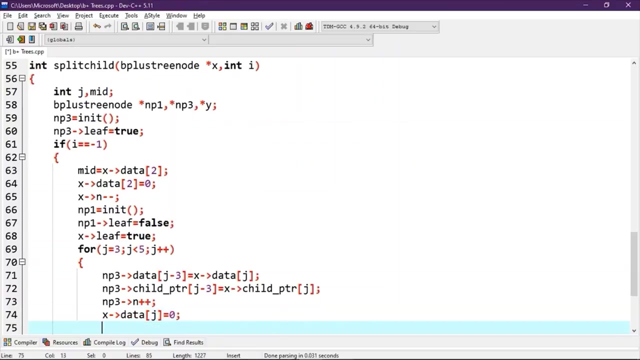 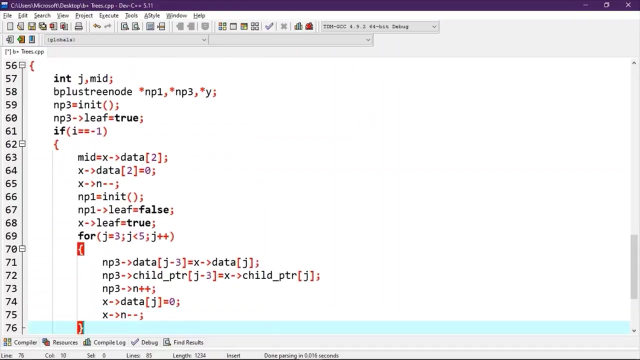 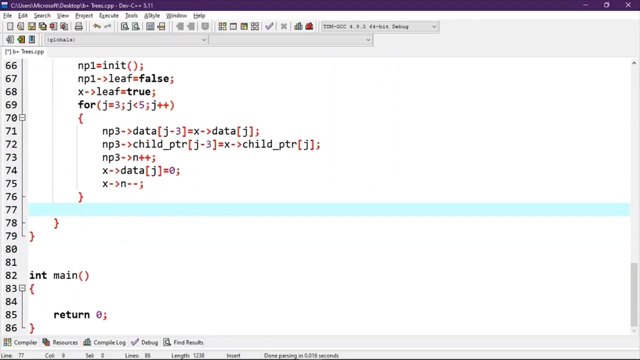 will be equals to x data and j and p3. child PTR at J minus 3 is equals to X at child PTR record J and p3 and plus plus X data. like a J is equals to 0 now, X later than and minus minus another for loop. 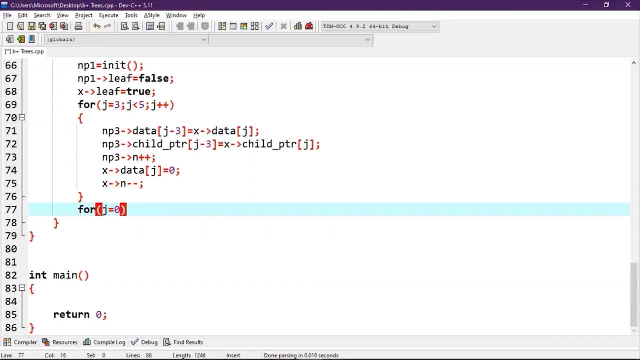 from J is equals to 0 with J less than 6 at J plus plus rate X. child PTR at J will be stored at null now and P1 data at zero position will be equals to made and P1 child PTR at and P1 on air. 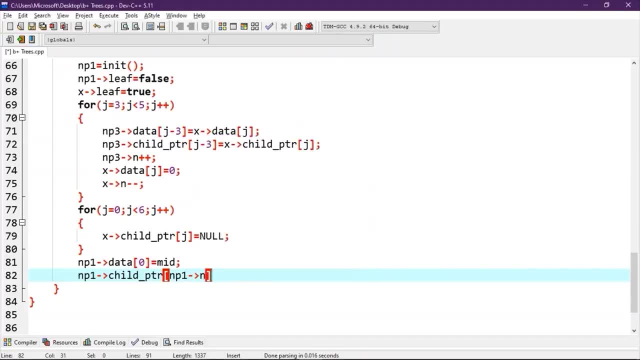 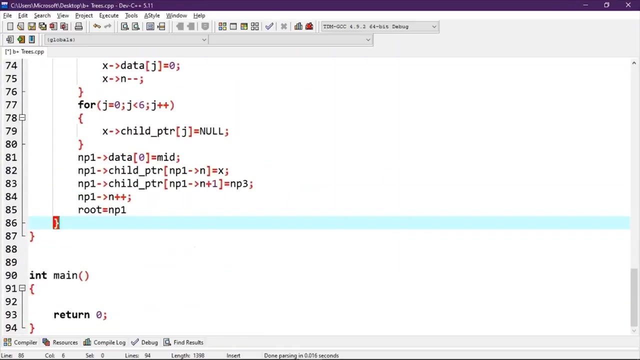 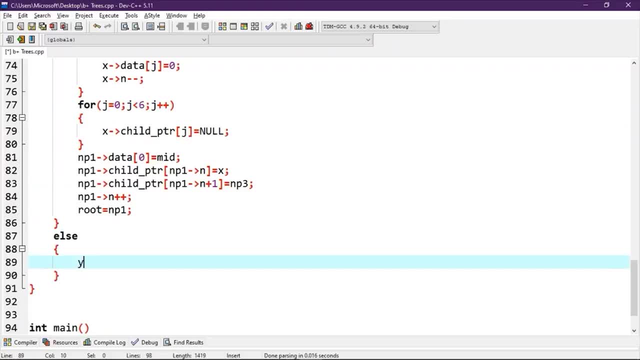 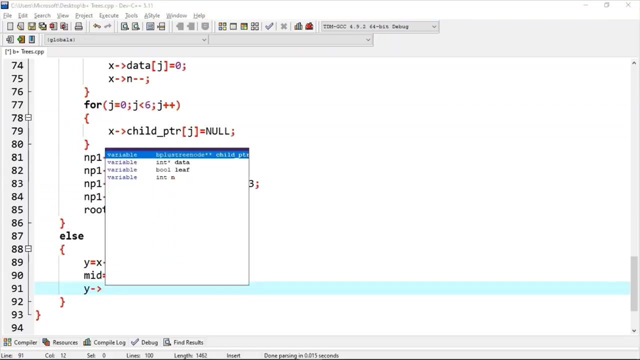 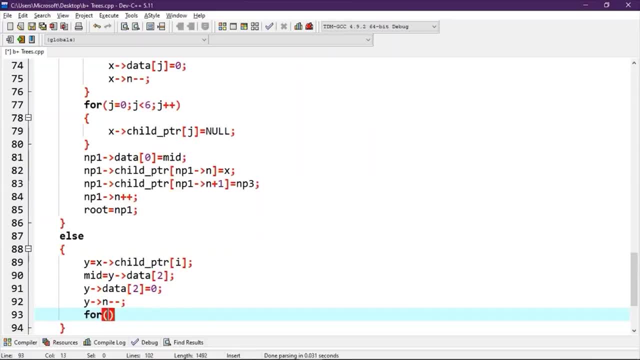 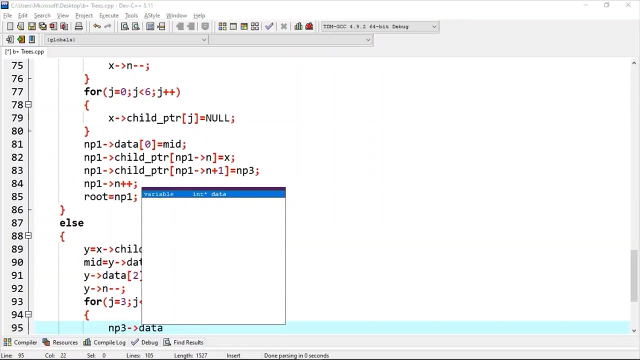 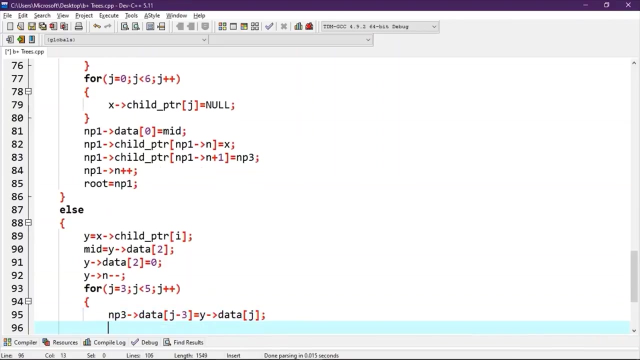 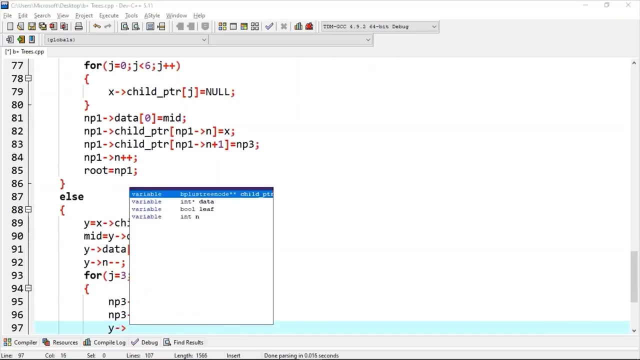 Now for loop: j is equals to 3, j less than 5, j plus plus, And p3 data j minus 3 is equals to y data j and p3 n plus plus y data bracket j is equals to 0. 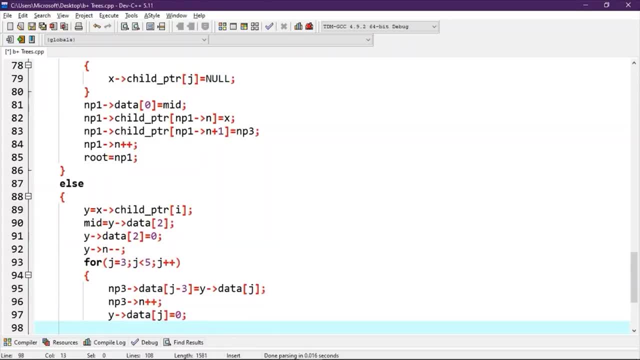 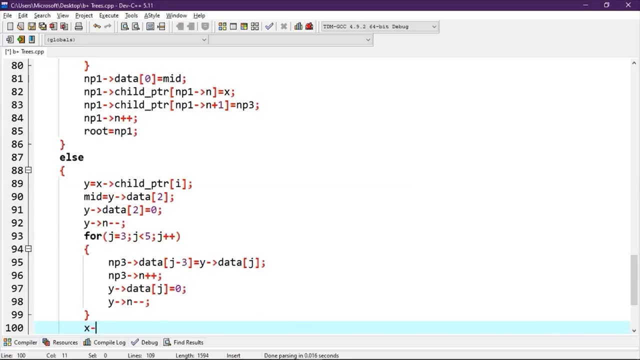 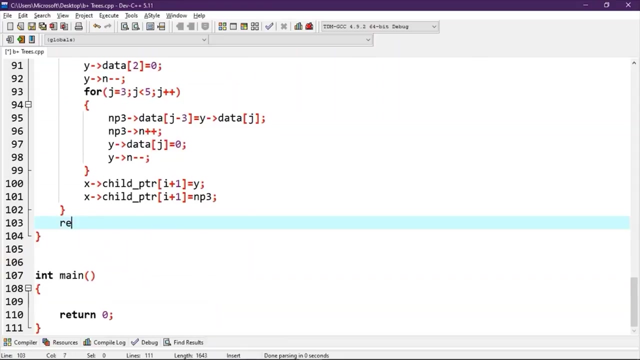 y, n-minus x. child ptr at i plus 1 is equals to y. x at child ptr at i plus 1.. x at child ptr at j plus 1 is equals to n- p3. Return- Return. Now we will write a function to insert into the tree void. 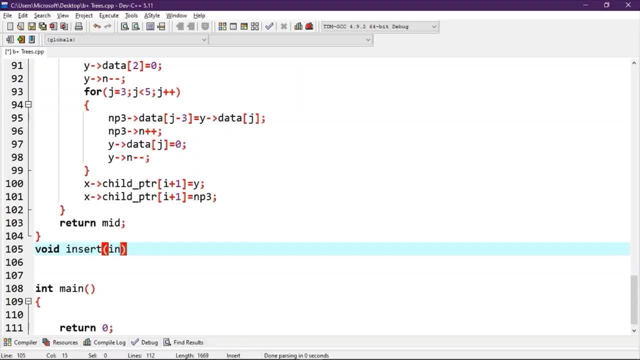 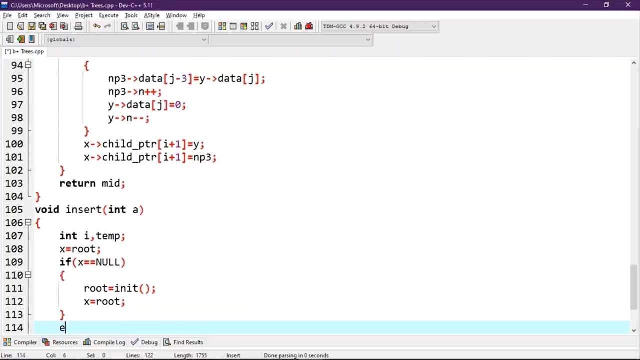 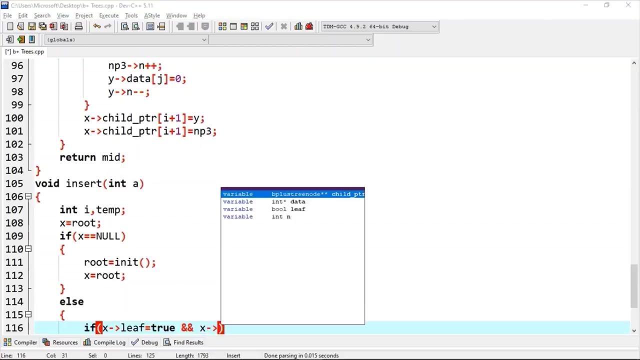 Insert argument as int a, so int itemp x is equal to root. if x is equal to null, then root is equal to finite and x will be equal to root. otherwise, if x is leave and x at 9 feet and x at n is equals to 5. 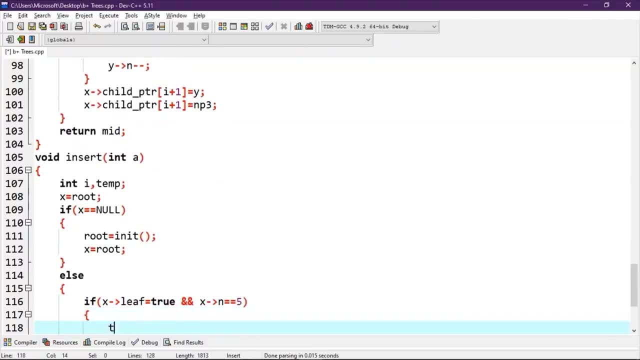 and temp is equals to split child x. comma minus 1. x is equals to root 0 0 0 0 0 0 0. a is greater than X at i and a is less than X at tata i plus 1. 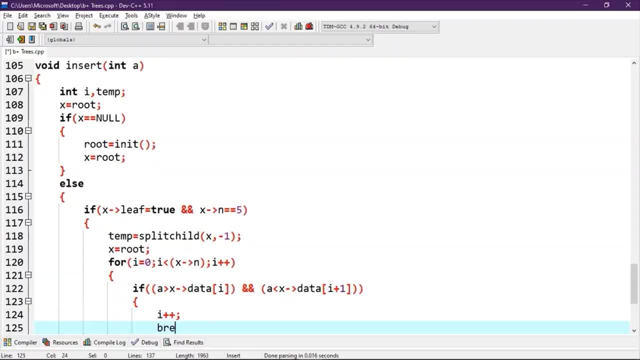 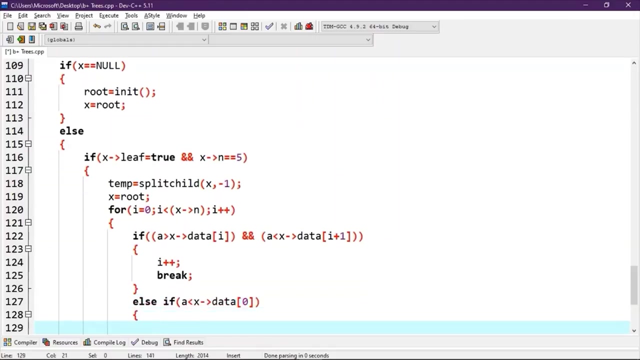 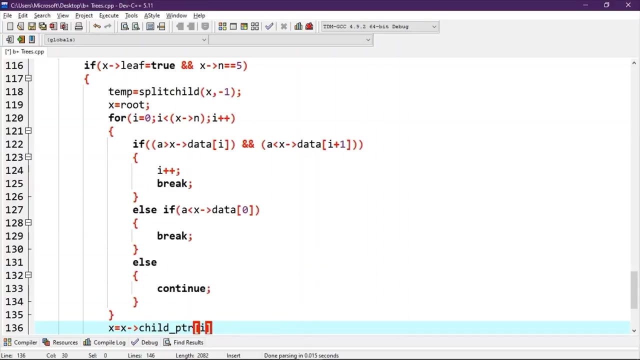 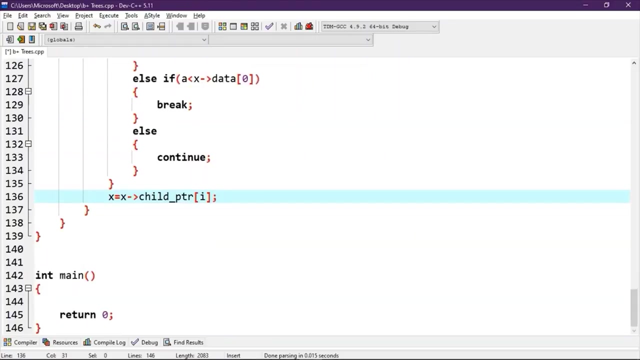 i plus plus and break else. if is less than X at tata 0, then break else continue. X is equals to X at child at I, else, while X leave is false, for loop i is equal to zero when i is less than X at n i plus plus. 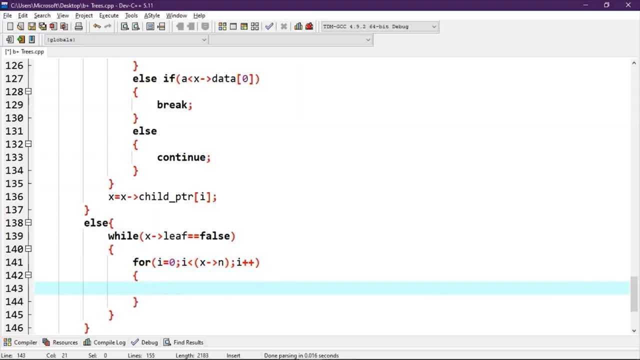 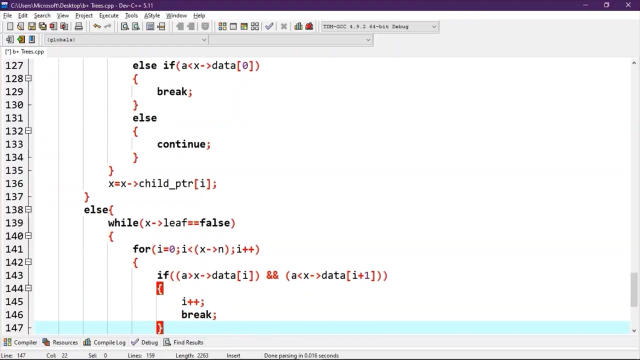 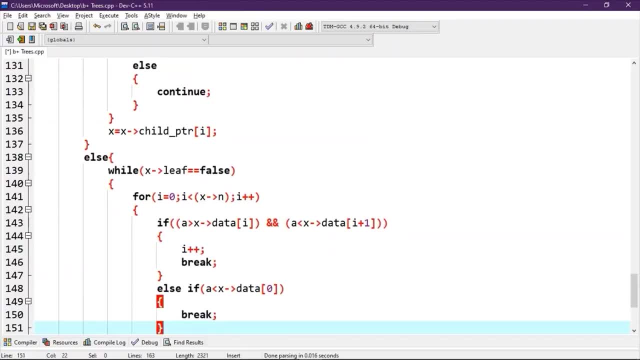 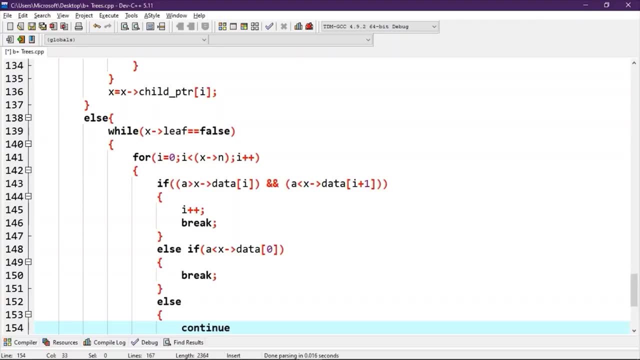 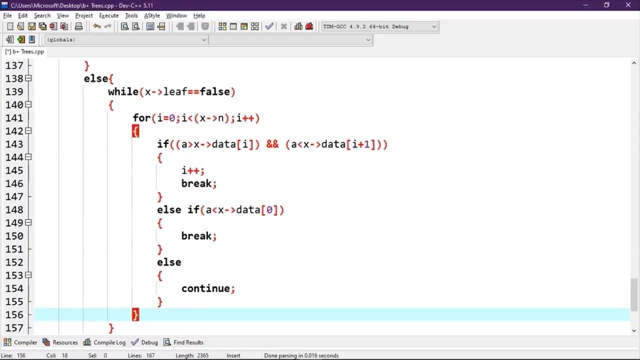 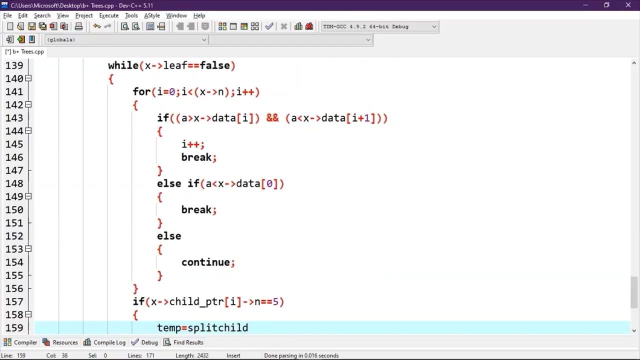 Else continue. If f is greater than x at data i plus 1, i plus plus break. If x is greater than x at data i plus 1, i plus plus break, Else continue. at n is equals to 5, then temp is equals to split child at X comma I. 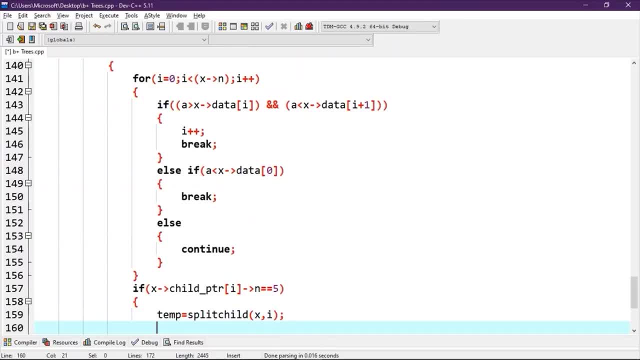 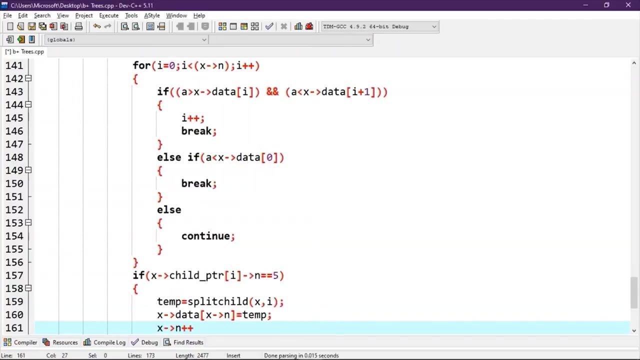 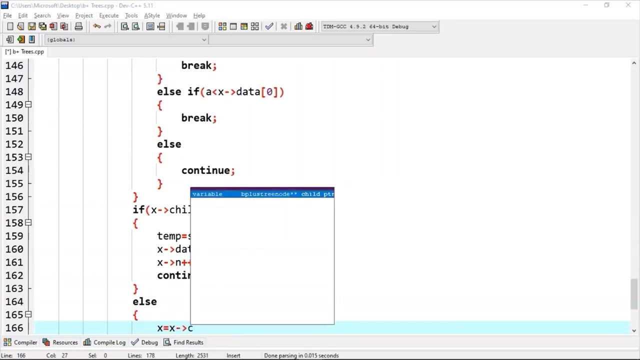 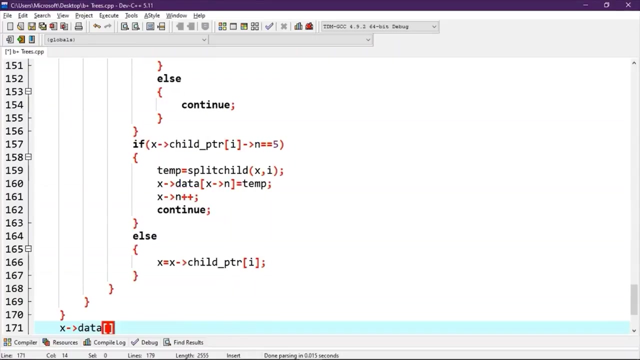 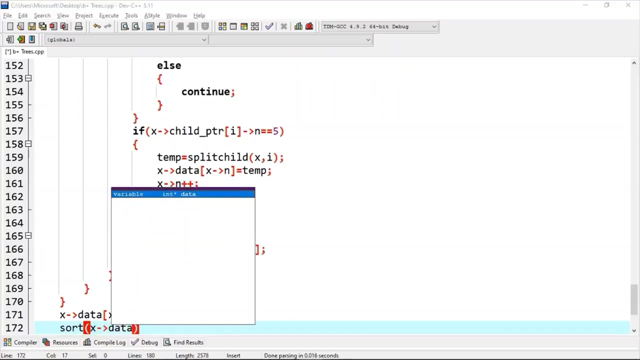 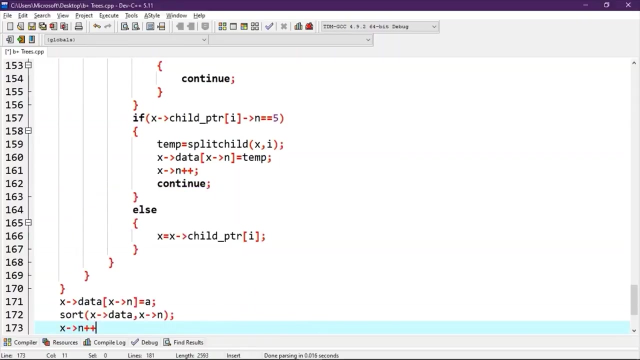 X. data at X. n on n is equals to temp. X at n plus plus continue. else X is equals to X. child meter I. X on data at X at n is equals to a sort. X at data. X at n. X at n plus plus. now let's write. 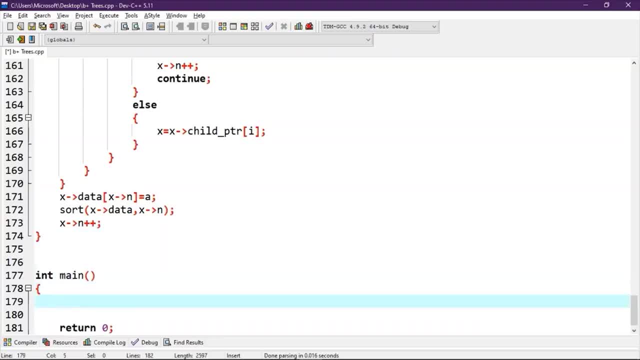 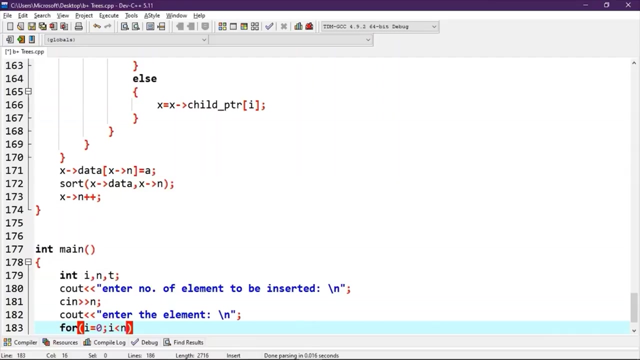 the code for the main block. first we will declare some variables as and I and N and T. Now we will request enter number of element to be inserted. Now we will enter the element. So enter the element. Now we will enter the element. Now we will write a for loop. i is equal to zero, to i less than n at i plus plus. 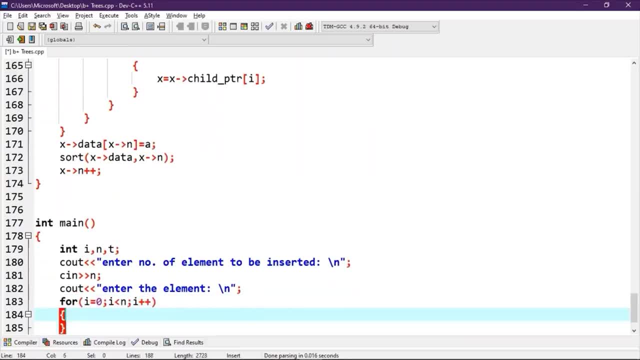 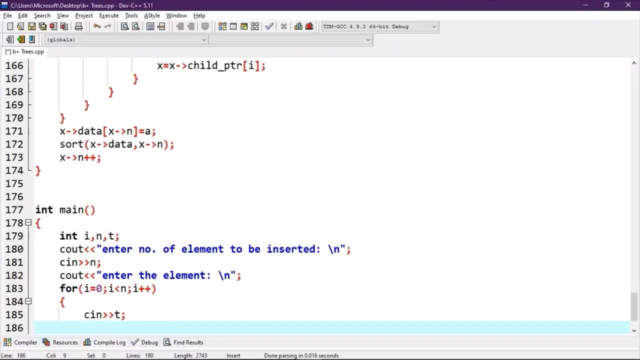 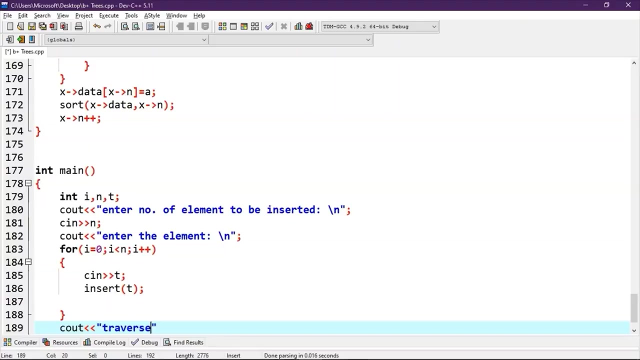 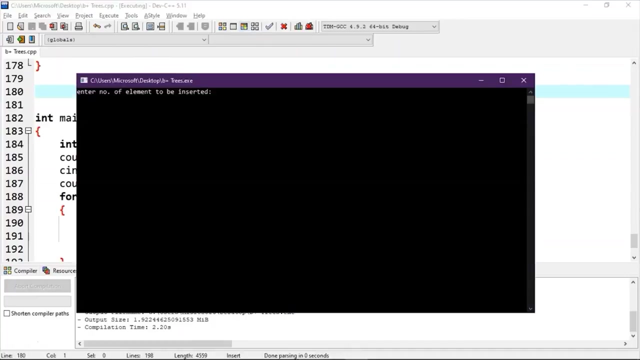 So cn D and insert D. Now we will traverse this tree, So cout Traverse Such of p plus 3, reverse root. let's execute this. we will enter 5 elements: 2 comma, 3 comma, 5 comma, 7 comma, 9. as you can see, we have. 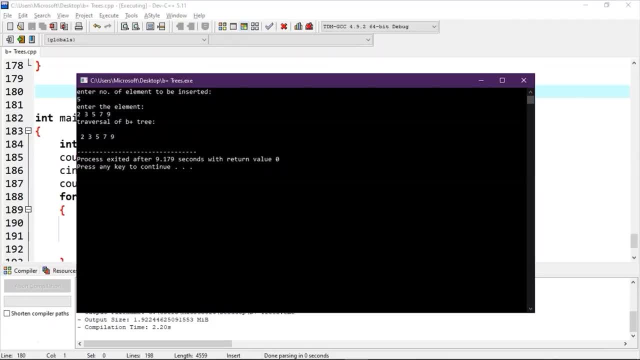 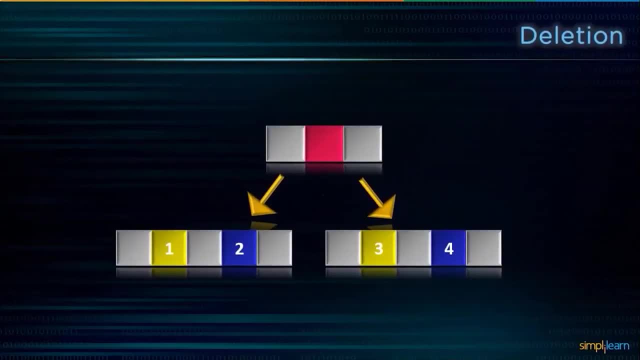 successfully traversed our first b plus tree. let's get back to our slides. next deletion: while deleting the first b plus tree, we will enter 5 elements: 2 comma, 3 comma, 5 comma, 7 comma 9. as you can see, we have any element from b plus tree. we have to be careful not to break any properties of b plus tree. 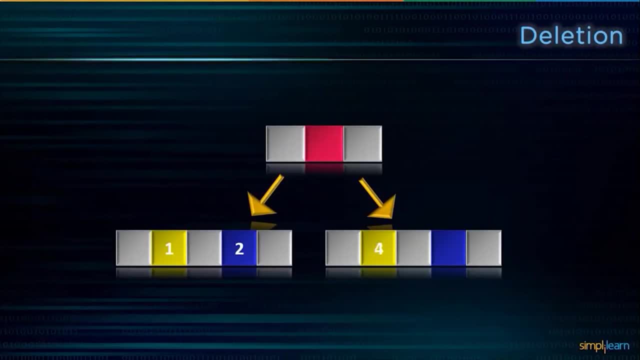 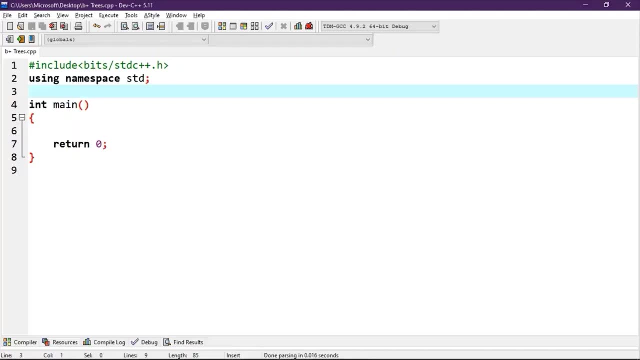 like all, the leaves must be present at the same level, or elements must be in ascending order. now let's try these operations in a code editor. let's start by creating a b plus tree. first we will declare a global variable, int max equals to 3. then we will create a class ep tree. 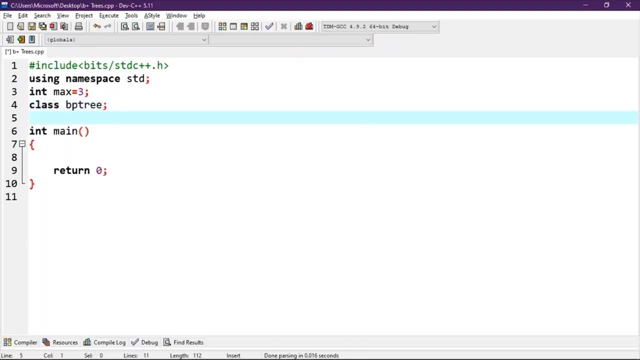 and a class node boolean its leaf. int star key comma size. node star, star, ptr. and a friend, class bp tree, now public node variable. now we will write class bp tree. now we will write class bp tree. so node start void. insert note star comma. note star void. 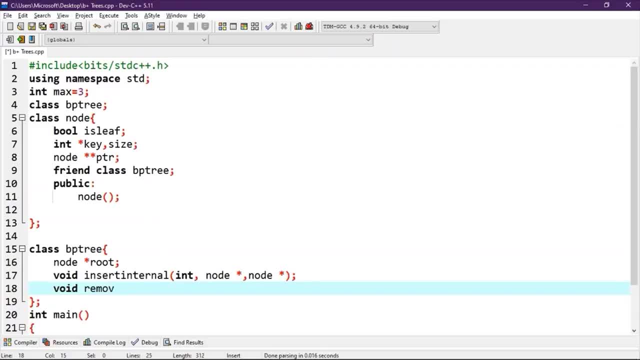 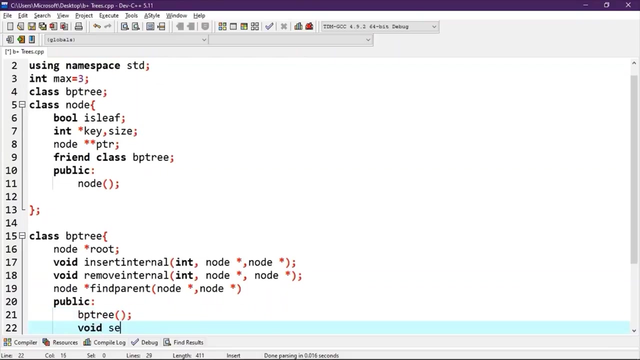 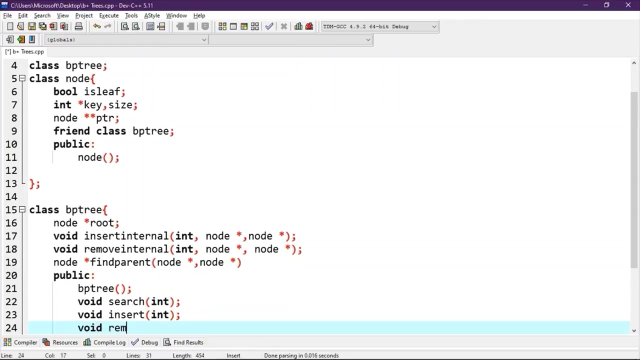 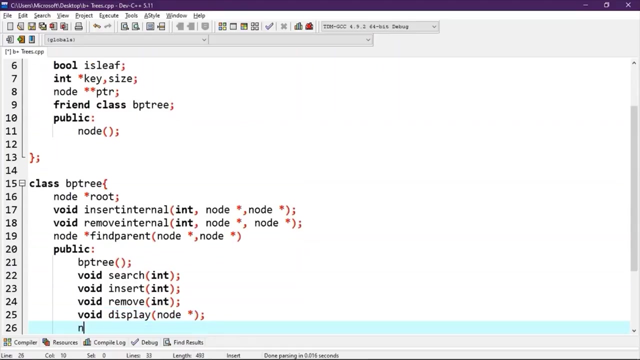 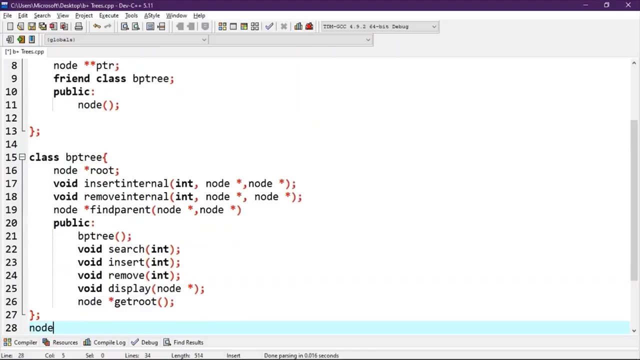 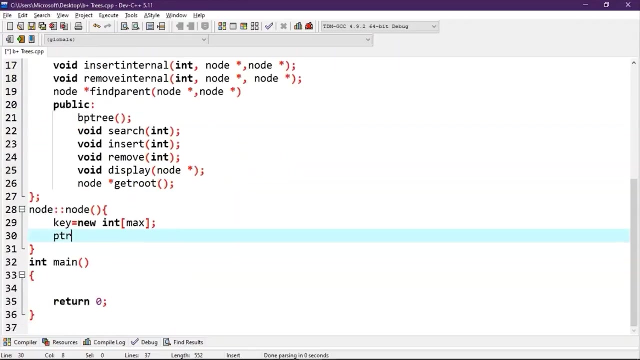 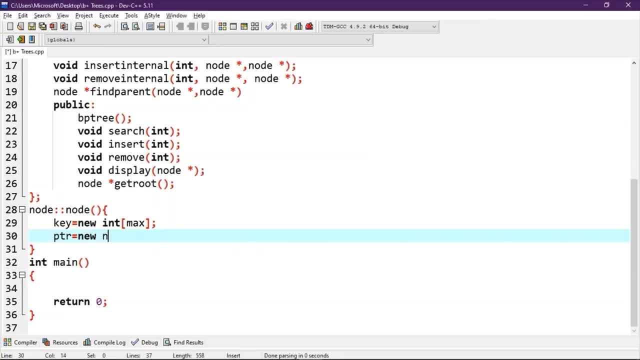 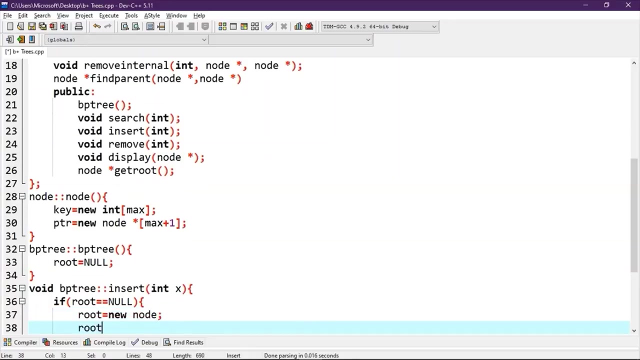 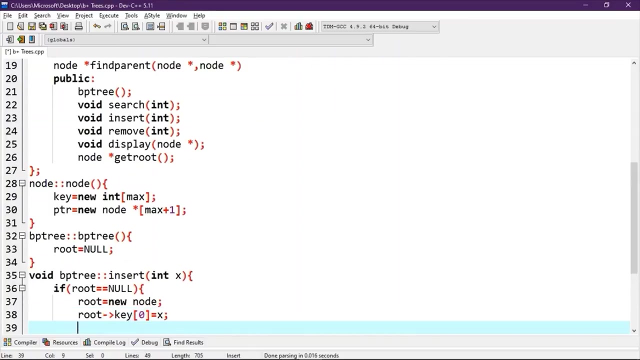 new node, star bracket, max, plus one pp tree plus two null. now void the bp tree insert and x, if true, is equals to null, then root is equals to new node in z. root calls key at zero and secures it. x. x. the root checks its leave. 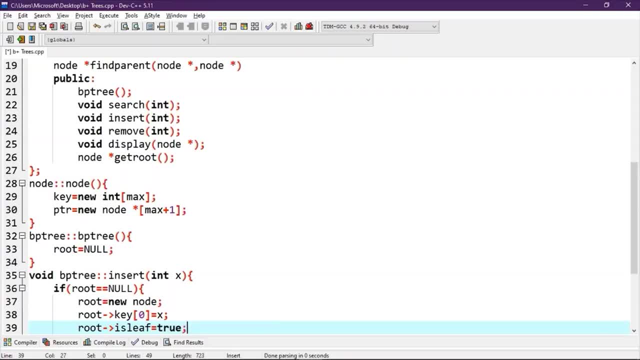 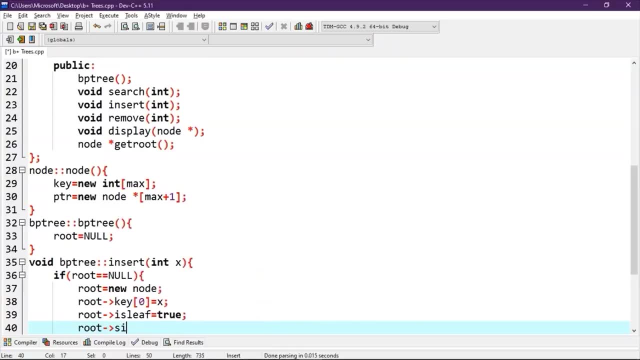 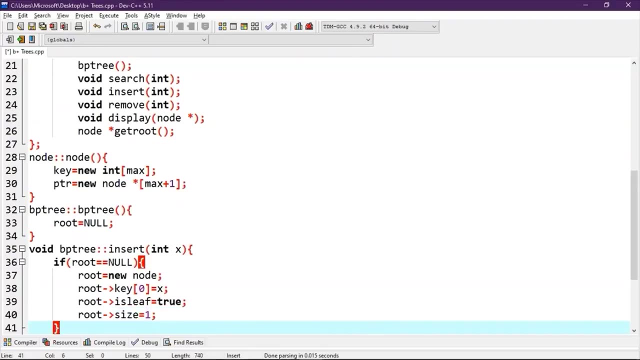 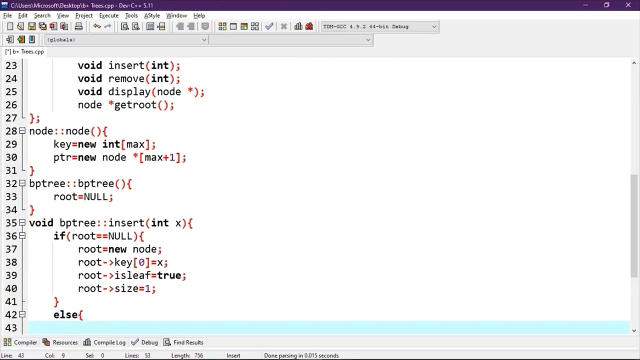 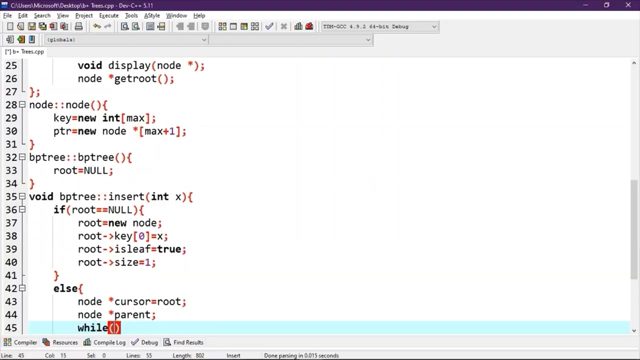 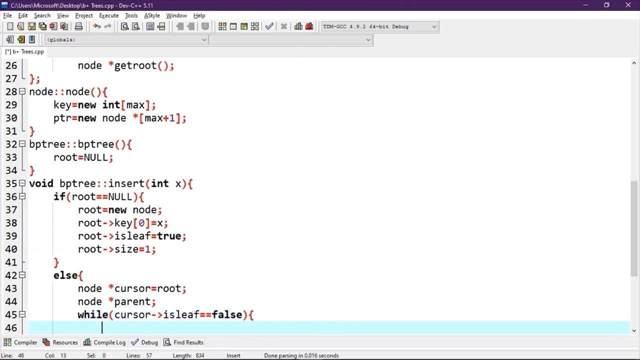 in a use: srcSRCSRCSRCSRCSRCSRCSRCSRCSRCSRCSRC. twice it equals to one else node cursor it equals to root node. star parent while cursor is leave is equals to false. parent goes to cursor. 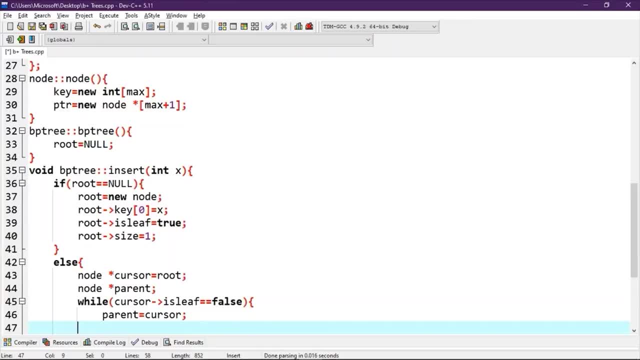 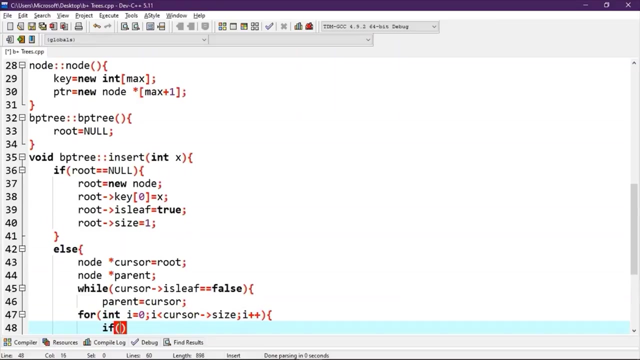 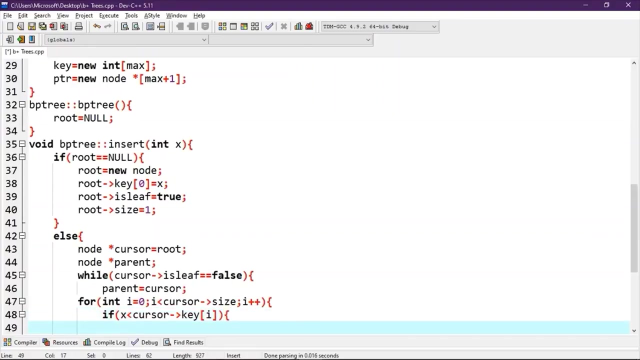 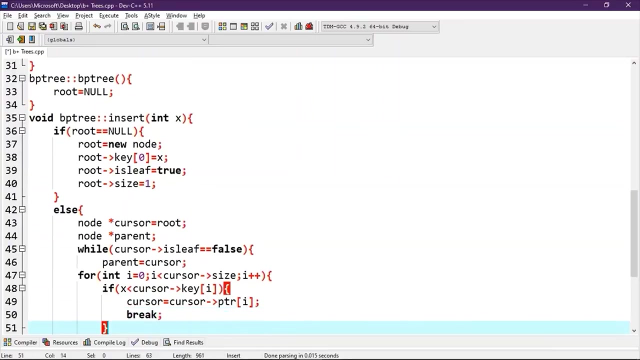 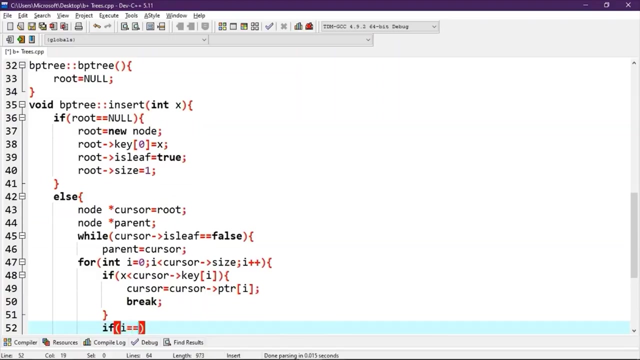 now for loop: and i is equals to zero to i less than cursor size, I plus i, i plus plus. if x is less than cursor key at i. if cursor is equals to cursor at ptr at i. if i is equals to cursor at ptr size minus one. 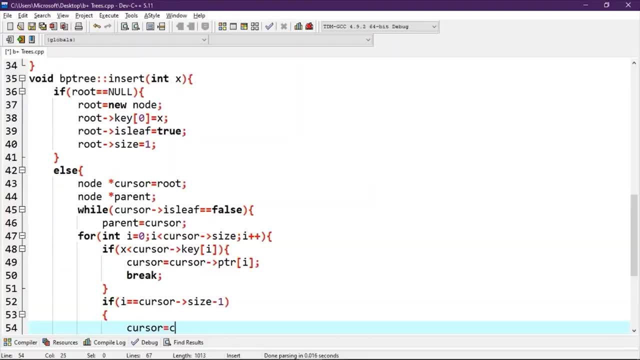 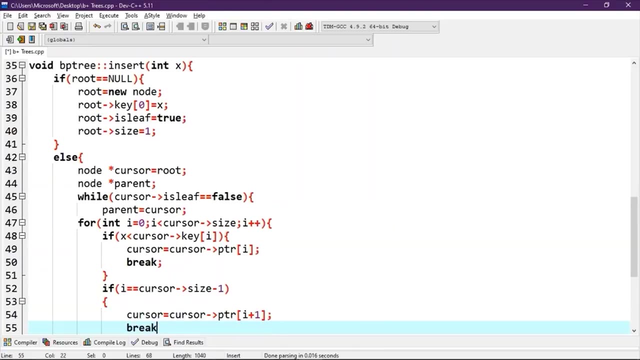 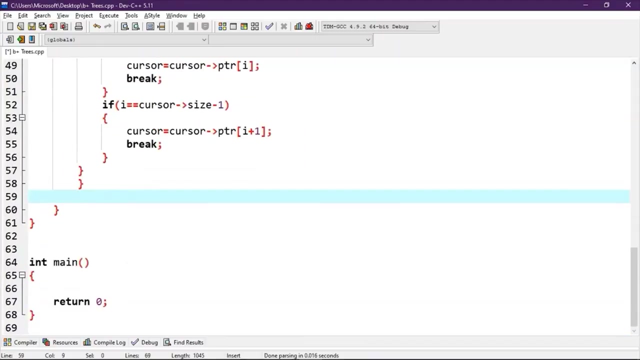 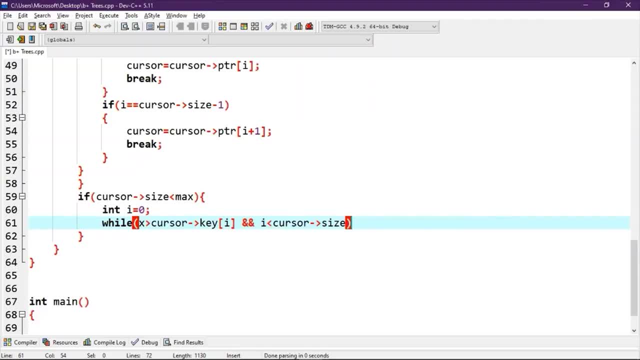 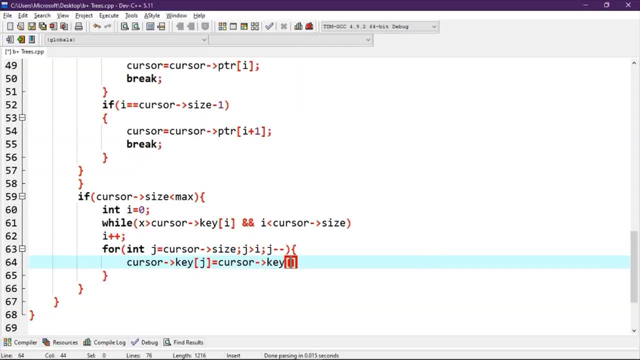 also key at J minus one cursor calls key at I is equals to X. cursor calls I is equals to X. cursor calls key at I is equals to X. cursor calls I is equals to X. cursor calls size plus plus. sir calls PTR. add cursor size. add cursor size. 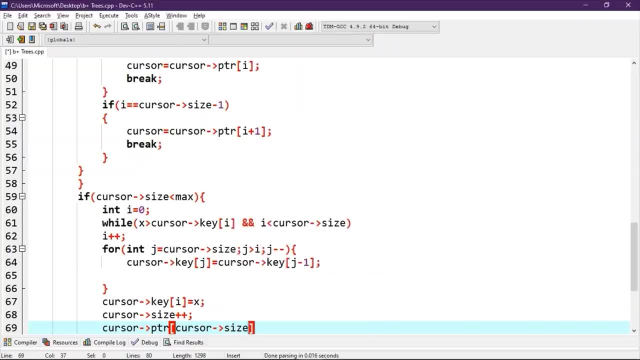 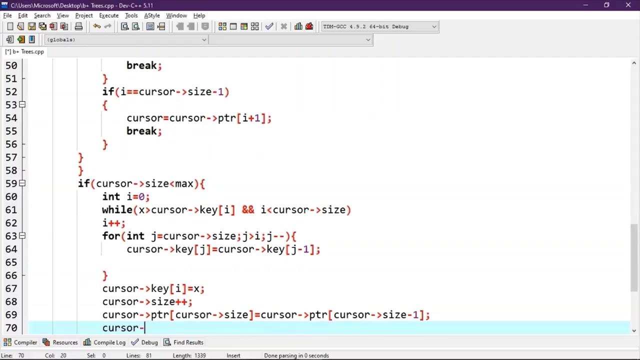 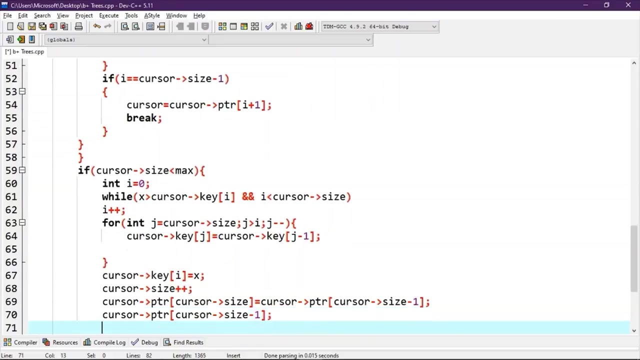 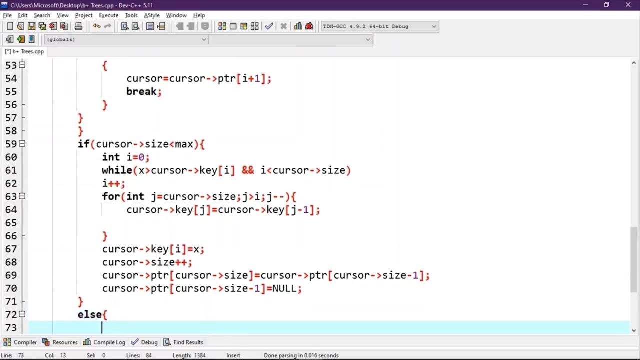 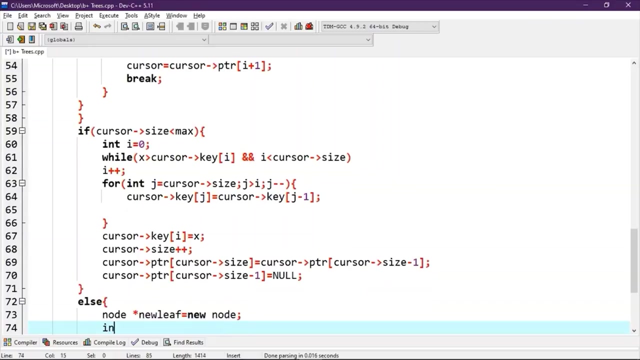 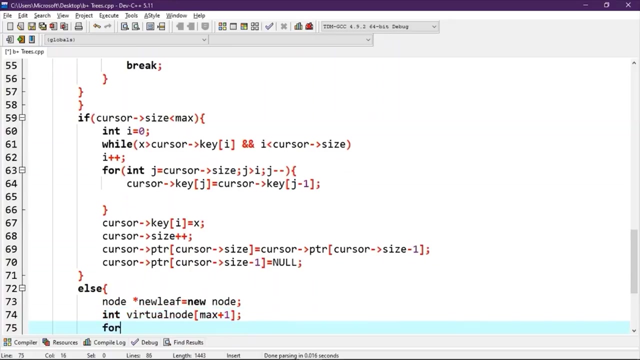 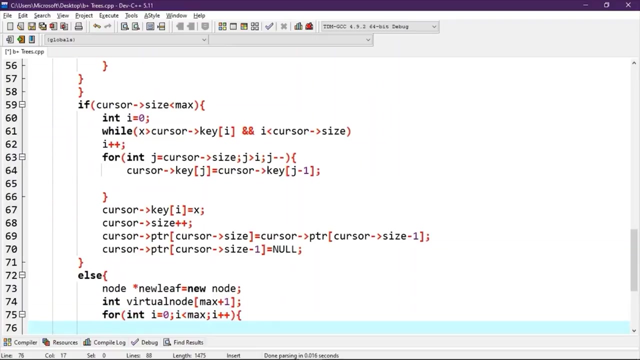 equals to cursor PTR at cursor size minus 1. now, cursor at PTR cursor size minus 1. Cursor, Cursor, Cursor, Cursor, Cursor, Cursor, Cursor. else. node equals to new virtual node max plus one for int. i equals to zero, to i less than max at the rate i plus plus. 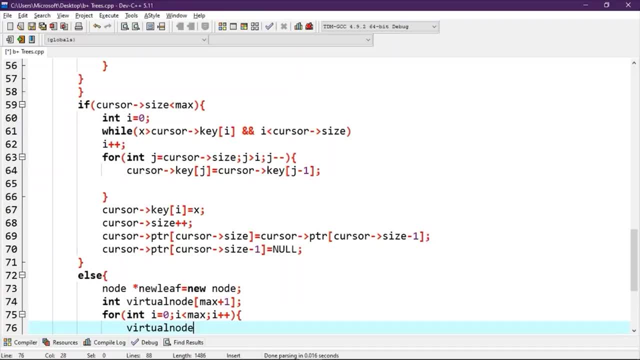 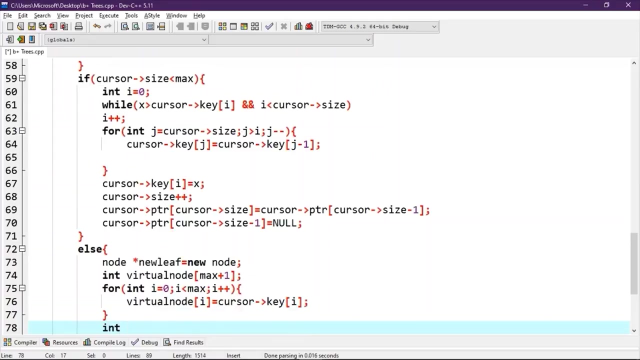 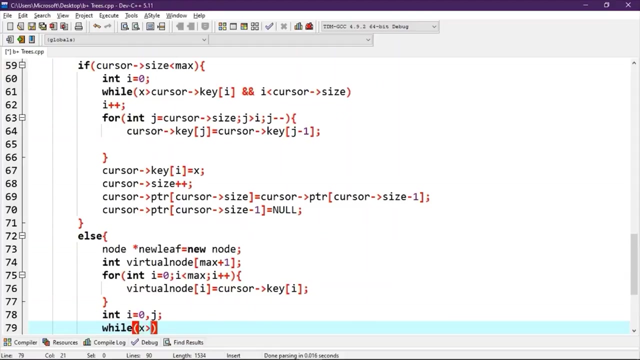 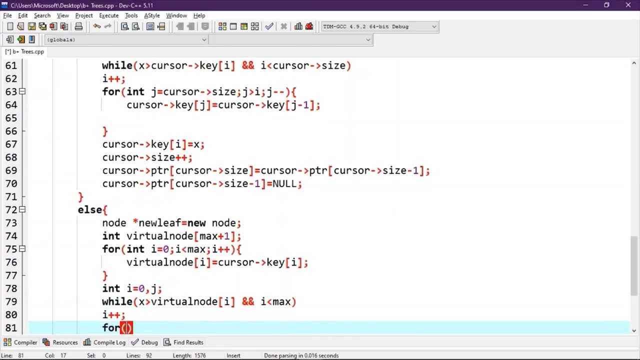 virtual node at i is equals to cursor e. at i. int i is equals to zero comma j. while x is greater than virtual node, make it i. i is less than max. at i is equal to zero comma j. i plus plus for int j is equals to. 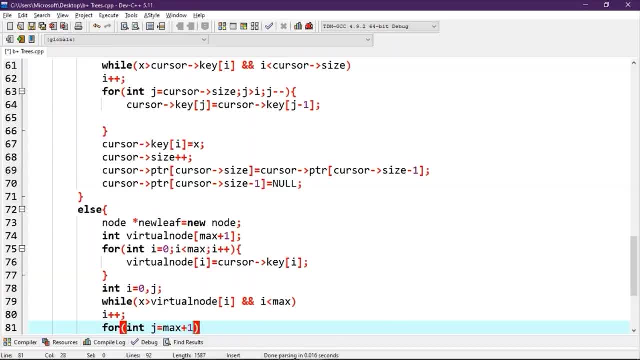 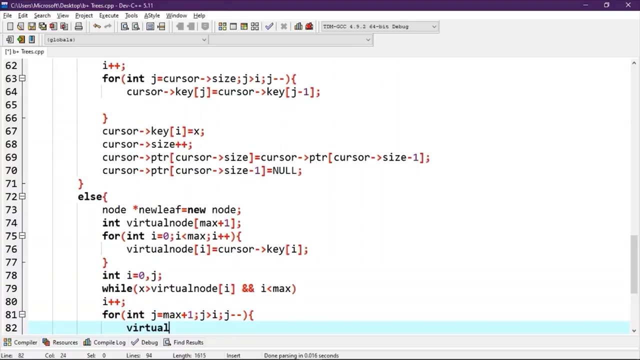 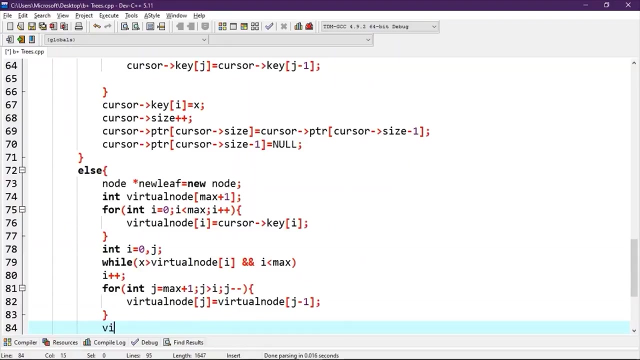 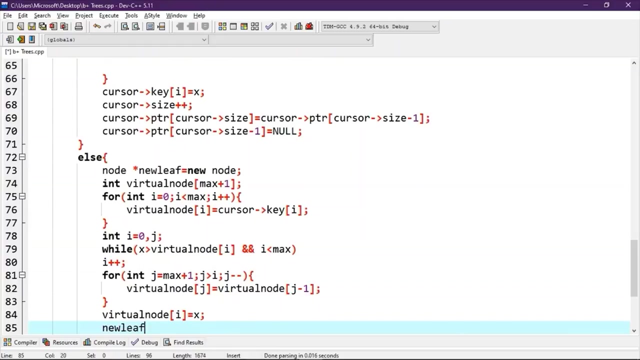 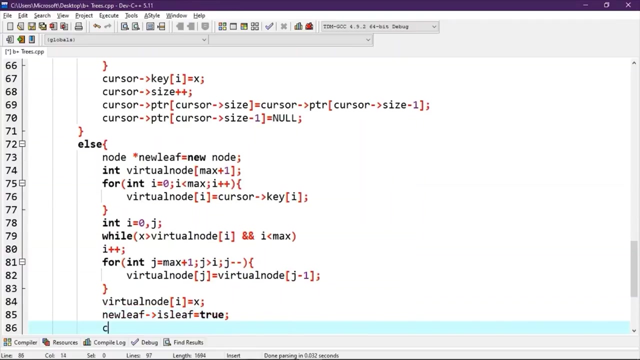 max plus one comma, j is greater than i, j minus minus, i no at j minus one and i, So virtual node i is equals to x, So new leave is. leave is equals to true, So cursor size is equals to x, So new leave is equals to max plus 1 by 2.. 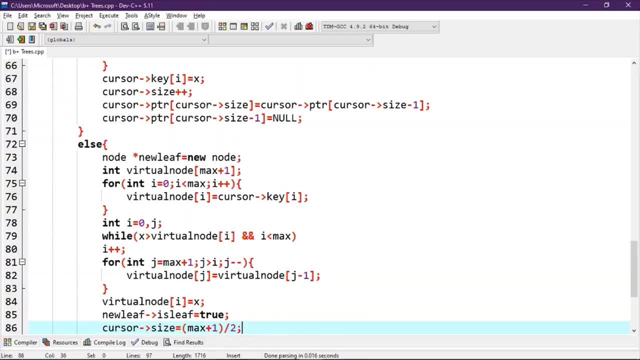 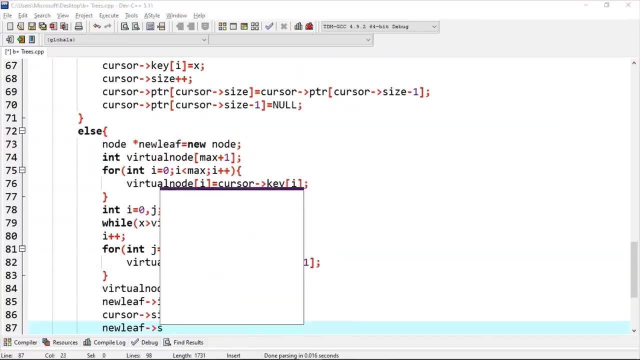 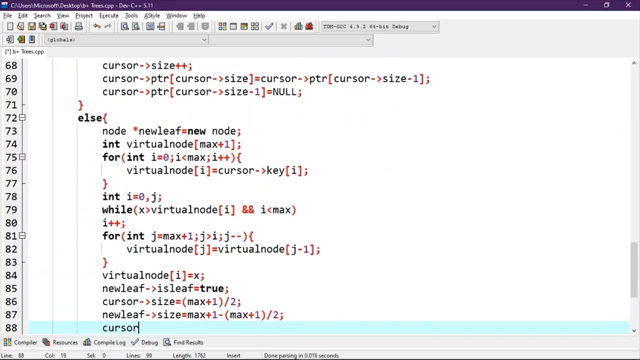 So new leave size is equals to max plus 1 minus. So max plus 1 divided by 2.. So cursor size is equals to x. So cursor size is equals to max plus 1 by 2. So cursor size is equals to x. 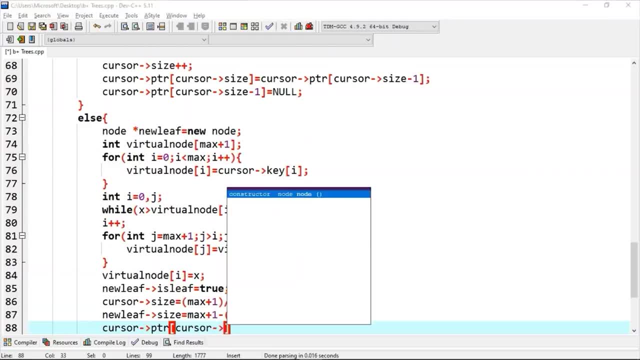 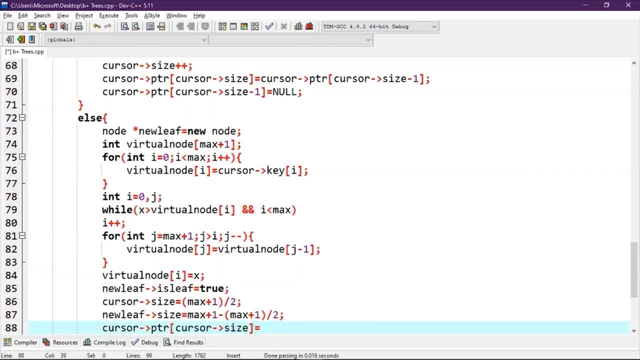 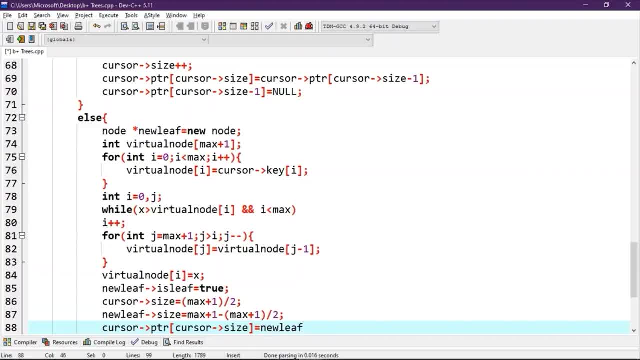 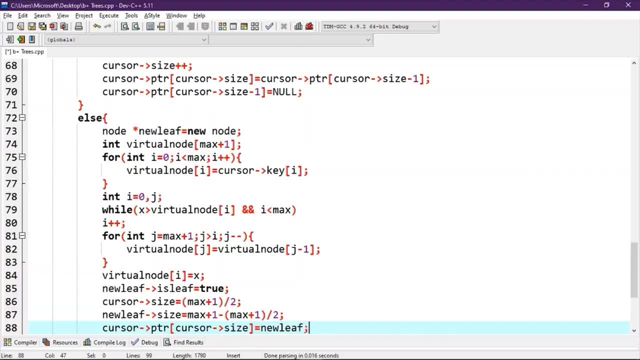 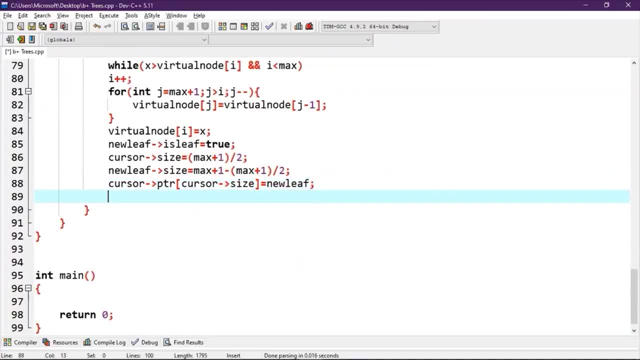 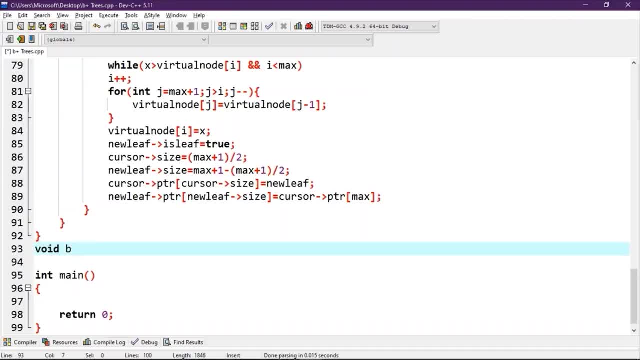 Now void BPTree. Insert- internal Insert internal Insert internal int x: node star: cursor. node star: child F: cursor size is less than max, Then int is equals to 0, while x is greater than cursor at key at i. 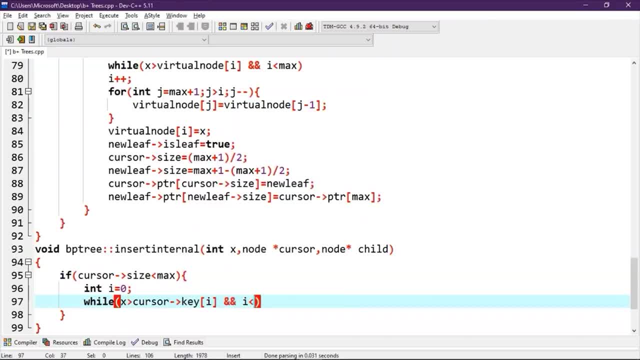 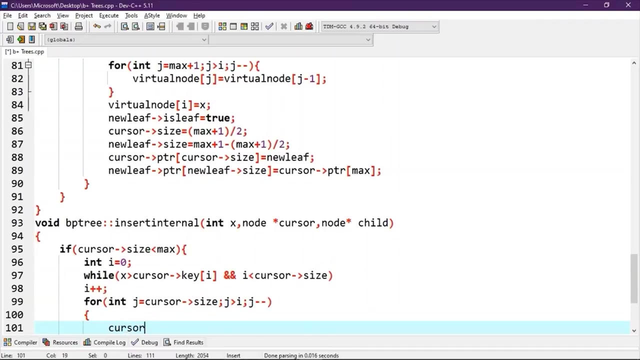 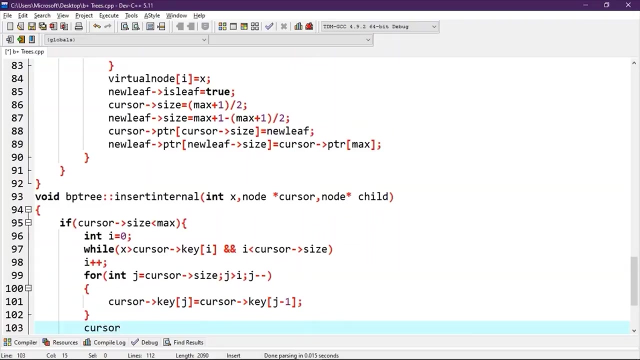 And i is less than cursor of size i++. For loop int j is equals to cursor size j is greater than i, j minus minus. cursor at key at j, j is equal to cursor j minus 1.. Now cursor at key at i. 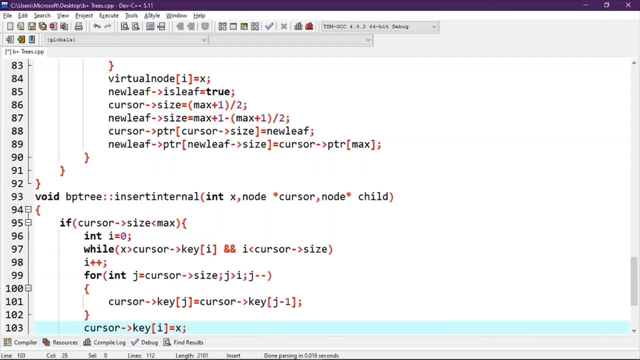 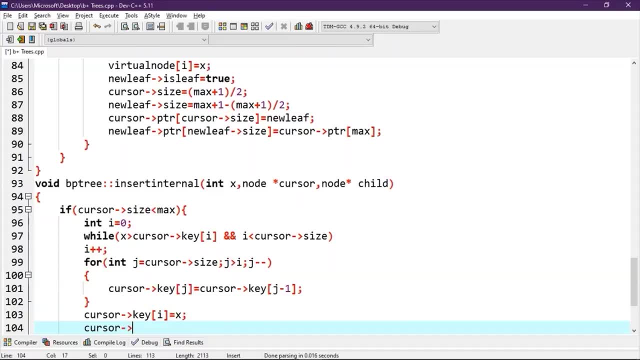 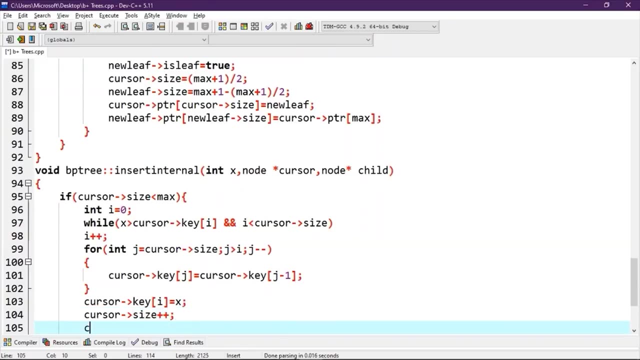 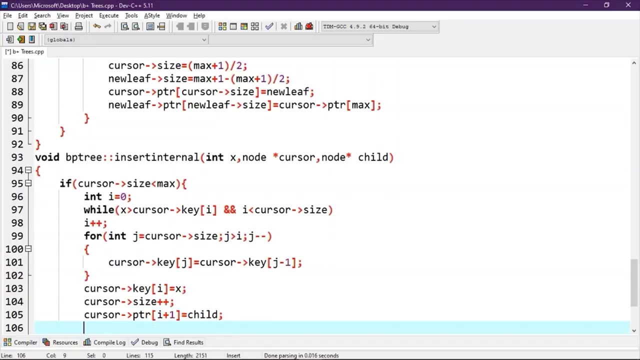 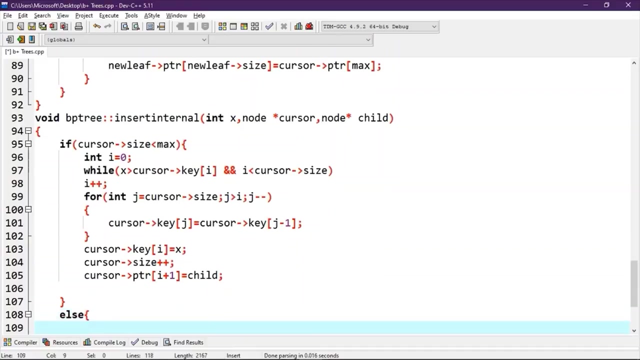 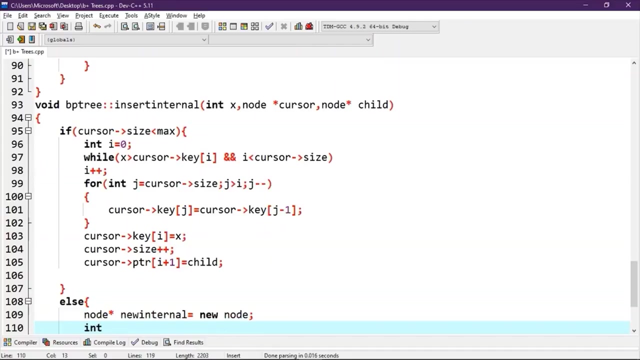 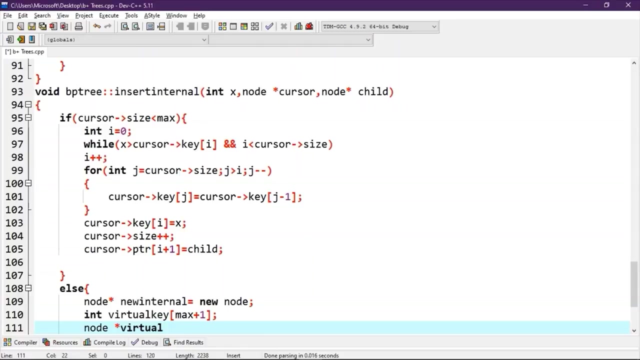 j is equal to x cursor size plus plus cursor at ptr bracket i plus 1.. j is equal to child s node star. internal is equals to new node print virtual key is max plus one node star virtual key at max plus one. 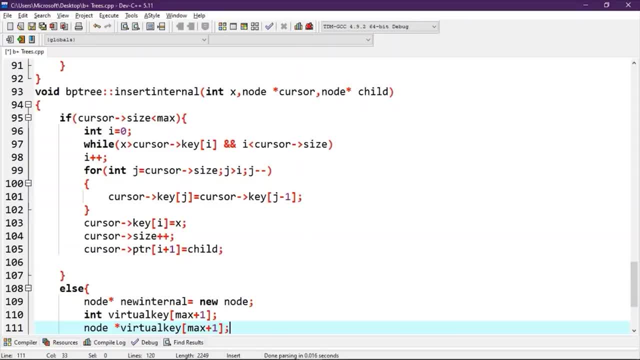 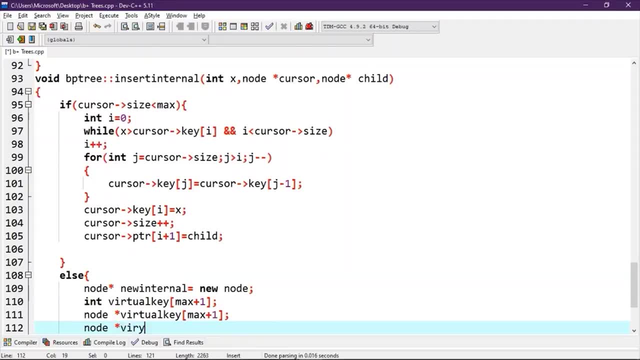 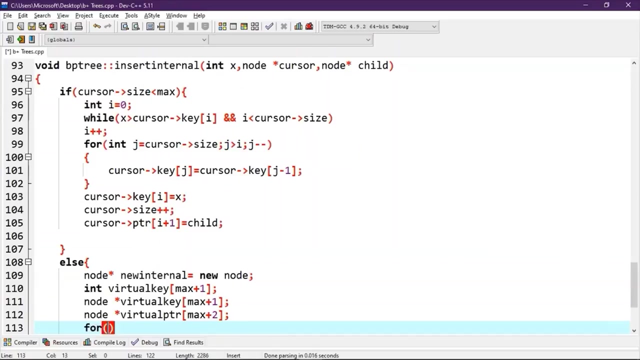 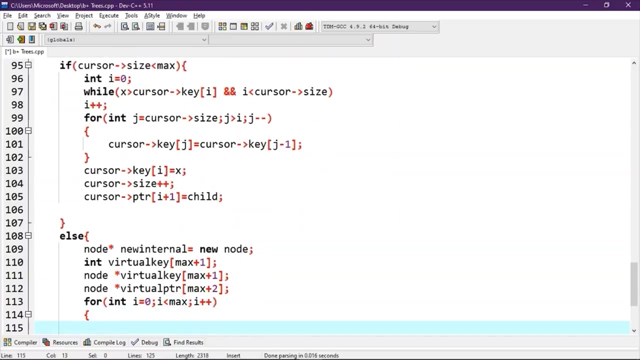 star virtual key at max plus one node star virtual key at max plus one node star virtual key at max, plus one atr at or. and i is equals to zero, and i is equals to zero, and i is equals to zero. i less than max, i plus plus. 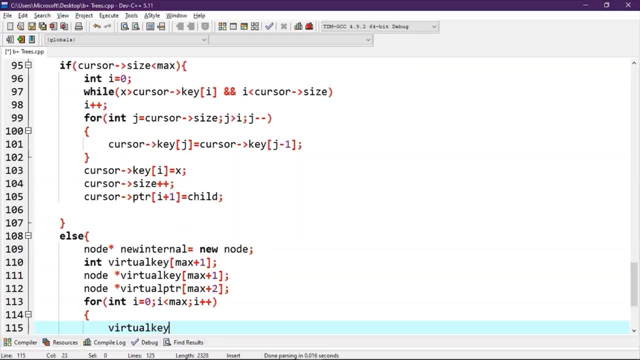 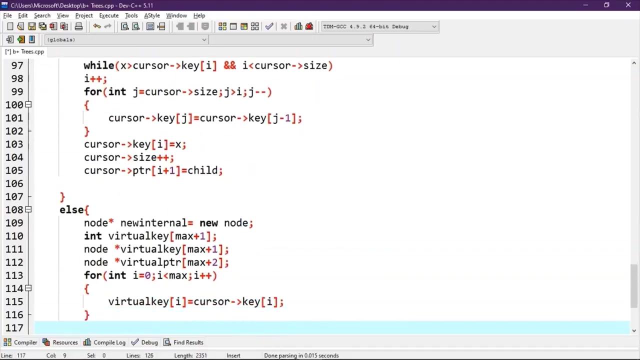 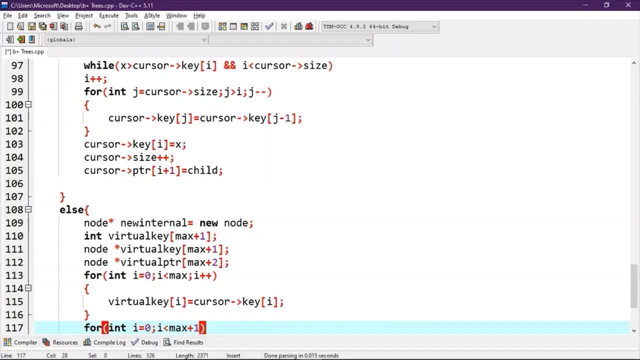 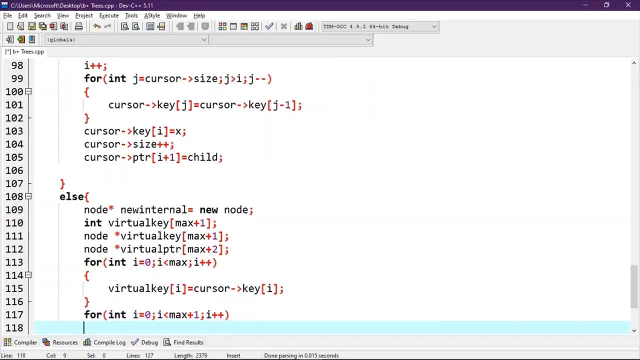 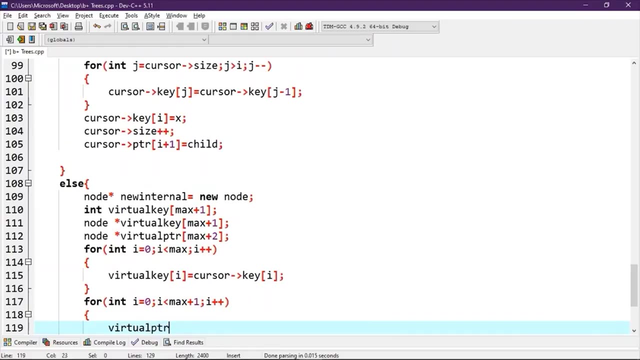 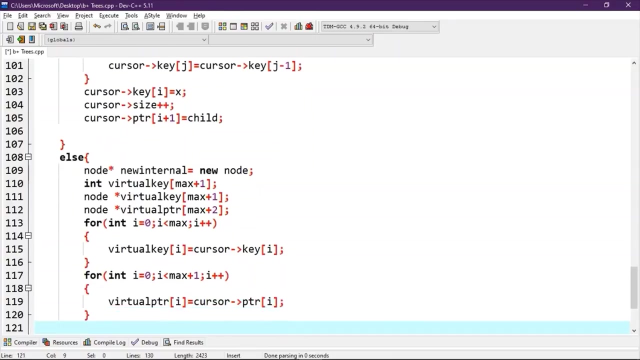 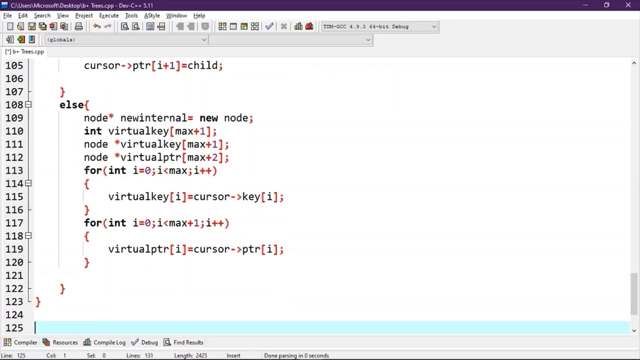 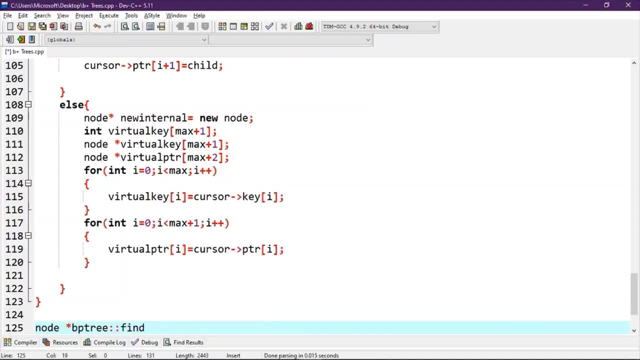 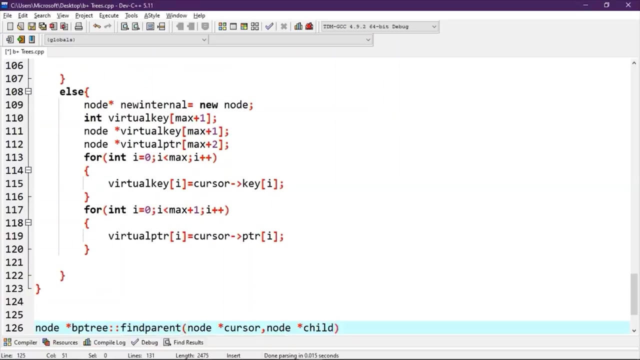 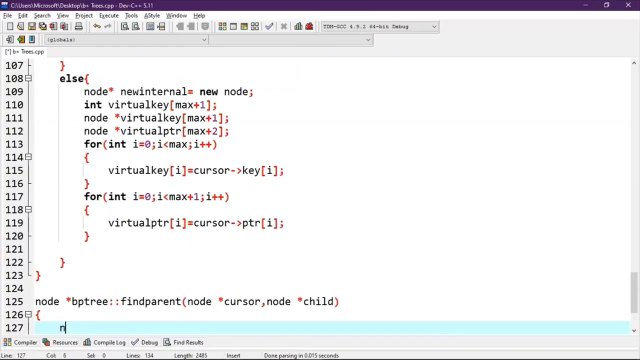 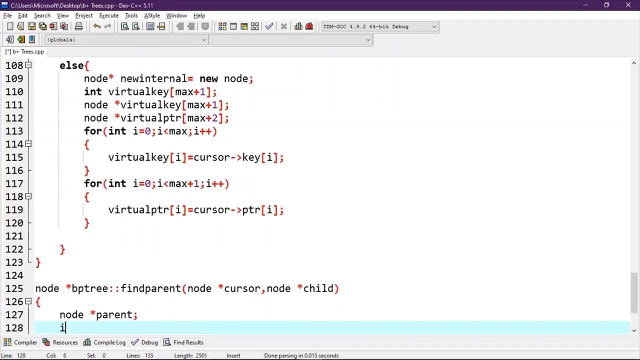 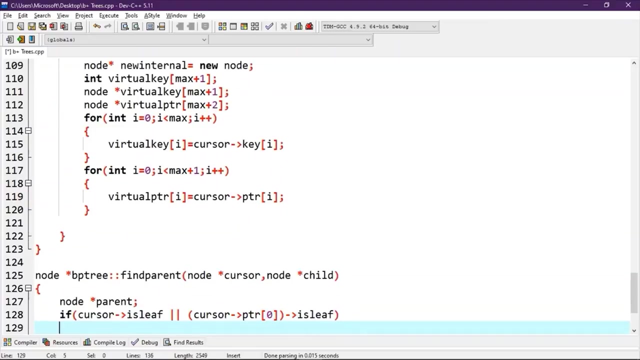 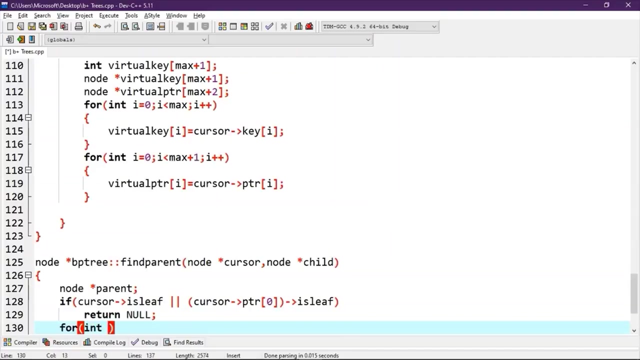 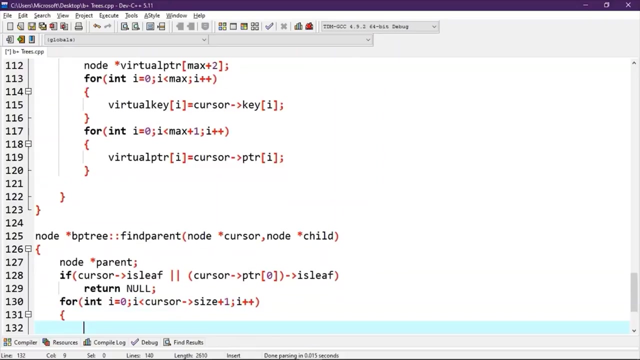 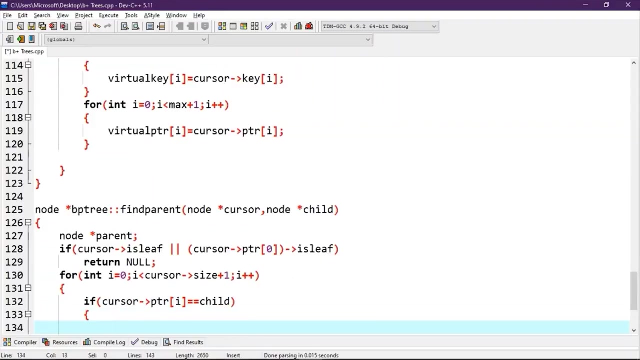 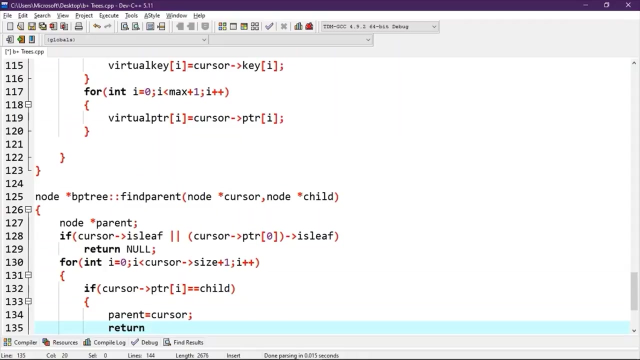 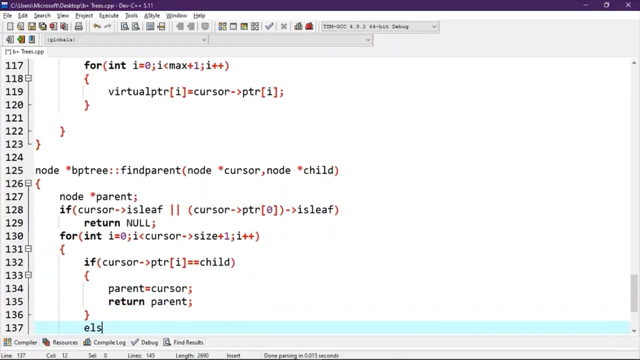 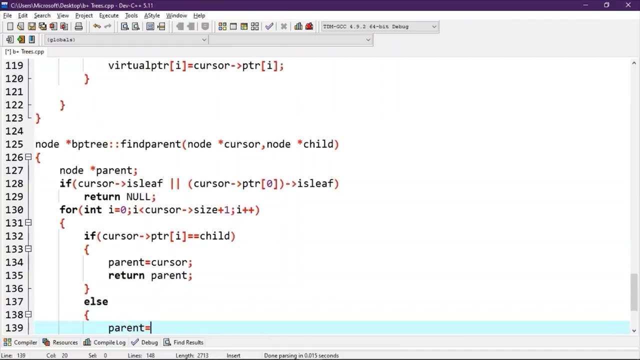 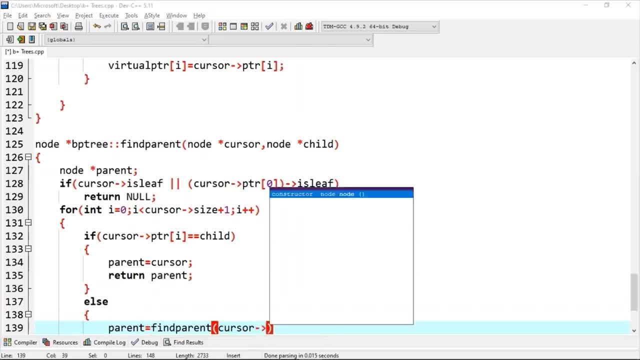 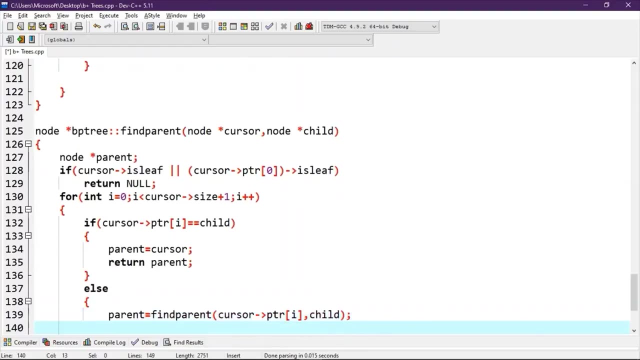 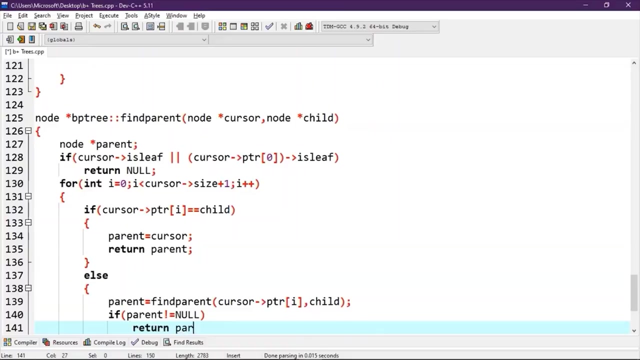 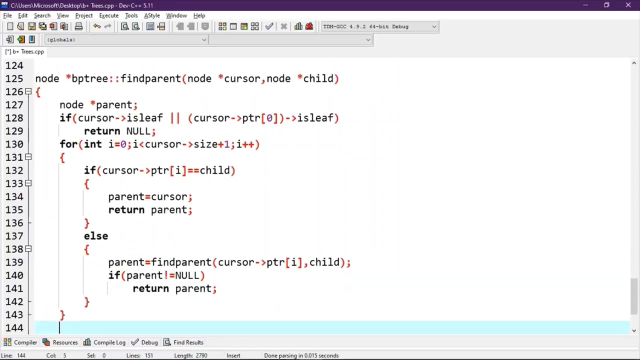 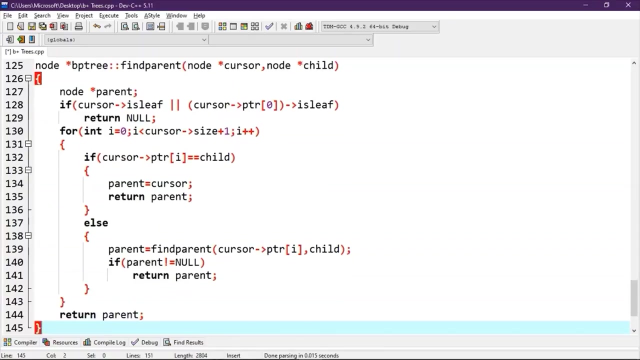 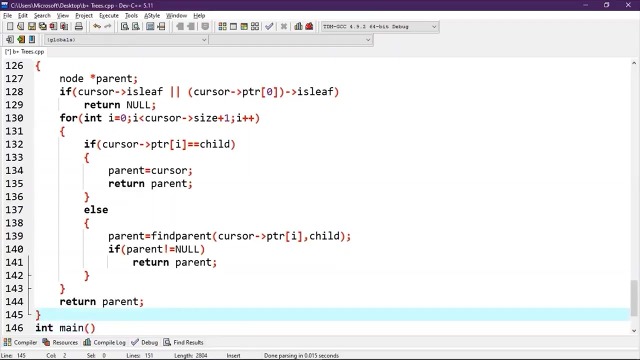 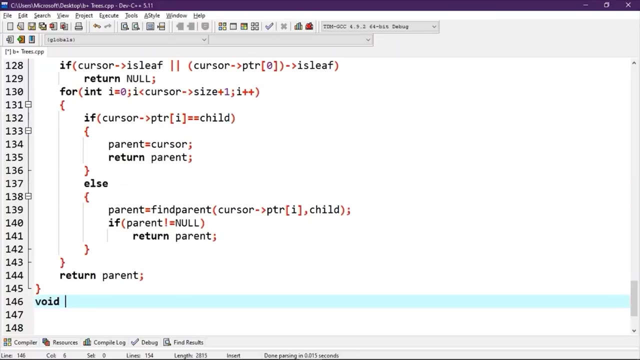 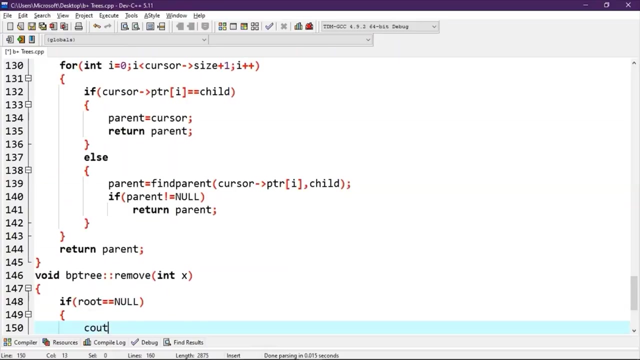 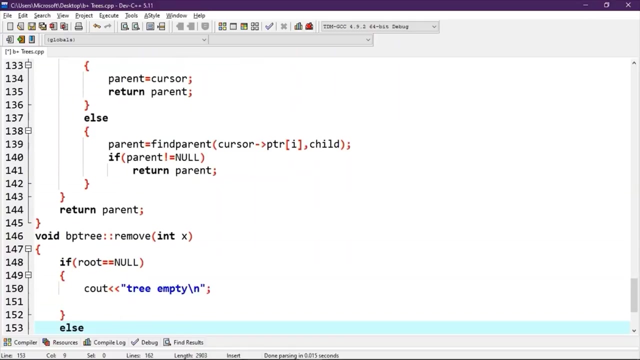 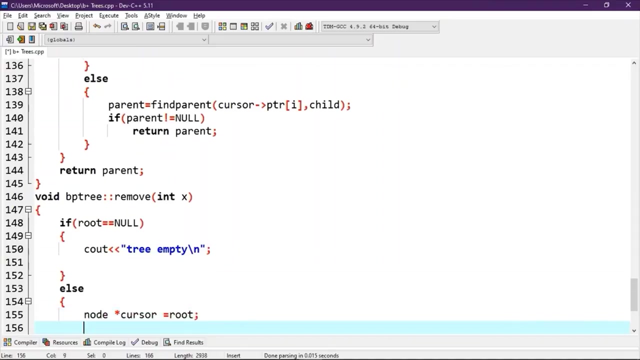 cursor PTR right. if parent not equals to null, return, return parent. now void PTR, remove PTR and x ending end, end, end. If root goes to NULL then cout is empty, else node star cursor goes to root. ok, ok, so cout, cout, so rld, ok. lecture 4: 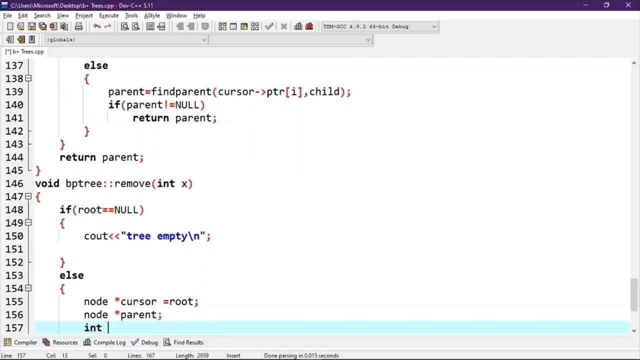 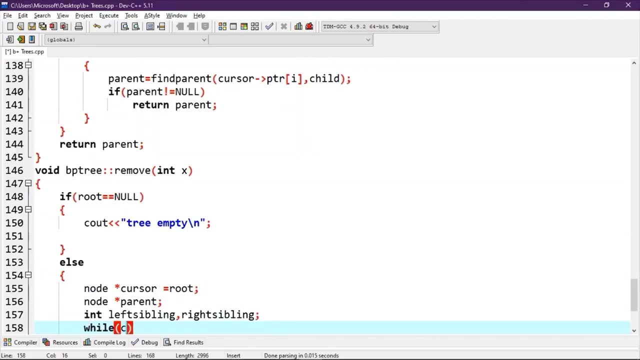 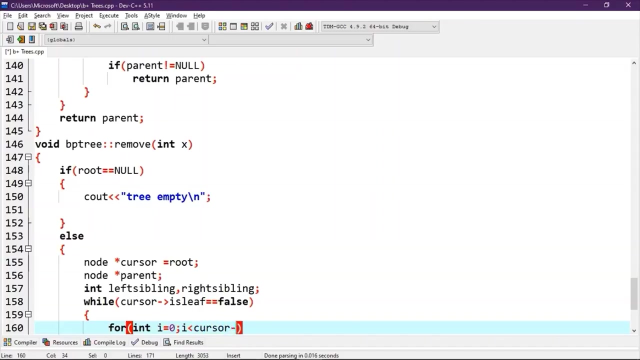 4 star parent. int char masa, moins technically so, while Cursor is leave equals to false. Cursor for int i is equals to 0, i less than cursor size and i plus plus. Cursor for int i is equals to 0, i less than cursor size and i plus plus. 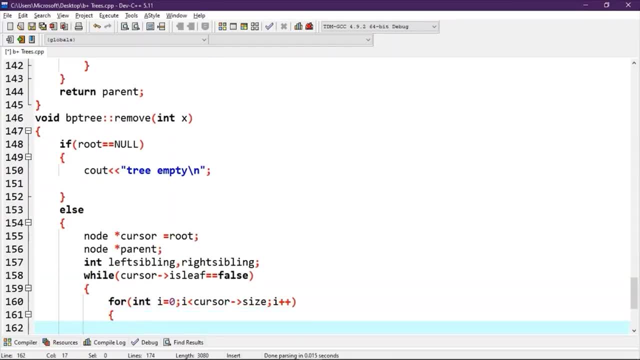 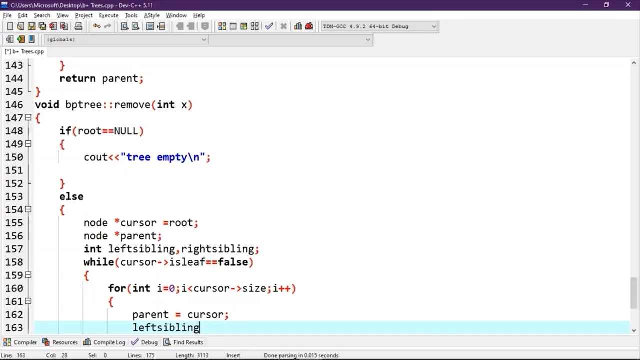 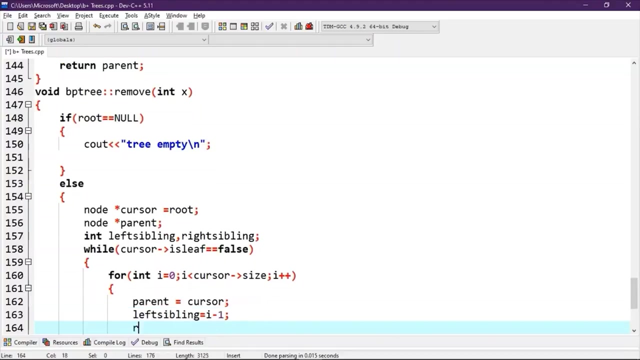 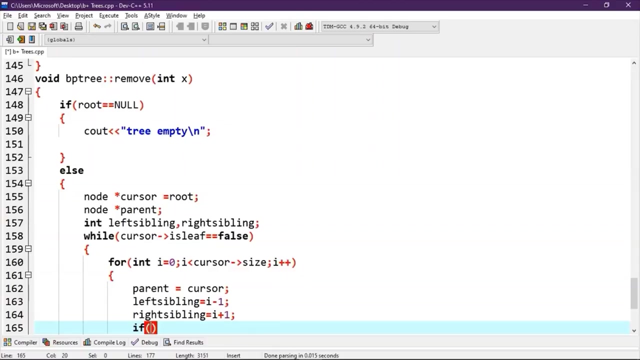 Cursor for int. i is equals to 0, i less than cursor size and i plus plus Parent is equals to cursor. left sibling is equals to i minus 1.. Right sibling is equals to i plus 1.. If x is less than cursor size. 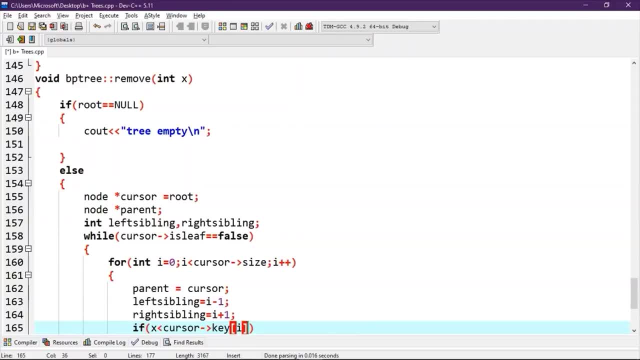 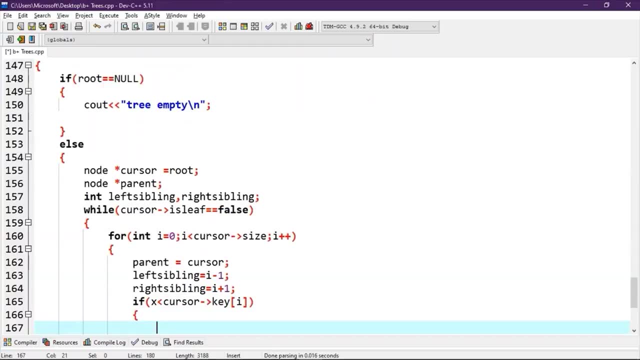 Right sibling is equals to x: 1., 2., 3., 4., 5., 6., 7., 8., 9., 10., 12., 14., 15., 16., 17.. 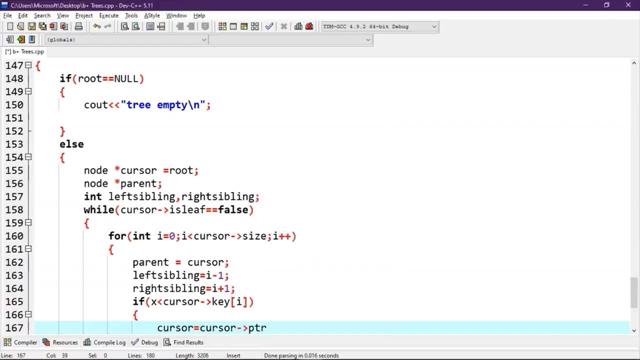 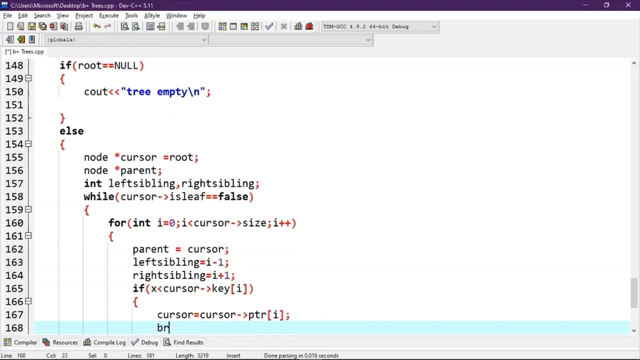 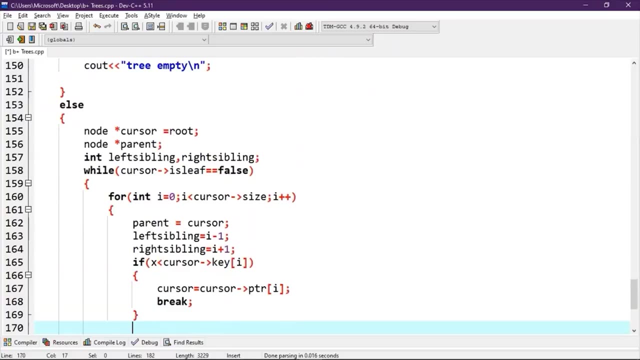 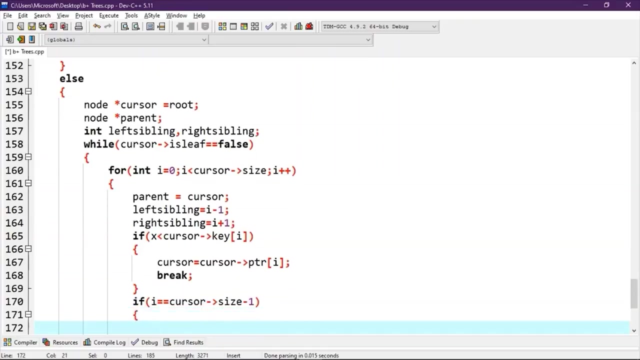 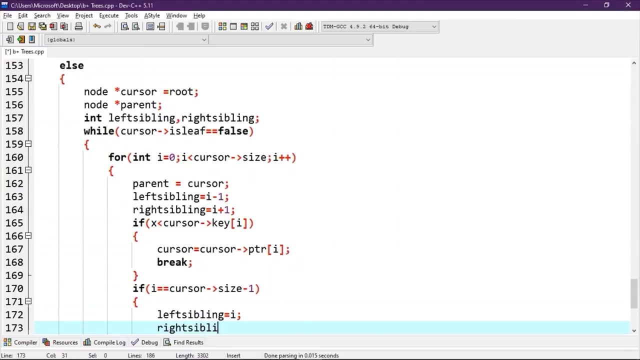 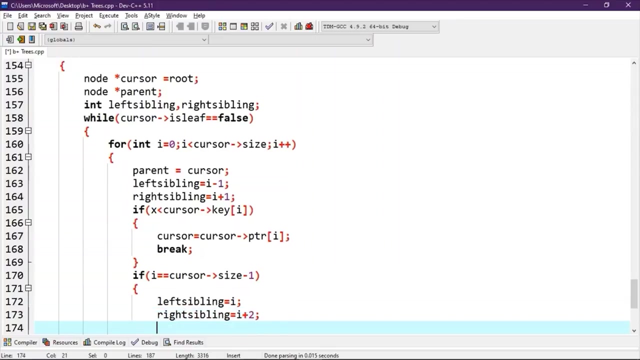 18., 22., 24., 25., 30., 31., 22., 32., 33., 54. 26.. Now, if i is equals to cursor size minus 1.. If i is equals to height, sibling equals to i plus 2, cursor is equals to cursor size. 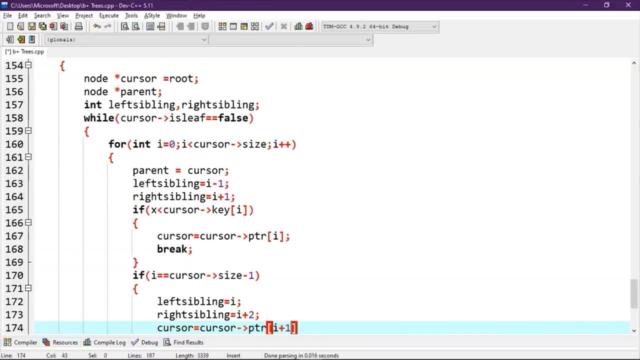 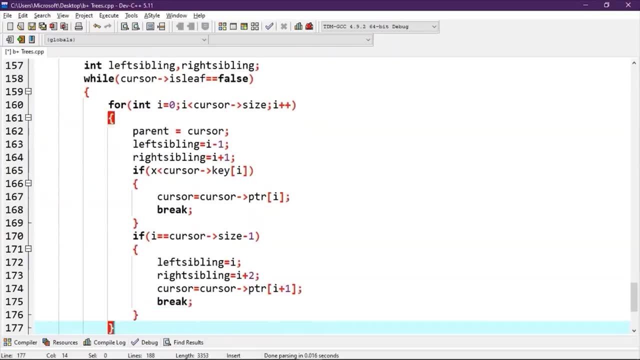 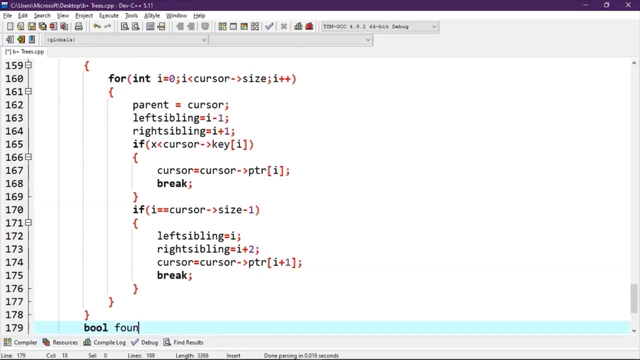 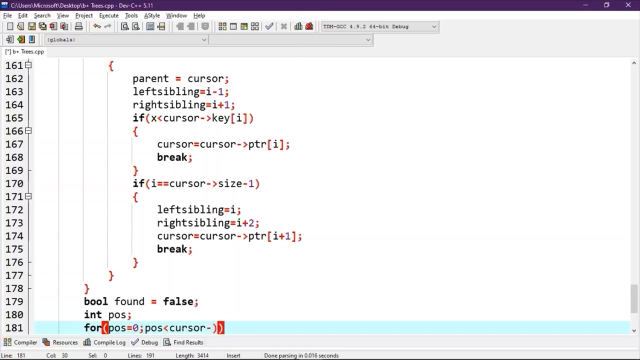 Here: Bracket height plus 1. Bracket height plus 1. Bracket height plus 1. Round is equals to false, False, False, False, False, False, False is less than cursor size. False plus plus, Plus. 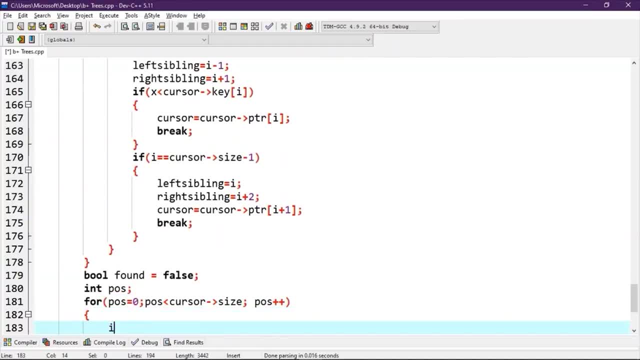 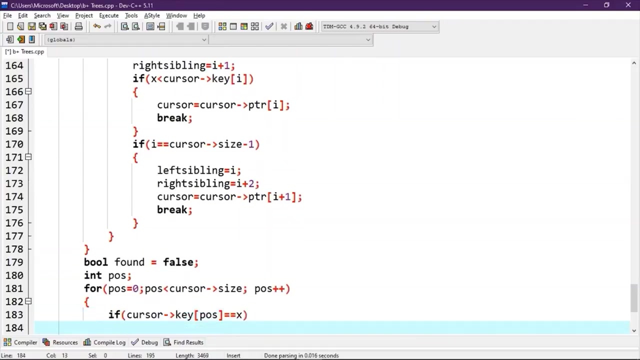 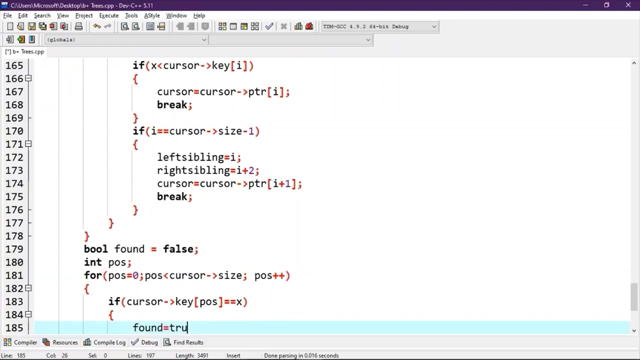 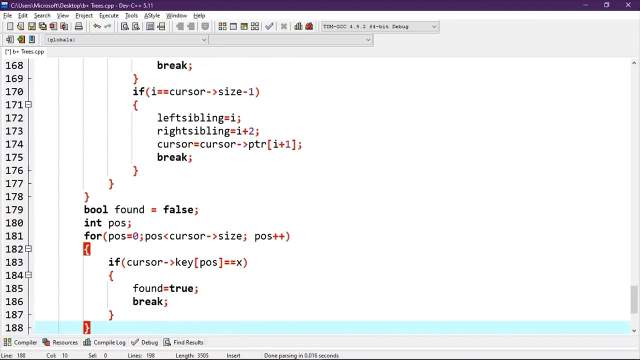 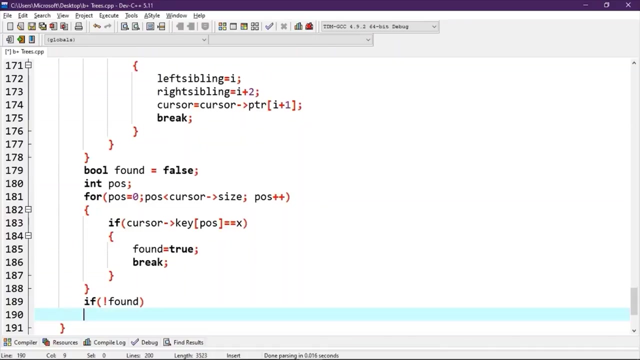 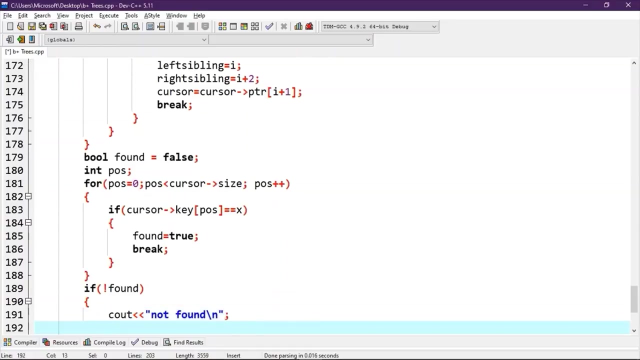 F Pressure key at force is equals to x, then found equals to true and then break Now. if not found, then be out. Not found Now, if not found, then be out Now. if not found, then be out Now. if cursor size. cursor size. 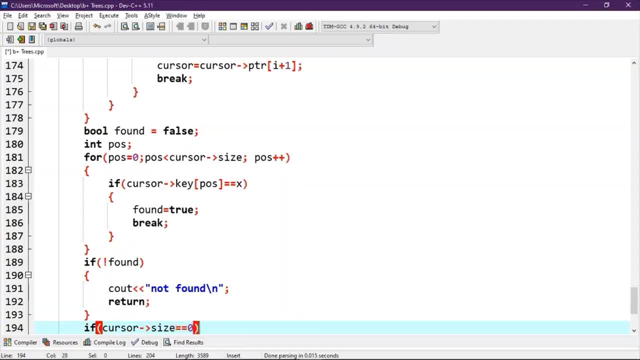 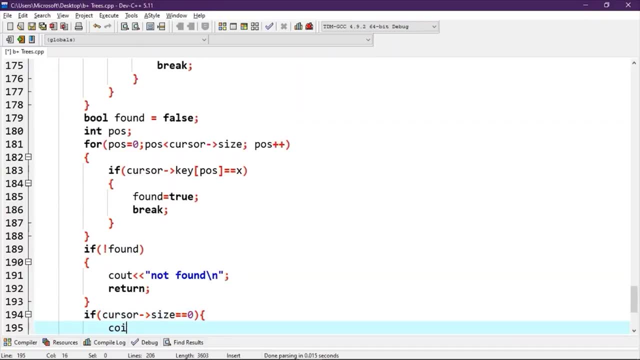 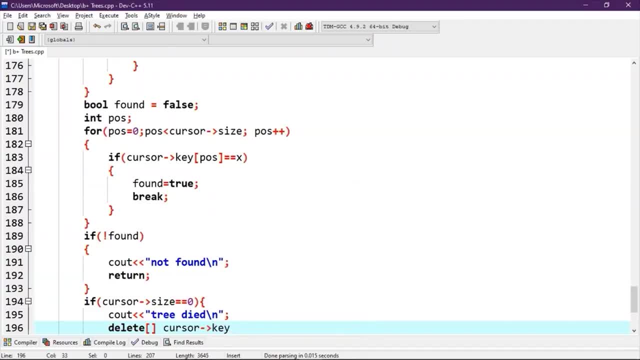 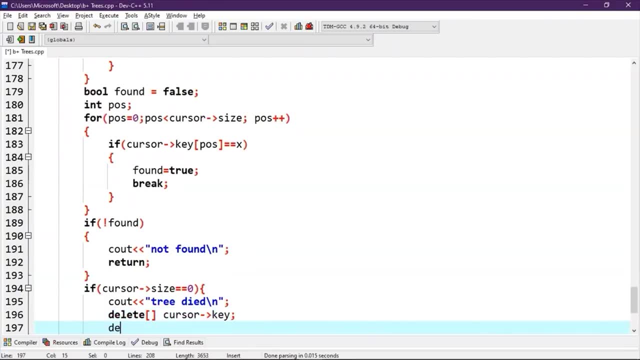 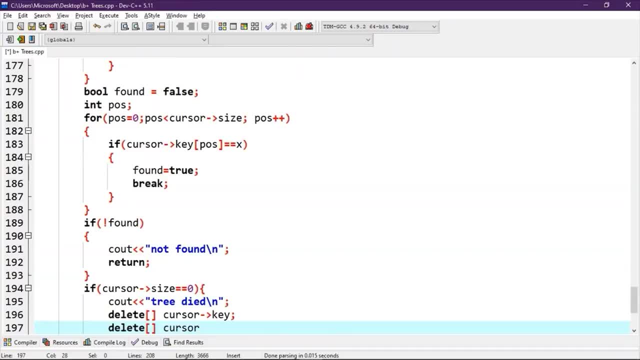 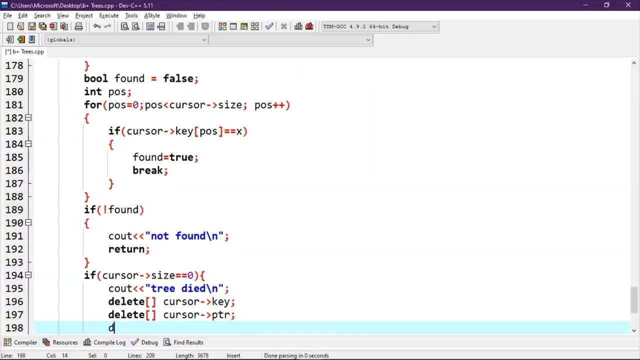 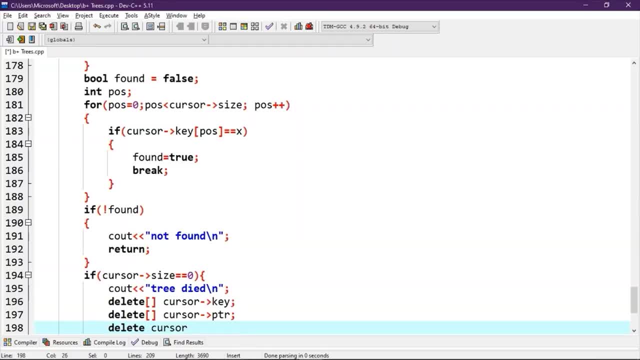 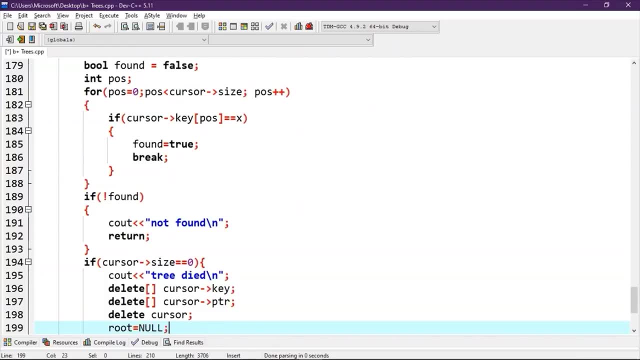 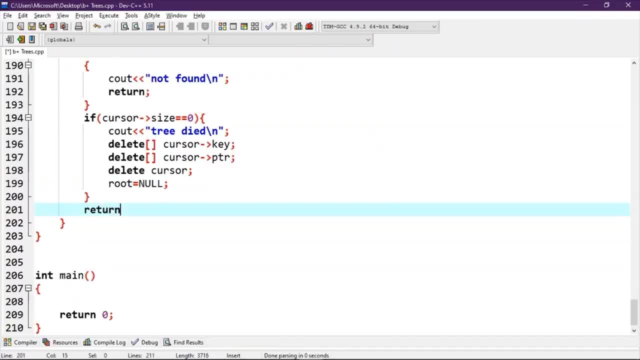 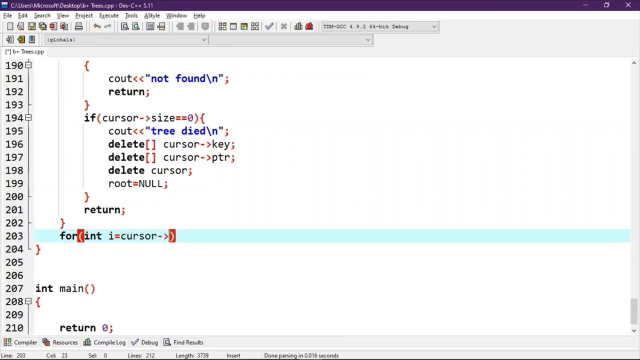 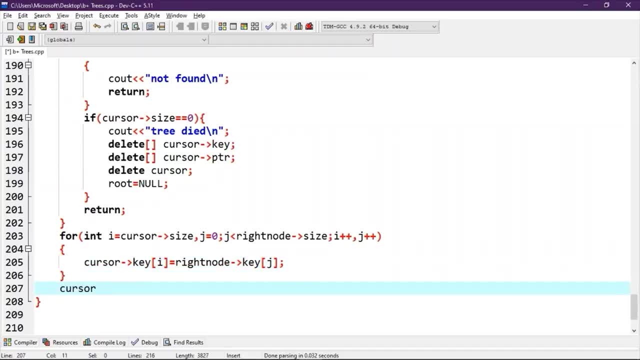 Cursor here. add cursor size is equals to null. Now c out Merging to remove internal set right sibling right minus 1, comma parent comma right node delete. 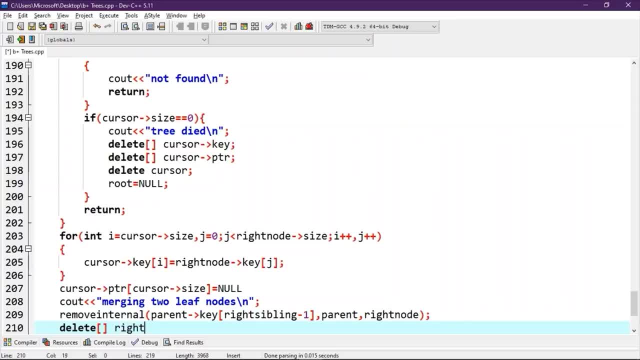 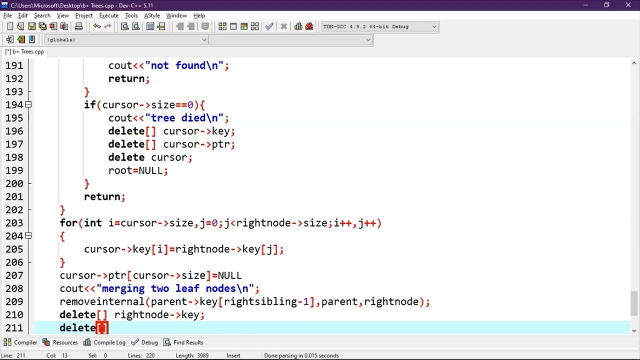 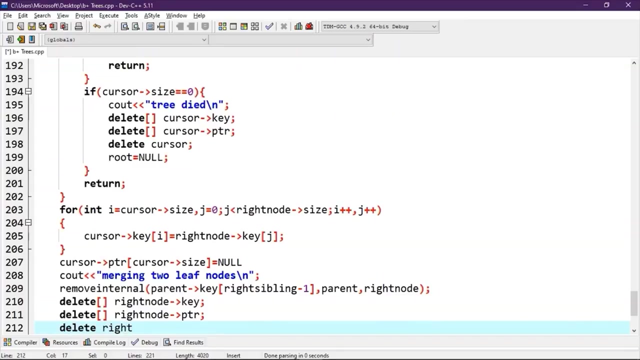 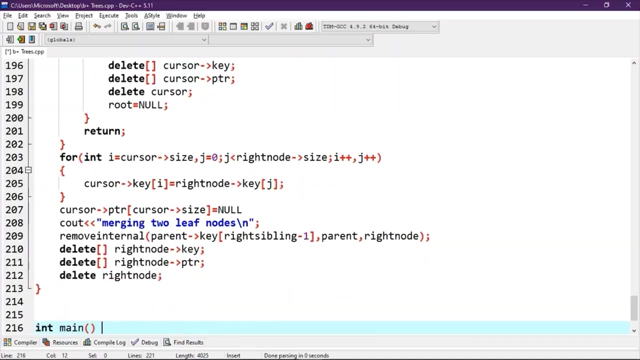 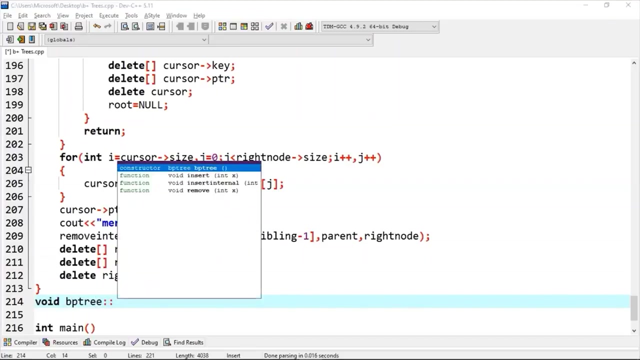 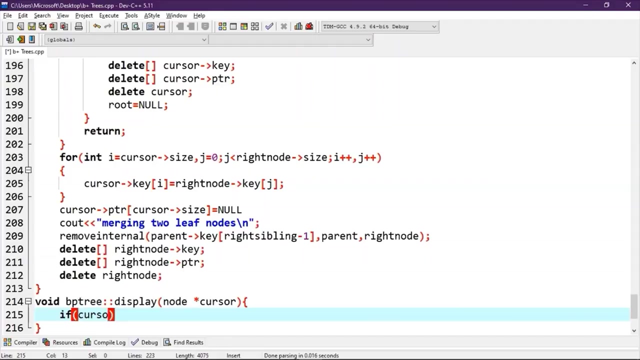 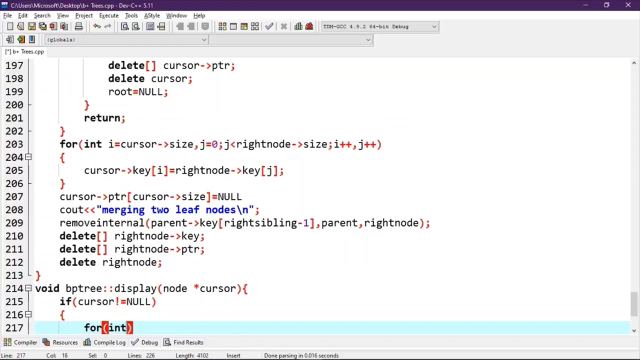 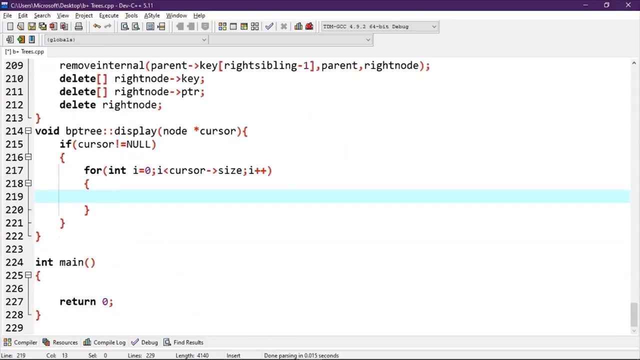 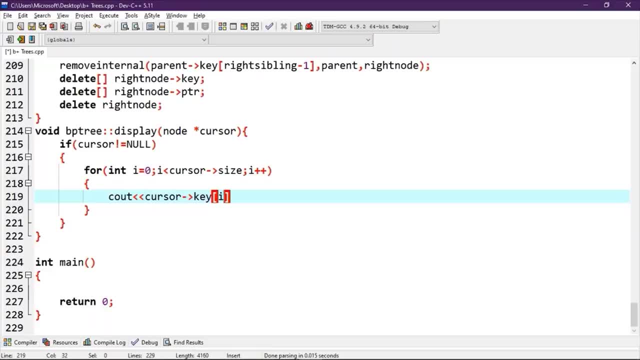 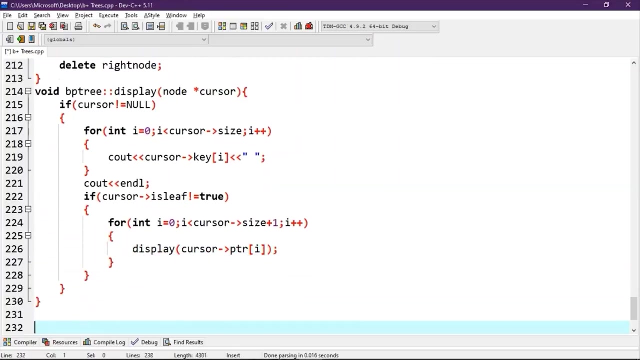 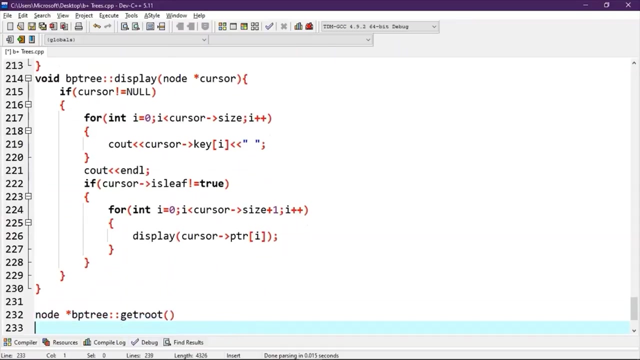 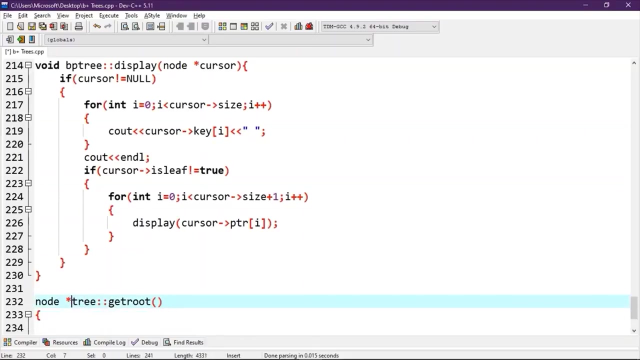 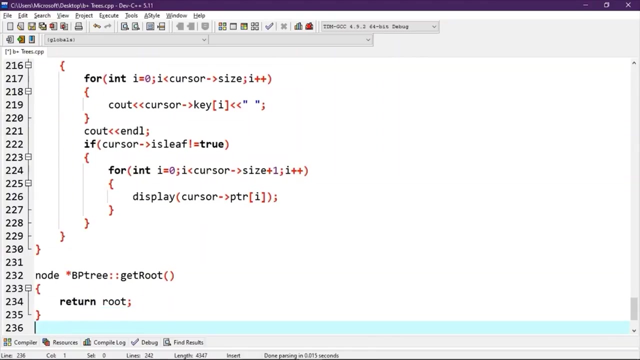 key at i. i cout, cout cc cursor. cursor is leave not equals to true and for and I equals to 0. I less than cursor eyes plus 1. a plus plus a. sir PDR, no star bp3 at root. you return root now to write the main block. 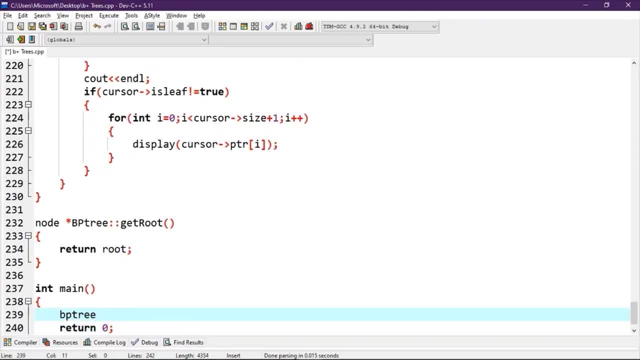 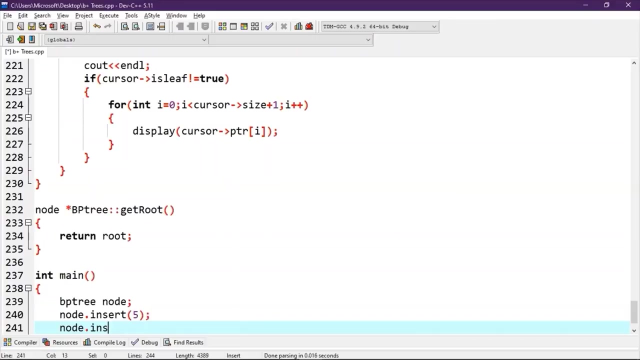 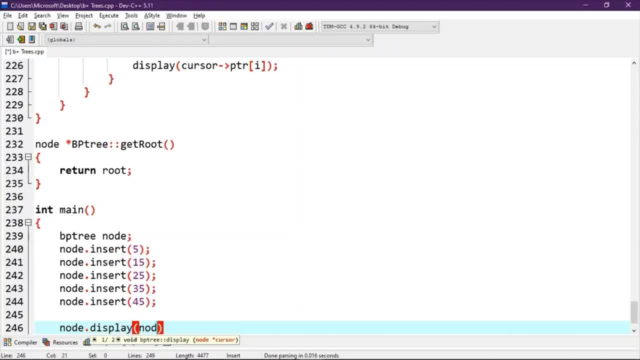 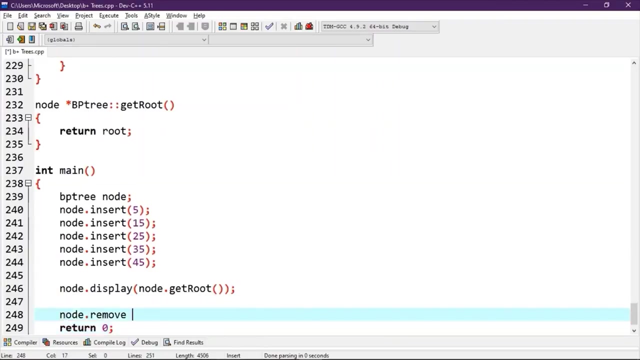